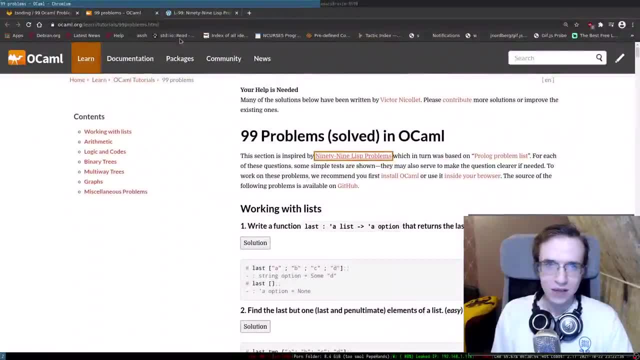 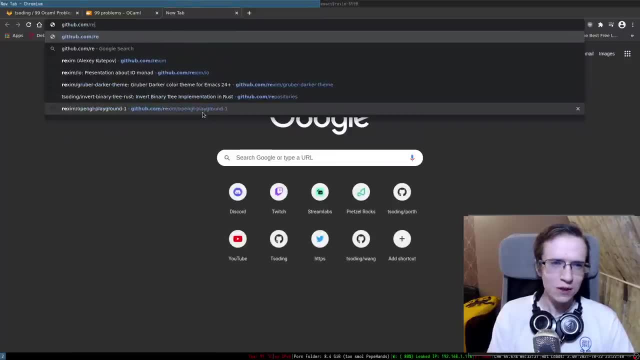 like using this set of problems Some time ago, I think, like I don't know, I think I was not already a student, I think I graduated from uni. But some time ago I already attempted to solve some of the problems And I think I still have. 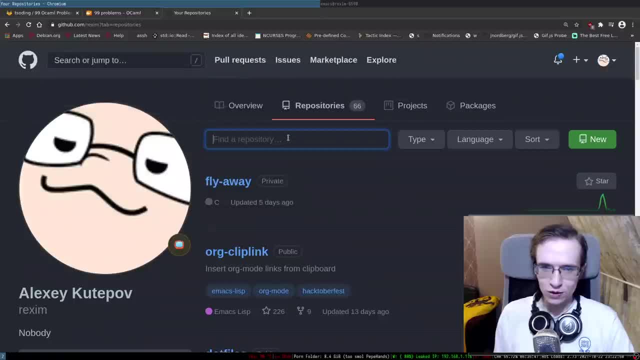 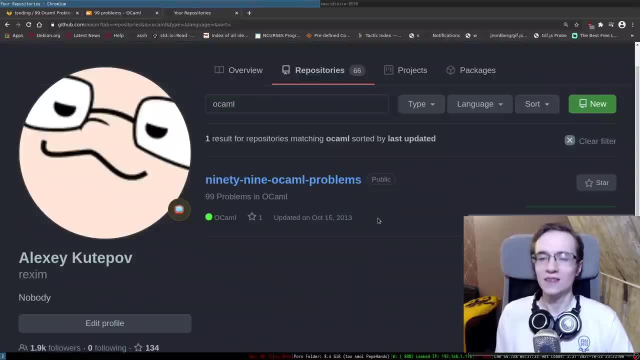 like a repo on GitHub where I tried to do that. So let's actually search for OCaml in here. Yeah, 99 OCaml problems in 2013.. Oh my god, I was a student. I was actually a student. I was in uni. 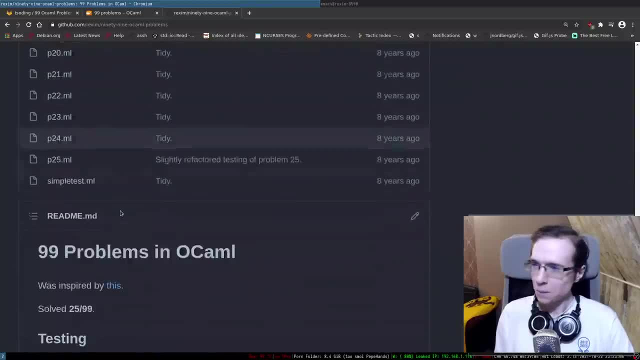 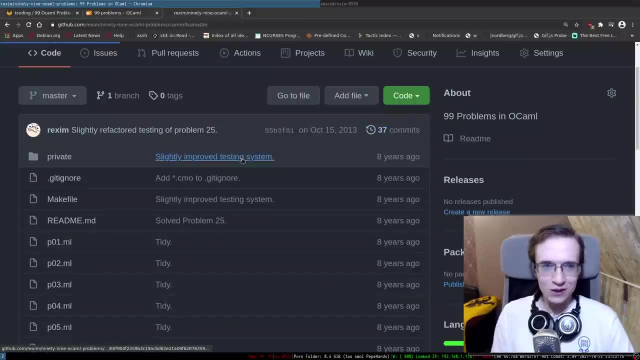 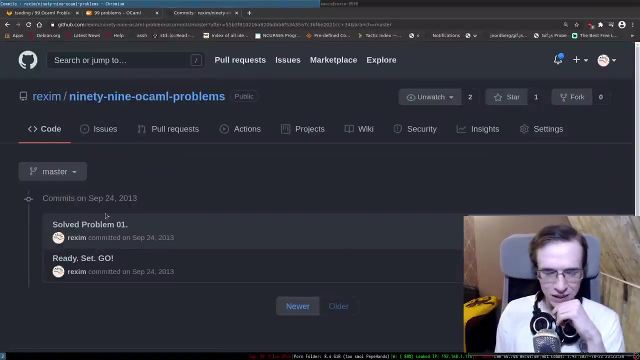 when I was trying to solve Okay, so I managed to solve like 25 of them. So, yeah, but that was long time ago, like eight years ago, And this is eight years. is the last update? right, It's the last update And I started this entire thing. Well, I mean, yeah, I basically briefly, 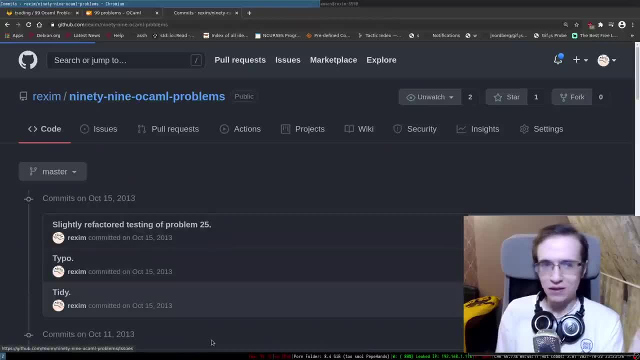 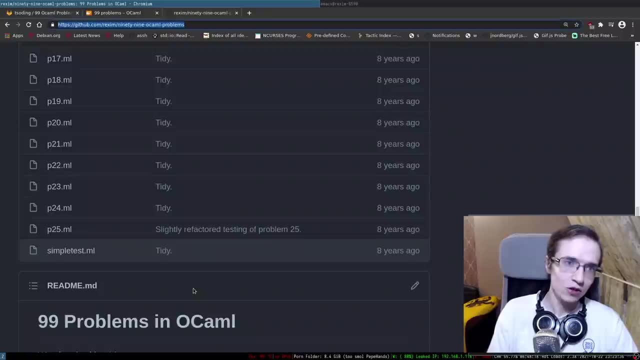 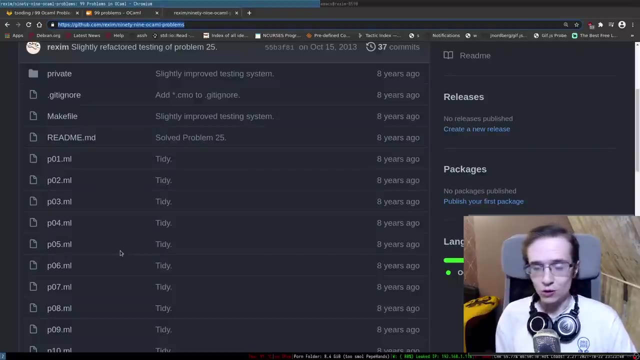 tried to solve this entire thing And I just like stopped Right. So back when I was a student, I managed to solve 25 of them. So I'm not going to look into any of these solutions And I'm going to try to attempt to solve them today with my current knowledge and see how much. 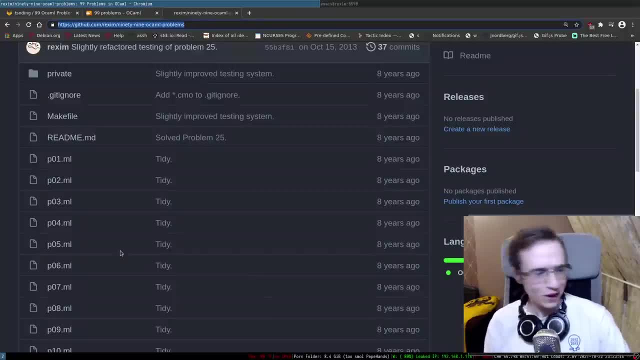 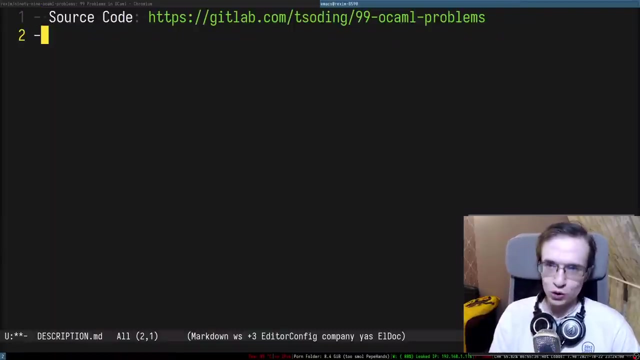 I degraded as a developer right, Because I'm getting older, I'm getting dumber, losing brain cells, So probably I won't be able to solve 25 of them today. So, yeah, I'm going to give the link to this repo in the chat And, for people who's watching on YouTube, I'm going to. 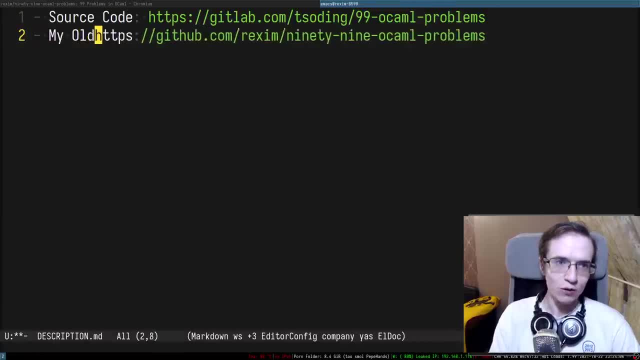 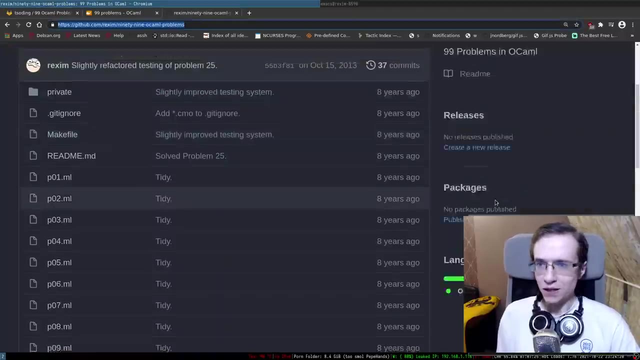 give the link in the description: my old attempts at solving these problems, right. So, but today we're going to actually start in a completely fresh and new repo. We're going to start on GitLab, because the buttons on GitHub are poo-poo. We already established that the buttons on GitHub 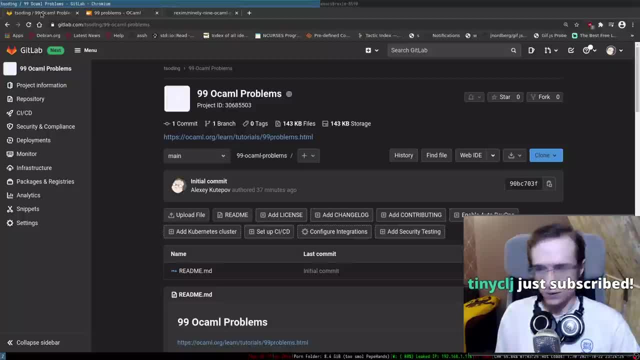 are shit And that's why we're using GitLab. So tiny CLG. Thank you, CLJ. I'm sorry for my English. I thank you so much for three months of Twitch Prime subscription. Thank you, Thank you, Thank. 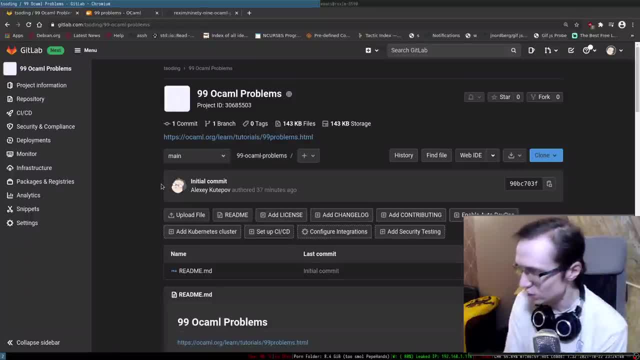 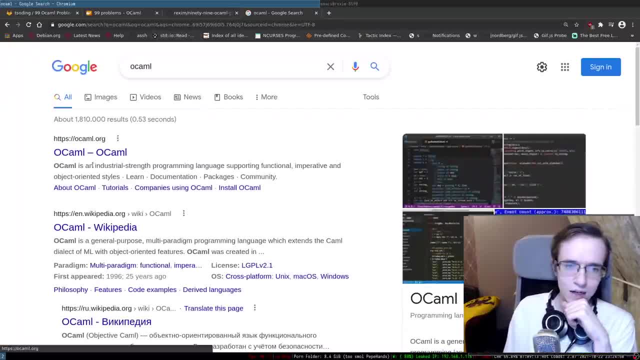 Sort of like function-ish programming language. It's more of, like, you know, multi-paradigm, because it also has OP part that nobody uses And also it has imperative parts right. So essentially it has like a seamless experience between functional programming and 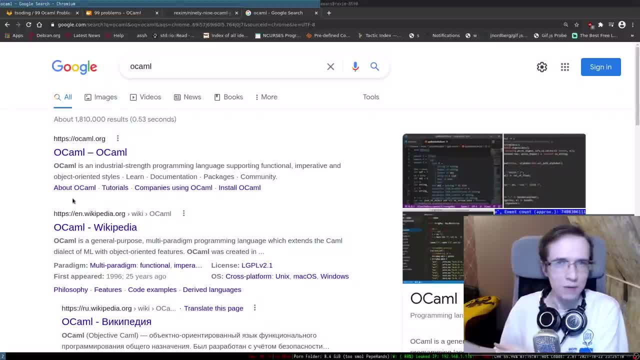 imperative programming. It also claims to have object-oriented programming, but nobody fucking uses this piece of shit, right? So everybody who programs in OCaml, they usually use the functional aspect of OCaml and imperative aspect of OCaml, right? So object-oriented programming. I think they just added it because at the time of the OCaml development there was like a huge hype around OOP. So to market the language better, they just added OOP. well, because of the time. So, and since there's already code that depends on OOP features, I presume 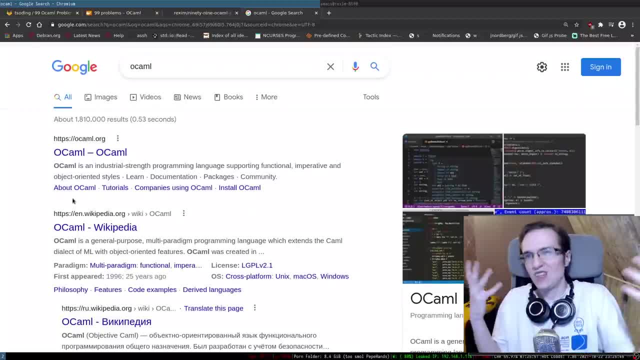 the object-orientedness of OCaml was left as a scar on the face of the language. right, You cannot really get rid of it, because there's still code that uses that, But at the same time, the new code rarely use those features. So you don't really know what to do with this shit. So it's just like 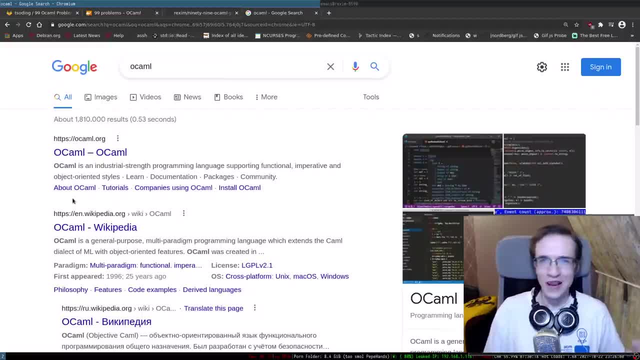 there, right? So that's what usually happens with features like that. So I presume it's purely for marketing purposes. So it's rather interesting. It's rather interesting. It feels like Haskell, but it's not lazy, right? So one of the things in OCaml is that it's 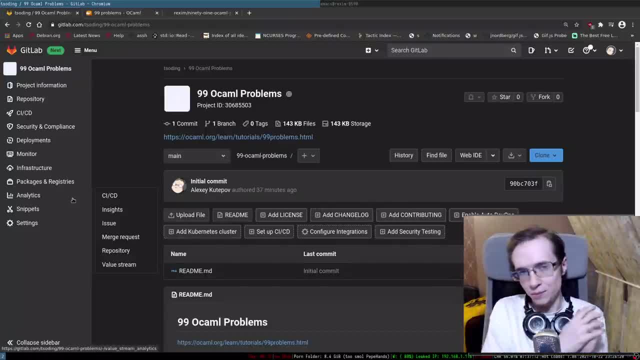 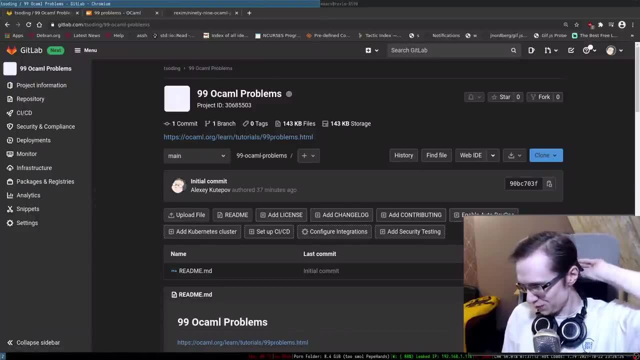 not lazy, but it has lazy evaluation, right, Just in case you need it, right? Hello, hello everyone, Hello O. underscore camel user says: OCaml is cool. Well, thank you for your unbiased opinion. Thank you so much. Yeah, I also think that OCaml is cool. So how are you guys? 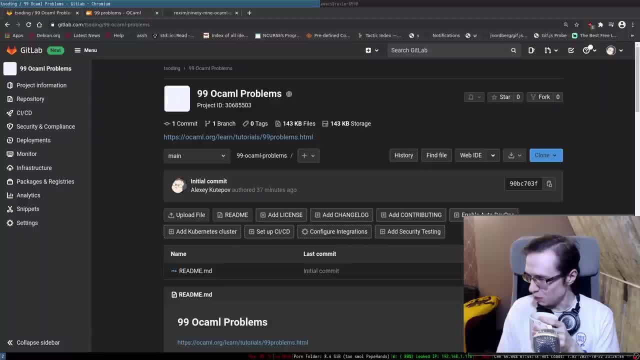 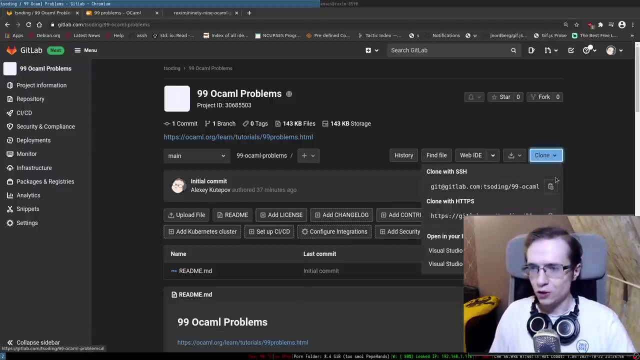 doing Hello, hello, Hello. this used Demki, Fluffy, Poga, Eddie, Popit, Chan, Crazy Chicken- so many cool names. Hello, hello, Welcome, Welcome, Welcome Cheers, by the way. Alrighty, So let's actually clone this repo And let's take a look at the problems, shall we? 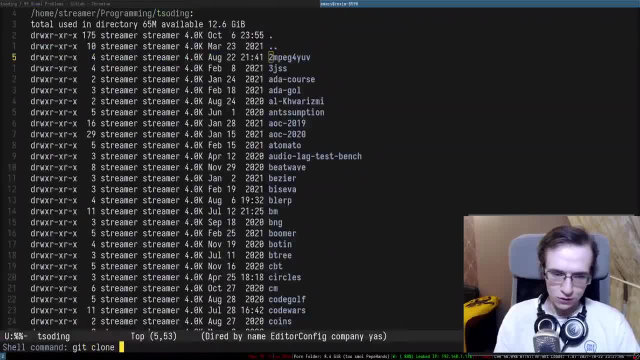 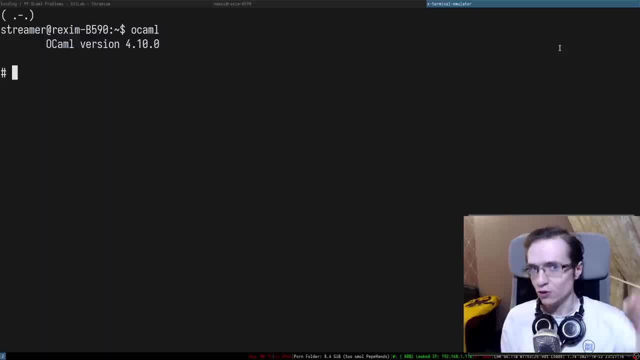 So this is a zozing and I'm going to do git clone. Do I even have OCaml installed on my machine? I do. I have OCaml 4.10.0.. I'm not sure if that's the latest OCaml, but OCaml is not Rust. You don't have to have the 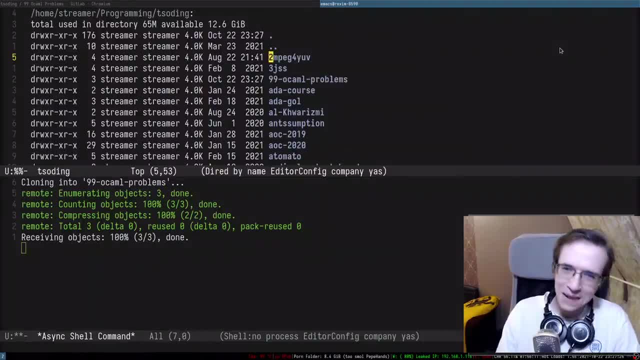 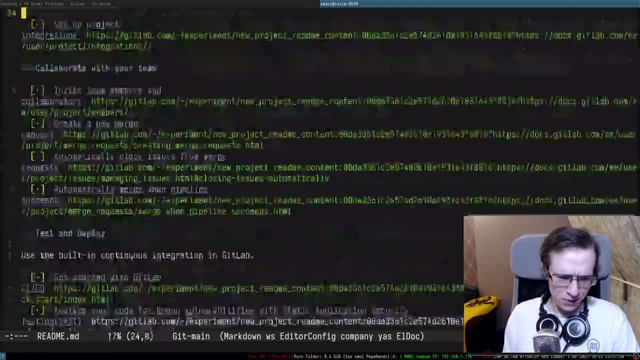 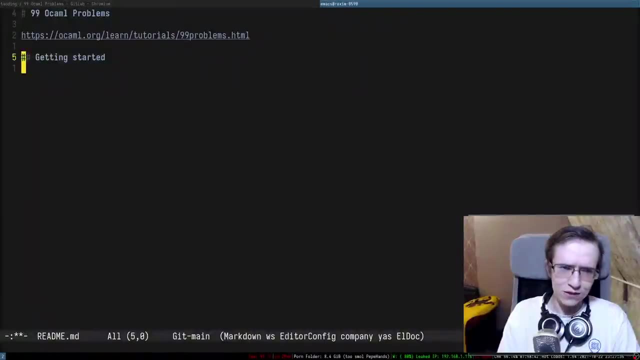 latest OCaml right, So got them All right. So we have this readme And so this is like a crap that was auto-generated by GitLab. So I think I'm going to actually remove all of that, So, at least for now. So we're only going to have this thing And, in terms of the license, I'm going to 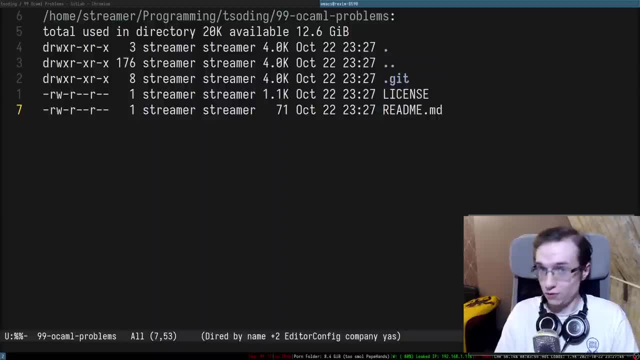 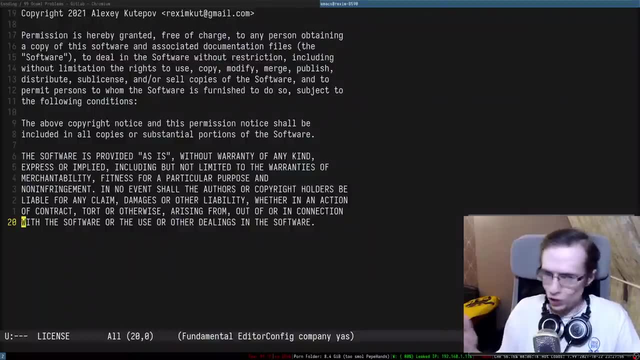 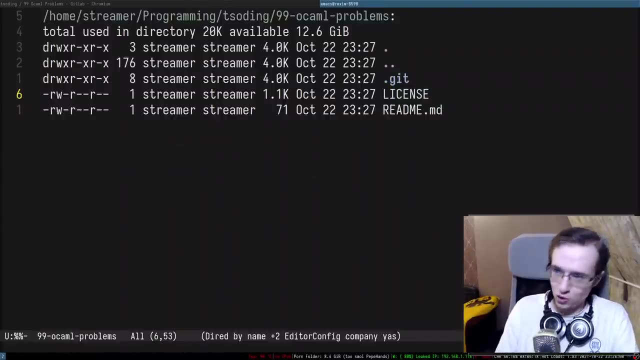 distribute all of that on the MIT license. So you can do whatever the fuck you want with it, right? Except claiming that you made this thing right. So this is basically MIT license. Do whatever you want, except claiming that you created this thing, including selling. by the way, You can make money off of the code. Just don't say 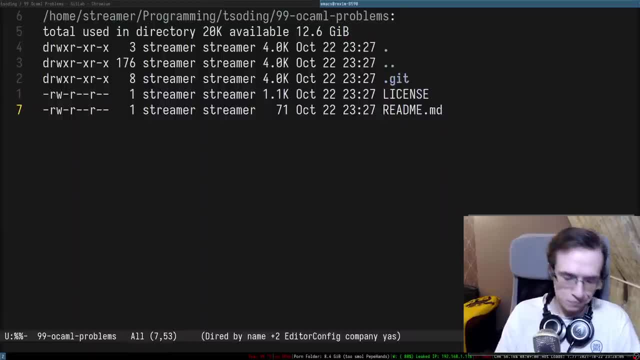 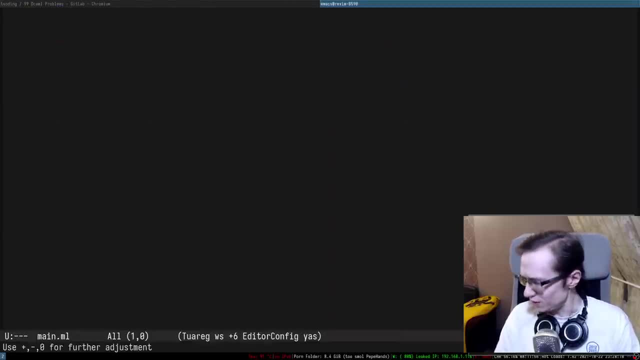 that you made it right. So this is that. So let's create a simple hello world in OCaml. Um, I wonder if I still remember how to program in this language. Well, the OCaml from eight years ago is probably the latest. So effectively, you have the latest OCaml. 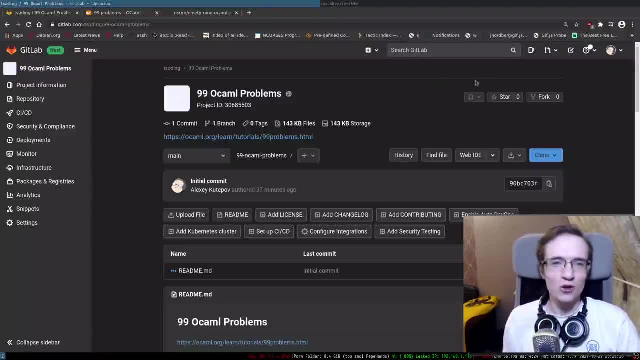 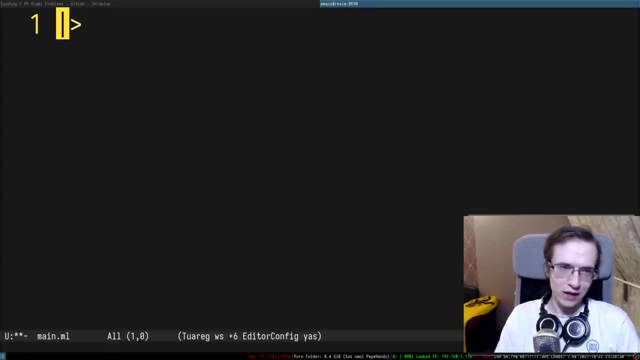 without even trying. What's funny, when I was solving this problem I think OCaml didn't even have the pipe operator right. So in the pipe operator essentially allows you to sort of pipe values through a sequence of functions and so on and so forth. I'm so fucking old I remember OCaml. 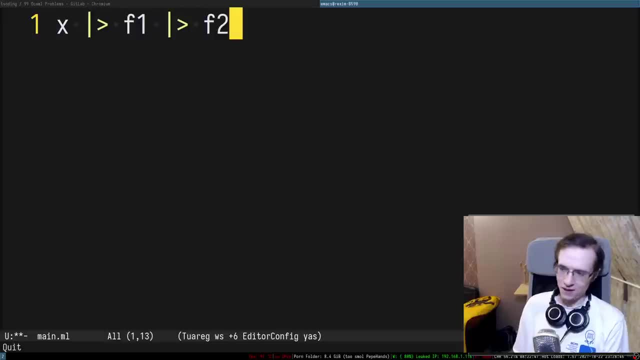 not having this operation. That's how fucking old I am. So, and I remember the time So, when I was ranting about OCaml not having this operation right And how all the other languages, all the other cool kids do have it And I have to implement that operator myself. That's how. 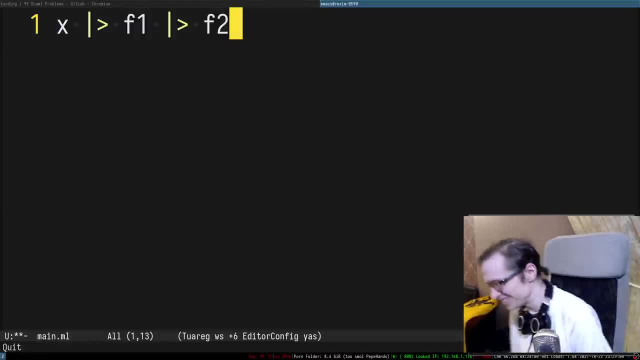 fucking old I am. Uh, so, oh shit, Boomer Zodian. Yeah, exactly, Uh, Boomer Zodian. Okay, So let's write hello world. I think you write it like this: Uh, I almost actually wrote hello world, and then 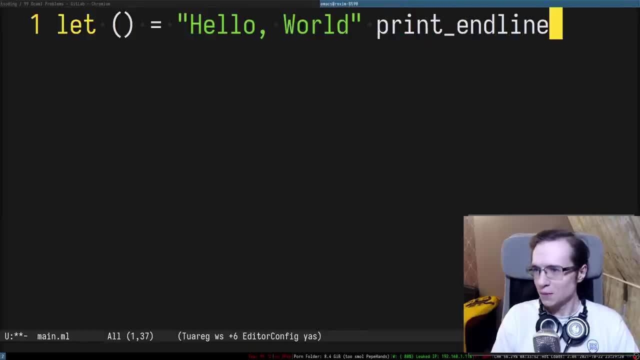 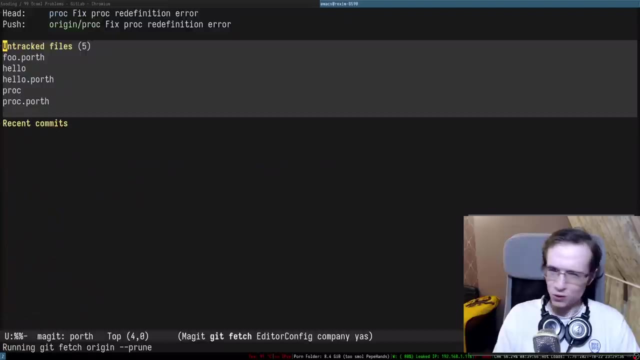 uh, print and line, because I've been programming in Porth too much lately, right, Because I'm right now I'm actively rewriting Porth in itself, And in fact, uh, right, So I think it's already like thousand lines of code or something. I don't fucking remember. Uh, so let 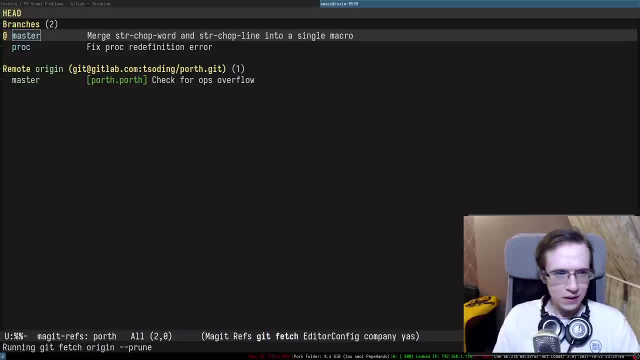 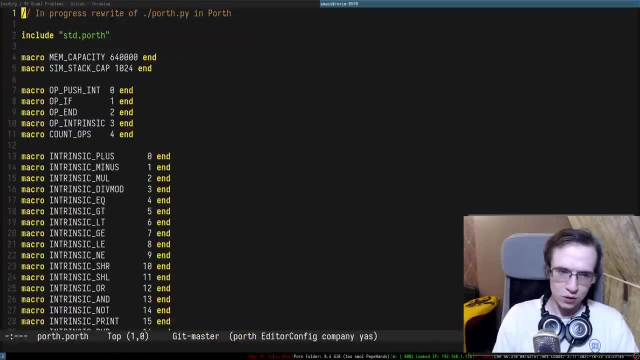 me take a look at the current state of Porth. Uh, so I'm going to fetch the latest shite and uh, take a look at the Porth, Porth, Porth, uh, dot Porth. So here's the current state of Porth. As you can see, I already added all of 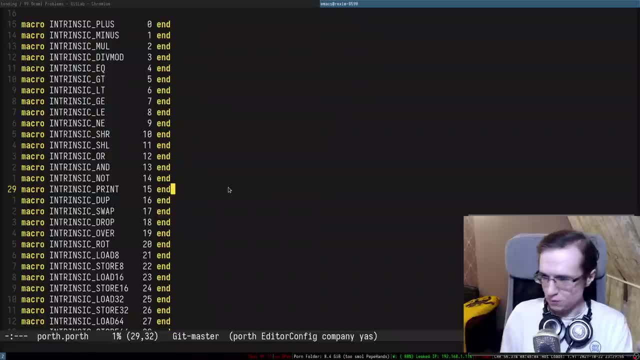 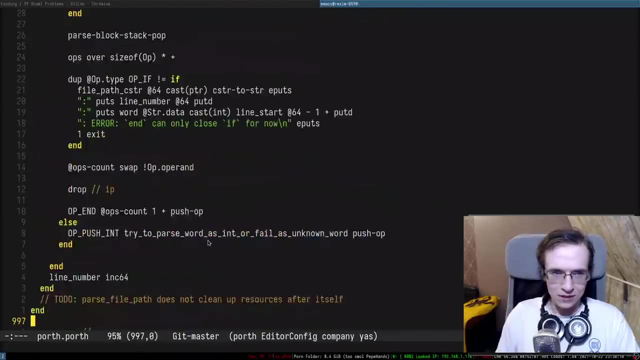 the intrinsics. uh, adding all of the intrinsics was relatively simple because we already have implementations for them in Python, So I just had to click, copy paste them into Porth Um, right, So? and the current size is 1,064 lines of code. right, So, and that's basically the current state. 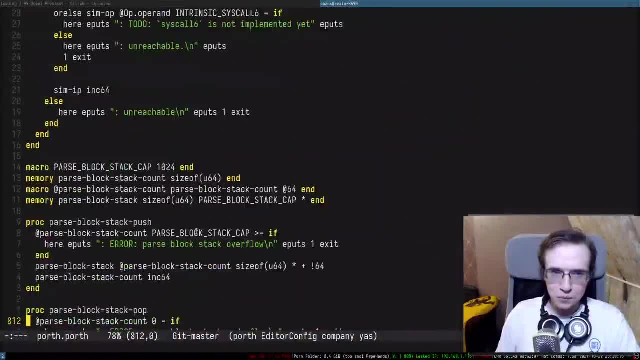 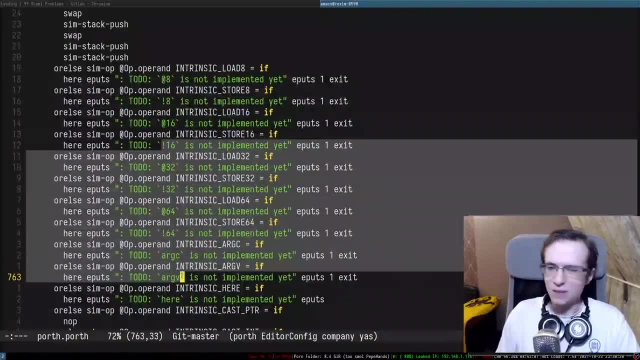 So here is the parsing of all of the intrinsics. Um, right, So here we have Porth in uh, Porth um, and I'm going to do a simple uh simulation. So the interpretation for some of them is not implemented because it may require, like a simulating, memory management. So 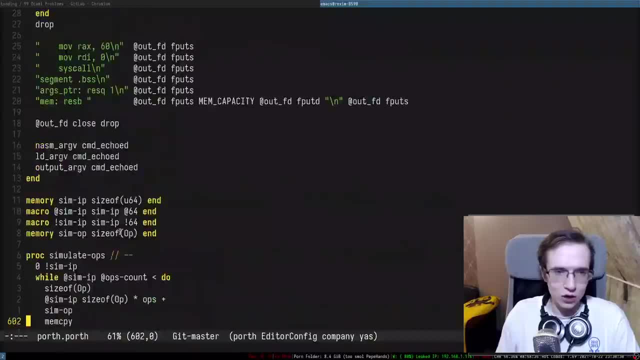 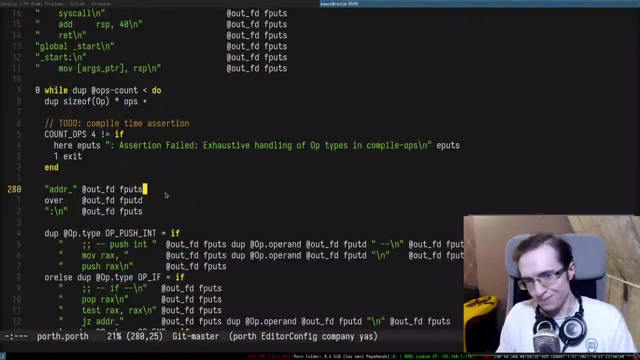 and I didn't come around to actually do that, but simulation for the rest of the things is actually there. So you see, we have a simulated stack and we're basically simulating this. instructions and also compilation, for all of the intrinsics is pretty much there, right? So here's the compilation. 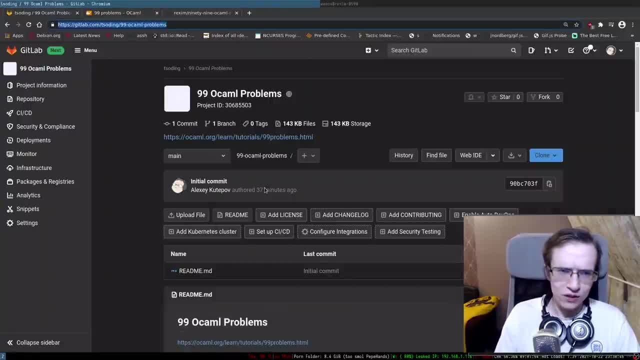 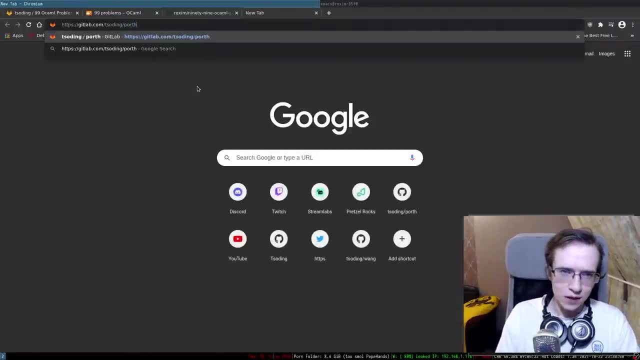 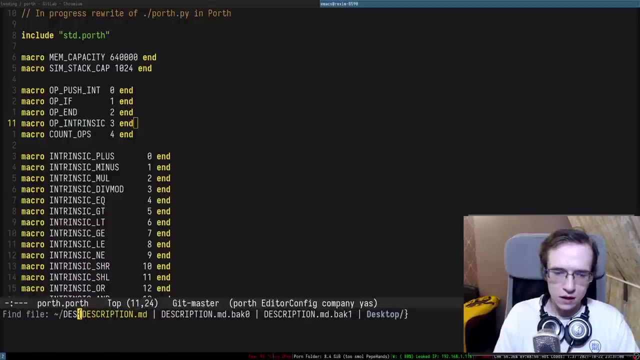 and all of that works actually. So all of that works. Uh, language that I'm developing from time to time on this channel. I'm gonna give the link to the source code in the chat for people who just joined and for people who's watching on YouTube. I'm gonna put this thing in here, my 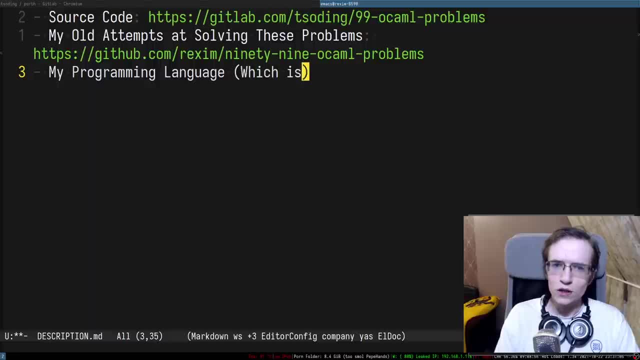 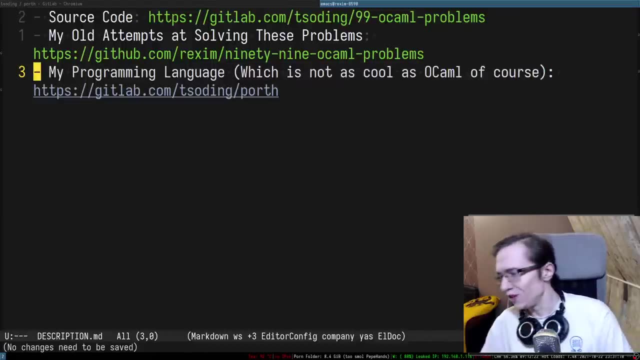 programming language which is not as cool as OCaml, of course, right. My language doesn't have OP, right? so which makes OCaml even cooler than my language. Okay, so yeah, what I want you to do, I want you to implement Hello World. 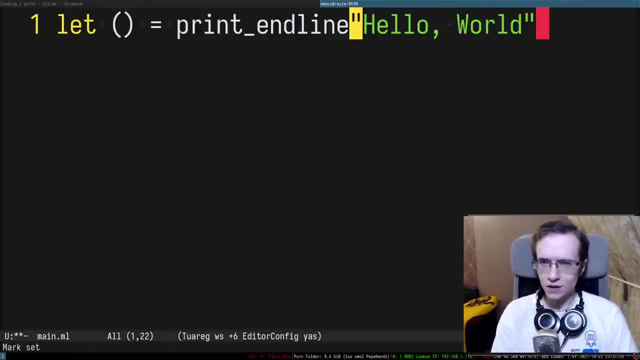 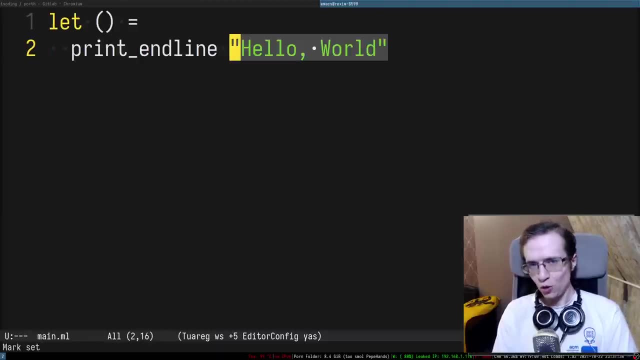 If I remember correctly, you implement it like this. so you call functions in OCaml without any parentheses. so it's almost like Porth, but the other way around. you see, So in Porth I would first put the string literally like this: 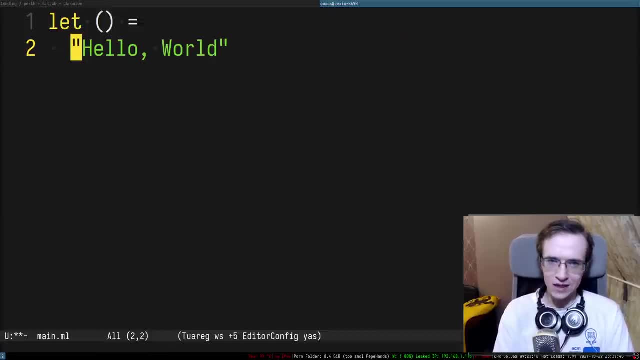 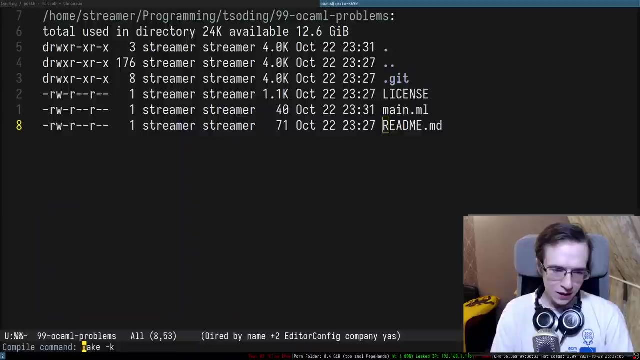 and then the function. In a camel, I first put the function and then the string literal, So basically it's pretty much the same thing. All right, Let's see if this thing is going to work. As far as I know, you can interpret a camel right, So let's actually do all of that in. 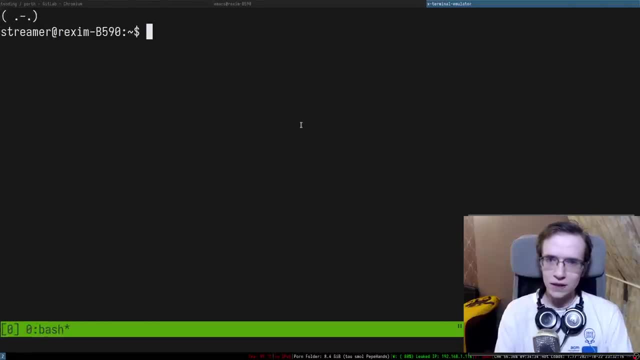 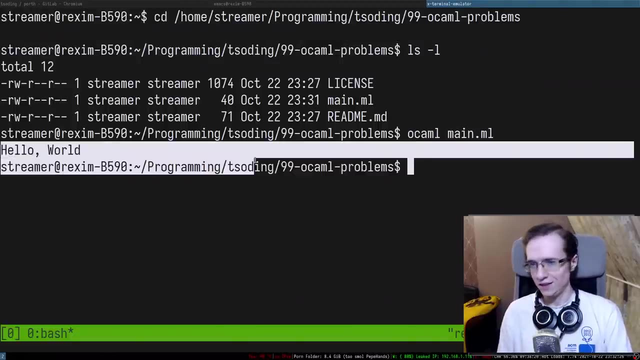 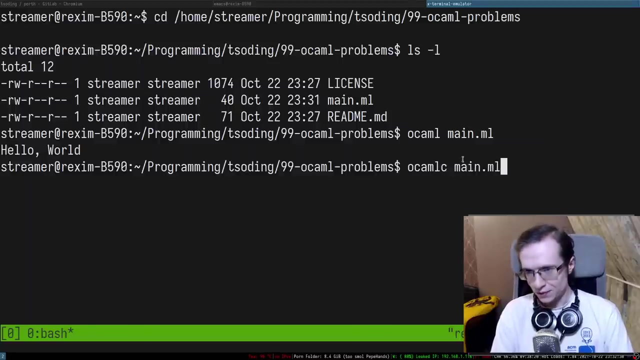 the terminal And let's go to this folder. So if you do OCaml mainml, it will just straight up interpret this entire thing. Nothing particularly special. But OCaml has a compiler called OCamlC, right, And what it does? it compiles OCaml into an executable. 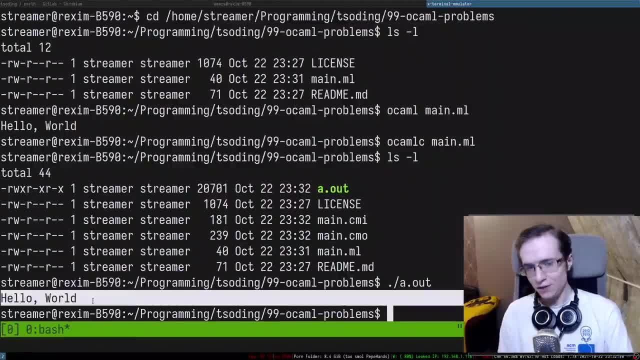 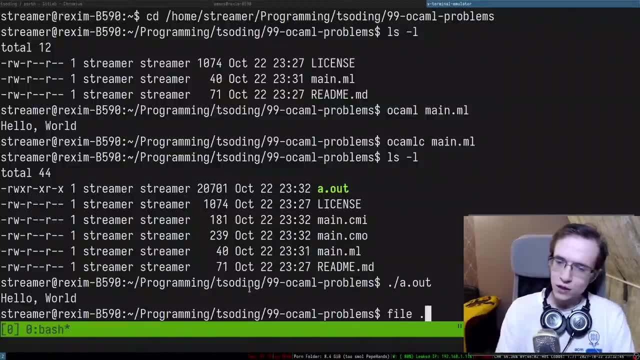 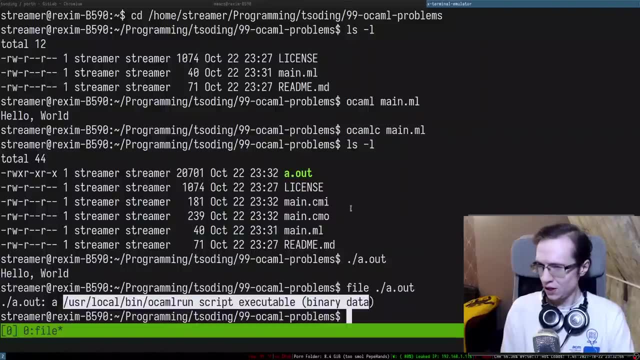 Which you can run, like so, And, as you can see, it says hello world. But you know, what's interesting is that you may think that, okay, it's a native executable, probably. But let's actually confirm, Is that a native executable? It's a OCaml run script, This mother flipper. instead of generating, 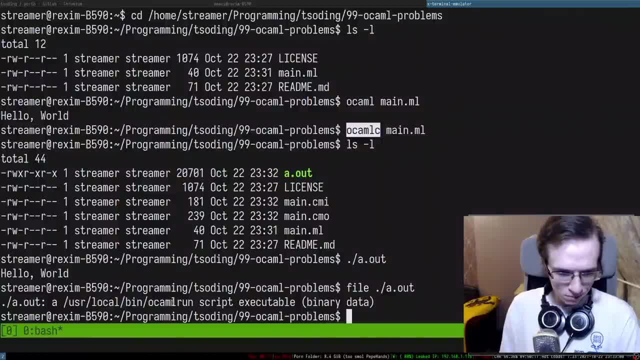 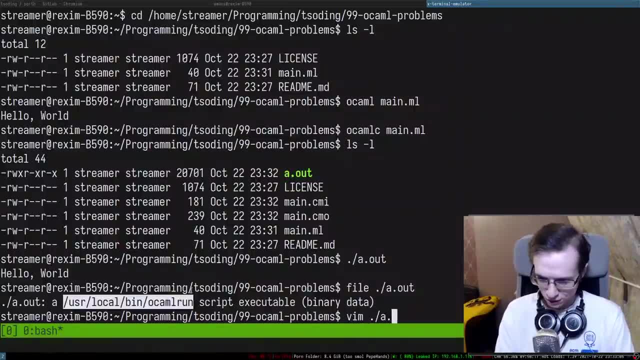 a native code, just jebaited us and generated some sort of a freaking script. The fuck. Okay, Let's take a look. Let's take a look inside of this thing. That's a funky looking script. Look at that. 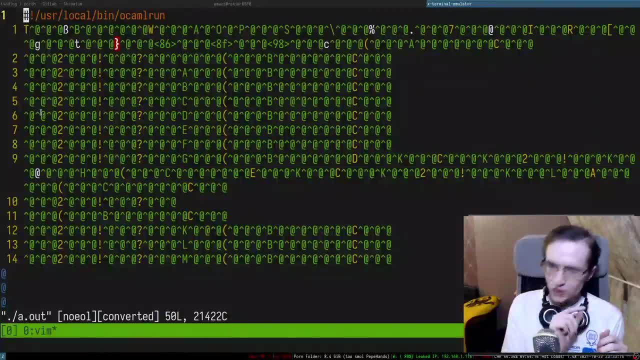 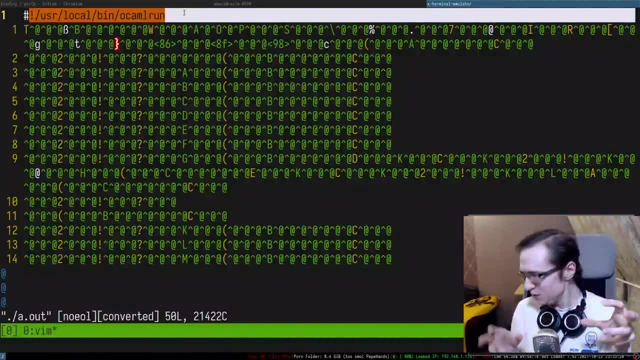 So essentially it didn't really generate a script, It generated a bytecode. But here's the trick: It basically wrapped it into a shebang. So have you ever seen a bytecode binary with a shebang Like I don't know? Like the only place where I saw this shit like that is in OCaml Does. 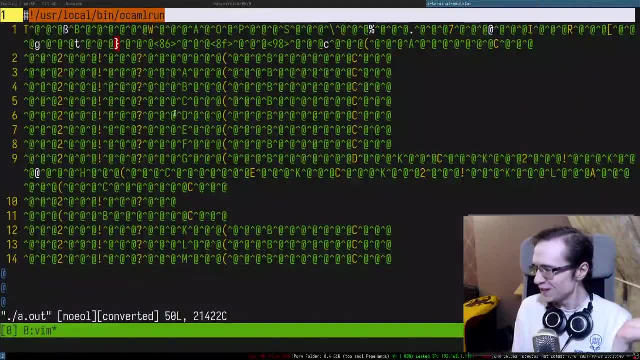 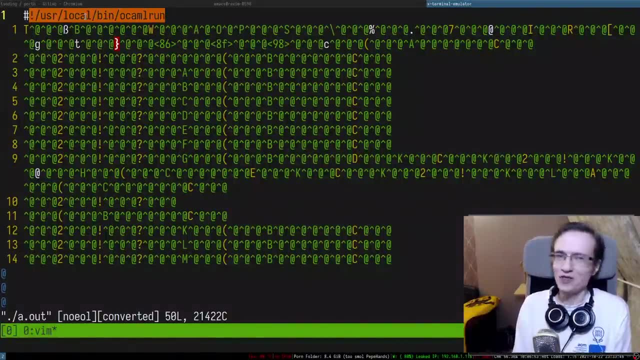 anyone know anyone else doing this kind of trick, Right, Because I've never seen it like anywhere except in OCaml. I mean, bytecode is fine, but it's just kind of an interesting idea. I mean, it works- It's actually five head. I do agree with that, But I would never think about doing it like that. So 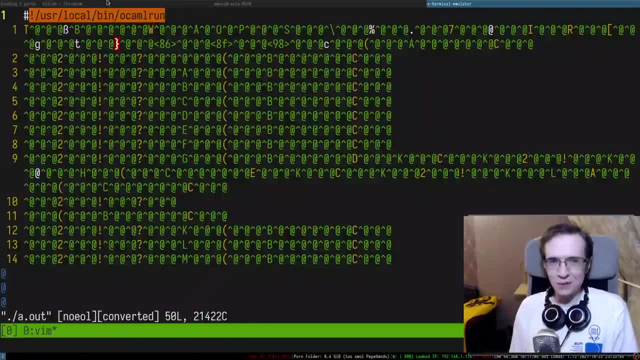 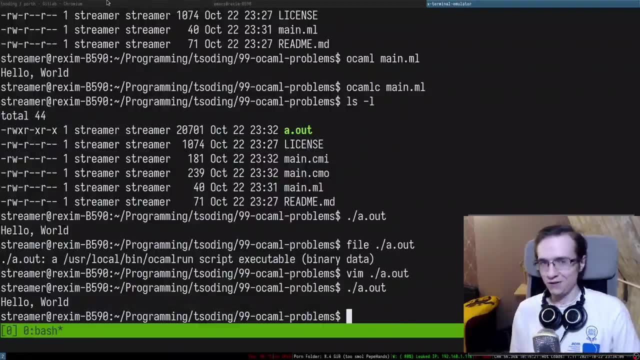 it's kind of cool. So it's a really big brain Right. It kind of looks like a native executable and you can run it as an active executable, But it's not an elf. It's not an elf executable. It's actually like a shebang script. What's interesting is, though, it doesn't mean that 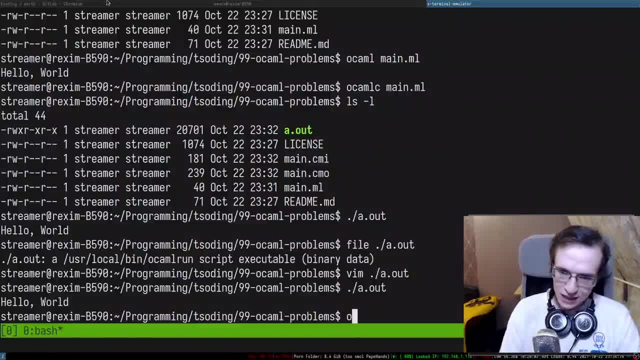 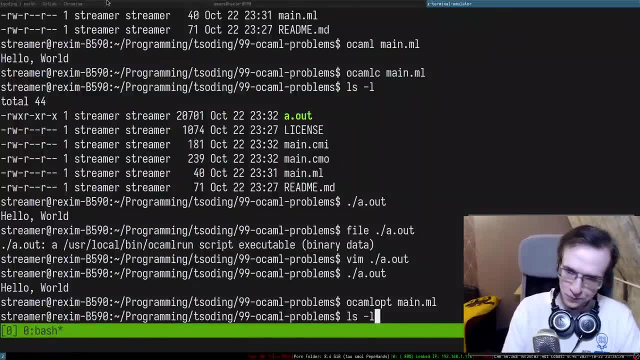 OCaml is incapable of doing native stuff, So for native stuff it has a separate compiler called OCaml OPT Right, And if you try to use OCaml OPT right, it will generate this thing again And, as you can see, this thing is a little bit beefier than it was before, Before it was 20. 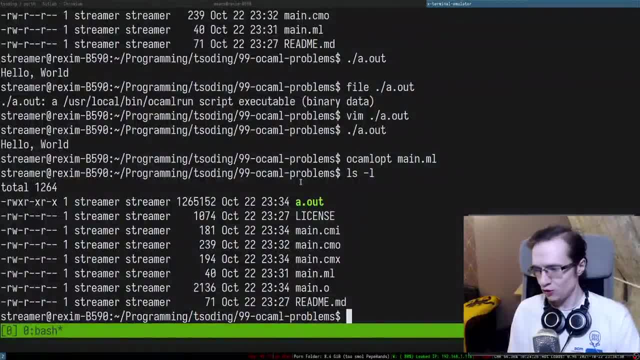 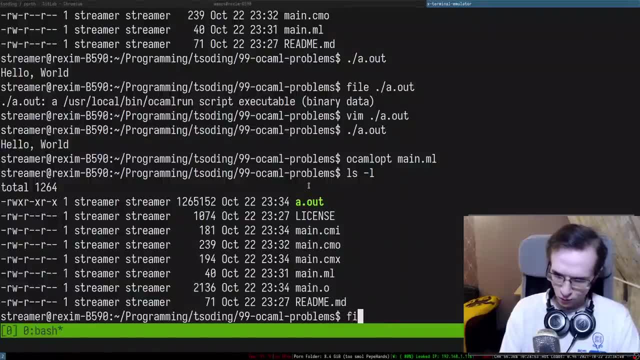 kilobytes, Now it's actually one megabyte, So it generated a shit ton of crap And if we take a look at this file- right, if I take a look at it- not FIKE- I don't know what this FIKE even means. 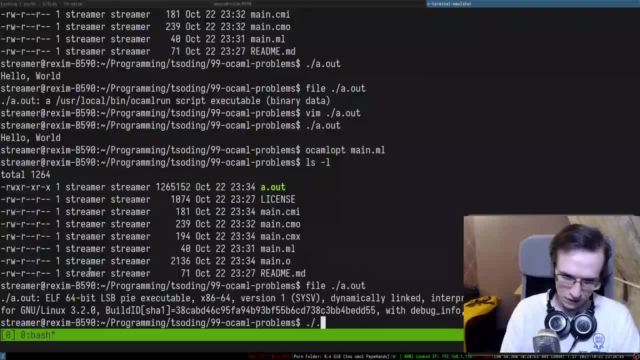 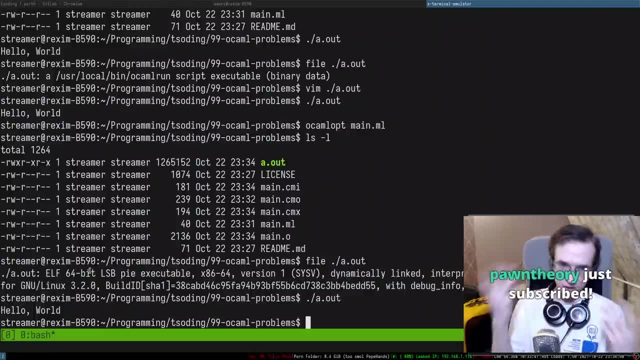 Yeah, So, as you can see, it's an elf 64-bit executable And if you run it it says hello world. So, basically, you have several options. You can use OCaml as a script, Right, You can. 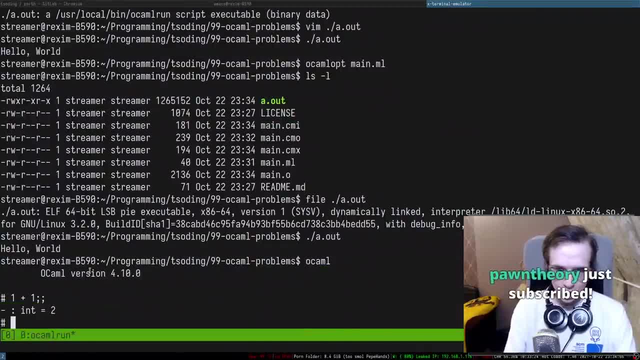 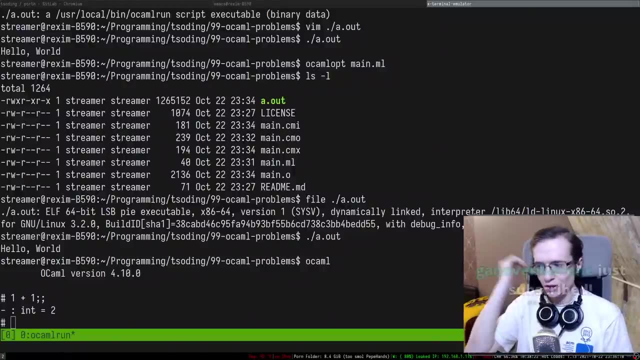 interpret it. with OCaml You can have a ripple as well. You can compile it down to bytecode which is cross-platform Right. So you can have like a sort of like a JVM Right, JVM bytecode, where you compile program once and run it everywhere And also you can then compile 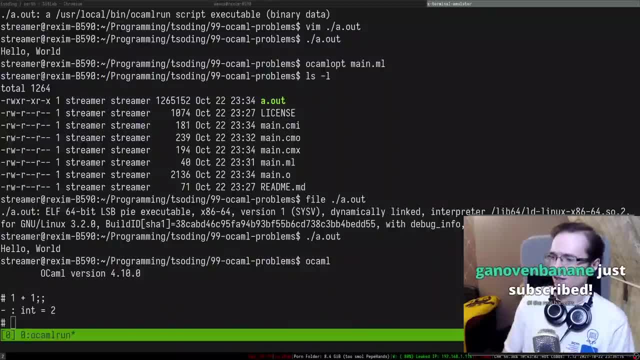 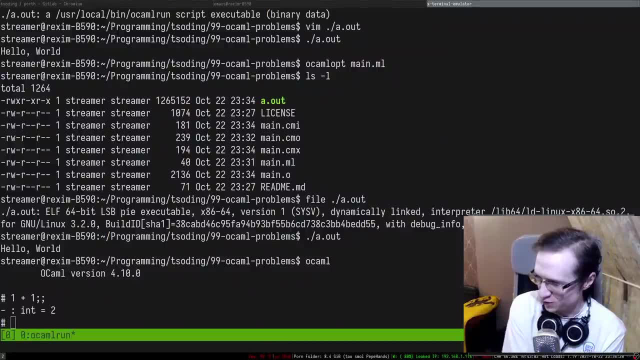 the entire thing to native code if you need them. speed Right, All right. Thank you so much. Pwn Theory for five months of tier one subscription And thank you so much for 15 months of tier one subscription. So the real bangers. 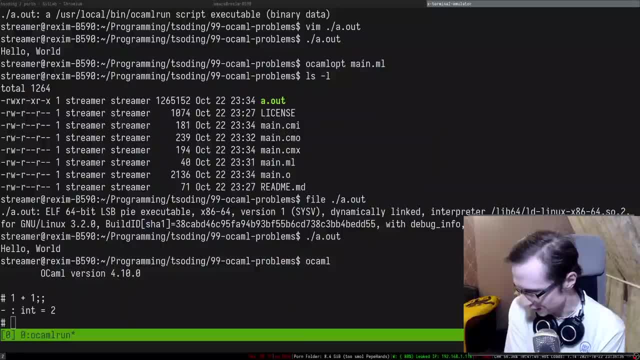 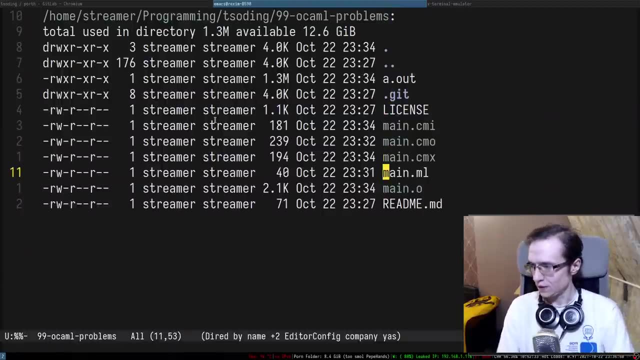 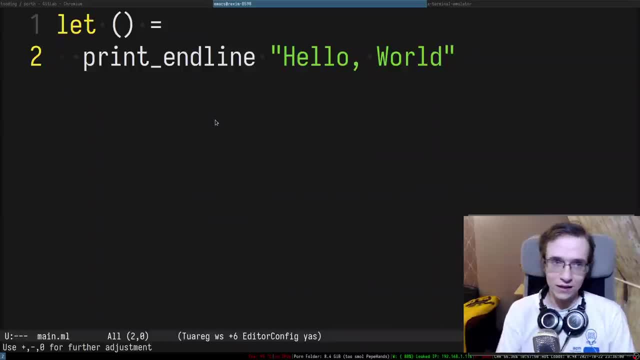 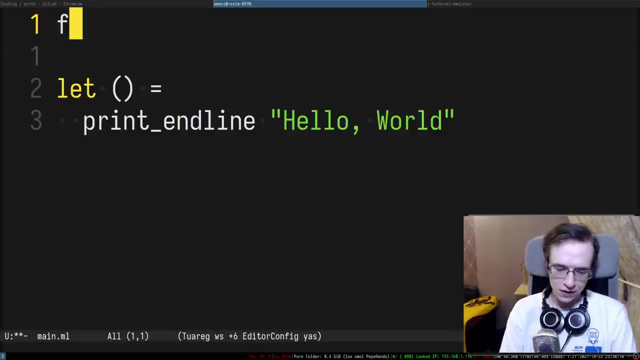 So this is how OCaml language looks like essentially. So, through a, let you define like sort of a binding, sort of a function- And this is an entry point, Right So- and you call functions like: so You define, you provide a function name and then the 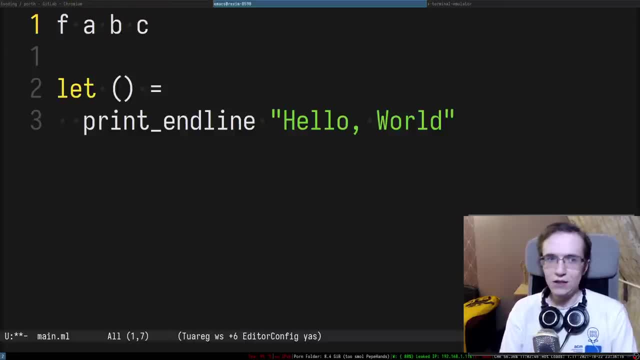 arguments like A, B and C, And this is equivalent to F of A, B and C in conventional languages. So this is how you do this, but in OCaml Right? So first comes the function name and then the 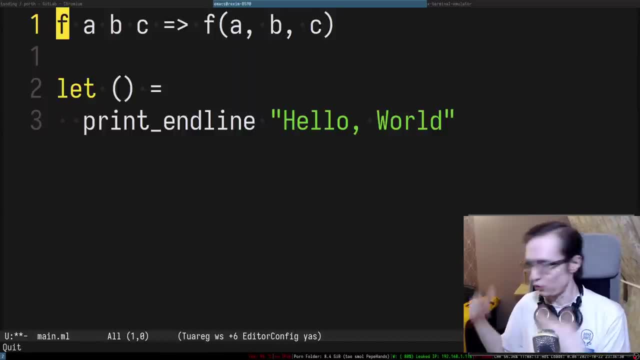 like, separated by spaces, the rest of the arguments. So this is basically how you call this function. So you may ask how would you call this function? You may ask how would you call something like this, Right? So if you have like two nested functions composed together, 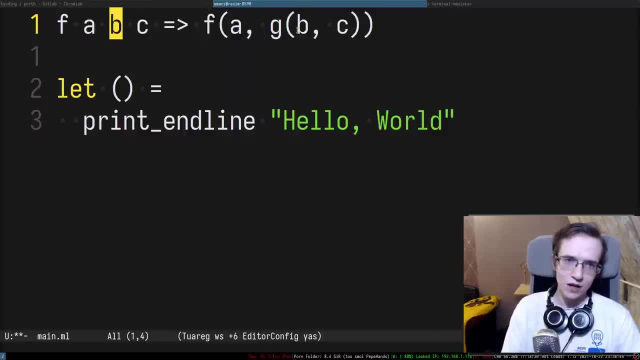 how would you call something like this? Well, in OCaml you will have to do it like that, and then you will have to wrap this thing in parentheses, So you still kind of use parentheses, but just to emphasize what is a function and what is not a function. You see, 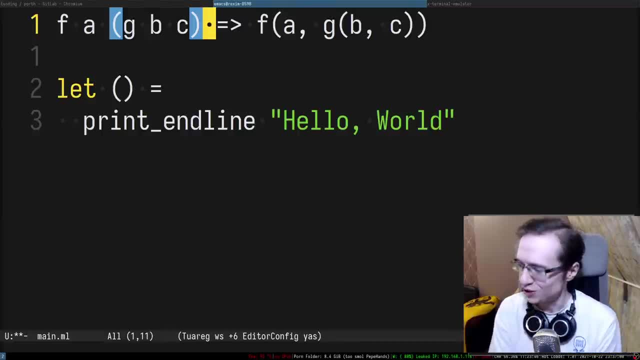 So that's basically the difference, like syntactical difference, between the function calls of conventional languages, like C-style languages, and languages from the family of ML. right, So right. ML in that case doesn't stand for machine learning, It stands for: 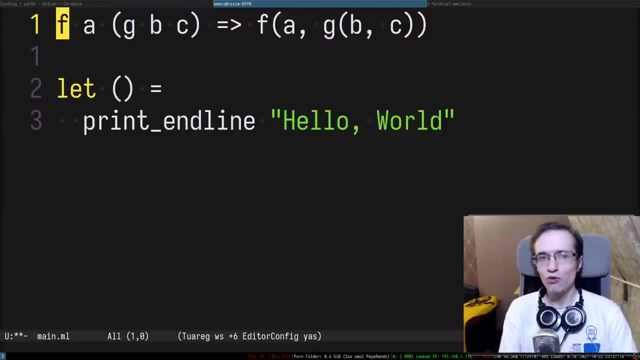 meta language, So there's a whole family of languages where you call functions like this, Not like this, Right So? and one of such languages is also Haskell. In Haskell, you also call functions like this. Another one is OCaml, so then SML, and so on and so forth. 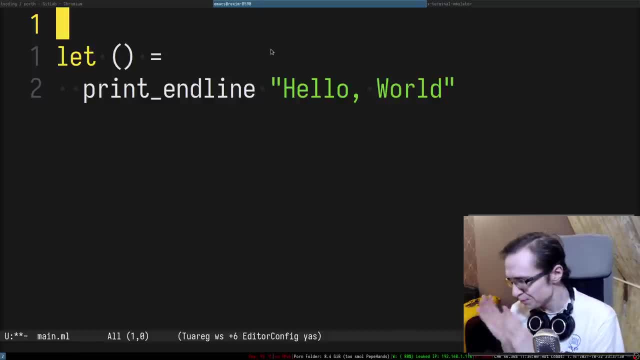 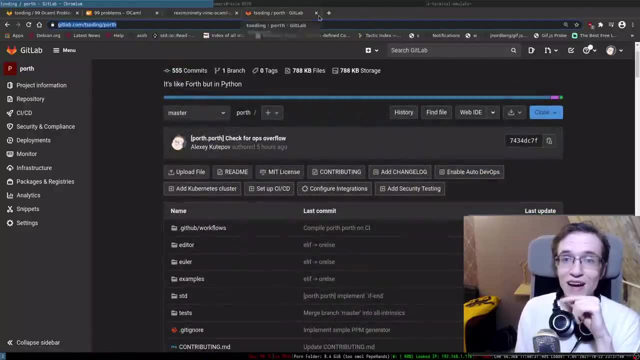 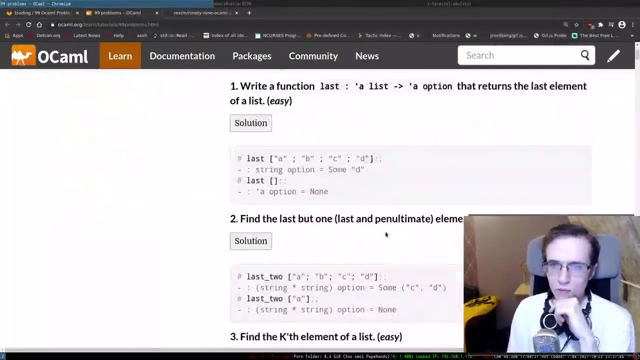 There's a whole family of functions like that, Of languages like that. All right, So let's take a look at the problems that we need to solve. right, So we need to solve 99, not even 69, 99 OCaml problems. Okay, So what's the first problem? The first problem is: 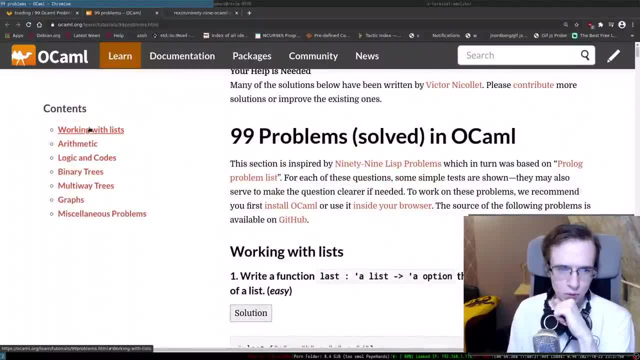 working with list. Working with list is like a section, So all of the problems are split into seven sections: Lists, arithmetics, logic and codes, binary trees, multi-way trees, graphs, miscellaneous problems, right? So we start with like working with lists. 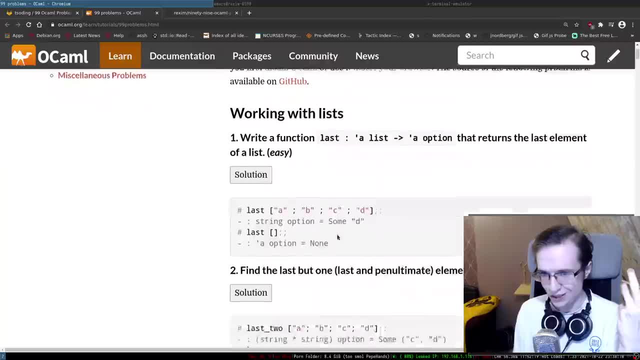 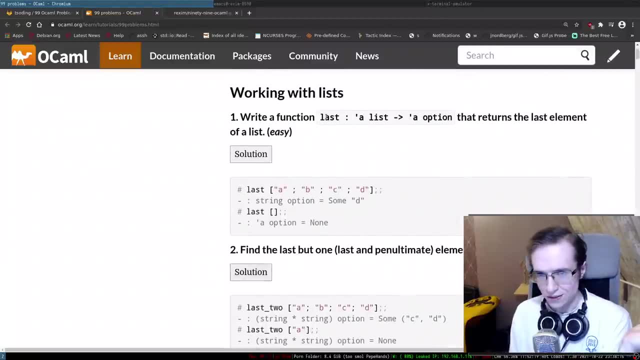 And lists is a fundamental data structure in OCaml, just like in Haskell or maybe in Lisp as well. right, So we need to write a function that is called last and it accepts a list of elements- A right. So, basically, this is a generic list and returns an optional A right. It returns the. 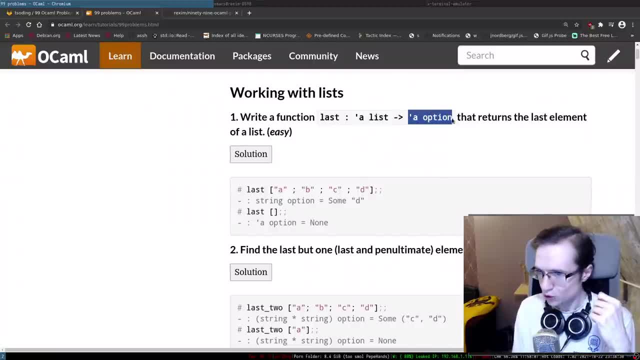 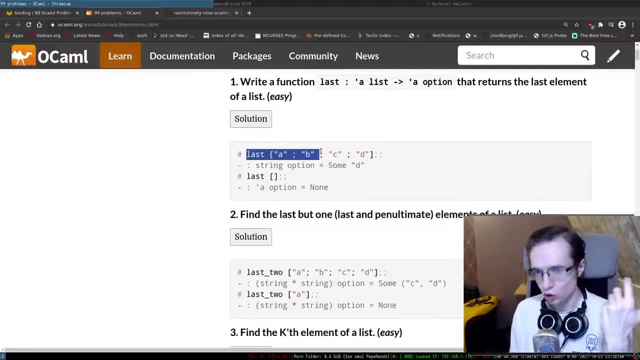 last element of that list- And the reason is why it's optional- is because if the list is empty, there's nothing to return. You should return none, right So? and this is how it should work. You call last on this list. As you can see, list is separated by semicolons, not commas, right So? 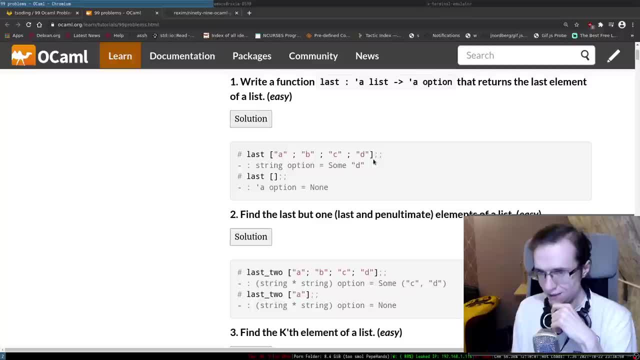 it is needed to actually debate you and make a lot of compilation mistakes, And then if you pro, And this thing should return some D, where D is the last element of that list, And if you provide an empty list, it should return none. So that's basically what we need to implement. 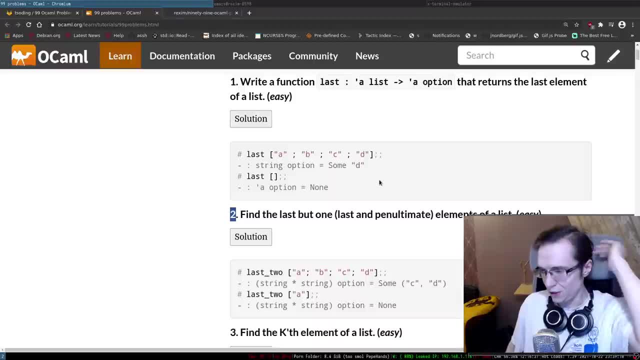 What kind of syntax is that LMIO? Well, it is a different syntax, right? Different languages may have different syntaxes, right? So, in fact, there is nothing fundamentally correct or incorrect about the C-style syntax. It's just like something that was established historically. But you may. 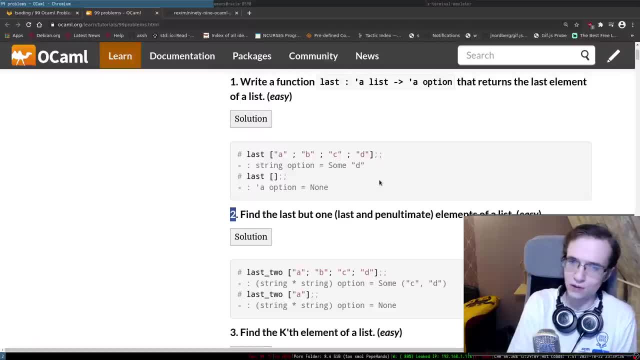 have a different way of expressing things, right? So you're not necessarily have to write. think one way, You can write them the other way, Right? So a syntactic thing is just like a comprendable of the bike shed. It doesn't really matter. What's important, in my opinion, is: 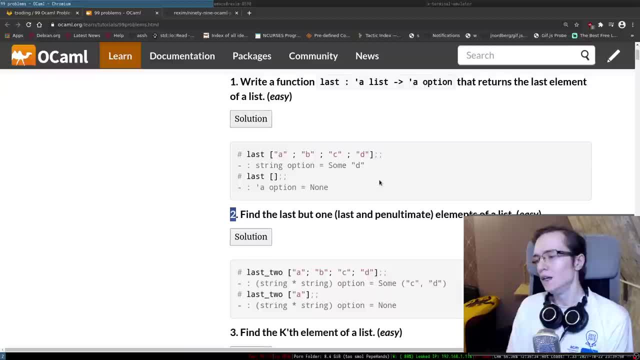 the semantical difference And semantical differences between the camel and classic C languages are actually rather interesting. Syntax is just something that you can quickly get used to. Usually when I compare the languages, I rarely care about the syntax of the language Like. 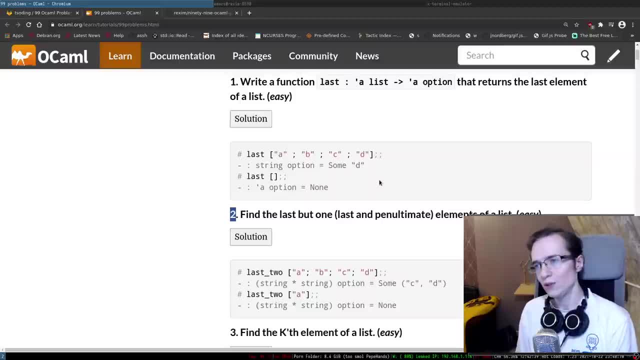 rarely care. For me, what's more important is the semantic of the language. In fact, this is one of the reasons why I'm not excited about Lisp as a lot of Lisp fans, because for me, Lisp is just a Python with S expressions, Since I don't care much about the syntax. 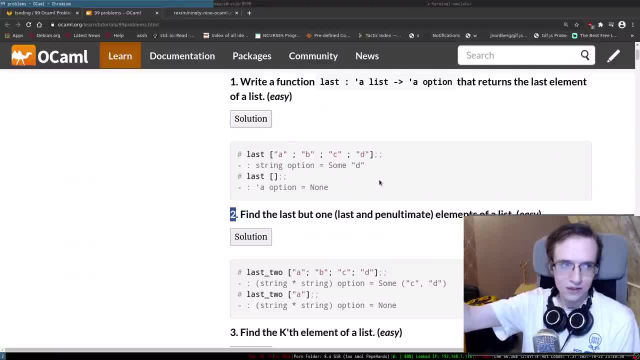 I look at Lisp beyond its syntax and beyond its syntax. Lisp is basically Python, Especially common Lisp. It's just straight up Python, Nothing particularly special about it. It's just like: yeah, you slap S expressions on top of Python, you get Lisp. But maybe there's 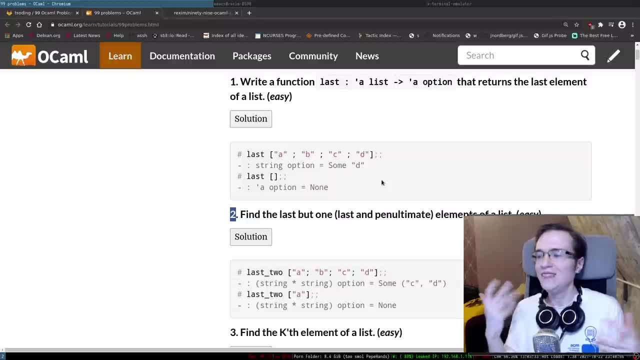 something with my brain, right? So my brain does not find syntaxes of languages exciting or interesting, because it's just like something you slap on top of the language. It doesn't really matter. Hi Tiro, Thank you so much for 26 months of tier 1 subscription. Thank you, thank you. 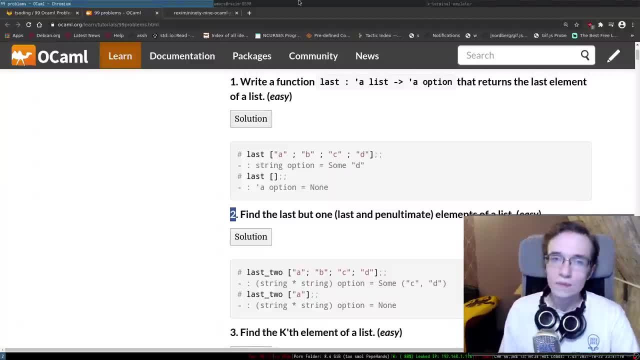 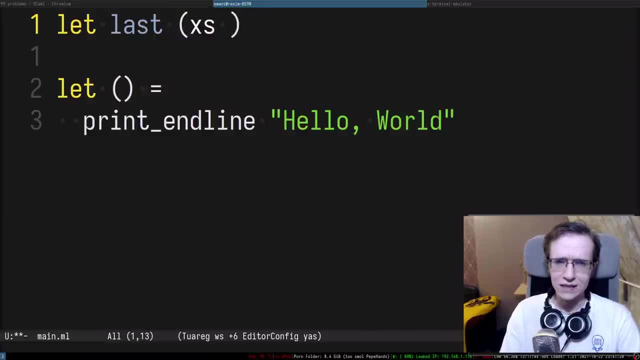 thank you And welcome to our epic camo club. Okay, So how can we implement Lust? Right, So we're going to have Lust and this thing accepts a list of any elements, Right? So the way- this way, you say that you have a list of A's and A is sort of like a generic Right. 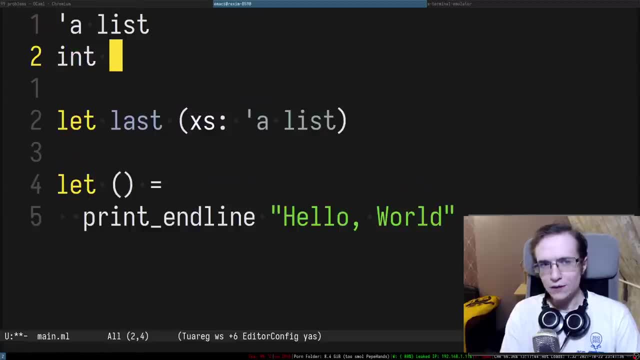 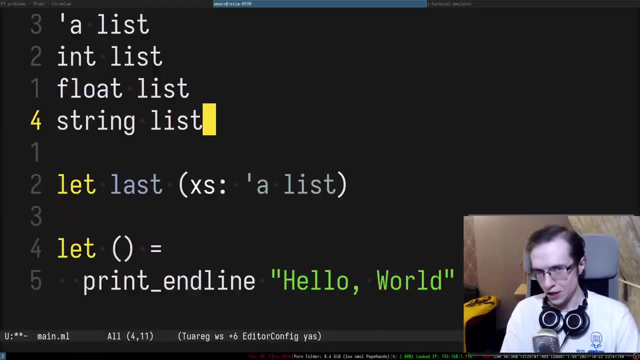 So list of ints, Right. So list of integers would be int list. List of floats would be float list. List of strings would be string list, List of any element. we don't care what that element is is going. 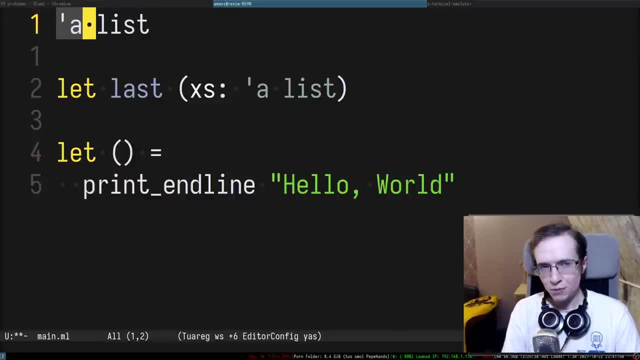 to be prime A list. In fact, prime A is basically a generic. So basically this is equivalent to something like list of T, Where you know, prime A is basically that T that you don't care about, Right? So that's basically what it is. 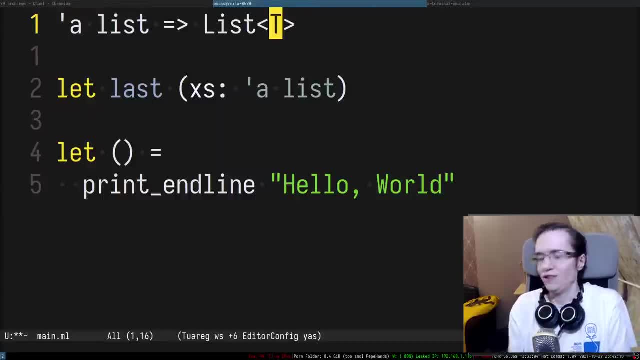 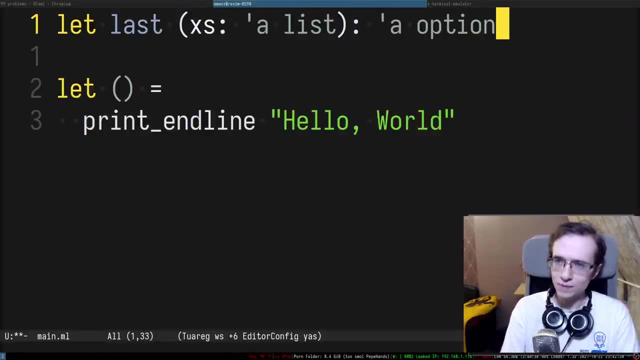 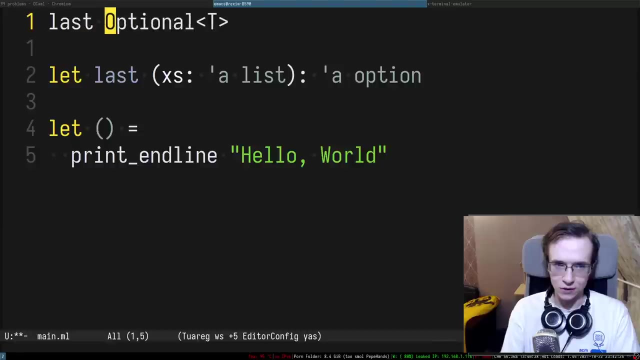 Right, You know, prime A list is basically a list of T, It's just a generic list. And then you want to say that Lust is supposed to return an option, right, and that basically means that it will return like optional T, Right, You have a function, Lust, Right. 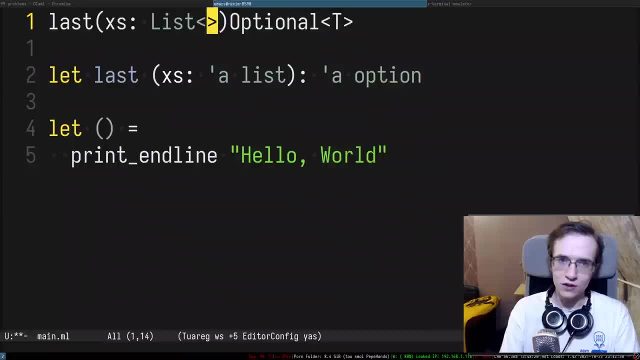 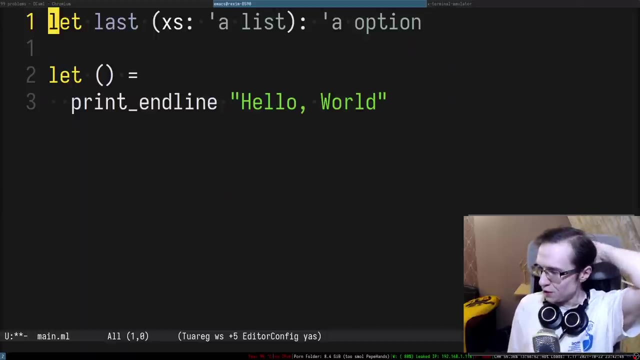 Function Lust That accepts list of T and returns optional T. So that's basically what it does. So it's just like an alternative syntax to that right. An alternative syntax to that. that's what it is. So when the camel type variables come before the type, 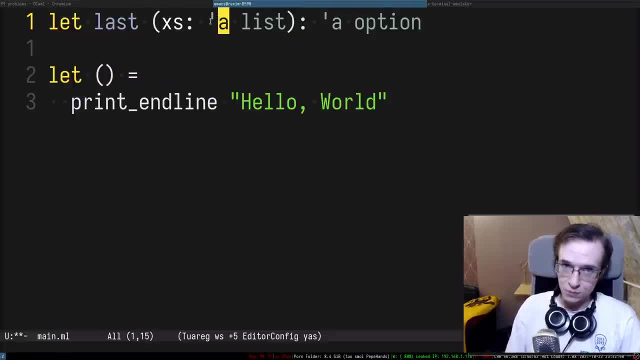 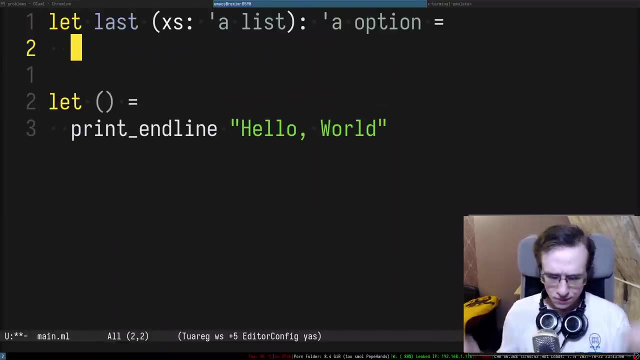 yeah, yeah, yeah. So if you have a type that is parameterized by another type, the parameter of that type comes before the parameterized type. so, Alrighty, so what we need to do? we need to pattern match access, right. 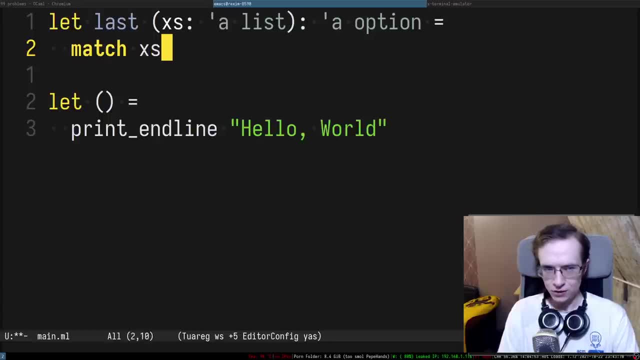 If I remember correctly, you pattern match in a camel with match with right, So that way you can check. Okay, so if the list that we've got is an empty list, right. If it's an empty list, we have to do something, right. 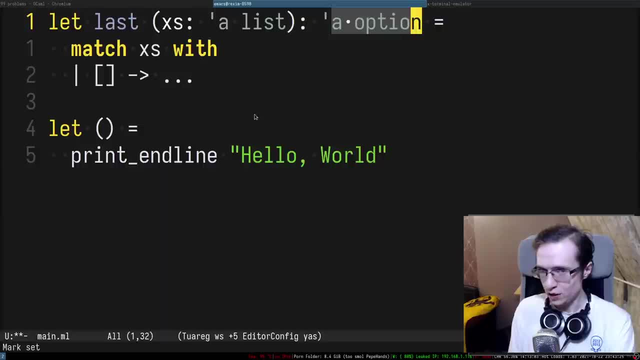 So in case of an empty list- I already mentioned- there is nothing to return, So we have to return none, if I remember correctly. So maybe this is incorrect code, but the compiler will tell us if something's wrong. Okay, so then we need to deconstruct the list. 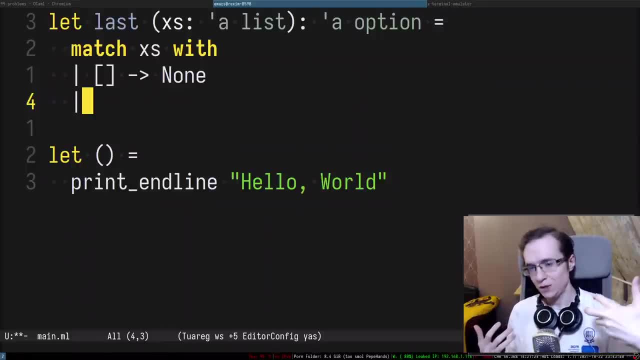 We need to deconstruct the list into its head, the first element and its body. Maybe it's too late. actually, If you think about it, what's the most trivial case for the last function? right, So you need to implement the function. 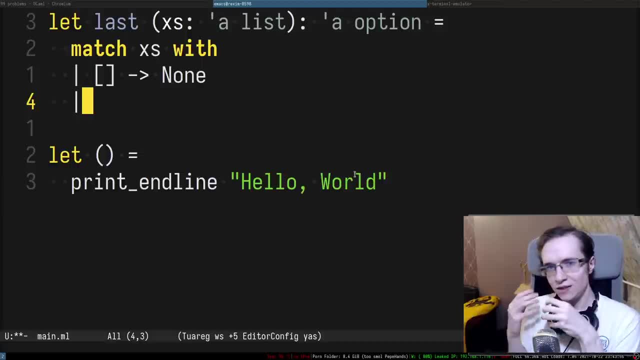 that gets the last element. What's the simplest and the most trivial list, from which it is obvious what is the last element? So it's the list with a single element, right? If you have a list with a single element, the last element of that list is that element, right? 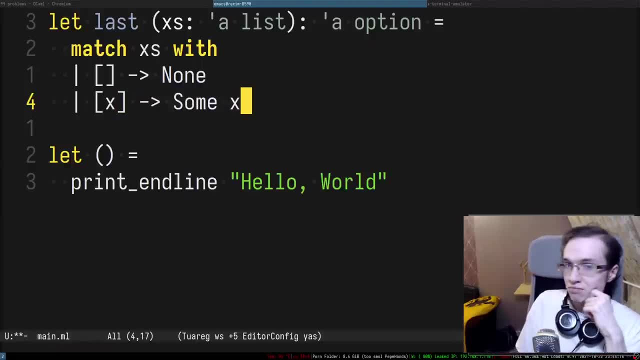 So you just basically go ahead and just return x. It's pretty straightforward. It's the simplest case of when you can just get the last element. All right, so, And the general case is gonna be when you have more than one element, right. 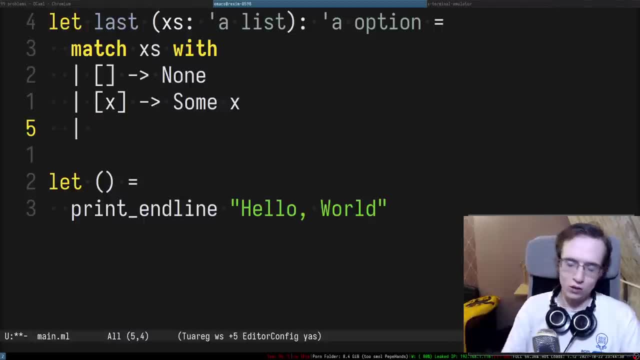 So in that case we can try this. We can try to destruct, right, structurize the list into its like head and the rest of the elements, right. so in this particular case, as you can see, like x is the head and this is the rest of the elements, right, since none of 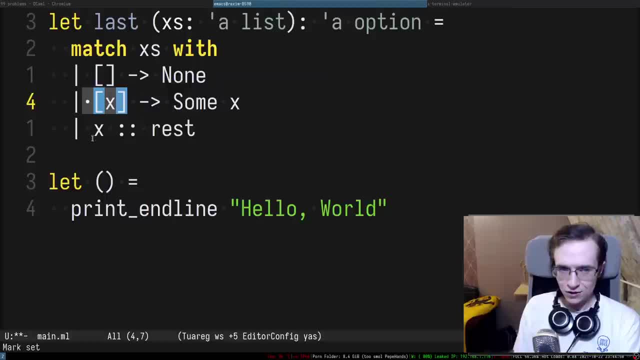 these patterns were like successfully matched. it will try to match this pattern. and how can we get the last element out of here? right, so we know that there is more than one element in here, so that means the last one is not going to be this one. the first one is not the last one. so in that case, 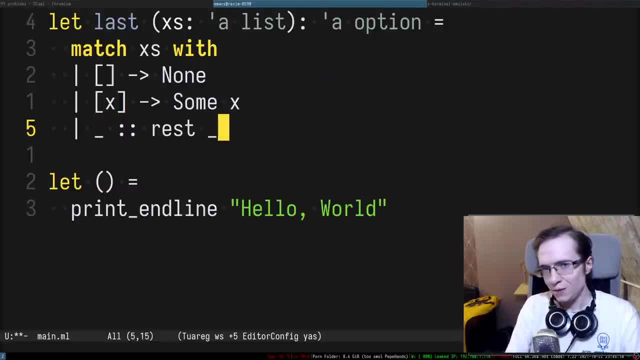 I can say, okay, well, let's just ignore that one. so, and the last element of that access list is going to be the same as the last element of the rest of the element without the head, right? so that means we can do this entire thing recursively. and there we go. we implemented a function that finds the 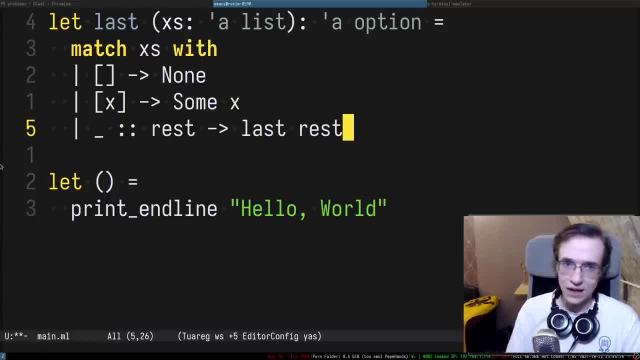 last element recursively right. so we have a couple of bases of the recursion. in case of the no elements, you just return none. in case of a single element, it's a trivial case. it's the base of the recursion, we return that element, and when you have more elements, it's. 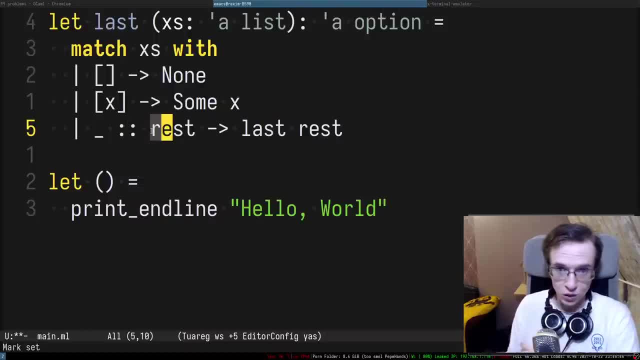 the same as last element of the list, without the first one. and as you go, we have like a recursive process that basically chops off the element of the list until it reaches the list of the single element and it just returns that list to you. so here is the function. is that clear? does it make? 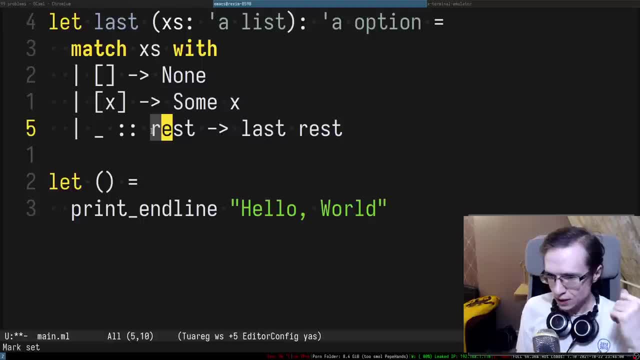 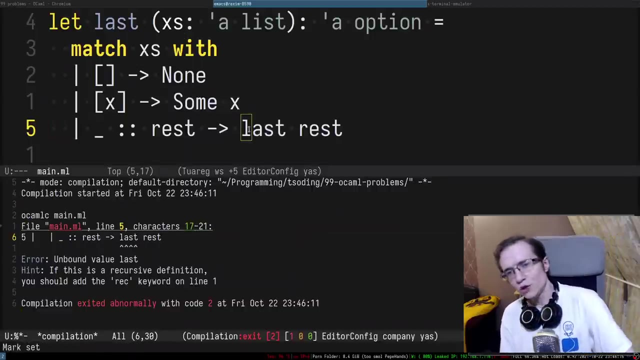 any sense. hopefully that makes sense. okay, so what we can do in here, I think we can try to maybe compile the entire thing I forgot how to use. ok, actually, so, okay. so here is an interesting thing: I'm trying to call last while being inside of last and the compiler complains that it cannot. 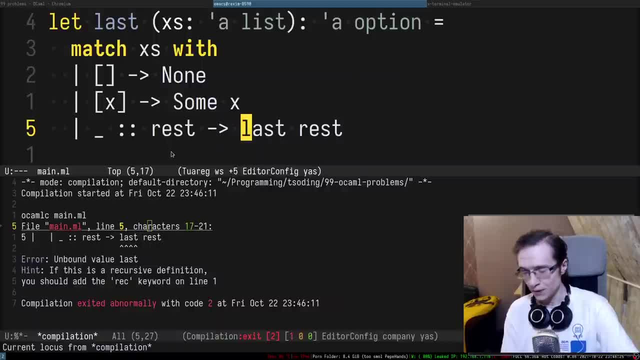 find the last. and this is because you the function is not going to find the last element of the list is because the function is not going to find the last element of the list. so there are other functions in here called recursive, recursal. you t the functions by: 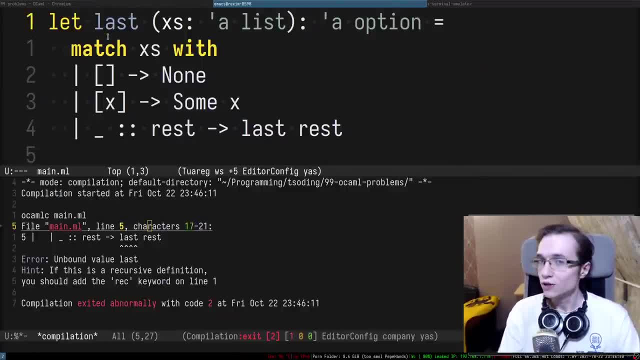 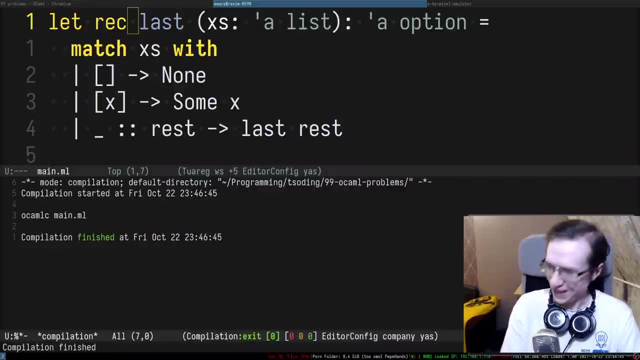 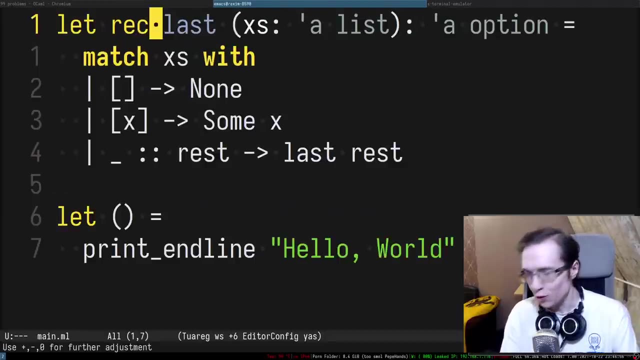 default in a camel are not recursive right. they are by default not recursive. so to indicate that a particular function is a recursive you have to put a wreck in here, and only then you would be able to compile your program if it has a recursive function. so this is very interesting. so 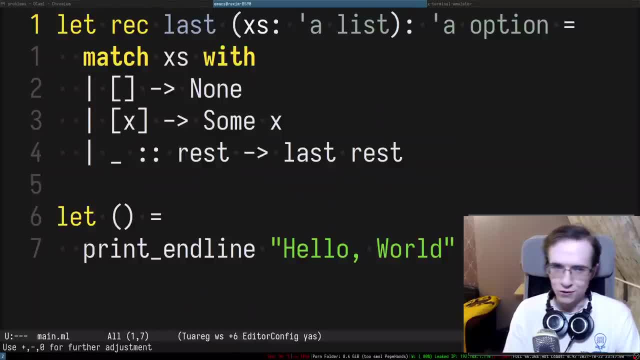 all of the functions, like in the camel, if you define them, you cannot call them recursively and you have to specifically say that it's a recursive function and it's actually fine after the falta on MI over gram is from jum울 and wineer, who I talk about before. for example, it is normally possible from A to M, which is common, withulously the fals fresh distribution of join early井. 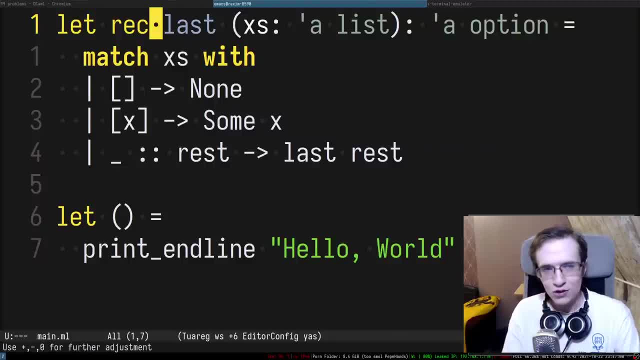 wonder why? why it is so maybe because the uh camel is um one pass compiler right, so until it actually uh has the whole function, it doesn't know its name. so you have to sort of like indicate that, like forward declare it or something. so it's kind of it's kind of strange, but it is. 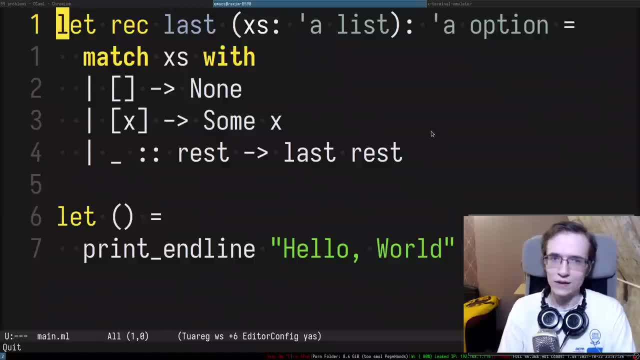 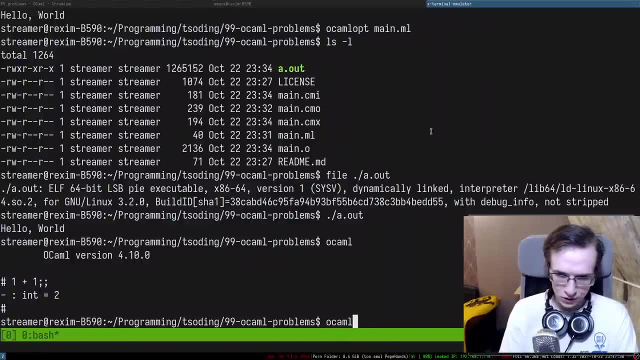 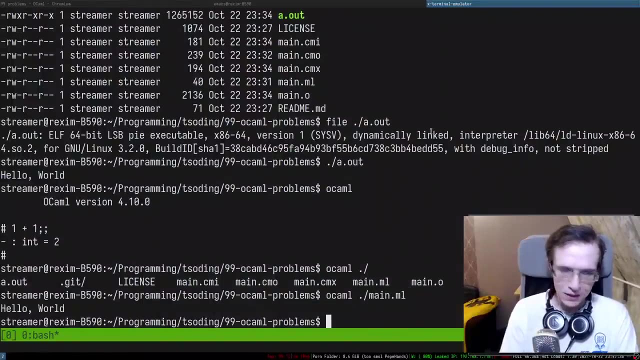 what it is and it isn't, uh, what it isn't. so right, so we have a function uh lost. okay, i wonder if i can just like load some of the function in a camel, right? so if i provide a camel um a ripple, so it's gonna be ml and it doesn't allow me to just have a ripple and load this entire thing um. 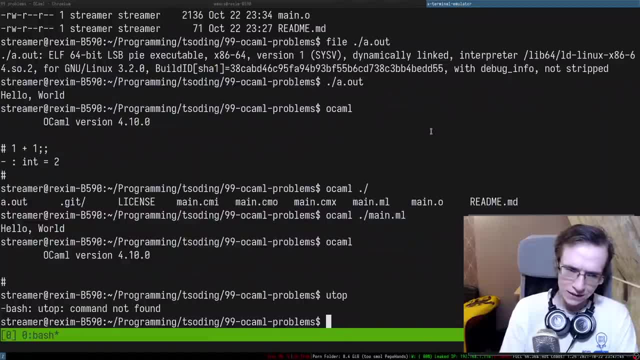 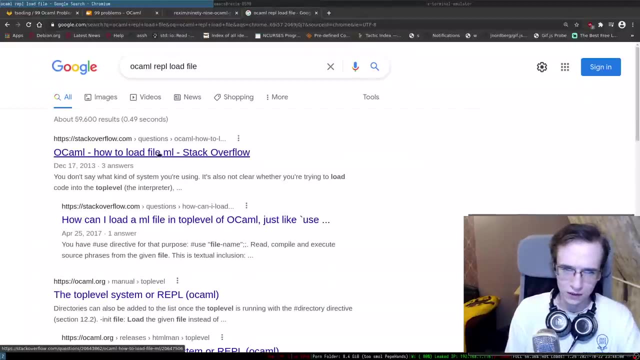 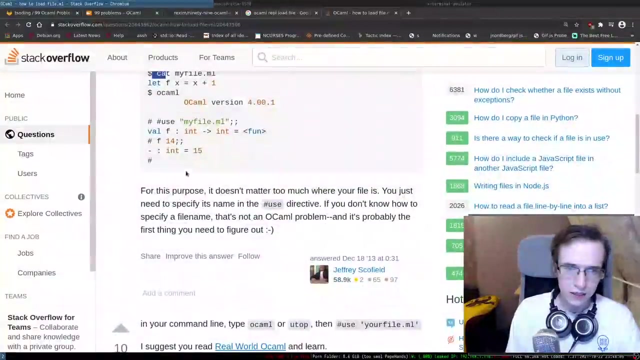 so i do remember that, uh, i had utop or something, but uh, i don't quite remember. but but anyway. so, uh, a camel ripple load file. i really don't remember how to load files into into a ripple or camo, i forgot how to do that. so, uh, okay, cut file, you can use that file. that's actually pretty cool, okay, uh. so if i do use, 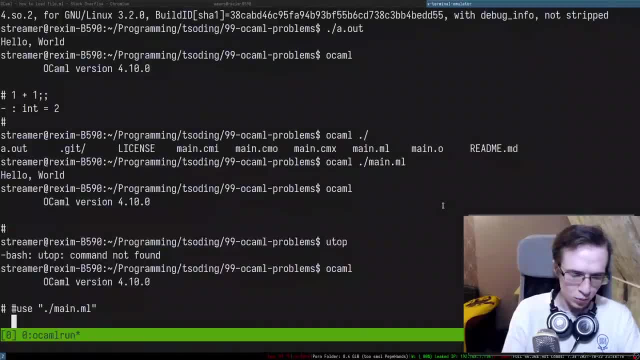 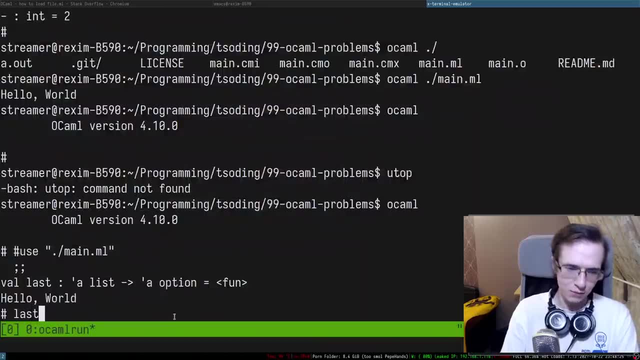 and then i say: mainml, will that work? so i also have to put this double semicolon and that kind of worked. and now i have lost in my repo so i can define a couple of things like one, one, two, three and uh, there we go. so, as you can see, we have- um, you know, we have this list. 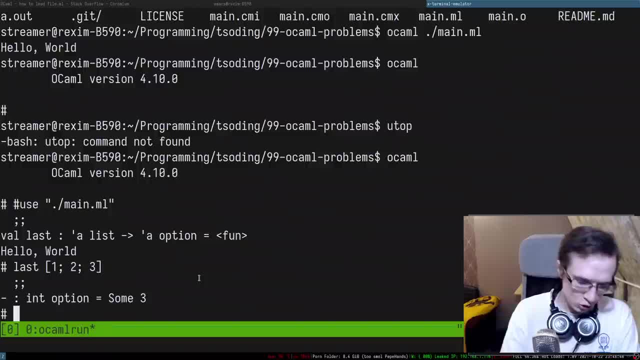 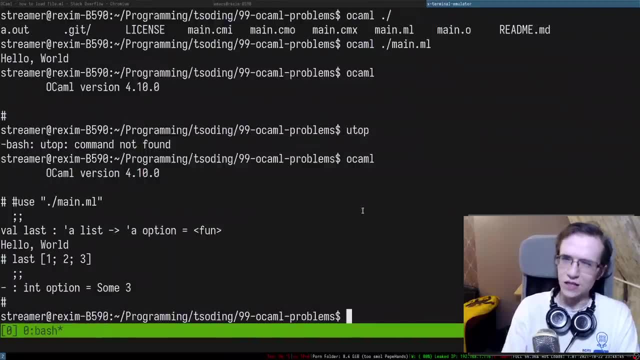 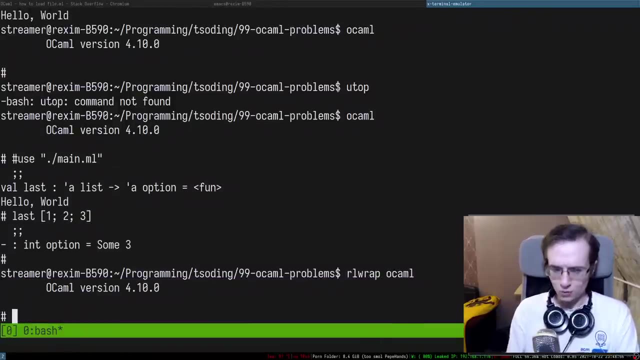 and uh last, return the last element. right, so it's not particularly convenient, right? so a camel by default does not define um any functionality like a read line functionality. uh, right, so we we may want to use something like rl or rl wrap, for those who doesn't know, by the way. so it's. 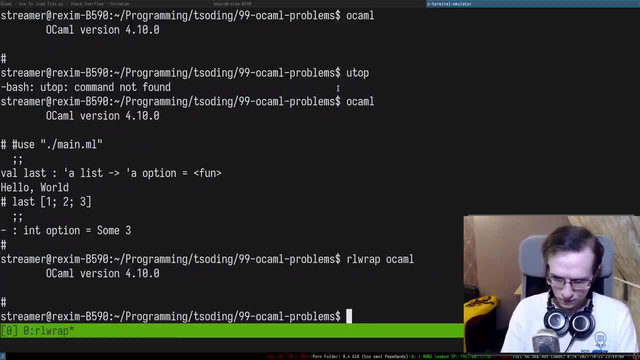 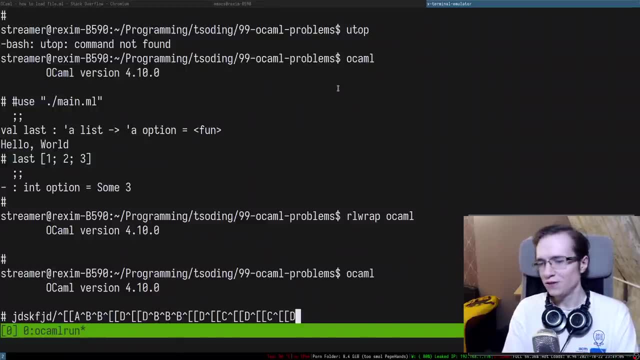 actually a very cool thing. uh, if you want to use something like rl wrap, uh, you can use the rl wrap if you have a program. right, if you have a program that, by default, doesn't have any history and doesn't allow you to, like, move around left and right with arrows, you can always just uh install. 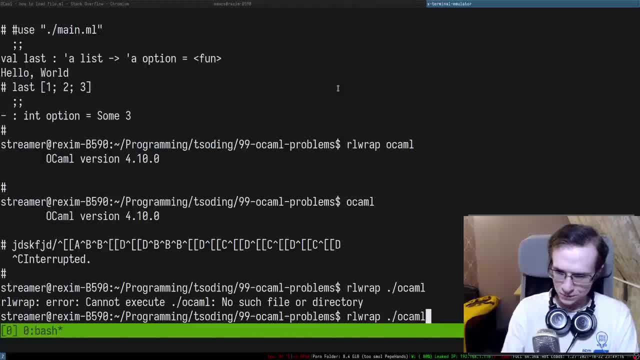 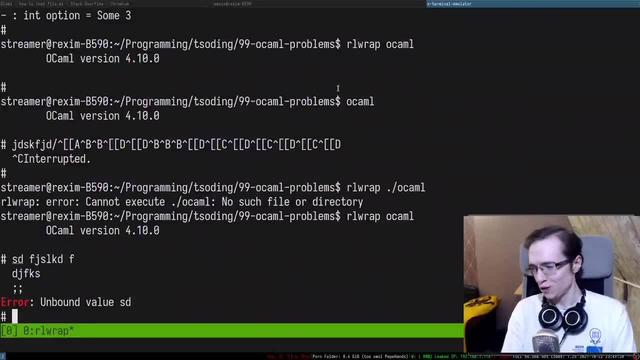 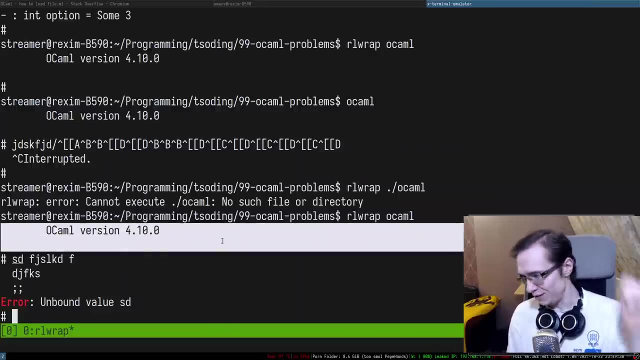 a program called rl wrap right, um, and it will automatically have a history and like everything that you get used to, so it automatically adds like a read line functionality to uh, to your ripple uh that you have in here. so i think it's actually a pretty cool thing, uh, so um. 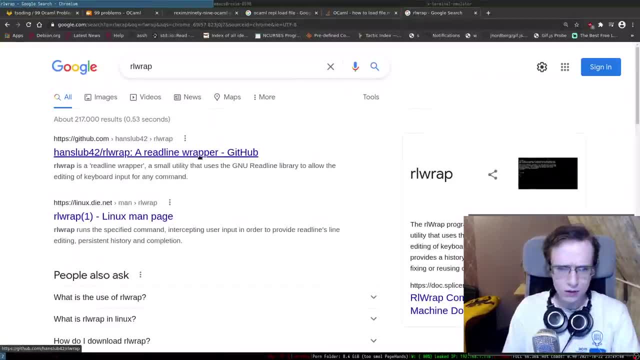 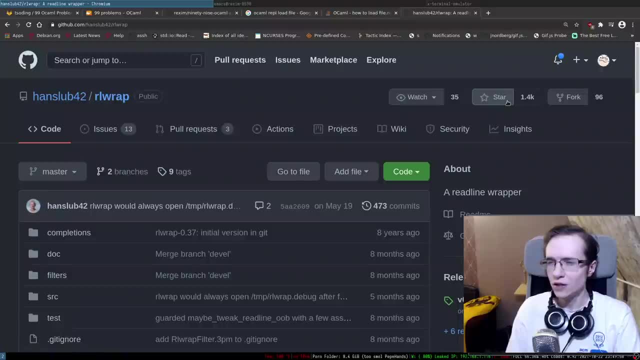 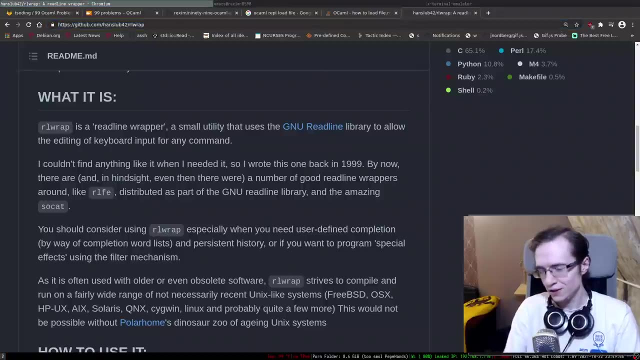 our l wrap, our l wrap, so uh, read line wrapper. is that the official repo of this, of this thing, i think? well, it has a lot of stars and it definitely deserves a star. if that's the official reaper, it definitely deserves the star, uh, and i suppose you can find it in here, but it's usually available. 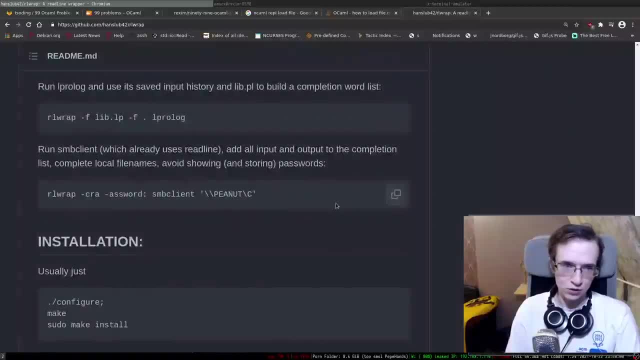 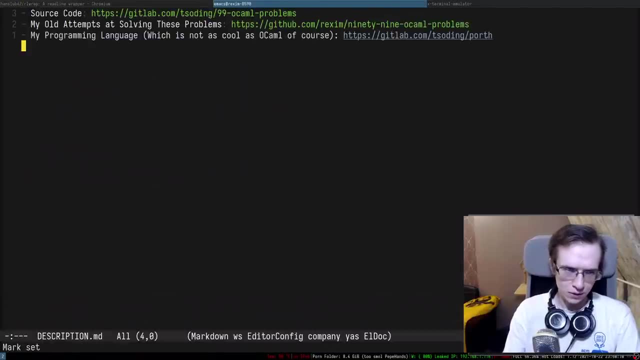 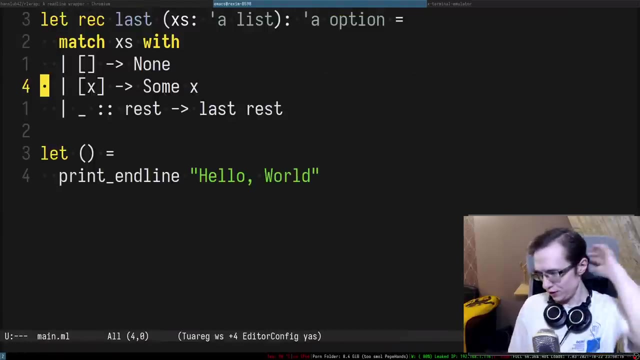 in all of the like linux distros that i used. so it's just like: yeah, it's available. uh, and i'm gonna put that in the description for anyone who's watching right now: um, so, rl wrap, there we go, so you can use this thing in here if you want to, of course, 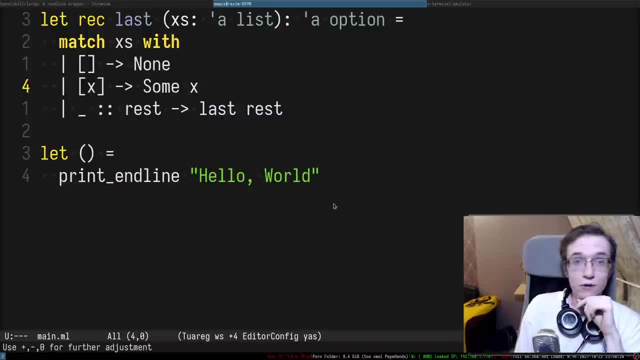 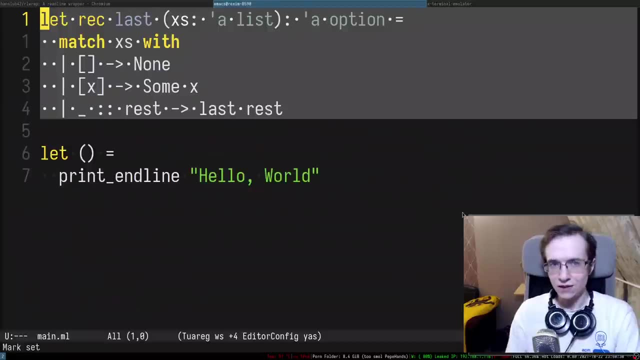 okay, so we've solved the first problem, believe it or not, we solved the first problem, we solved like last, and uh, let's see. first problem. we solved the first problem, we solved like last, and uh, let's. What's interesting is that, since lust is a generic function- we already discussed that it's a generic- 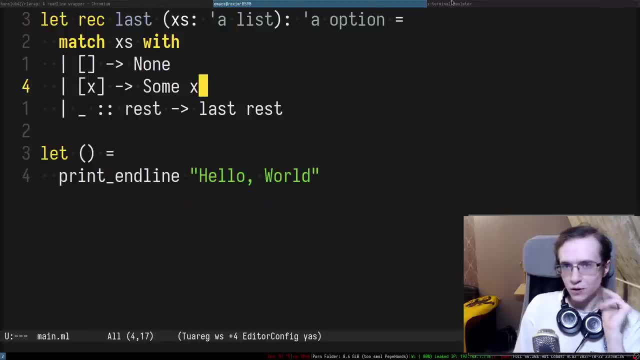 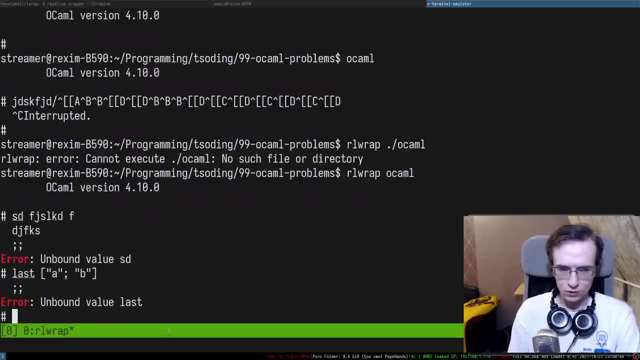 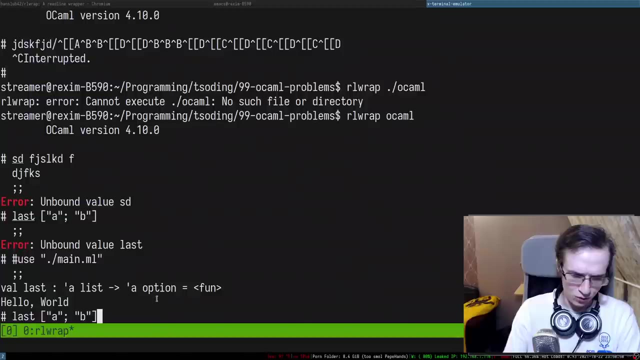 function, So you can use it not only with numbers, you can use it with strings, right? So you can do lust and it will return you about we have to use this entire thing, So it has to be mainml. There we go, And then I can just do something like this: And there we go, So it also works. 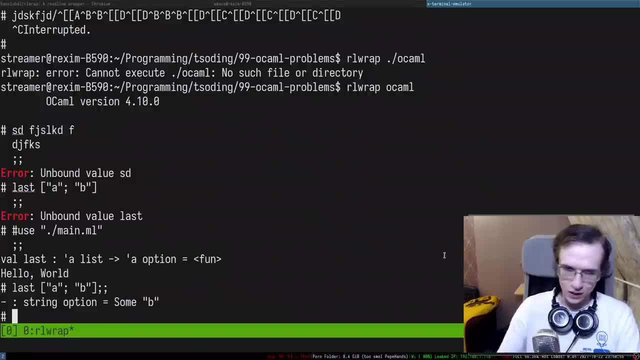 with strings. It works with any types because it's generic, right. So, unlike some of the modern languages that are younger than a camel, a camel is actually a pretty old language. A camel does have generics, right. I'm not going to point any fingers on any of the modern languages, right? But 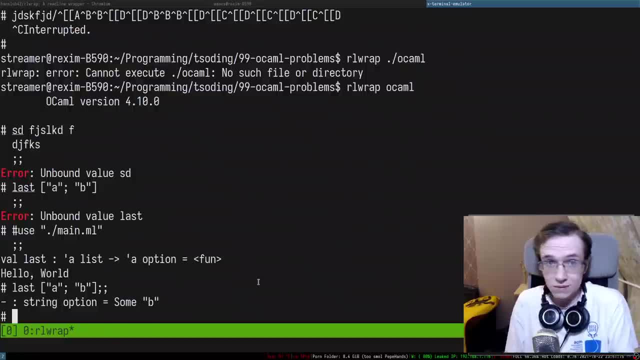 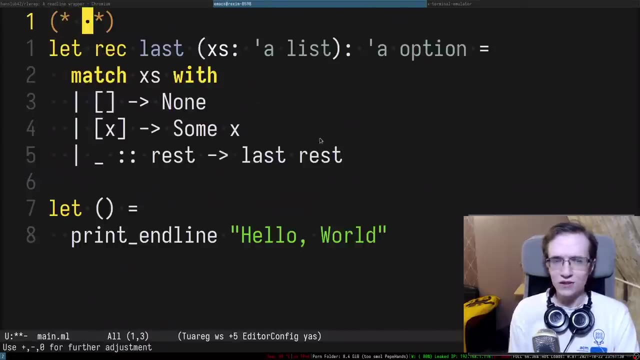 this thing has, you know, generics and they work pretty fine. They work fine, All right. So, and again, if you use this thing on an empty list, right, It will return none, Okay, So this is the first problem, As far as I know the comments in OCaml. 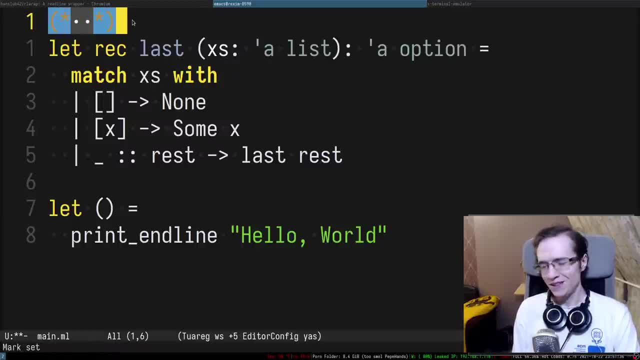 are kind of weird. This is the way you define comments And as far as I know, there is only multi-line comments. There is no comments. that comment a single line. OCaml has generics, but it doesn't have a single line comments, right? So there's always a trade-off. That's the price. 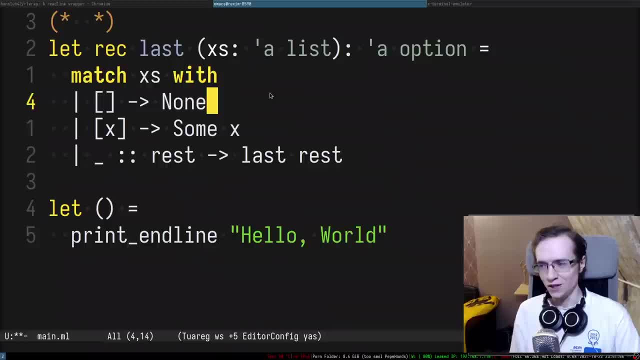 you have to pay, you know, to have generics, right? It's like with Python, right? So there's a trade-off. You can either have, you know, a newbie friendly language or a fast language right In here. it's the same. You can only have generics. 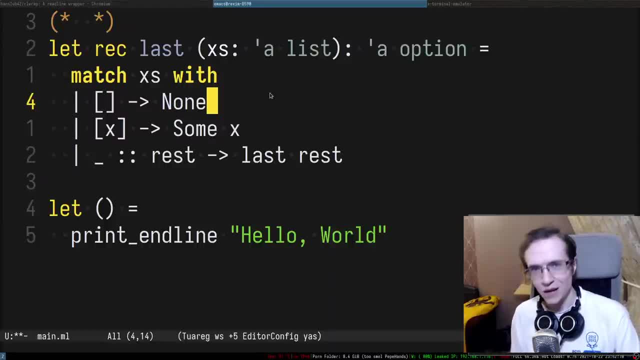 or like single line comments. right, That's the price you have to pay. You cannot have both. right, It's impossible to have a fast and newbie friendly language. It's literally impossible. Computer science haven't solved that. The same goes with, you know, single line comments and. 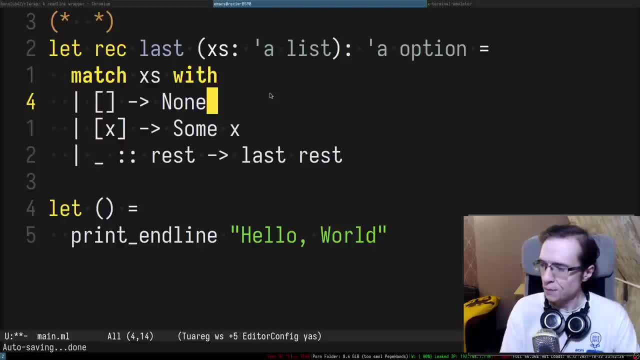 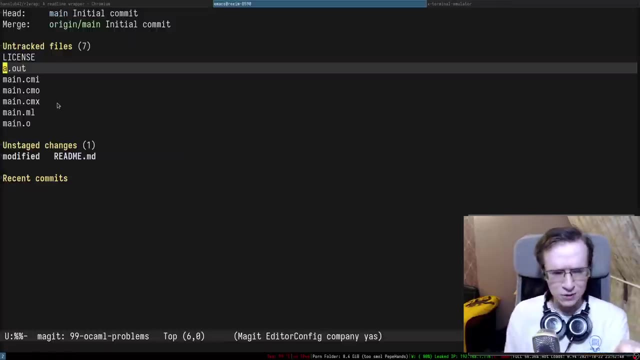 generics, right? So these are mutually exclusive Things. Okay, So this is going to be the problem. The problem zero one, Problem zero one. Cool, So maybe we're going to actually just comment everything. So also OCaml. one of the problems with OCaml is that it produces a lot of garbage, right? So every time you compile, 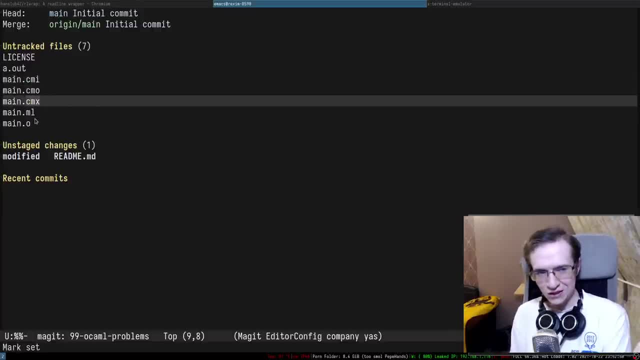 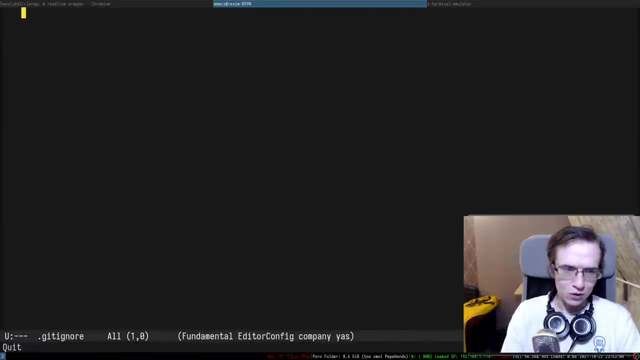 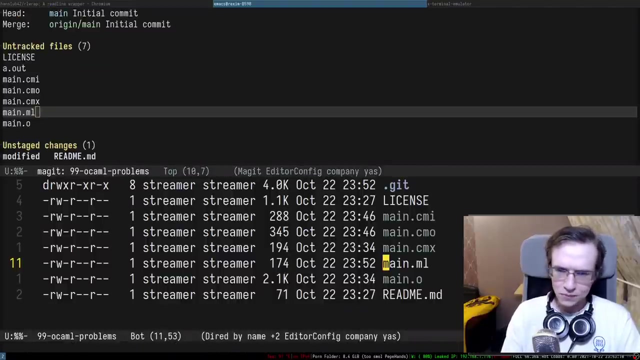 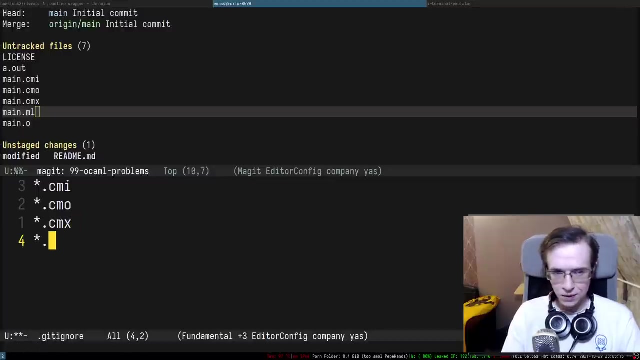 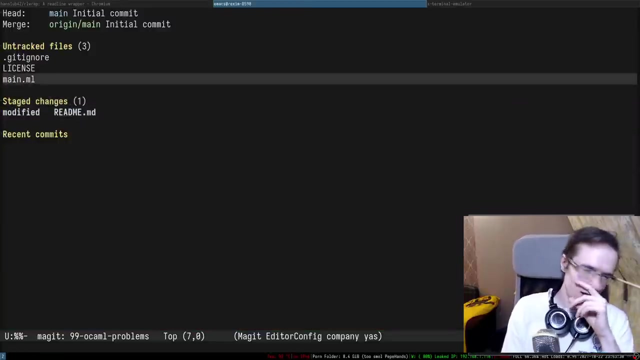 it's just like: CMI, CMO, CMX, ML. Well, ML is the garbage that I wrote. It's my garbage, Like o. so I'm going to just straight up like: remove this entire thing. There we go, There we go. So are we going to have, like some I don't know, like a quick start. 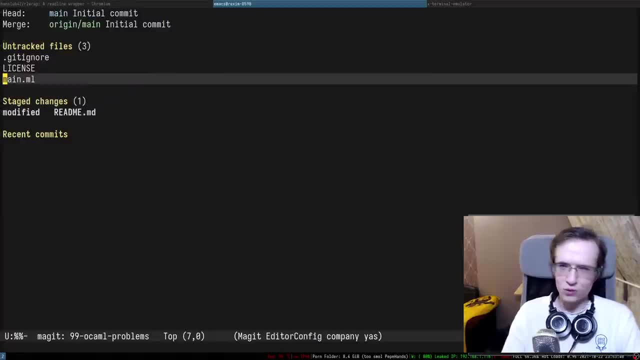 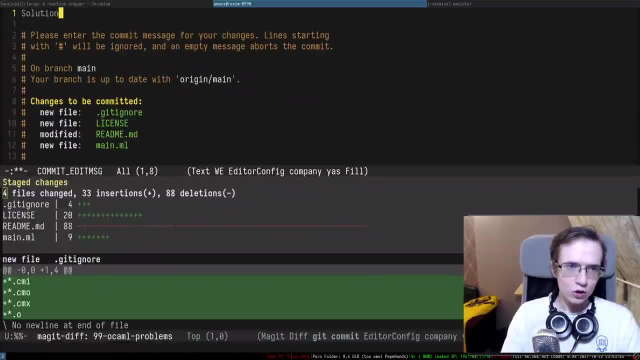 instructions? I didn't think so. We don't. we're not going to have any quick start instructions because we don't have that many solutions anyway. Right? So let's do something like this: Solution for problem zero one, And I'm going to push that right into the repo. And yet again, 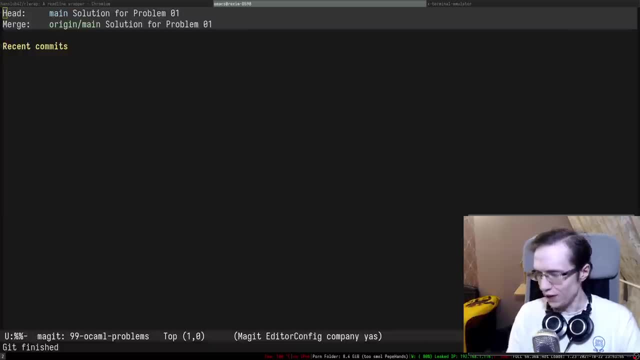 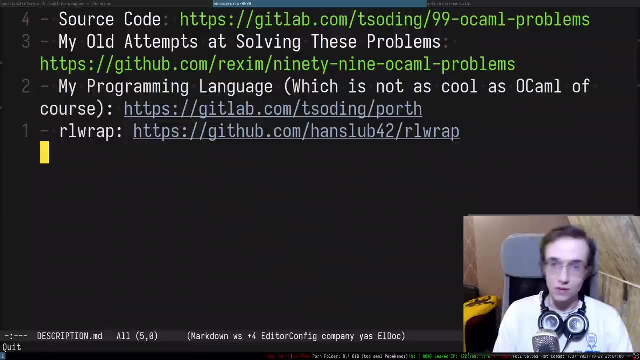 the source code is available Right here. right now. you can find it in here And, for people who's watching on YouTube, you can find the source code in the description. So I keep track of what I'm going to put in the description and hopefully I won't forget and won't lose this file when I'm 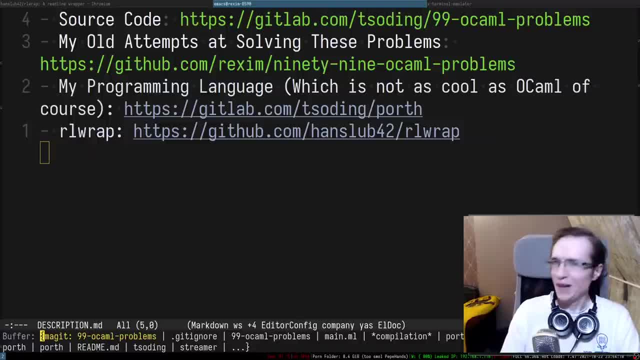 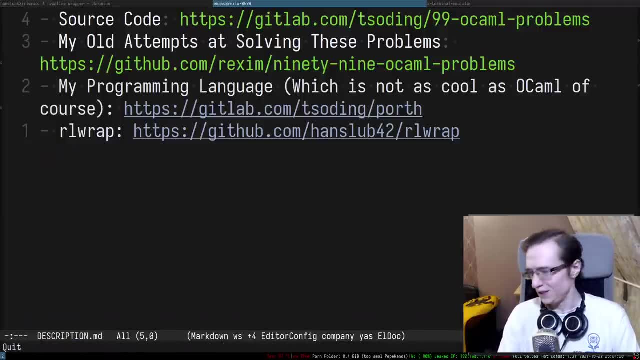 about to upload this video, So that might happen. That actually happened a couple of times. I remember actually keeping track of what I want to put in the description And then I just deleted that file and I don't remember what I wanted to put in the description. So if that will happen, 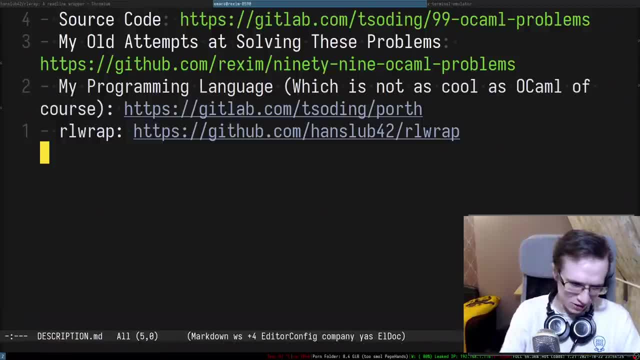 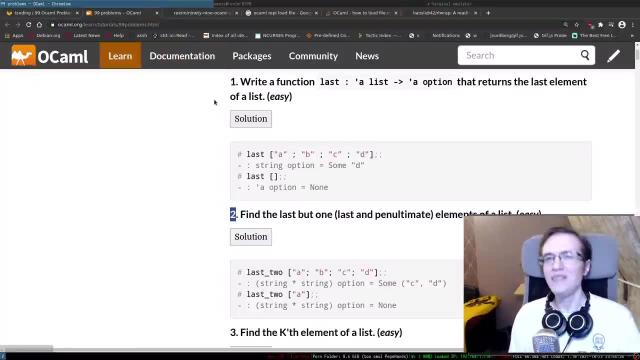 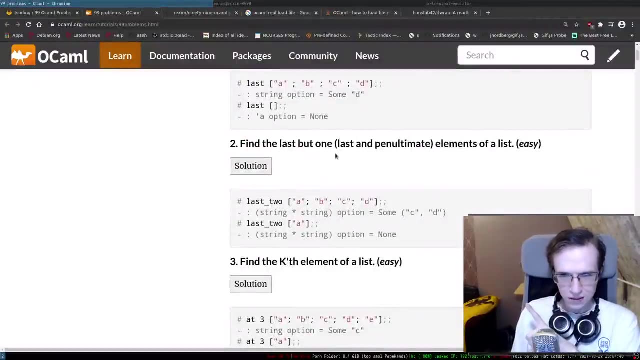 this time I apologize. You can always Google all these links, right, So it's just like: yeah, Anyway. so what's going to be the next problem? What's going to be the next problem? We have 98 of them. We already sold one. Find the last, but one last and penultimate elements of list. 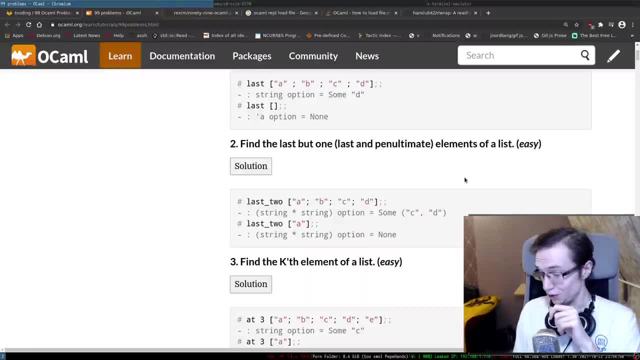 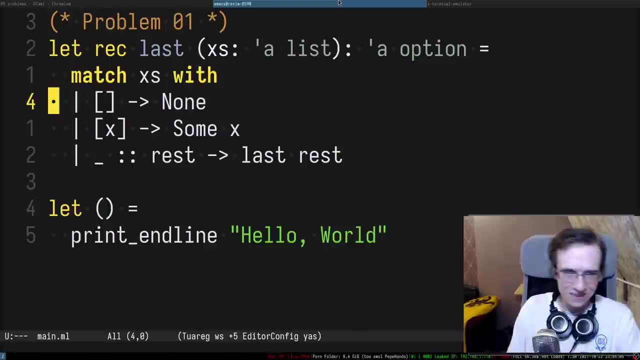 Easy. Well, it's not really easy to understand, but okay, Oh, I suppose you need to return last and the one before last, last two. Okay, So that makes sense, All right, So it literally even called last two. Holy shit, The function itself is called last two. 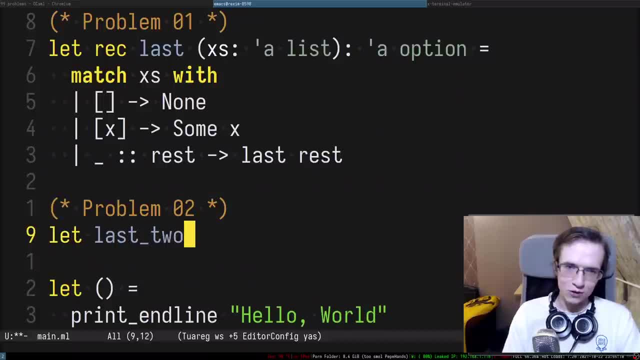 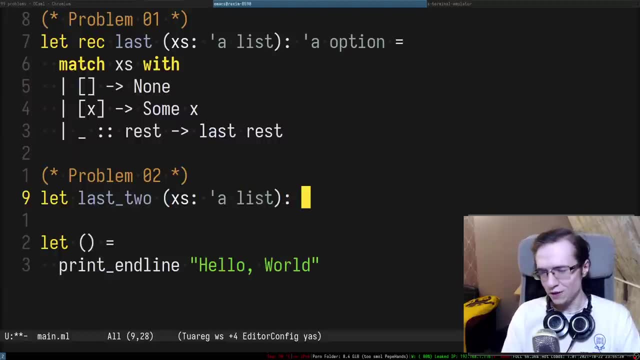 Problem zero two. Okay, So this is going to be last two And yet again, it is going to accept a generic list, right? And I suppose it is going to accept a return, a pair of elements, right? So it's supposed to return. 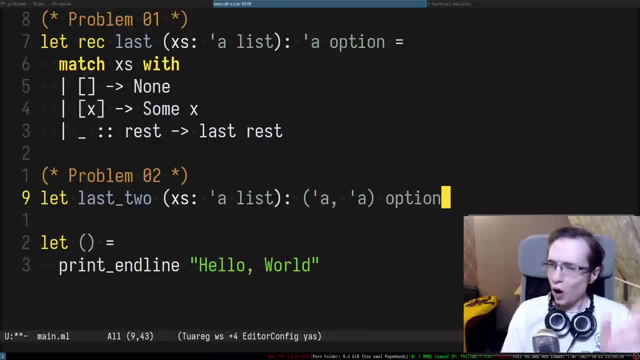 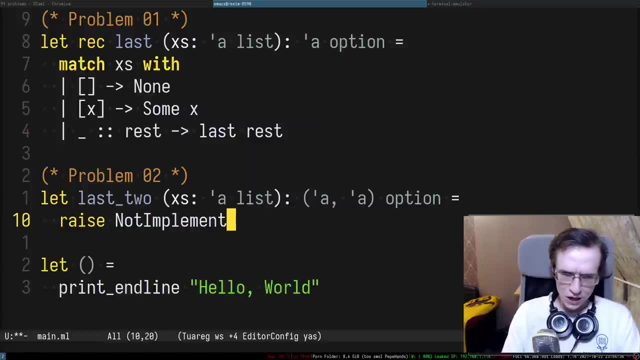 Oh, and I think I remember. So can I rise something like not implemented? or maybe like not implemented: Look, look, look. OCaml has exceptions and you rise exceptions like like in Python. It's literally like in Python, right? So majority of people believe that. 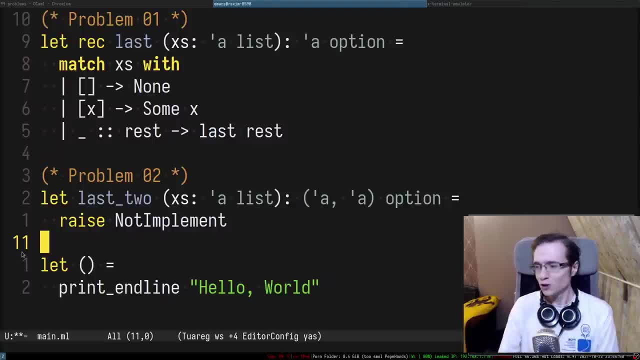 the syntax of the language equals to the language. So if some of the languages share words, that means they're basically the same languages. What is semantic? I've never heard of semantic. The fuck is semantic? The syntax. Syntax is the language. Syntax is the language. 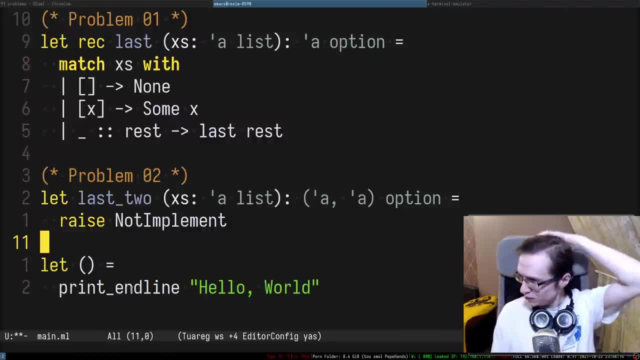 I bet Zosian could rewrite the port compiler in OCaml and that would be still faster than Python code. Yes, it would, Because I actually worked with both big Python projects and big OCaml projects, And big OCaml projects are generally way faster than. 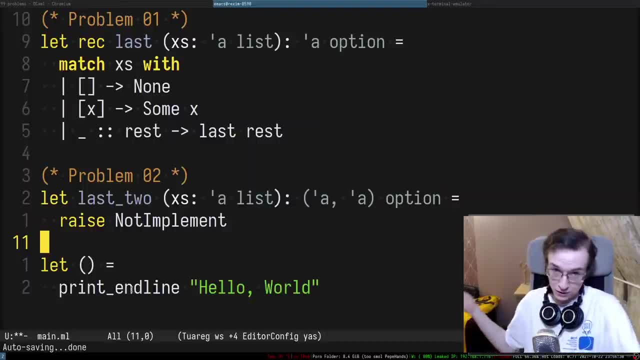 Python projects Way faster, Because I mean it compiles and optimizes the native code, Right, And in fact it has a way better type system so it catches more errors. But I mean, hey, at least it's newbie friendly, right, Anyway? so let me take a look. I don't. 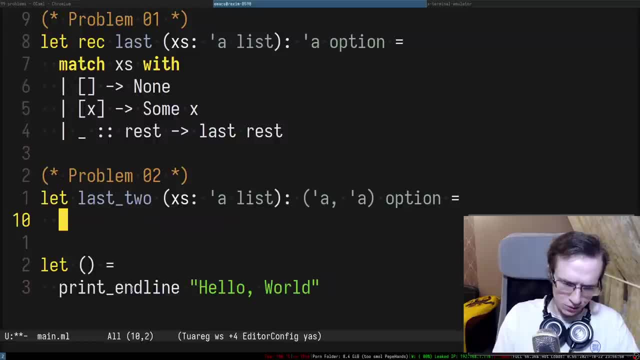 remember how to actually do not implement it. but whatever, Might as well actually do something like assert false. Maybe that will do So. here's an interesting thing about tuples. Here's an interesting thing about tuples. You define tuples not like this, right? So this is a tuple type, right? This is? 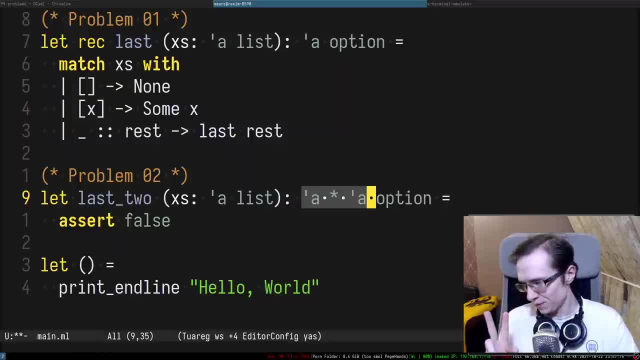 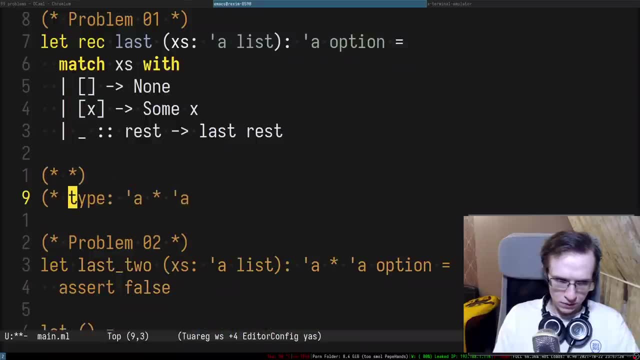 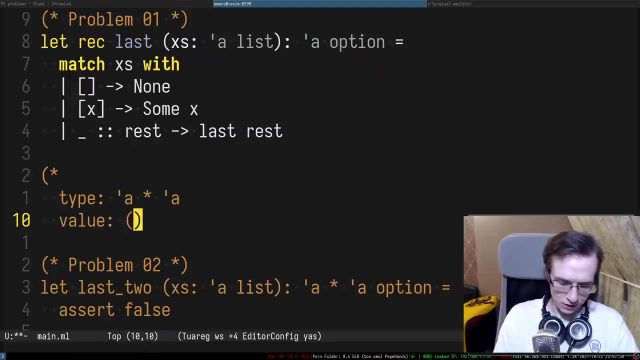 a tuple type. This is a tuple with two elements. But so this is the type, But the value of tuple, oh my god, The value of such tuple is actually going to be 1, 2.. So this is how you define a type, Since 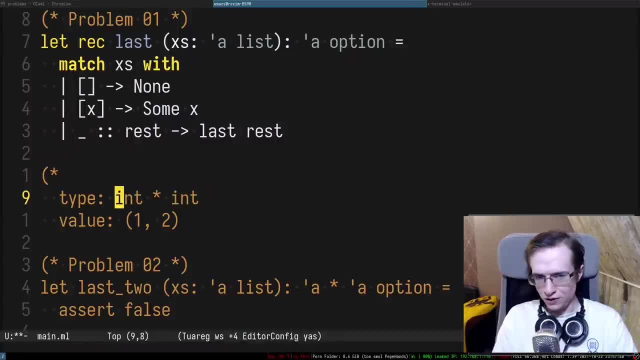 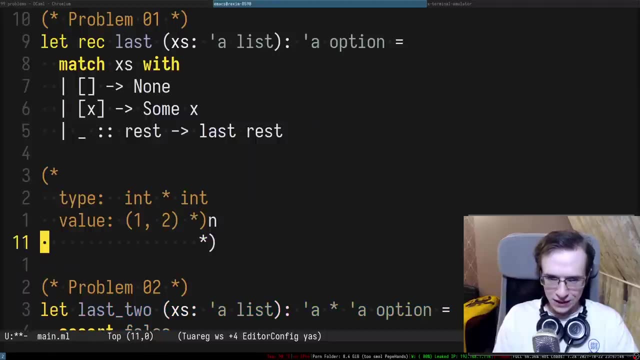 this is two integers. let's actually define this thing as two integers. Okay, So this is the type and this is the value, right? And it makes it super easy to make a mistake and confuse them, And I remember multiple times actually defining a type like this and then trying to understand. 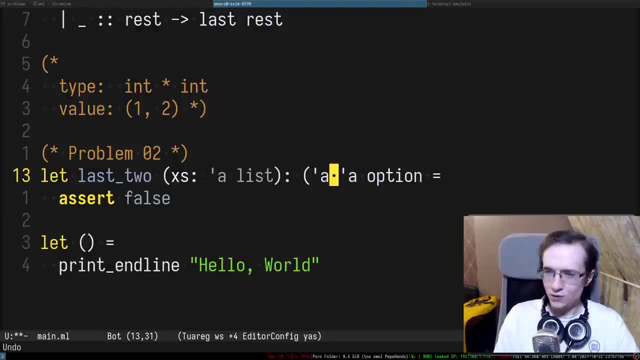 what the fuck is going on and why the compiler complains about that, when in reality you have to define it like this, And in fact there is another pitfall in here: You don't have to even put parentheses around the tuples, Just using 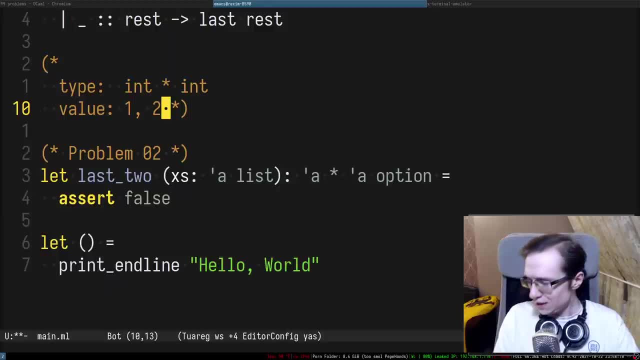 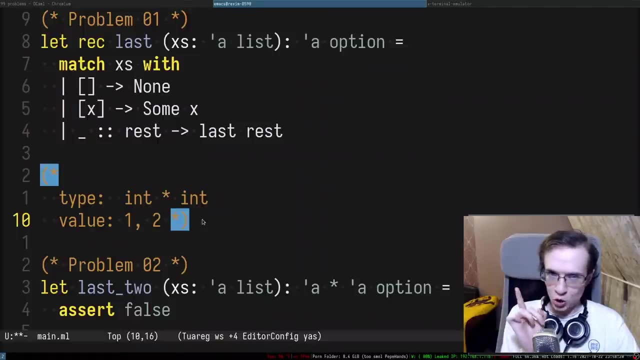 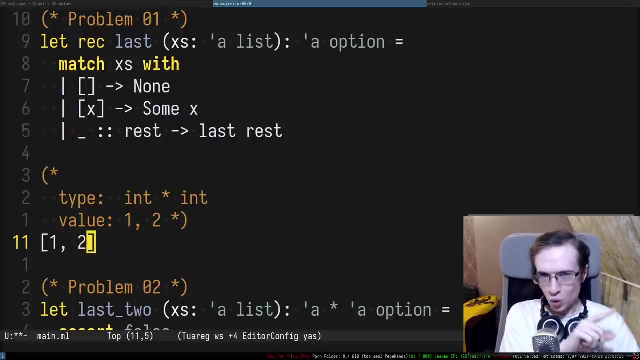 a comma is enough, And this is one of the reasons why lists in a camel are separated by semicolons, not commas, Because this is not a list with two elements. It's a list with a single element, and that element being a tuple of two elements. A list with two elements, in fact, is something like 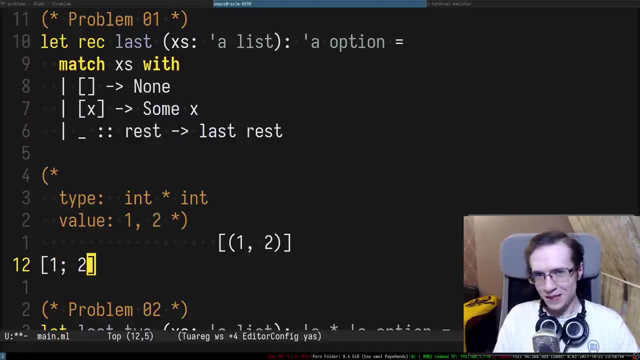 this. So yeah, It is very freaking easy If you're coming from a different language. it is very easy to make a mistake of defining a list like that and then still like looking at the compilation errors, thinking where the fuck did I make a mistake? right, Because? 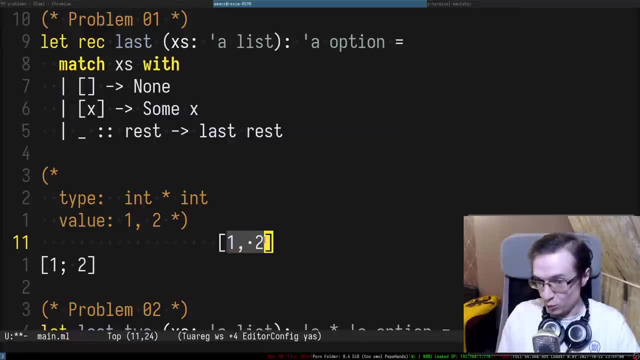 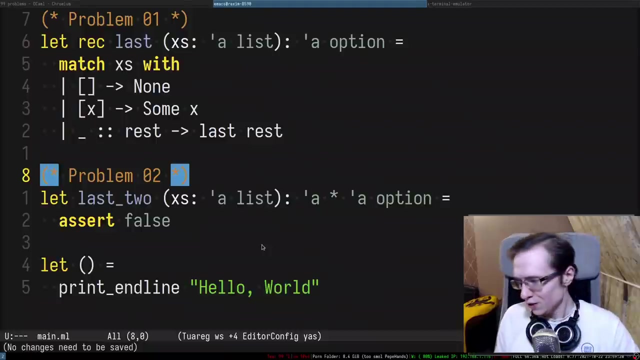 you're not defining a list with two elements. You're defining a list with one element, which is a tuple. So yeah, Welcome to a camp. So it is who it is and it isn't who it isn't. Anyway, But you get used to that quite quickly. 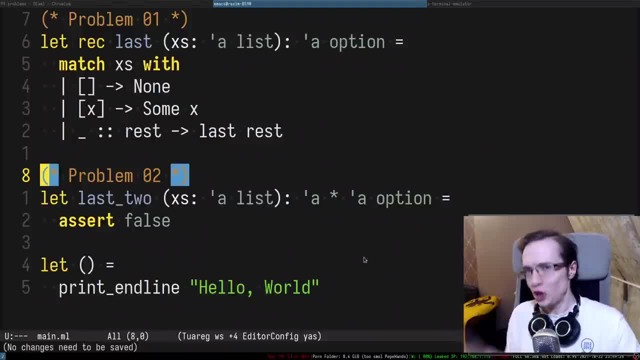 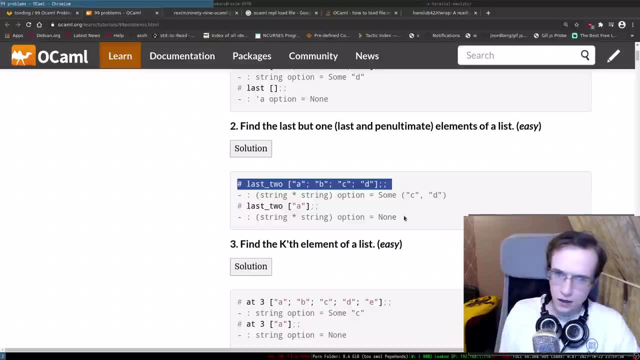 So it's just like Rust. It's like Rust: The language is not shit, You just have to get used to it. It is not shit, You just have to get used to it, Just like Rust. So now let's actually go ahead and implement this entire thing. So yeah, I've explained. 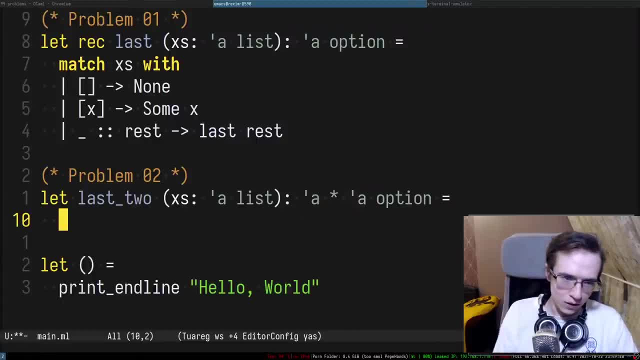 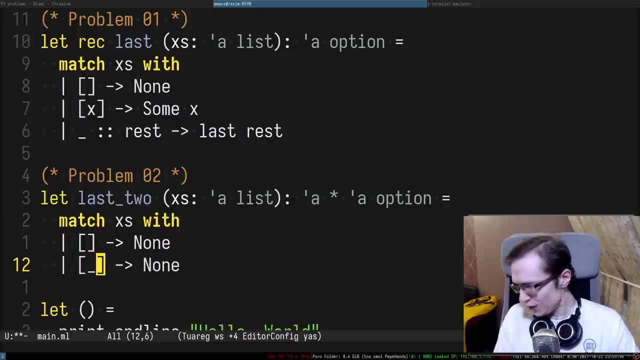 all of that just to explain what the fuck is going on here. Okay, So this time we actually have a couple of different cases. So in case of the empty list, we have to return none. In case of a single element, we also have to return none. I wonder if we can sort of 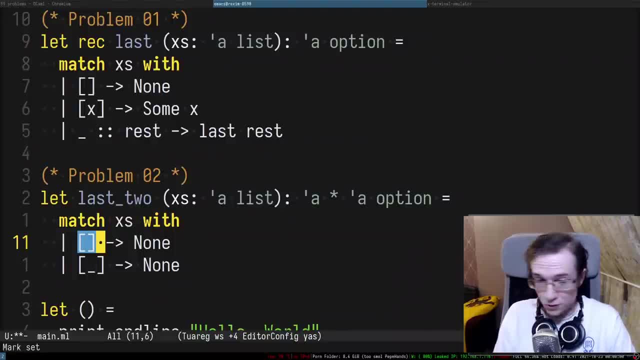 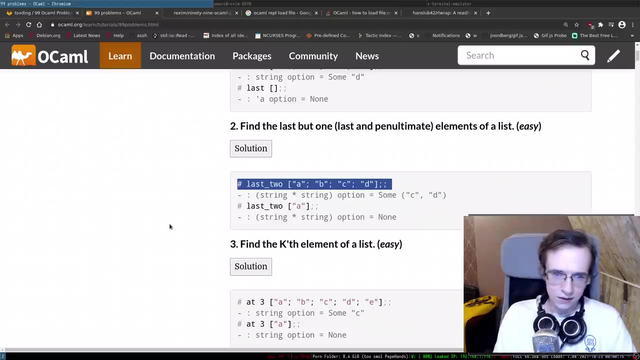 collapse? these two branches? Maybe not, I don't know. But in case of two elements, in case of two elements, you have to return those elements. So it's going to be sum x and y. There we go, So, and then what we have to do, we have to like repeat this iterative process. 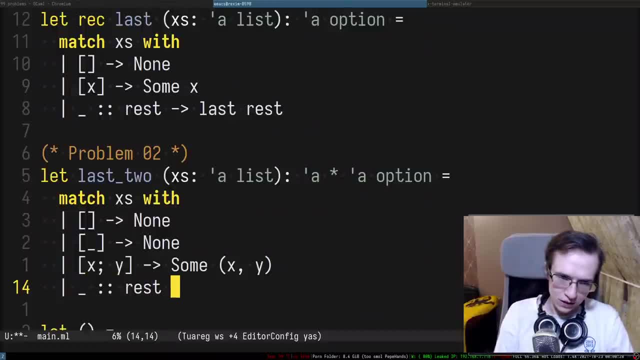 right, We're going to destructure the list into like two elements, So we're going to take the rest of the element and last two of that list is basically last two of the rest, Last two of the rest, And this thing has to be recursive. There we go, It's pretty. 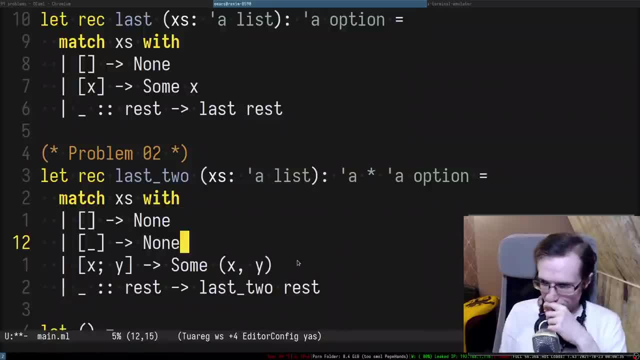 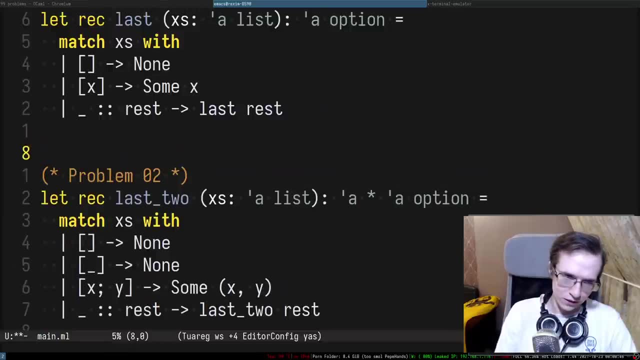 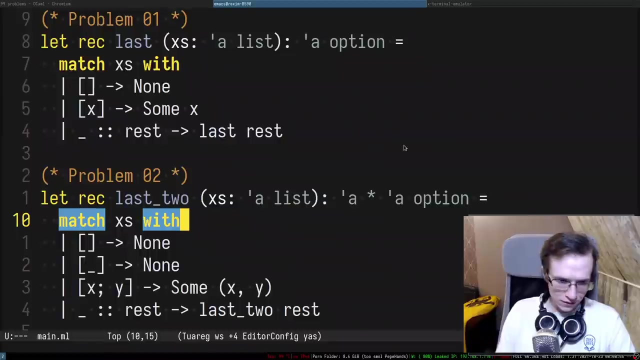 much the same solution, except we have additional case. How would you do three elements tuple? You would do it like this, Like so, Hmm, Okay, So let's see if this entire thing compiles. I'm going to try to compile and 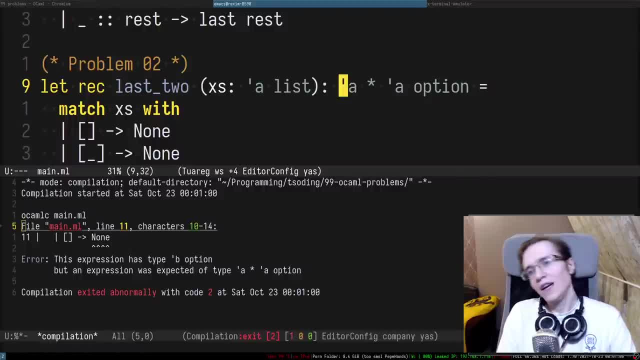 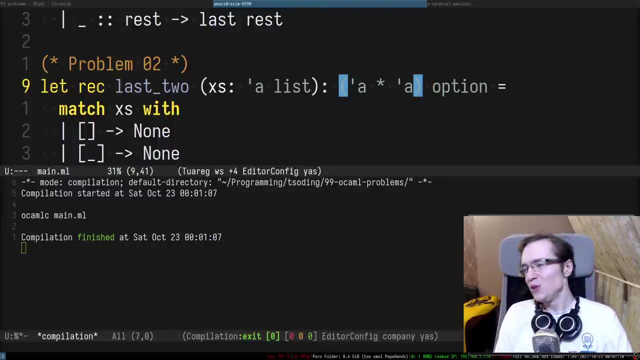 this thing returns none. I suppose I have to actually put parentheses in here, because, okay, so there is a difference. There is a difference between this and this. This is a tuple where the first element is a and the second element is optional a, If you need. 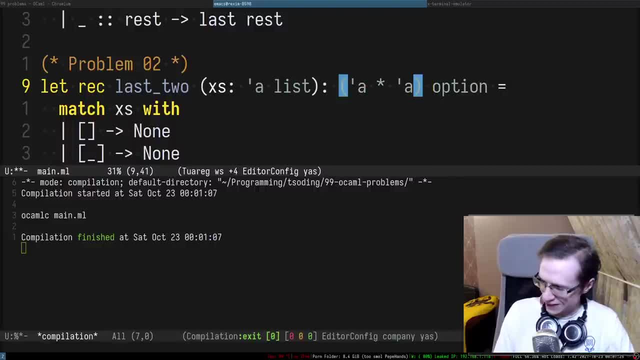 an optional element that contains a tuple of ace. you have to do it like that. You have to be careful with the order of things you define, right, Because this thing is not the same as the one with the parentheses, right? So this is like a tuple with two different elements. 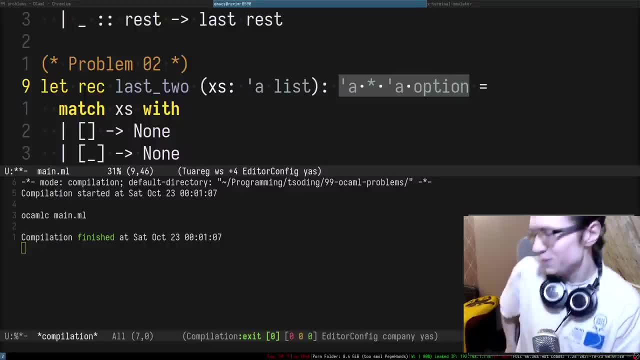 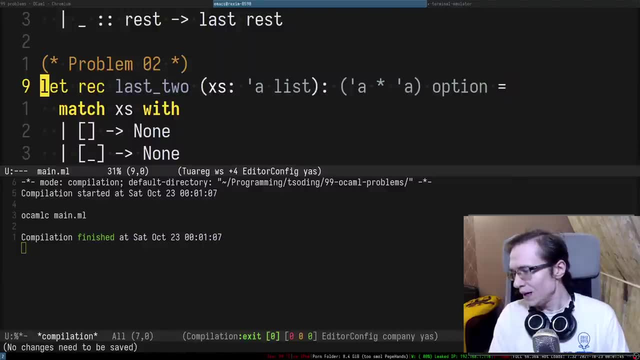 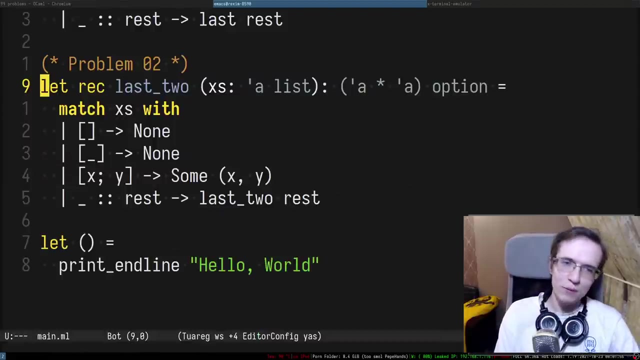 First one is not optional and the second one is optional, Right, So okay, Hmm, I always wondered the language creator's reasoning behind syntax choices. Well, the like a camel comes primarily from academic environment, and academic environment is usually quite 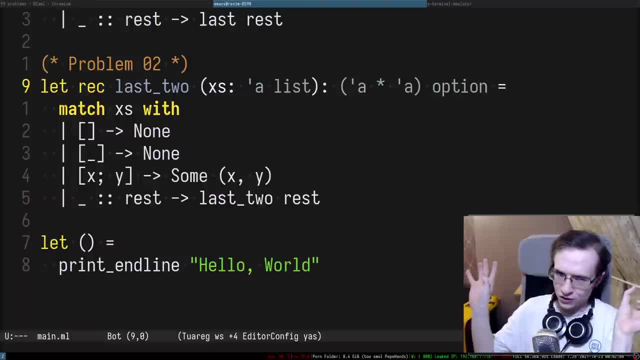 isolated from the industry and they don't care about the conventions of the industry, and that's the reason why you sometimes see the languages like that. So yeah, Right, Because people in academia don't even know that somebody programs for like, for money and for other. 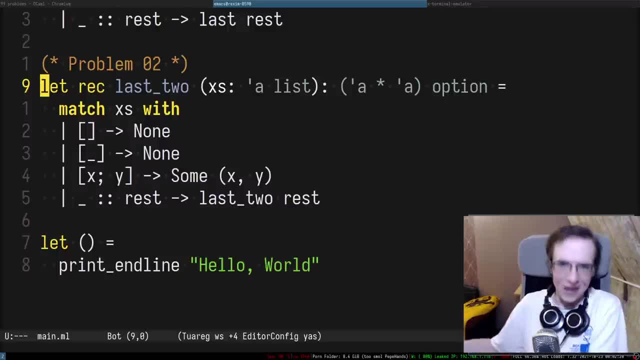 people. They think that programming is just like a branch of mathematics, right? So for like, for academic people, it's just yet another branch of mathematics. Yeah, And everything in academia. there is everything there is to programming and there is nothing outside. 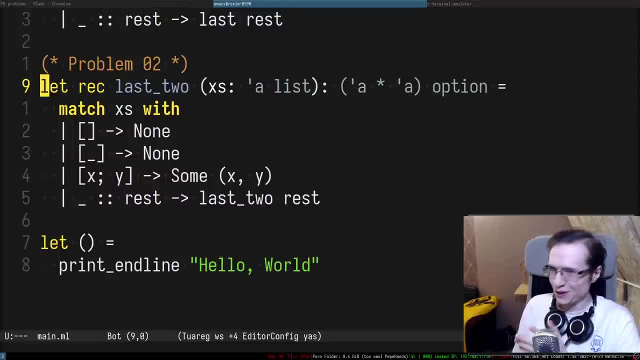 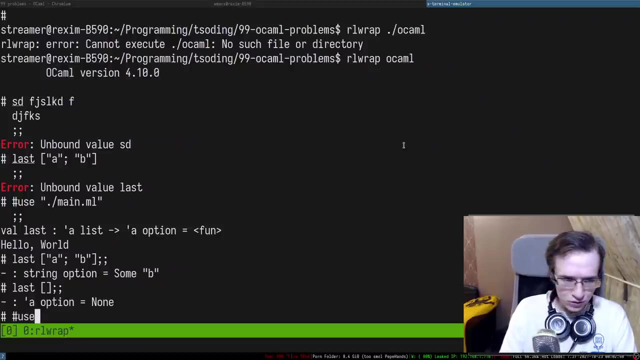 of academia in terms of programming. So that's why you end up with conventions and languages like that. So yeah, it's just another branch of mathematics, right? Just applied mathematicians, Nothing special. Anyways, I think we solved this thing right, Didn't we? Can I reuse? 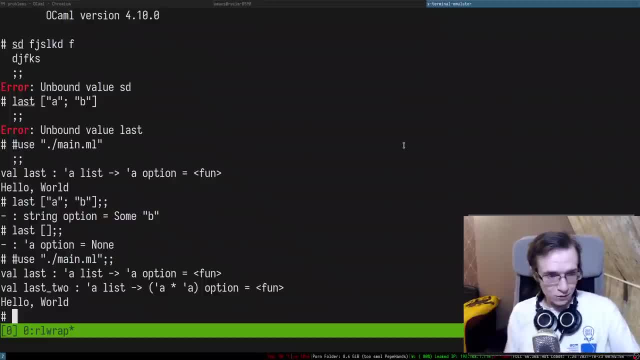 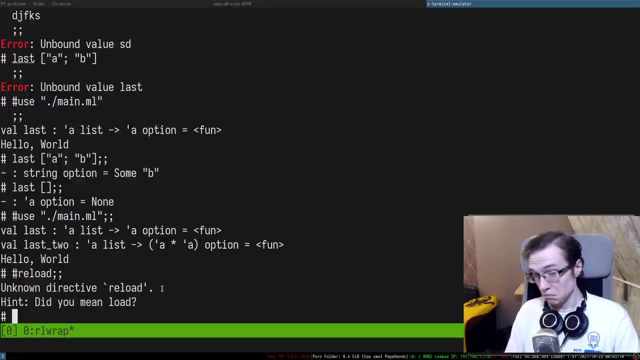 the same file And redefine some of the things I wonder I can, So I can stay in my repo and I can just update this function and just can reload them and stuff like that. Can I just reload or something like that: Unknown directive reload Did you mean? load, Maybe Did I mean. 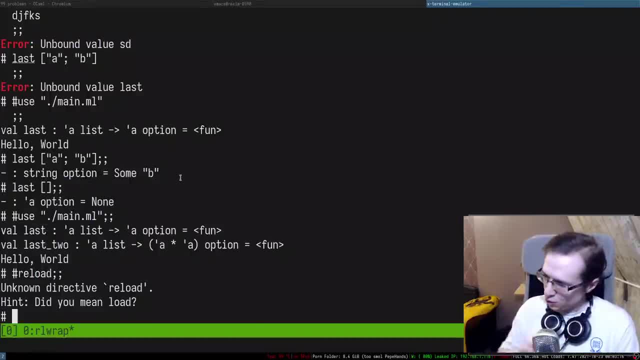 load. I don't even know what is load in terms of, like, a camel repo. I know a thing or two about a camel, but I know almost nothing about a camel repo, which is kind of strange, Okay, So, which is kind of sus, Not going to even lie. So if I try to do: Okay, Do we have? 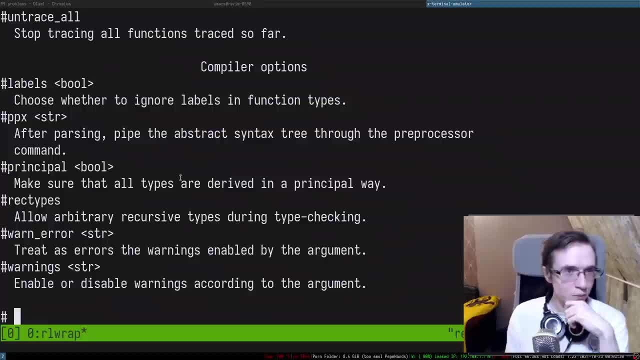 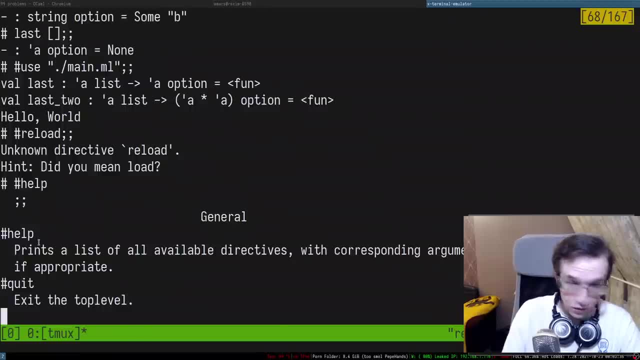 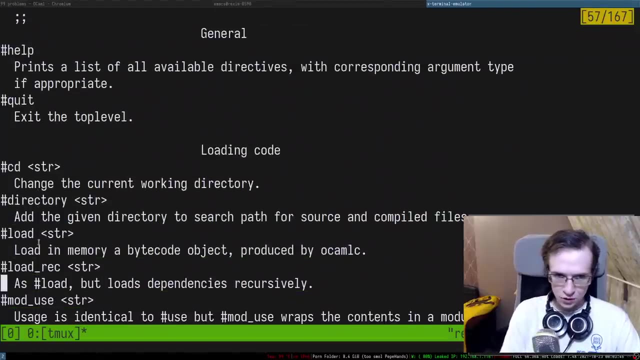 help. Do we have help? We do have help. Would you look at that? So apparently we have some shit in here, So we have help. We have quit. You can quit through the pound. You can do cd change the current working directory. add the given directory to search path for. 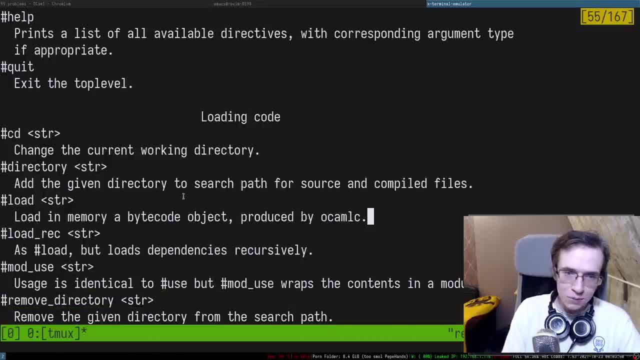 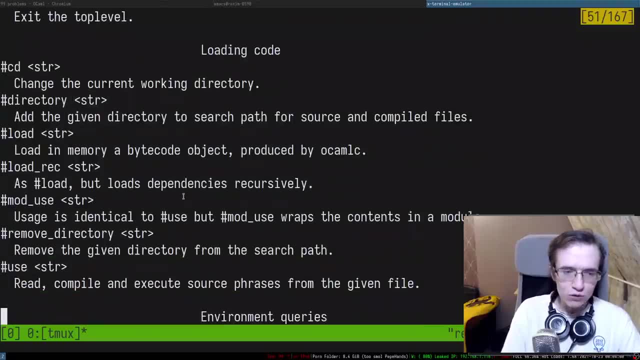 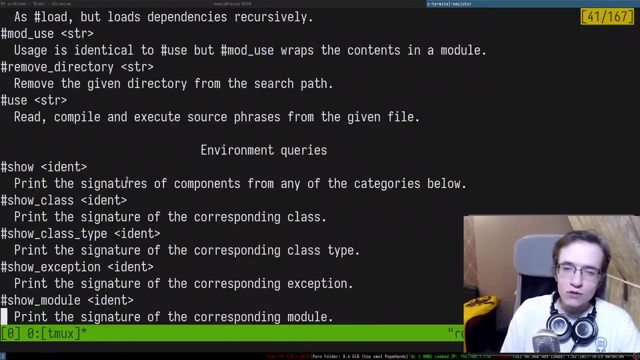 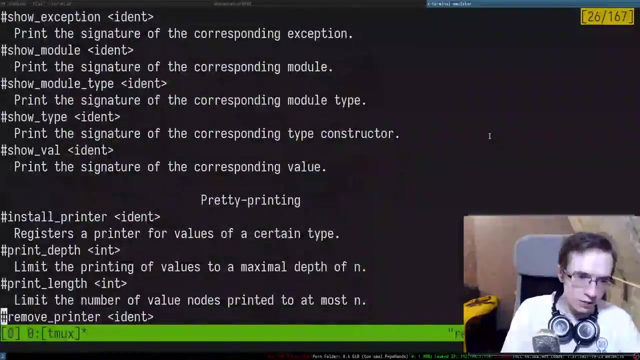 source and compiled files: Okay, Load in memory a bytecode object produced by C So you can load recursively things. You can remove directories and stuff. Read, compile and execute source files: Show print the signature of the components of any categories below: Show class, Show exception. That's. 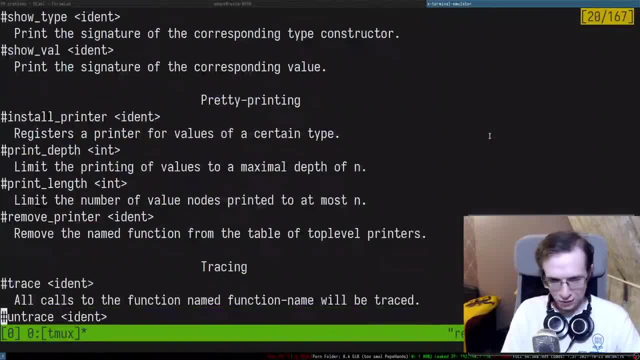 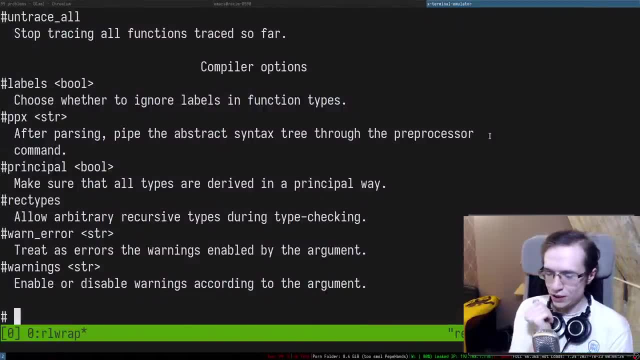 pretty cool. Okay, So I didn't know that you had so many, so many things. Anyway, even though a camel comes from academia, uh, right now, in 2021, as far as i know, it's used as an industrial language, right, so it's used quite actively in an industry and the biggest user. 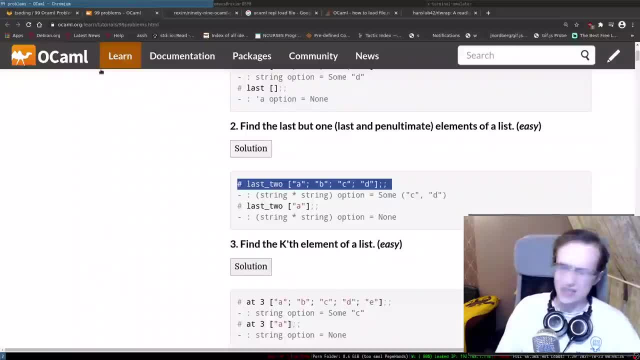 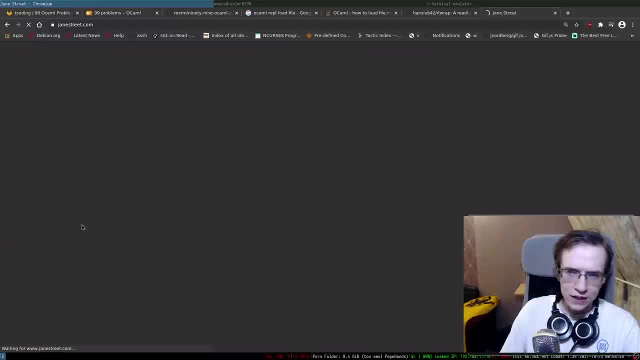 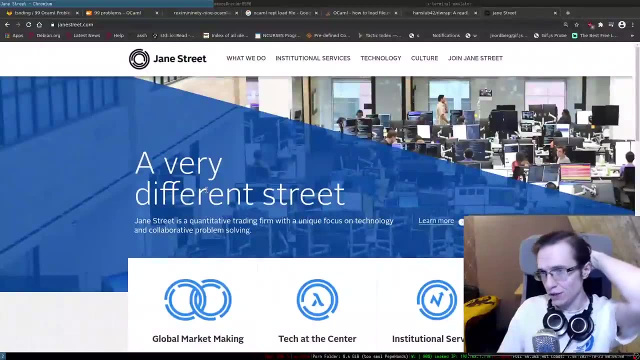 of a camel, as far as i know, is a jane street company, right, i think that that's the biggest user of a camel. uh, does anyone know about this company? uh, right, so it's basically a trading company, uh, and so one of these sort of like. uh, you know, one of the feature of that company is that. 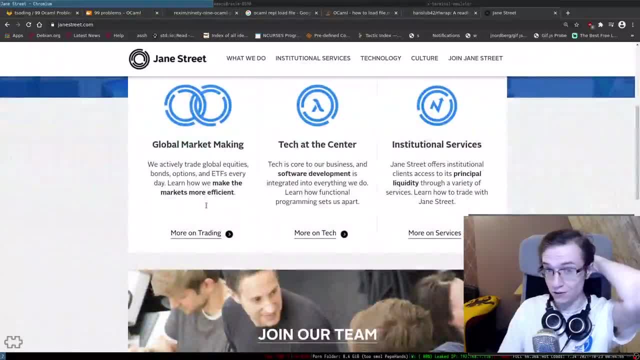 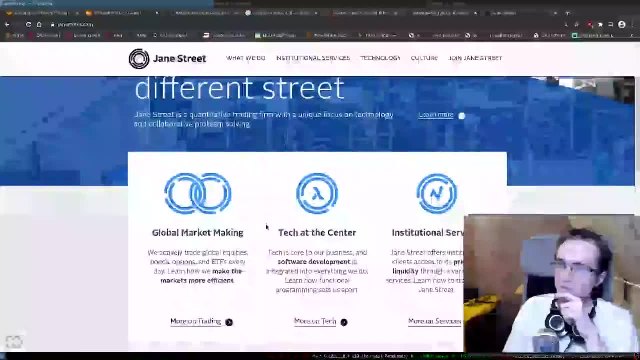 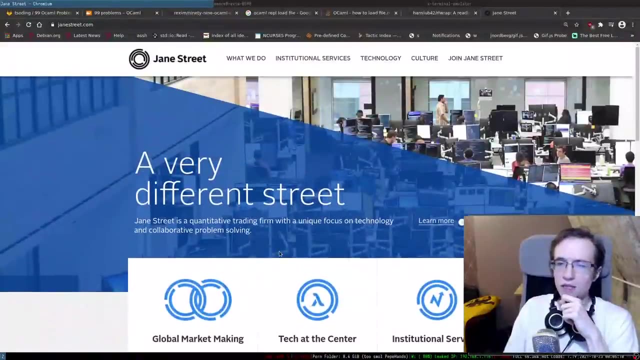 they're uh using a camel there for everything. it's just like the main language of this company, like everything is is in a camel, uh, yep. so i suppose a lot of people know about jane street if they're mathematicians and maybe watch some mathematical content on youtube like uh. 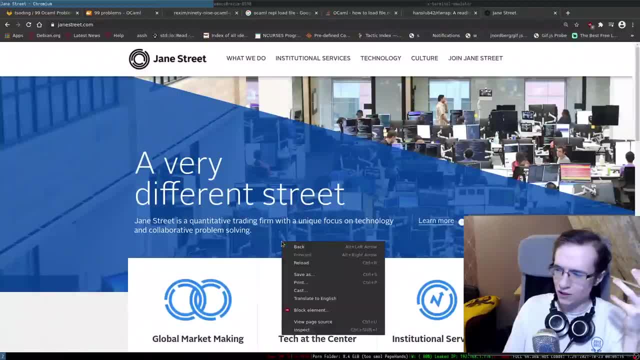 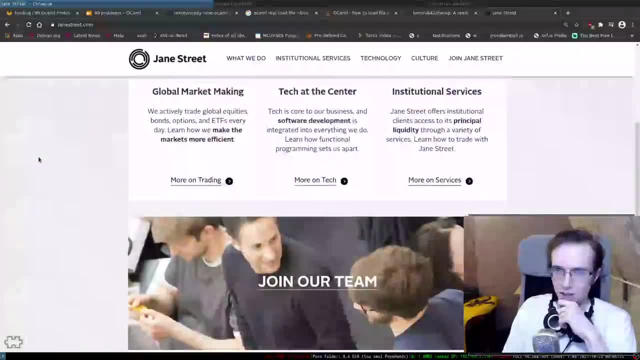 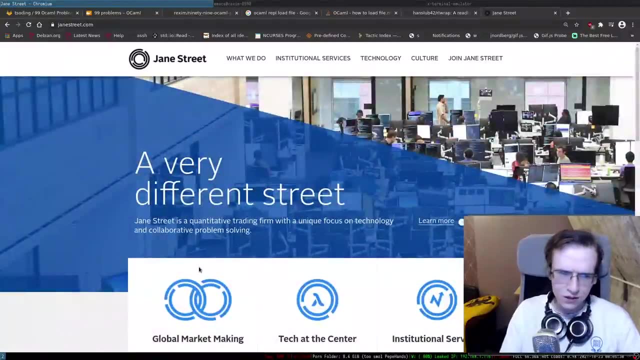 you know, stand up math. or a three blue, one brown, because, as far as i know, the math youtubers actually partner, uh, quite often with jane street, um, and they're sponsored by them to promote them as the workplace for potential like students, like something like that. so, yeah, i'm gonna leave the. 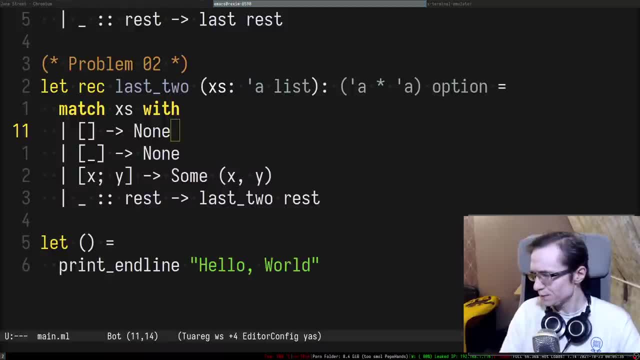 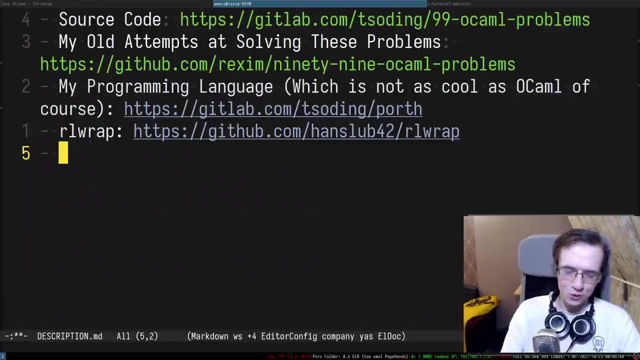 link to the jane street in the description for anyone who's interested, so i'm gonna put them in here. i'm too stupid to work in there, unfortunately, uh. so yeah, but it's uh, i heard it's a cool company, jane street, there we go, so um. 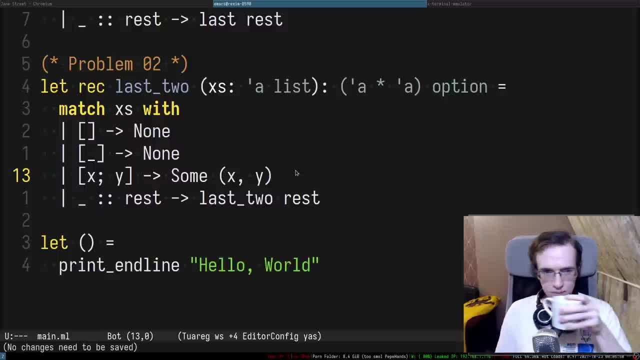 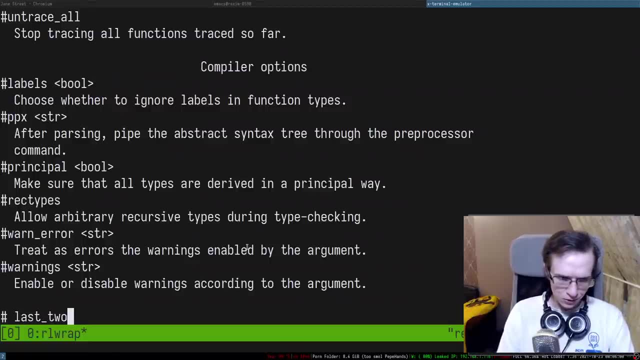 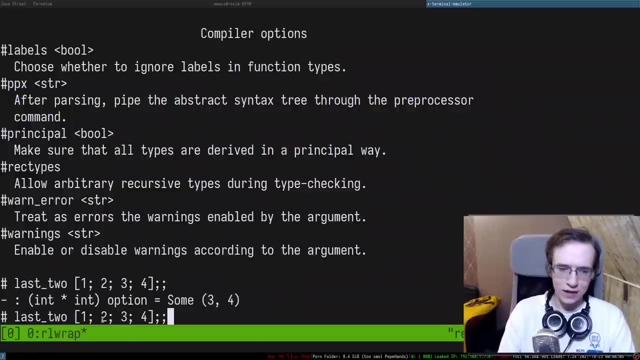 all right. so what i want you to do? i want you to test, uh, last two, right? so let's test last two. if i have something like one, two, three, four, right, it returns last two elements in here, and if you have a single element in here, it's supposed to return none. and if you have an empty list, it. 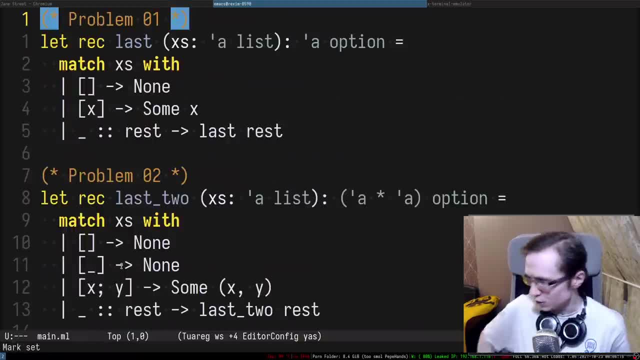 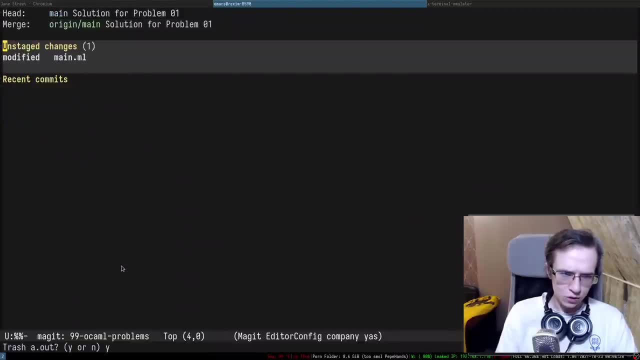 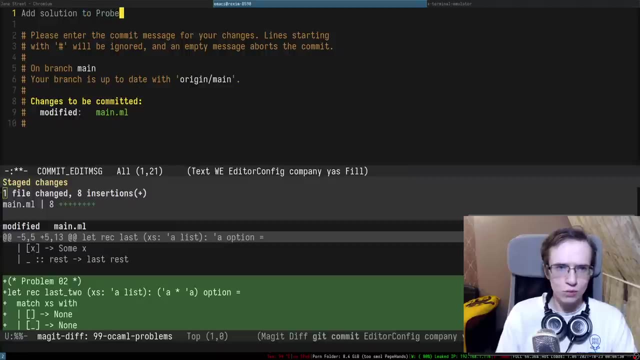 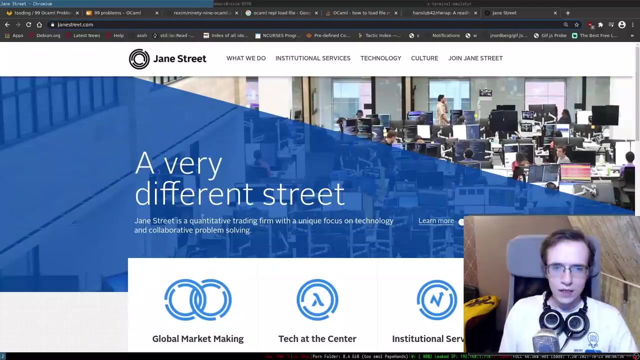 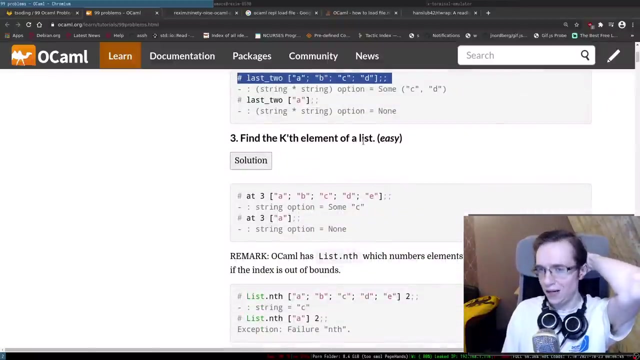 also returns none. so we basically will solve the second problem. isn't that cool? is that cool? i think it's pretty freaking cool, mate, uh, okay, so, uh, yes, okay, uh, add solution to problem. uh, problem zero two and i'm gonna push that right into the repo, okay, so what's the next problem? so we have 97 problems to go find the cave element. 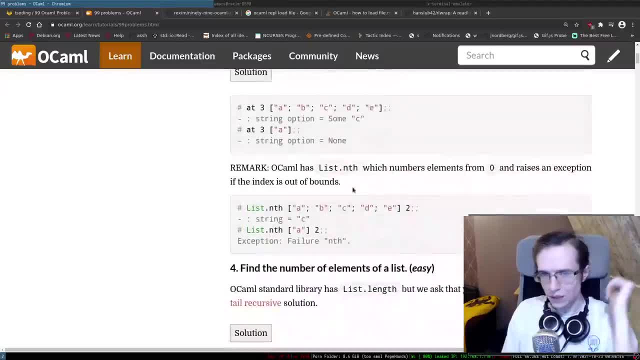 of the jane street and we're gonna put it in here and we're gonna put it in here and we're gonna push that the list easy. okay, so you have to define a function at which accepts the number and the list and returns you the nth element of that list. so in our case, three, uh, it will return one, two, oh. 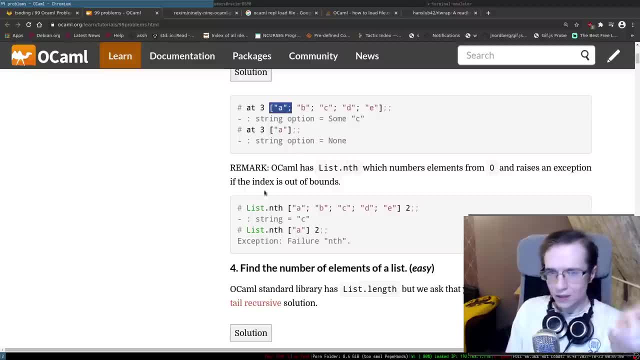 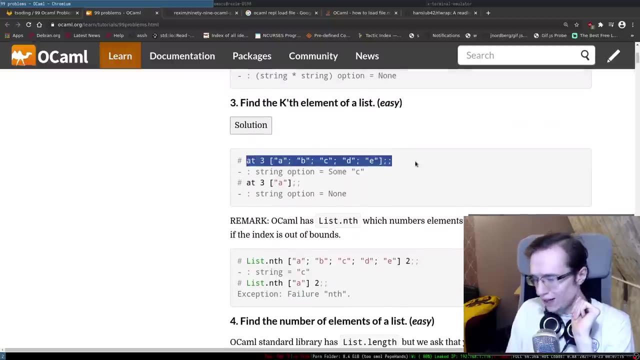 it even starts with one okay remark: a camel has least nth, which numbers elements from zero and rises. an exception if the index is out of bounds, right so and so people, to make people not use nth as a solution. this thing doesn't rise exception and also starts with one disgusting uh anyway. 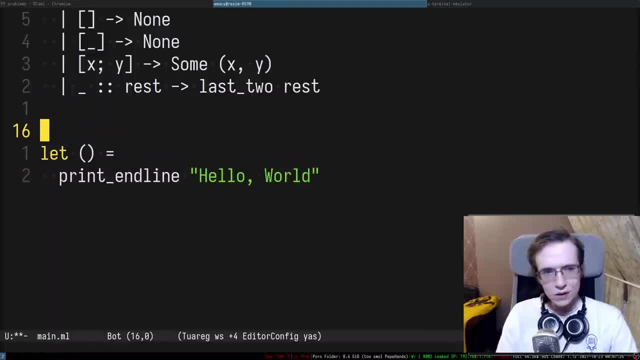 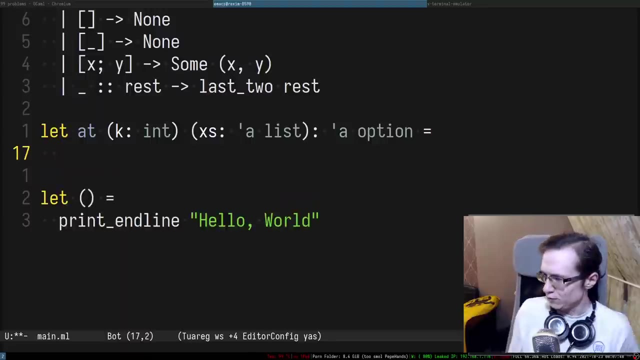 let's go ahead and implement this thing. okay, so we need to implement at. so, as you can see, it accepts uh integer k and uh list uh of ace and it's supposed to return uh optional a right. there we go, so we have to implement this thing. 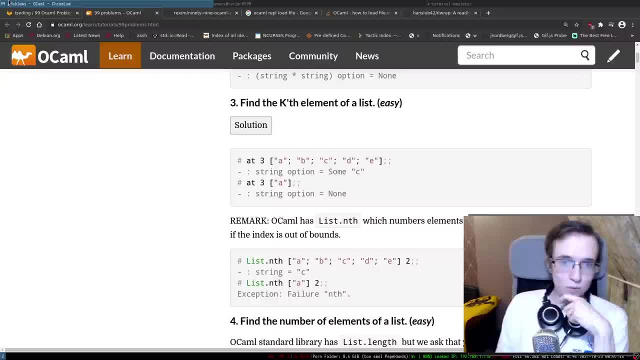 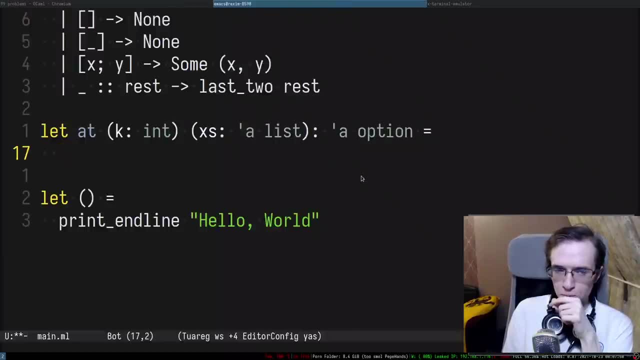 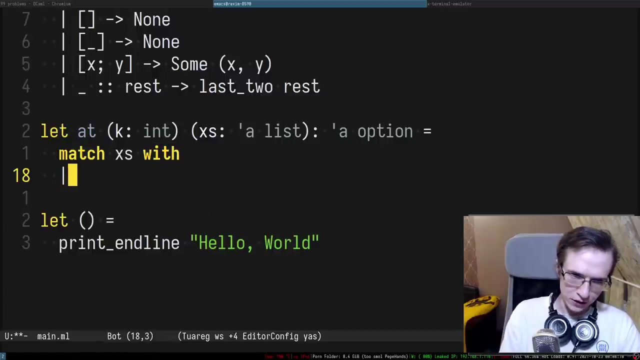 um. i wonder, if you provide zero, i suppose it also should return like none um um. so we have like a couple of uh situations like if k is oh boy, oh boy, oh boy, where is my soy, i guess we could match access like so. right, uh, you can match access like so, and in here you're gonna have 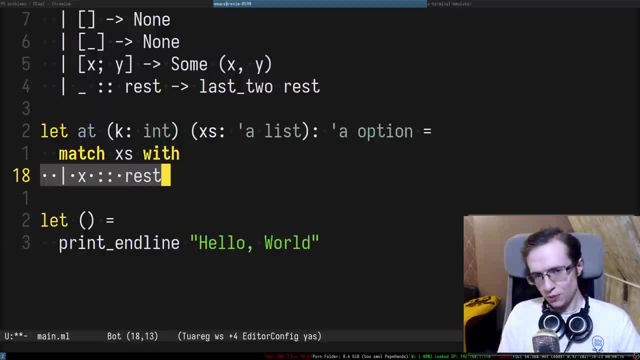 x and rest, if i remember correctly, on top of having the um, the patterns in pattern match construction, you uh can have like guards, right. so here is the pattern and there is also additional condition, and i think it's something like that. so when access has this particular pattern, 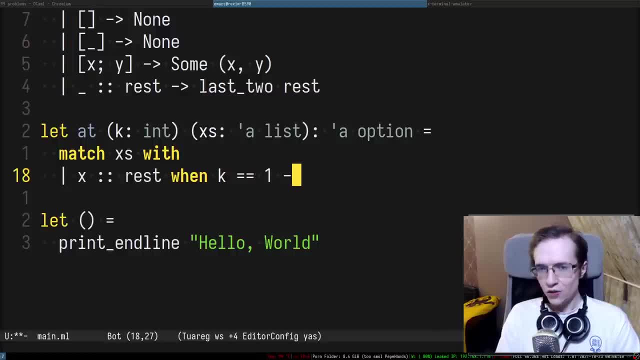 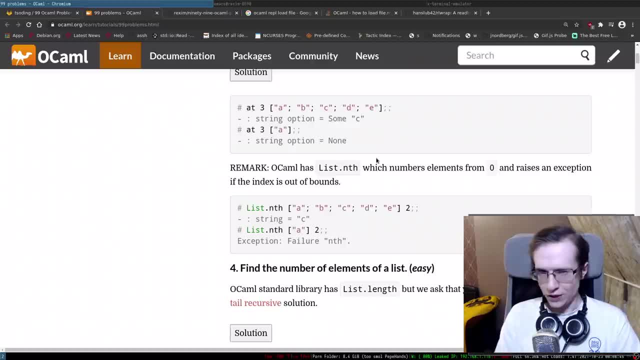 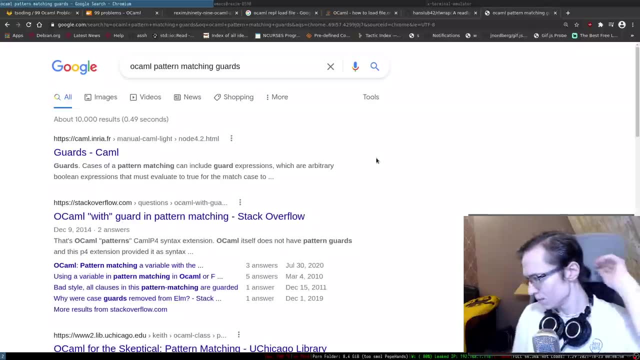 when access has this particular pattern and when access has this particular pattern and when access has this particular pattern, return x. but i don't remember for sure, right, so i want to actually google it up: a camel pattern matching and i think they're called guards matching and i think they're called guards. guards. it's like modes. oh yeah, there we go, so you can create different patterns for various types of games. of course, which is just not a great idea to test a bunch of time for you and your power points. so i hope you enjoyed this video. if you enjoyed it, please share it with your friends and, of course, a big thank you to everyone who's been watching this video and i'll see you next time. 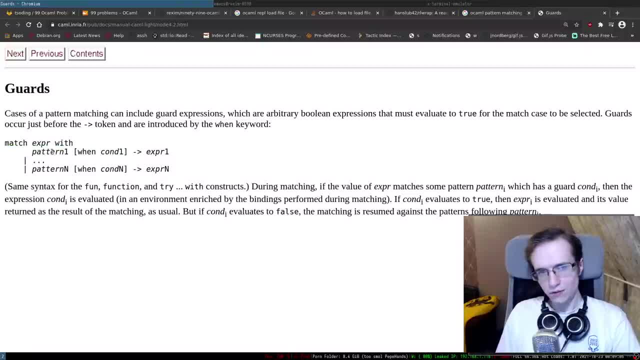 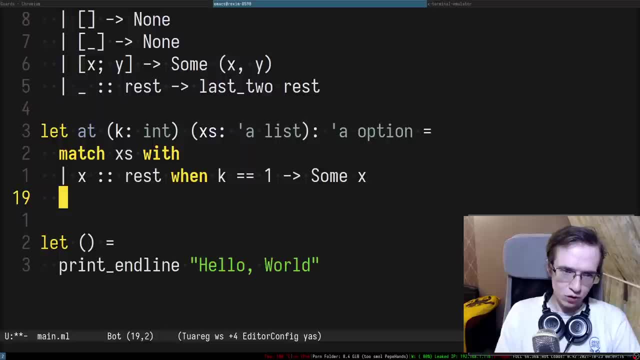 modes. oh yeah, there we go, so you can have a pattern and then you can have one with condition. pretty cool, it's pretty cool, uh, okay, so if we have um, just uh, something else, well, i mean, we have several situations right when um, uh, k is less than zero. right, when k is less than zero and when k is greater than one. 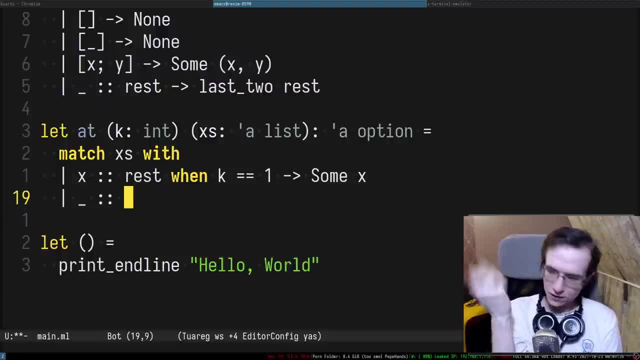 in all of those cases, we want to actually go to different places, right, so, right. so in case of uh k, like less than one, this is a straight up, none right, because you cannot go, uh, less than one. um, you cannot go less than one. but if it's greater, uh, you want to actually recur. you want to actually recur. 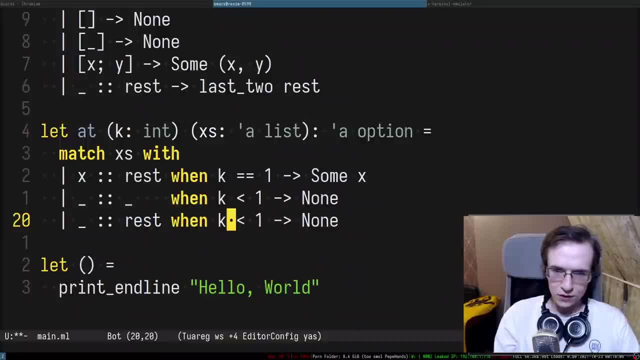 so, in case of um, this thing, if it's greater than one, if it's greater than one, you want to do something like at uh k minus one, uh, rest there, we go. so, and if you end up with an empty list for whatever reason, right. so with an empty list, uh, this is also none. 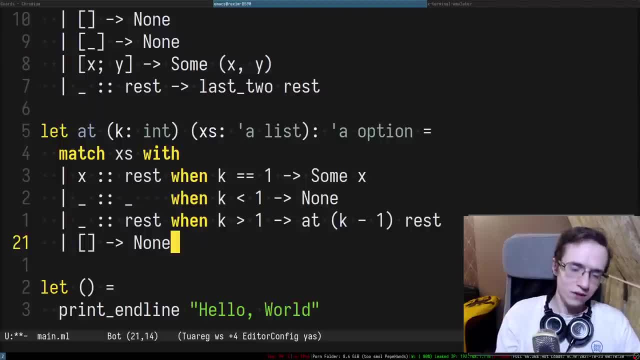 um, essentially so. can we simplify this entire thing? uh, we could probably move all of these conditions inside of this branch, um, but i don't know. is rest a special match word? no, it is not actually. it's just like um, it's just a name for a variable. 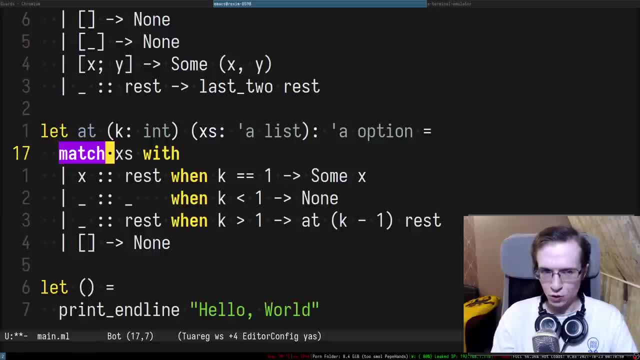 right. so basically i'm bounding the first element of x's to uh x and the rest of the elements except x to word rest. I can call it something like wise, And it's going to be the same. What's interesting is that in here we don't really care about rest, So I can do something like this: 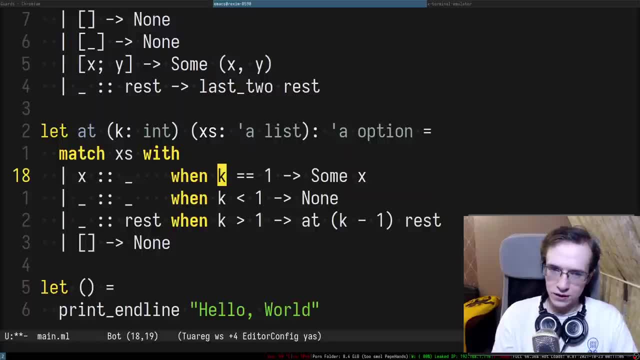 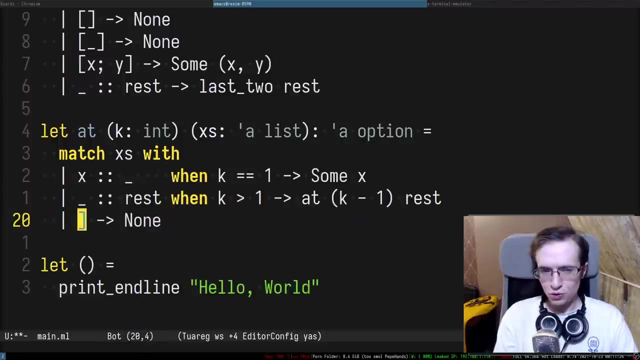 right. So, yep, if k is one and you have, like, at least one element in here, you can return that element. If, for whatever reason, for whatever reason, k is less than one, you have to return none. Interestingly enough, maybe we can even remove this case and just put something like: 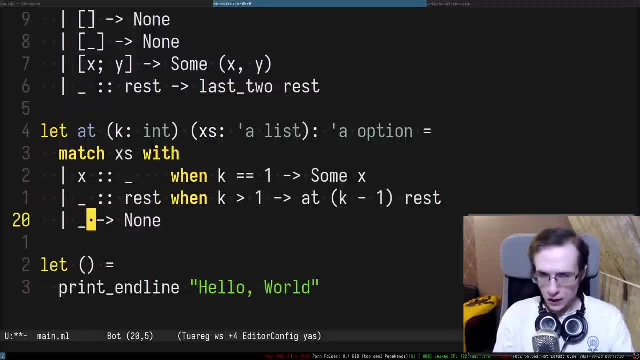 this in here And I think that will work. Yeah, this is actually greatly simplifies the situation, right? So if you have at least one element, k is equal to one. the result is that element. If you have more than one element, but the k is greater than one, you recur with k minus one and 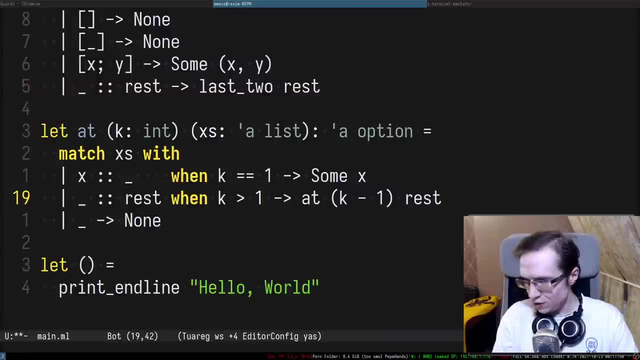 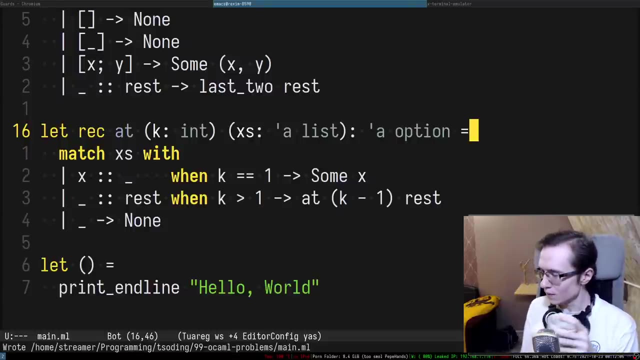 the rest of the element. If your list is empty or k is less than zero, well, in that case it's just like a straight up: none- There's nothing to do in here. There's nothing to do in here. That is very interesting actually. 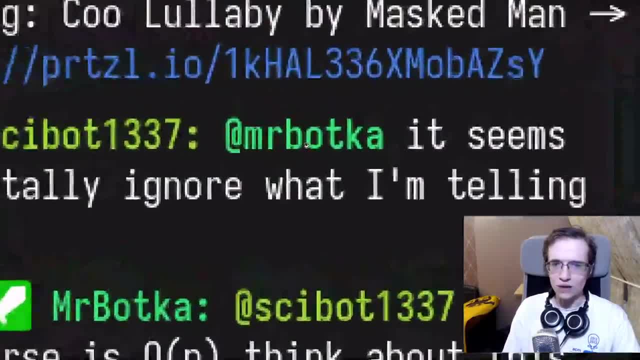 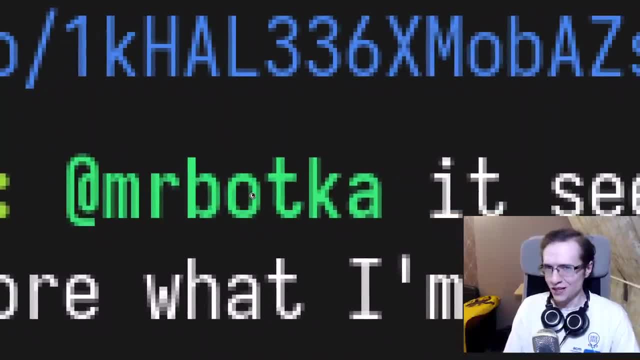 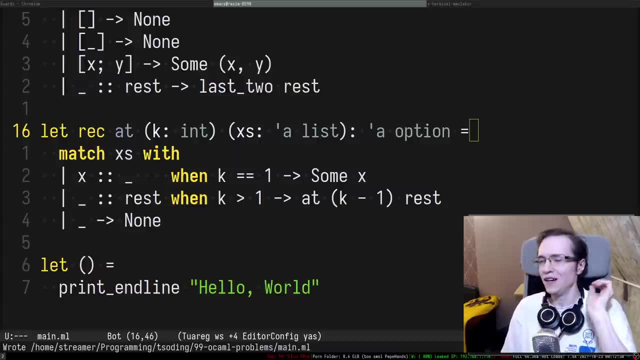 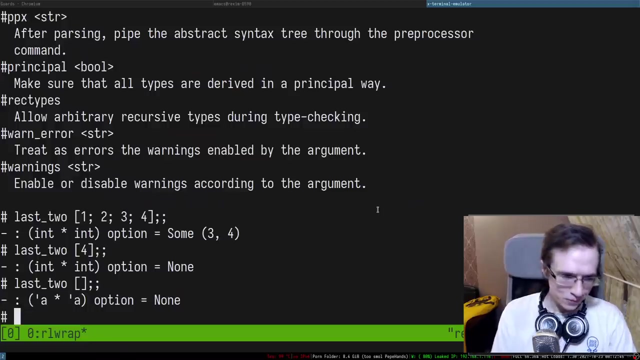 This channel, So it does, in fact, ignore everything you say, because it's a bot. I'm really sorry to tell you that, But I think, like I don't like to be that guy, But I think you need to know that Mr Vodka is a bot, All right, so let's see, Let's see. is it going to work, Can? 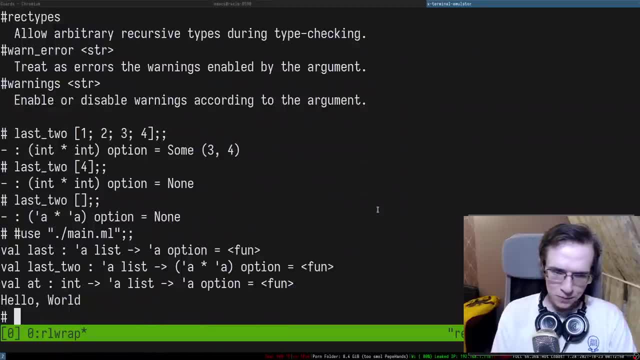 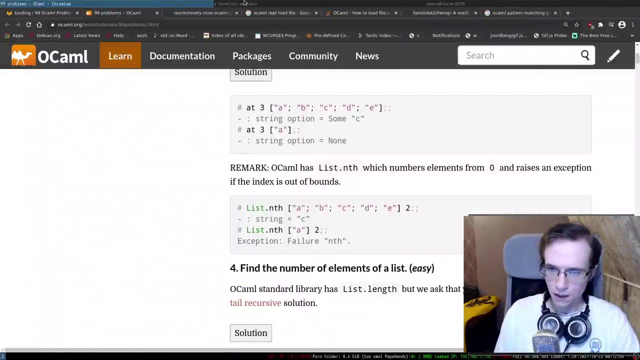 actually just like: do use Yep, yep, yep, And it seems to be working. So let's take a look at some of these test cases in here: 99 problems. I might as well just like: do that, And this thing should return some C. And, as you can see it, 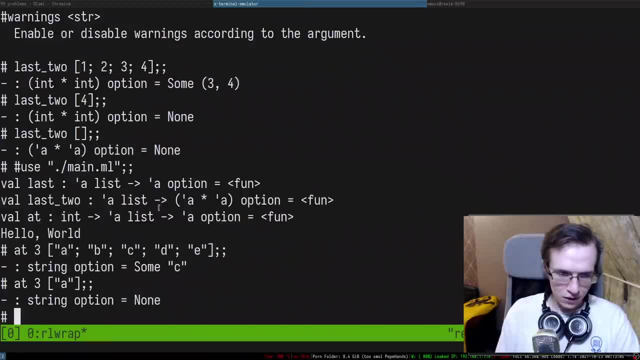 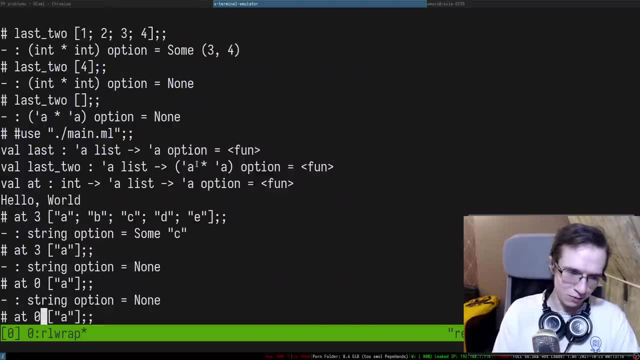 returns some C. if we're going to do something like this, it returns none. And furthermore, if I try to do zero, it also returns none. right, So that makes sense. But if you do one, it returns some A. I think this is a reasonable solution for this problem. What do you guys think? 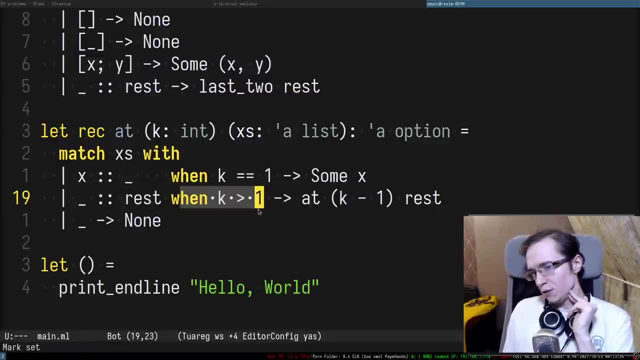 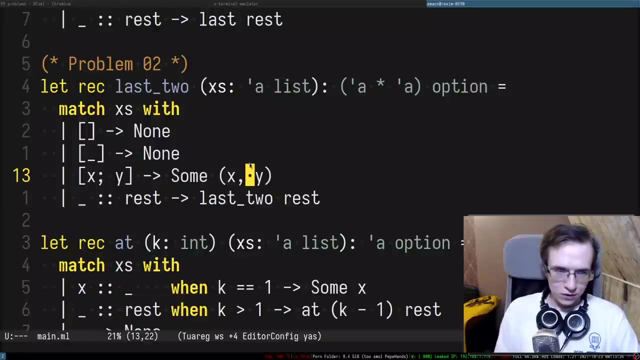 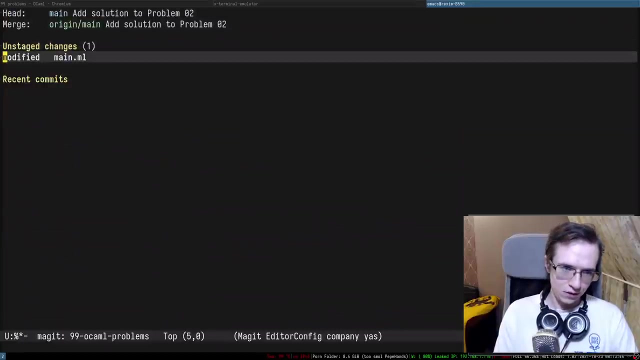 I think this is, in fact, a reasonable solution. Maybe you can compress it even further, right, But that's fine, It's fine, All right. so this is a problem, problem 03,, problem 03.. And let's go ahead and just commit. 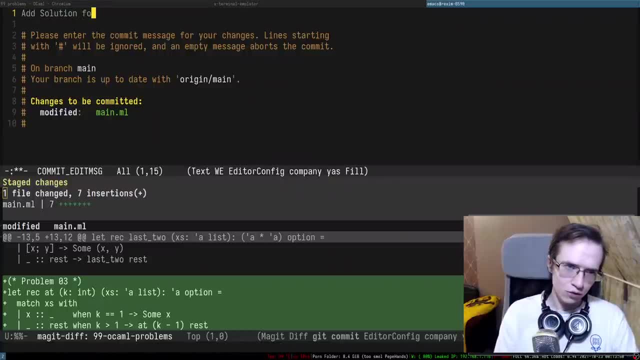 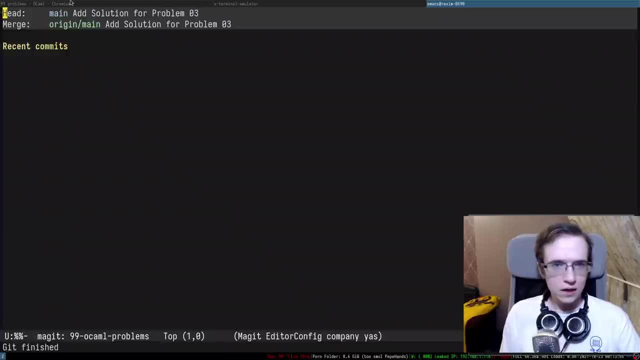 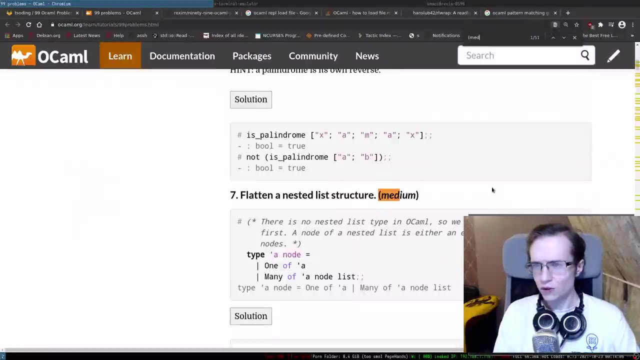 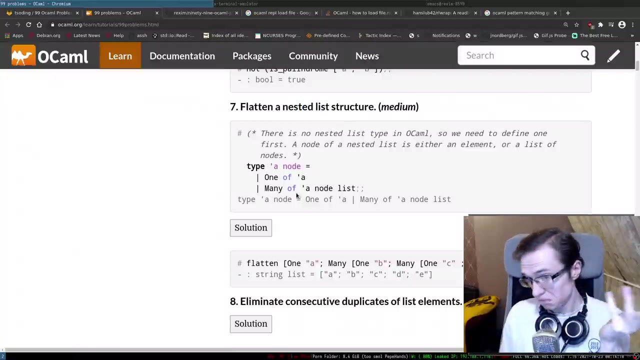 that Add solution for problem 03 and we're going to push that right into the repo. so what's going to be the next problem? so far, so good. so far we only have easy problems and as far as now there's also medium problems and the medium. the first medium problem is flatten nested list structure. it's actually 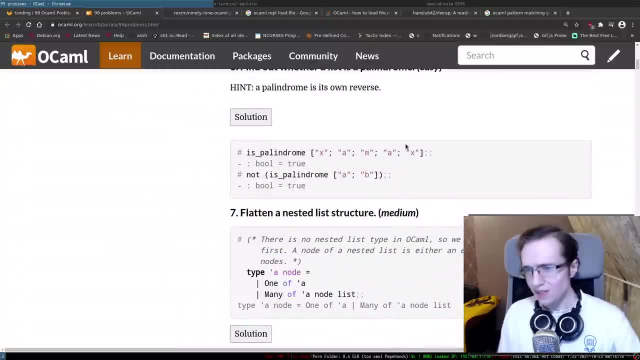 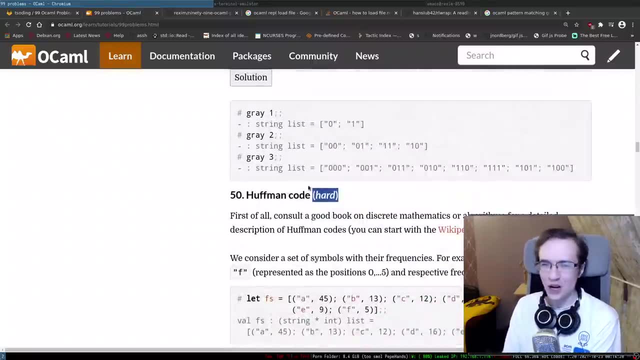 not that much difficult than the previous values. what is the first hard problem? uh, that's a quite a quite of a jump. i mean okay, between flattening the structure and halfman codes. i mean halfman codes are not that hard, but between flattening the structure. 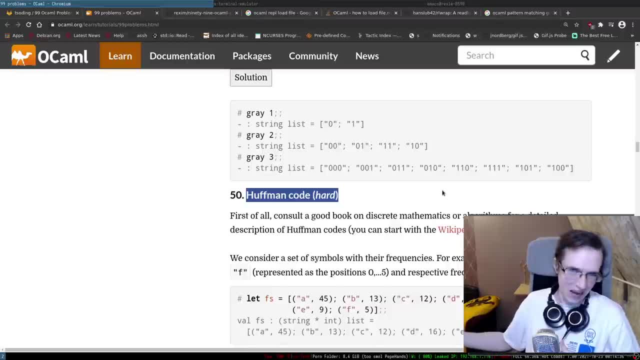 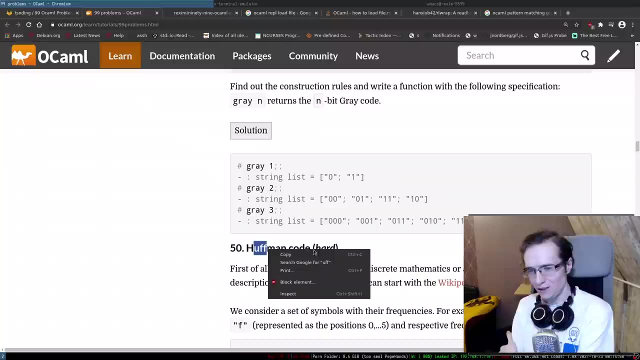 and implemented halfman codes, it's there's a quite a bit of a gap. it's not as much of a gap as between easy and medium, i'm not quite sure- and actually the first hard problem is actually 50. one. So, to be fair, I planned to implement Huffman codes as a separate stream topic, actually. So 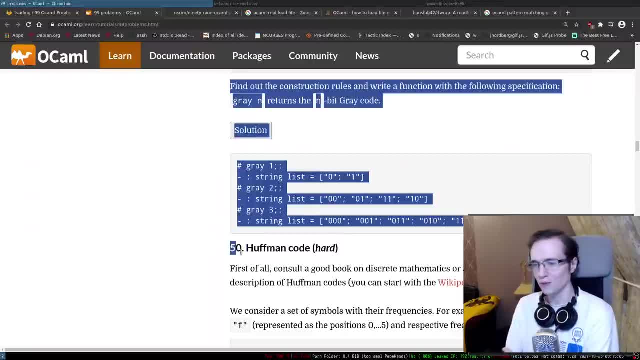 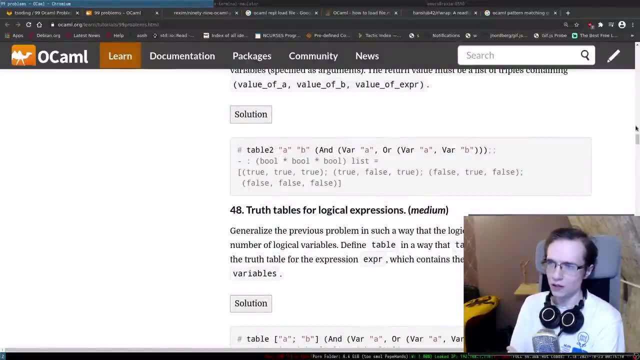 will be interesting. I don't know if we're going to actually get the 50th problem- It's actually it's a halfway through- But Huffman codes are actually very interesting. I remember implementing them when I was a student And they're really really fucking fun. So the idea. 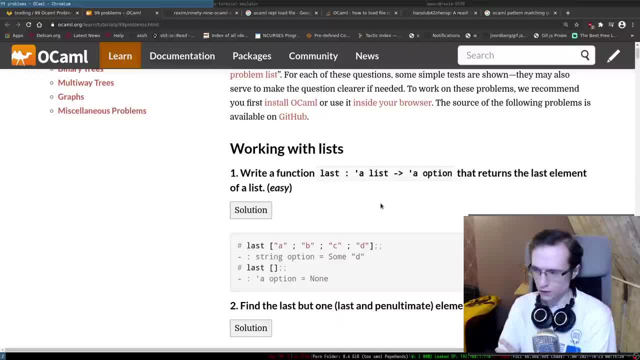 of Huffman codes is like: essentially, you have a sequence of like of bits And the most common, the most common sequence of bits, it should be represented with the shortest sequence of bits. And basically you gather, you build that substitution based on the statistics of the 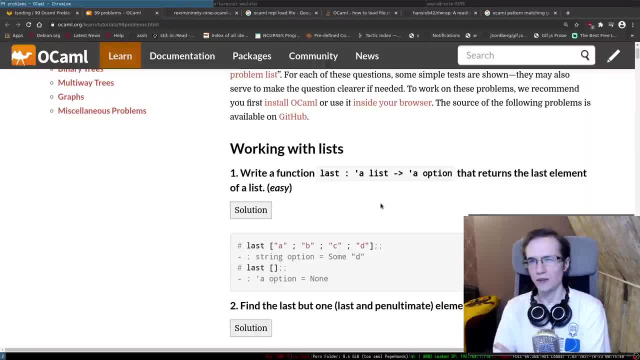 sequence of bits And you do that with a tree or something. Yeah, I think I quite remember, like roughly remember. So I probably need to read on Huffman codes a little bit more, But they're quite like they usually used for compressing stuff. Huffman code is small on the camel: Okay. 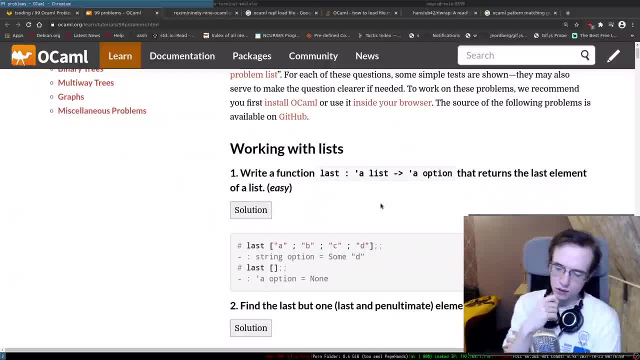 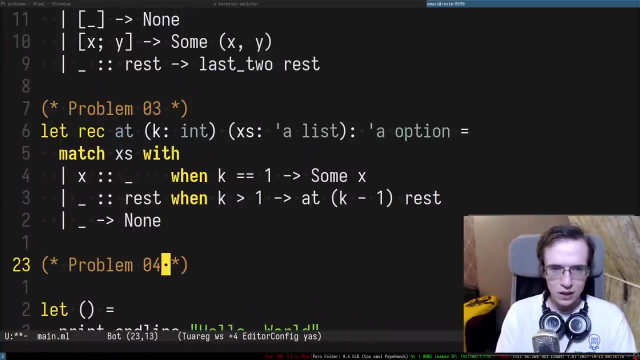 so maybe that's why they put it in there, Because maybe the functional approach works really well with Huffman codes. Okay, so what's going to be the next problem? right, Next problem is going to be something like a problem 04, problem 04.. 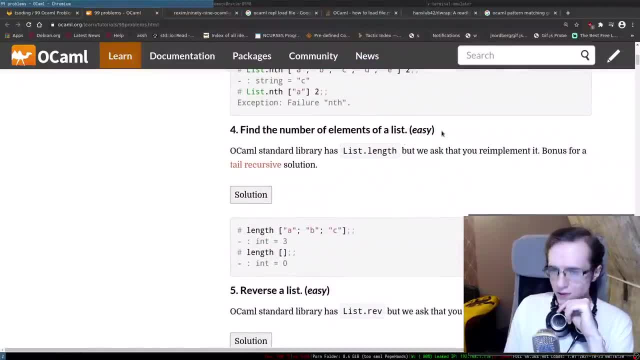 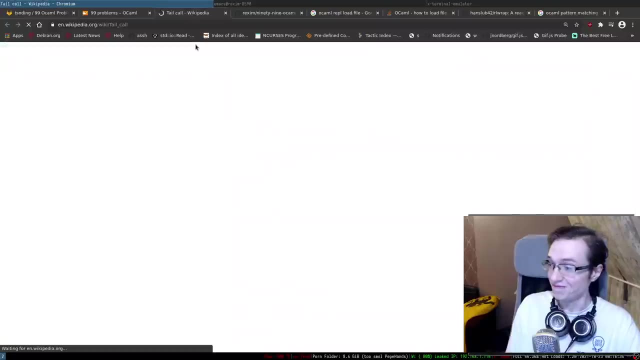 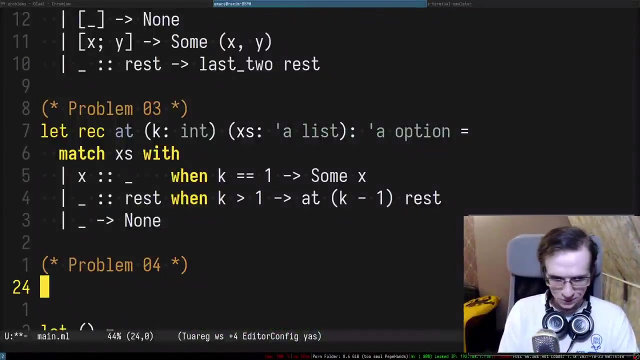 Find the number of elements of a list Easy, Okay. okay, most time the library has least length, but we ask you that you re implemented a bonus for a tail recursive solution. Oh, who knows what is a tail recursion? Tail recursion under tail recursion. So let's go ahead and try to do that. So this is going to be. 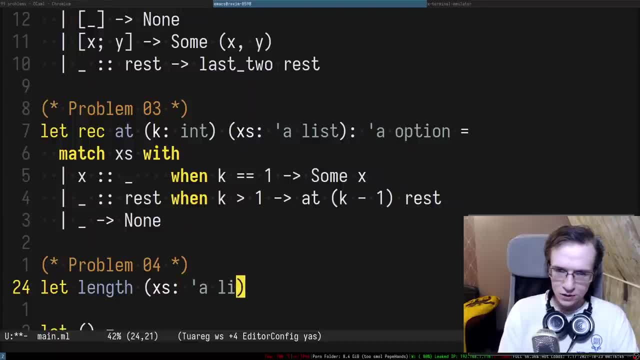 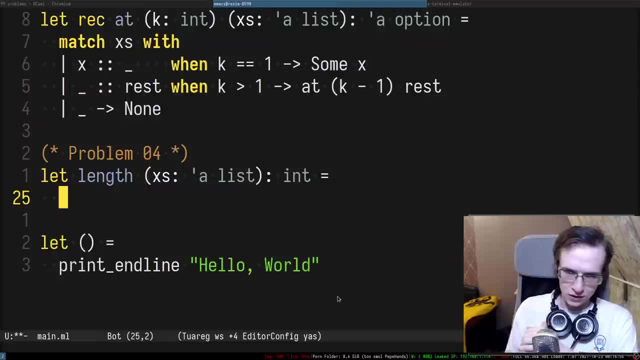 like a length, And in here we're going to accept the list, right, And this entire thing is going to return an integer. Okay, How would you implement the such function? Right? So let's go with the recursive approach. Yet again, we're going to match access, right. And what's the simplest case? What's the 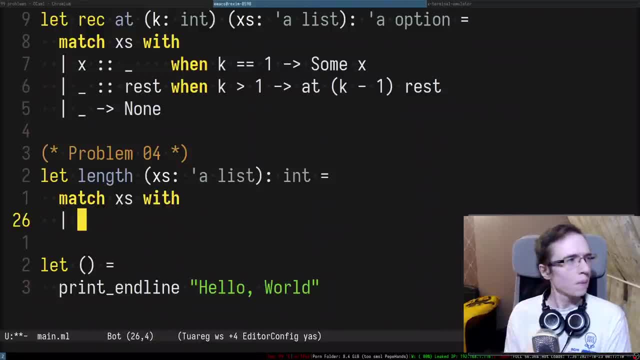 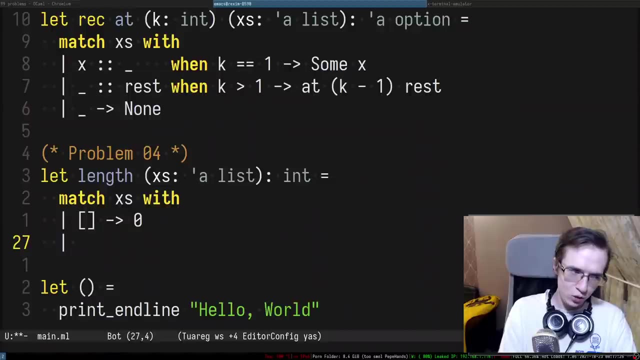 simplest list, the length of which you can calculate easily. Let's put it this way: I suppose it's a empty list, right? So if you have an empty list, you can straight up say that the length of that list is zero, right? If you have a list where you have more than one element, right? So the length 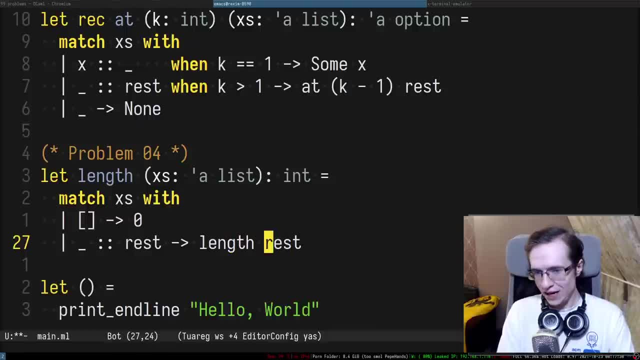 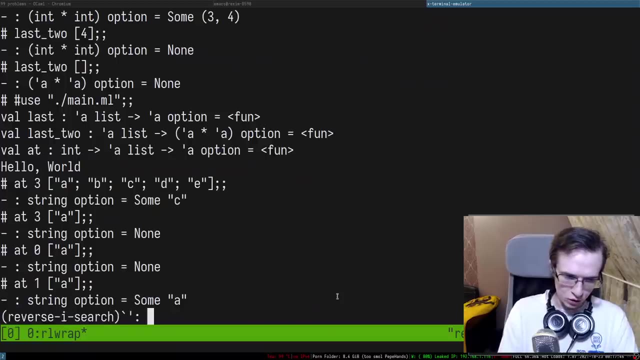 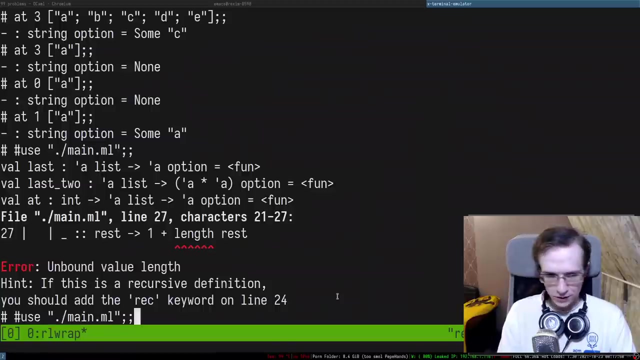 of such list is going to be the length of the list without the first element plus one. There you go. We implemented a very simple function that calculates the length of the list recursively. So let's actually do use- And it doesn't compile yet again, because you have to mark this function as a recursive right. 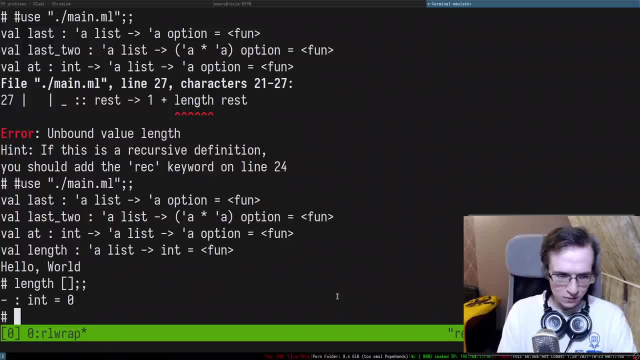 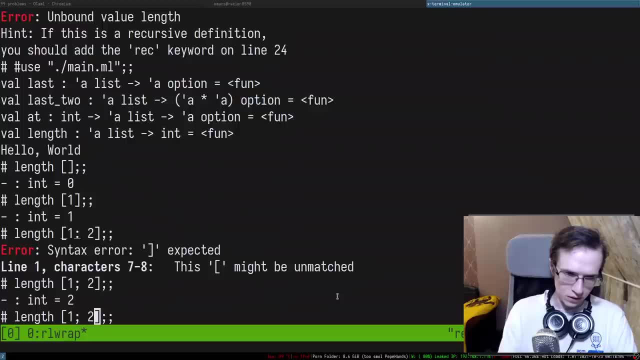 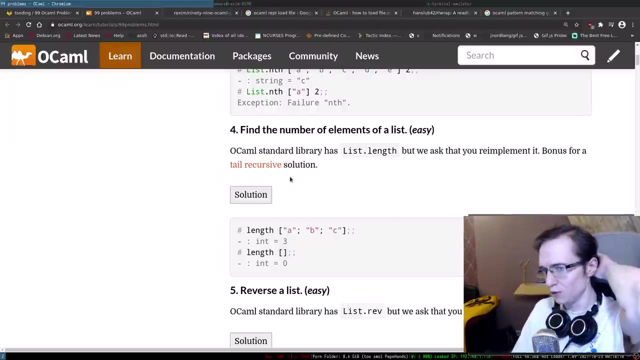 So, and let's do length, And I'm going to provide the empty list. It is zero, one, two- I'm sorry- three, and so on and so forth. Right So, but they also promised extra bonus for tail recursive solution. Who knows what is a tail recursion and how? 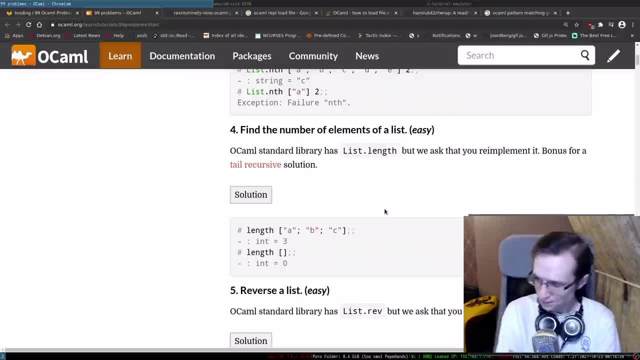 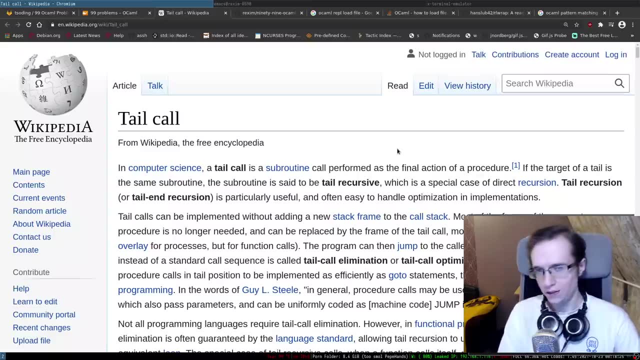 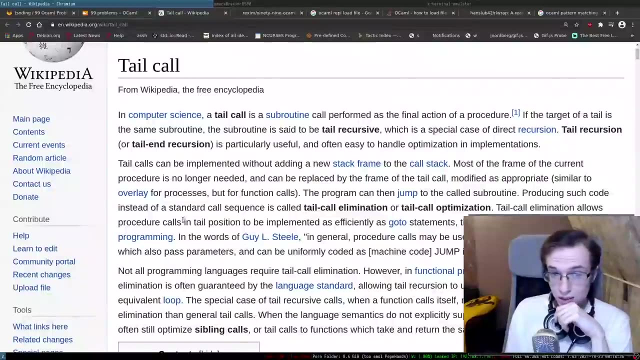 you can implement this thing, tail, recursively. Who knows what it is? So they even provide the link to Wikipedia article about tail call. So let's actually read about it. So I don't know what is a tail call. right In computer science, a tail call is a subroutine call performed as the 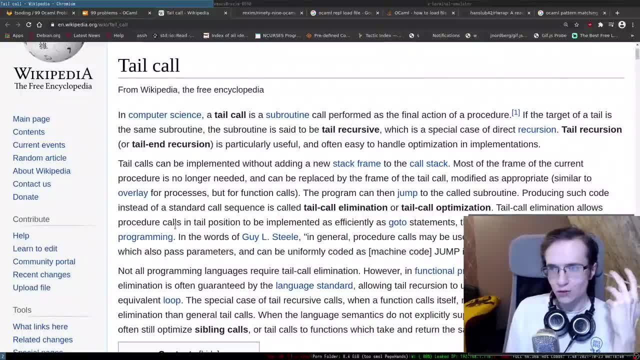 final action of a procedure. If the target over tail is the same subroutine, the subroutine is set to be tail recursive, which is a special case of direct recursion. Tail recursion or tail end recursion is particularly useful and often easy to handle. optimize optimization in implementations. 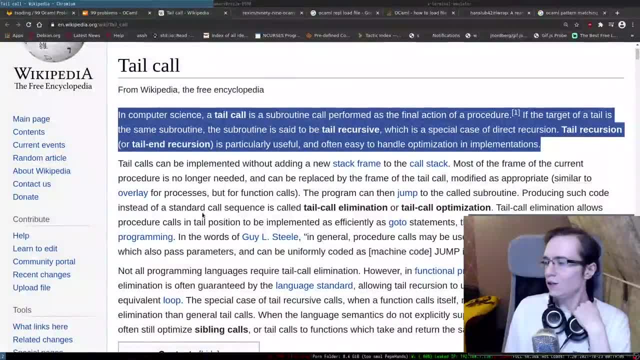 Thank you, Wikipedia. Very cool. This is a very clear description of a tail call, tail recursion, tail end optimization- whatever the fuck you want to call it. It's just the only important rule in here is just to have word tail on it right? So we have to use: 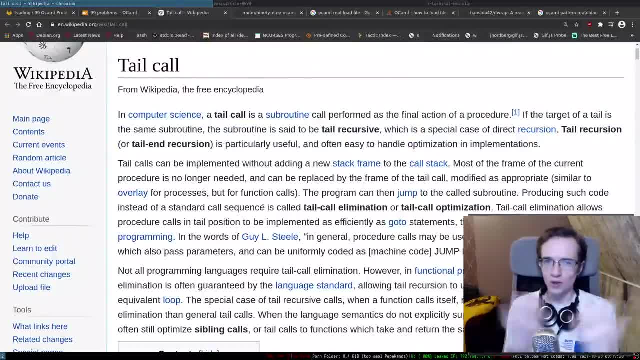 use words tail and call recursion in any order you want, right, And it will mean something. Tail recursion isn't even in fourth. Why would we need to know? That's a good question, We could probably implement. We could probably implement it. Yeah, GPT-3 text or whatever, Yeah. 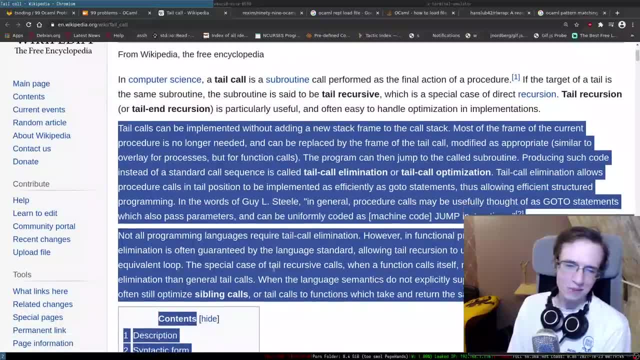 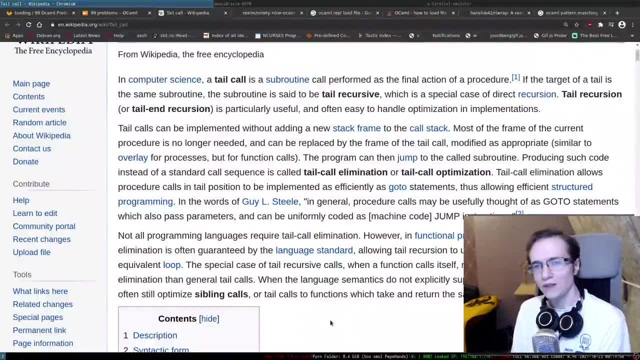 exactly So. it feels like it's generated by GPT. Like what the fuck is the GPT Like? is this shit? So maybe if we read a little bit further, maybe we'll know what the fuck it is. Tail calls can be implemented and implemented without adding a new stack frame to the call stack. 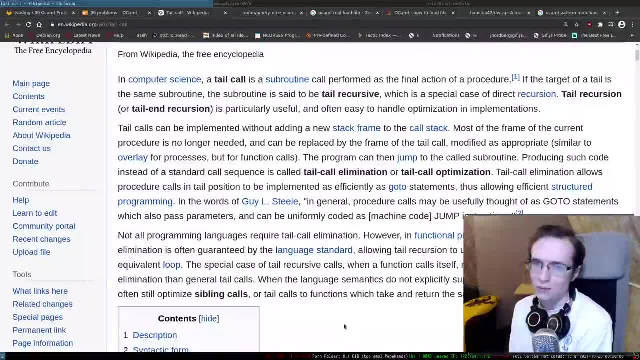 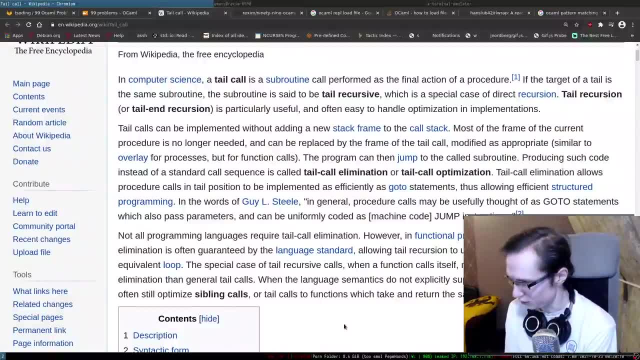 Most of the frame of the current procedure is no longer needed and can be replaced by the frame of the tail call, modified as appropriate. similar to overlay for processes but for function calls. Yeah, this is already a little bit closer to what it is right, Just a little bit closer. 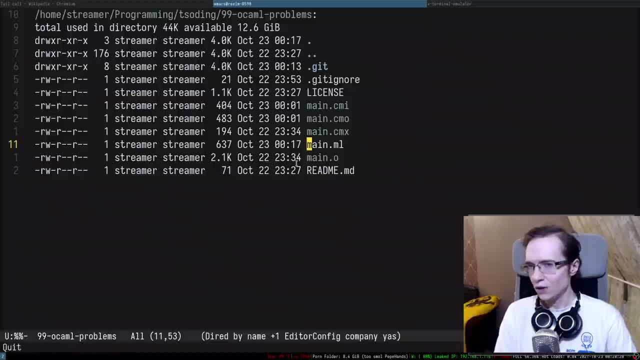 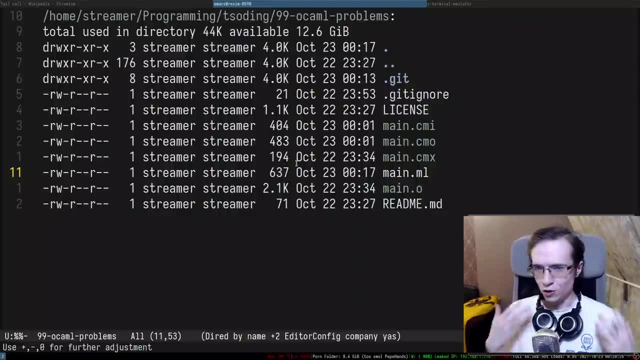 So let's actually maybe take a look at simple example like in C, right? So I would like to use C because it's more of a like a low level language. It's closer to the hardware and it's closer to what actually is happening, you know, on the hardware level. 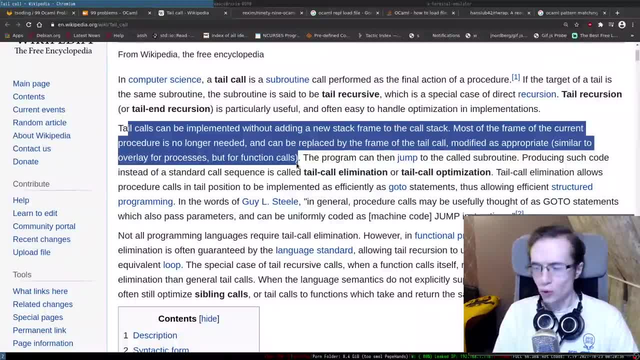 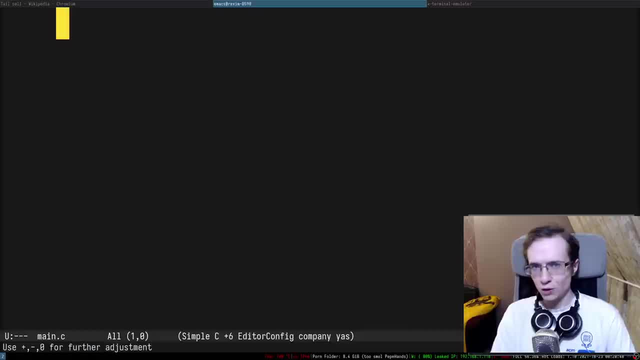 because tail call and tail recursion, it's more about low level thing. right, It's more about low level thing. So we have something like this. I'm going to explain what is a tail recursion and tail call optimization from my point of view. I'm very dumb person. 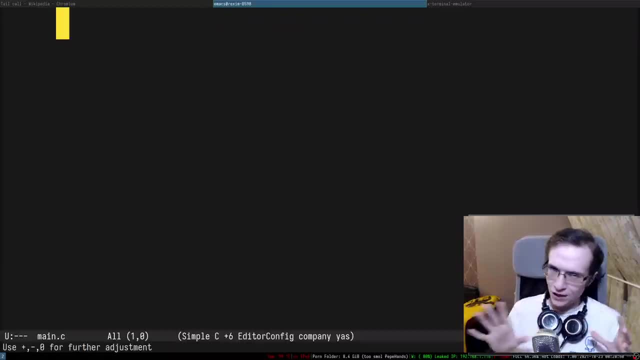 and I'm very uneducated So I may not know some things. I'm sorry. I don't have a PhD in computer science, So I'm going to get some of the academic terms wrong And I'm going to upset a lot of. 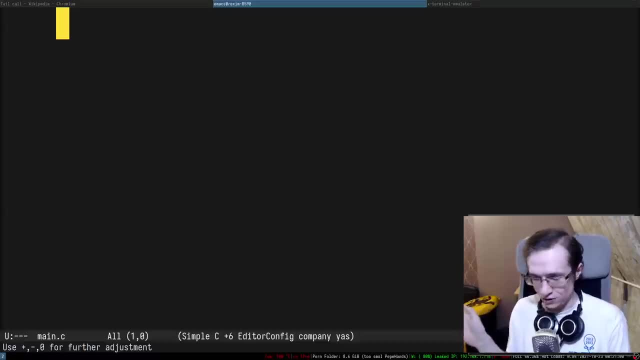 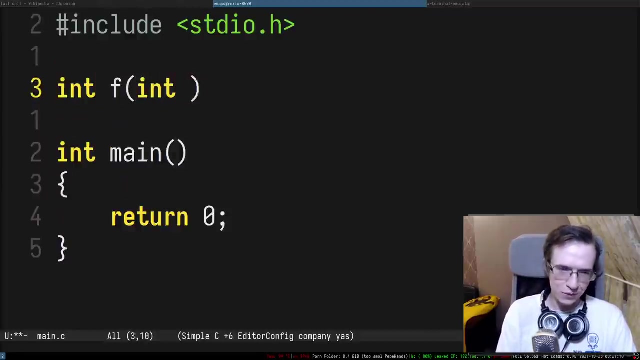 you know, PhD researchers. I'm really sorry about that. I'm going to just say how I understand this kind of shit. Okay, so let me see. So imagine you have a function that looks like this: right? So you accept an integer and you return an integer. right, If x is less or equal than zero, right? 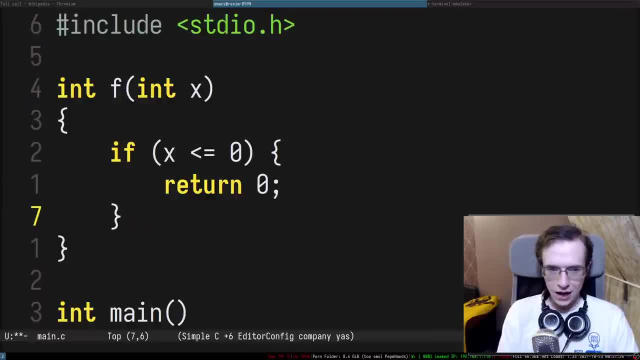 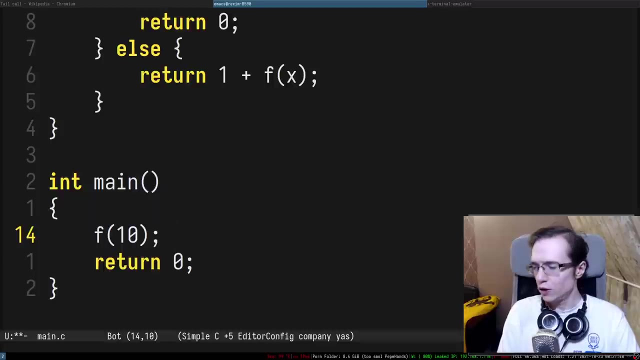 you're going to return zero, Otherwise you're going to return maybe one plus fx. right, One plus fx. So what happens when you call such function, or, in fact, any function? Right On a low level, we have so-called call stack, right. It's a small region of memory. 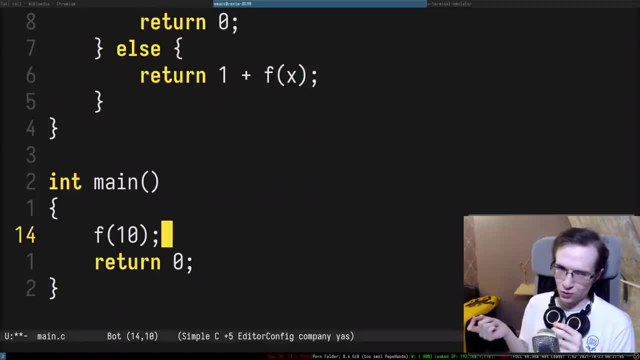 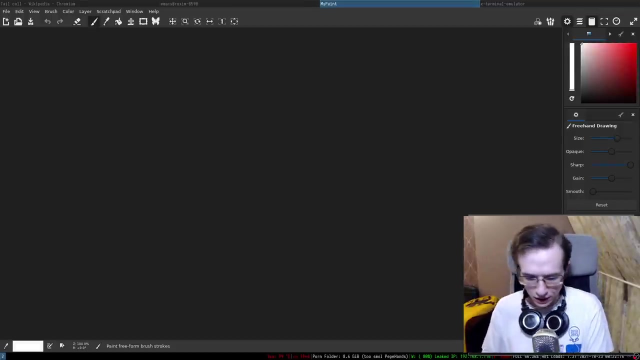 usually on architectures such as x 8664.. It is starting from one place and it grows towards, you know, zero address. maybe we want to actually draw this kind of thing a little bit, So something is wrong in here. Okay, So let's imagine that we have a memory, right? So here is the memory. 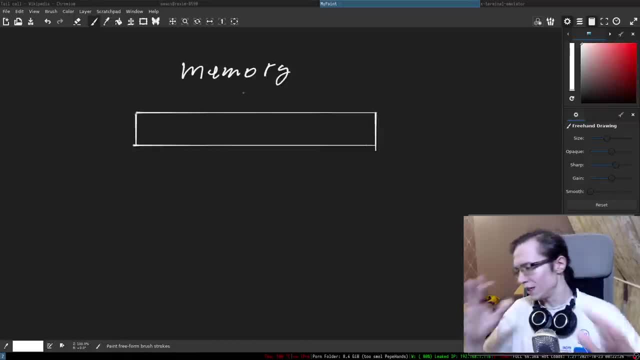 Here's the memory. It's more of like a virtual address space, So you have a stack that starts in the memory somewhere here. So this is a stack. As you push more elements onto the stack, they're pushed to one place, And so you have a stack that starts in the memory somewhere here. 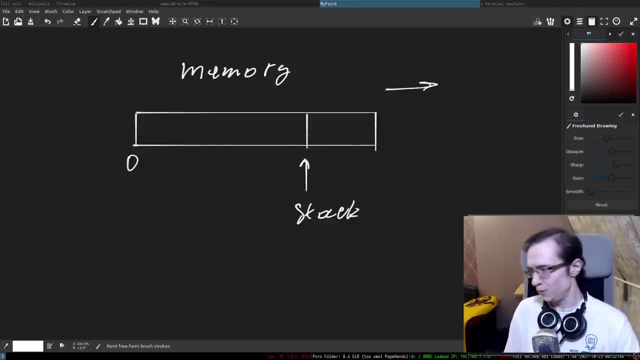 towards zero. So zero is located here and the you know memory addresses grow towards like right side. So a new element will be pushed like this right. And on x86-64 specifically, the end of the stack is kept tracked in the RSP register. So you have RSP register. it points at: 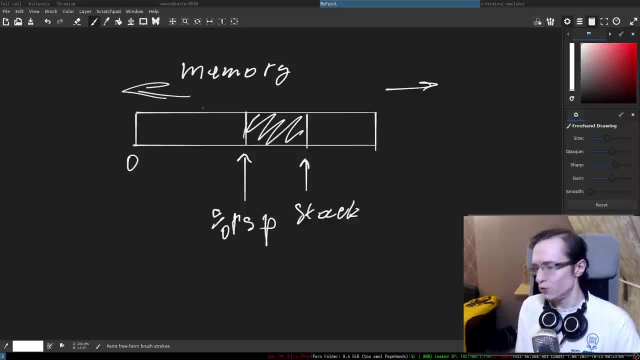 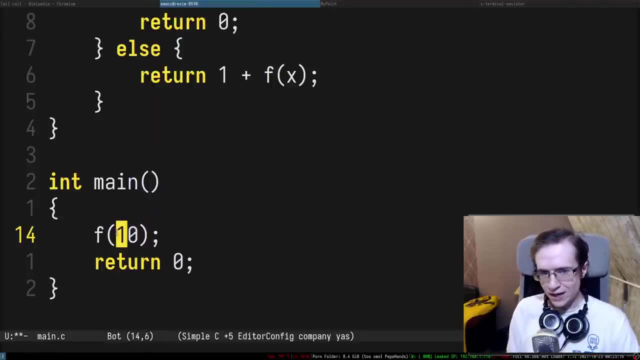 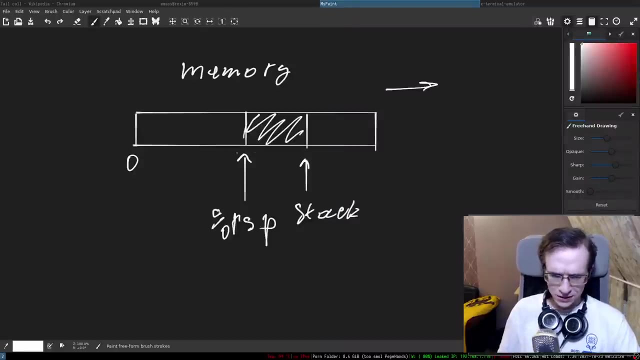 the top of the stack which grows towards zero. for whatever reason, it's x86-64, right. So essentially, when you perform a function, call so how an argument of a function is passed to the body of the function. So I don't remember specific details, But if I remember correctly, 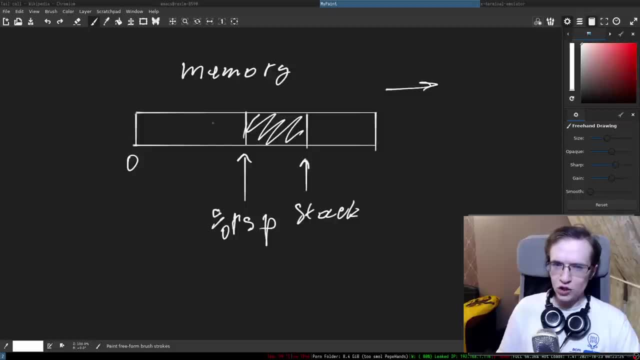 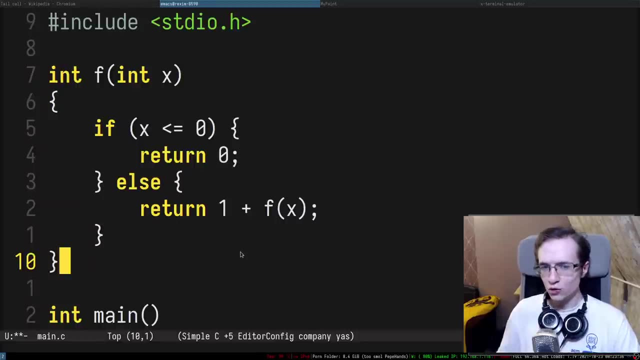 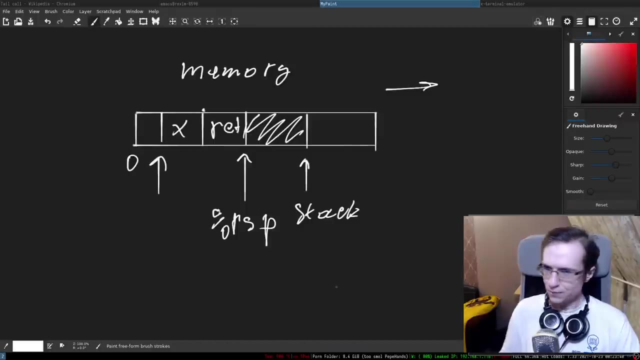 the call instruction will push the return address on this stack right. It will push the return address on the stack So it knows where to return when you do the return right, And it also pushes that x In here. There we go So, and of course that kind of like modifies RSP. There's also RBP. 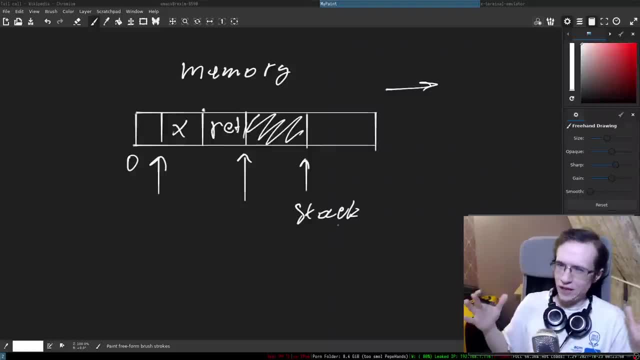 which is, you know, like a base of the frame and stack frames. we're not going to actually go in like that deep into the stack frames. we're going to only talk about RSP and stuff like that, Right, So here are the things, and when you're referring to like x, you're referring to that. 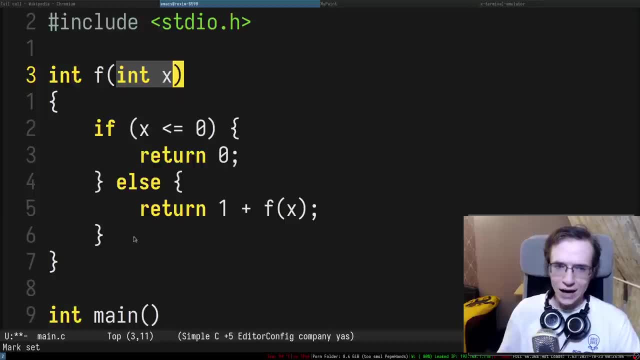 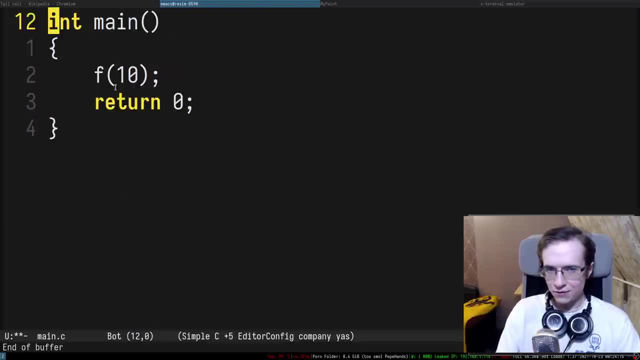 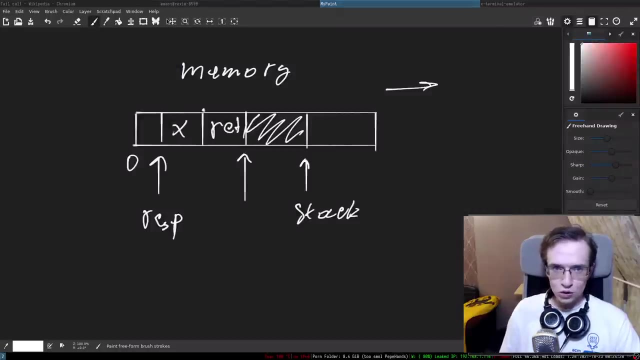 x on the stack. it was passed from y to u via the stack, So, recursively, when you call f yet again, when you call f yet again, you need to push today I forgot to do this thing. I think I forgot to do minus one right. 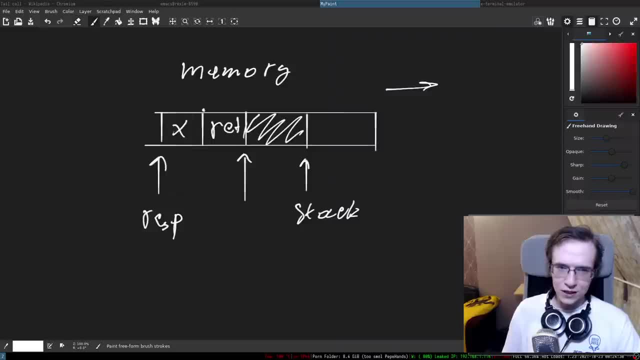 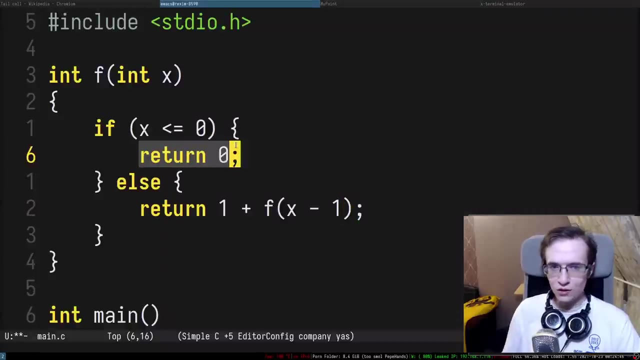 So you need to push another frame. So you call f yet again recursively. right, you call it yet again recursively. So that means it will push its return address yet again on the stack and then x minus one, and it will keep pushing elements until it will reach this situation. 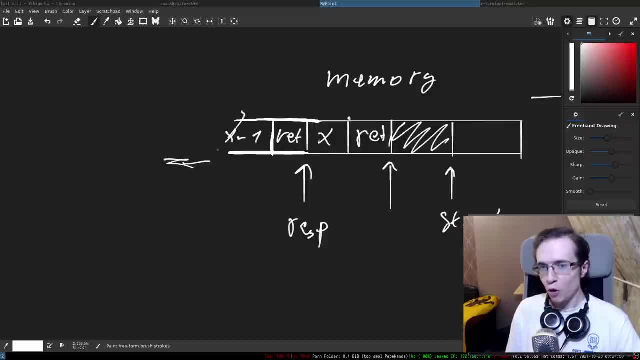 and it will start returning from this recursion by popping all of this element and returning back from the return addresses like: so, basically, as you go deeper and deeper into recursion, it will push more and more things into the stack And then, when it's time to return from the 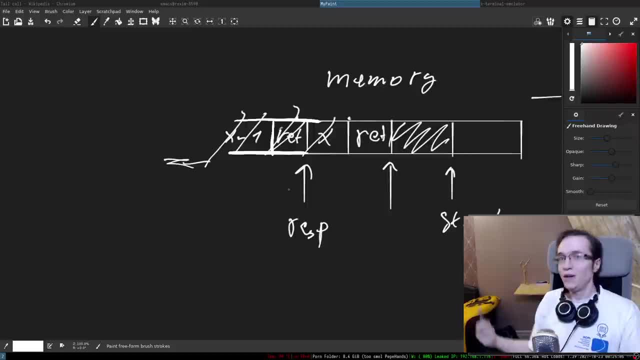 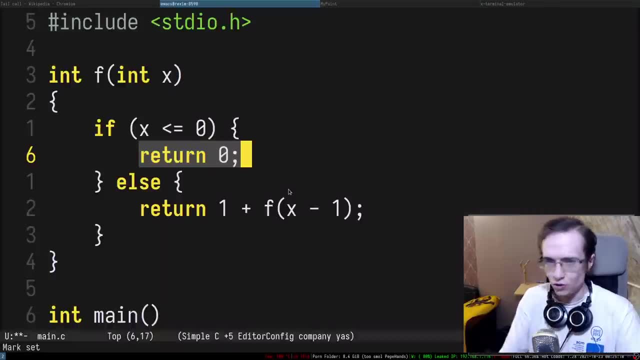 recursion, it will pop everything and return the results. That's basically what happens on the low level, on the machine level, when you program a recursion, and that's why i'm using c to sort of demonstrate. that doesn't make sense, right? so this is usually what we call a call stack, and this is how it's usually used. 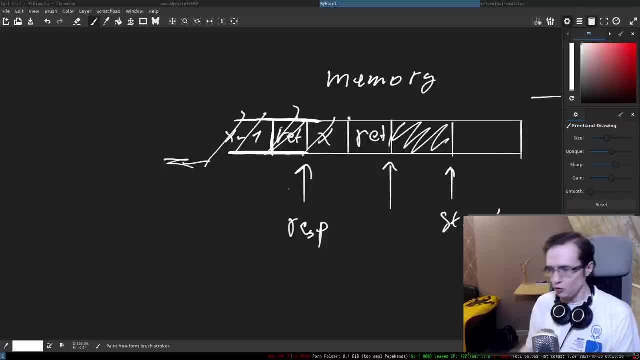 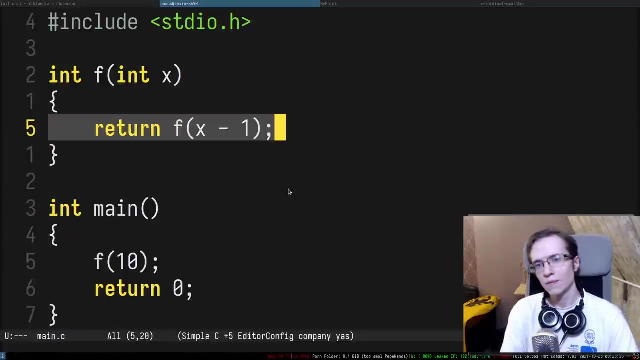 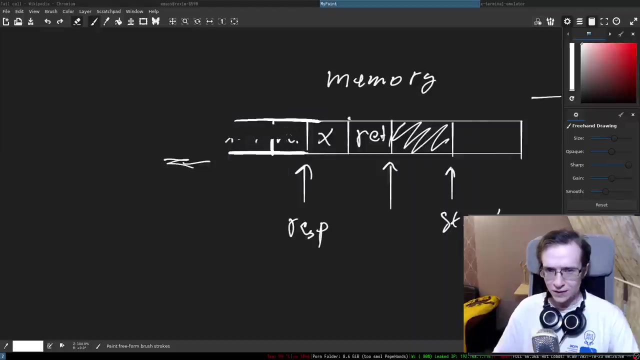 right, with all the call stack, you would be able to, uh, to do like recursive in the classical sense that we do. okay, here is an interesting thing. now let's take a look at the function. that looks uh like this. that looks like this, right, so, uh, essentially, um, we have just x on the stack. 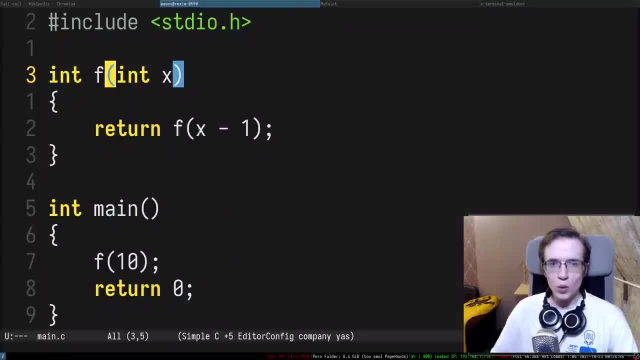 and the return address. and then, uh, we call this function again, but then we don't really need the result of this function up until we completely return from it, right? so in that case, we probably want to maybe assign it to a variable, right? so we keep calling. 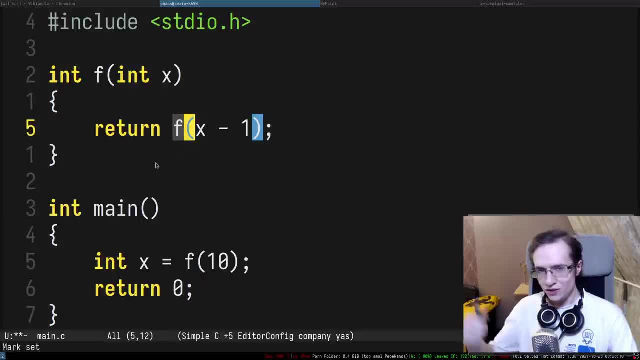 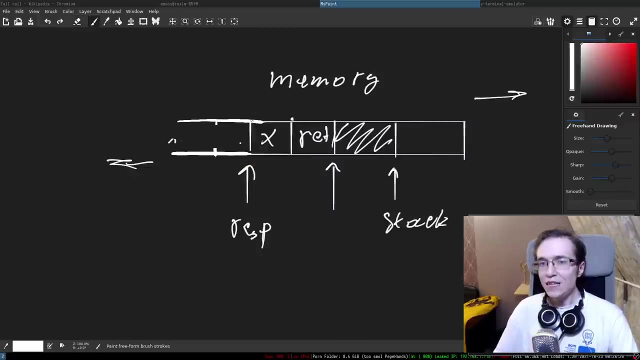 function to itself. uh, but it will only push the same thing over and over on the stack. so in this particular situation, one of the optimizations you can do: you can basically not push this pair of elements over and over again and basically reuse this pair for the next. uh, f call right. 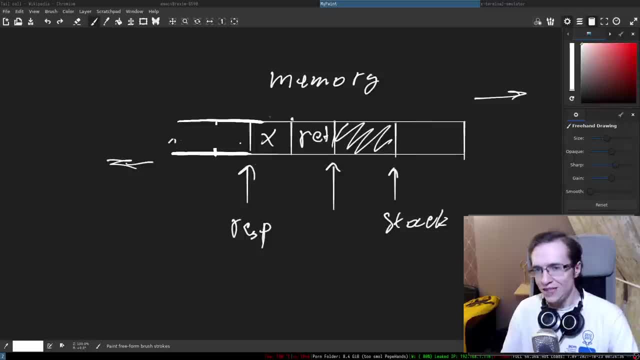 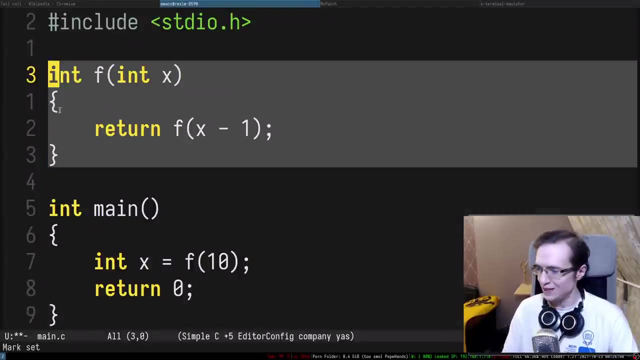 so basically, tail call optimization is basically not pushing yet another pair of this element, this stack frame, but simply reusing it and decrementing x in place on the stack. that way the stack is never going to grow and you can only achieve it when your function looks like this: when the last call, when the call. 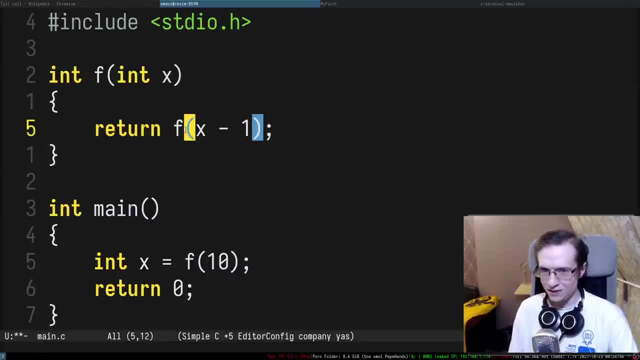 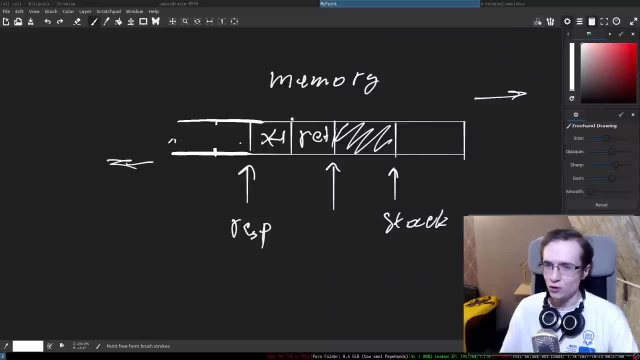 to the function. recursive call to the function is the last one and it's never like the result would never used except like returning. so when you have situation like this, like this, it's quite easy for the compiler to optimize everything and just not push additional frame and just reuse the 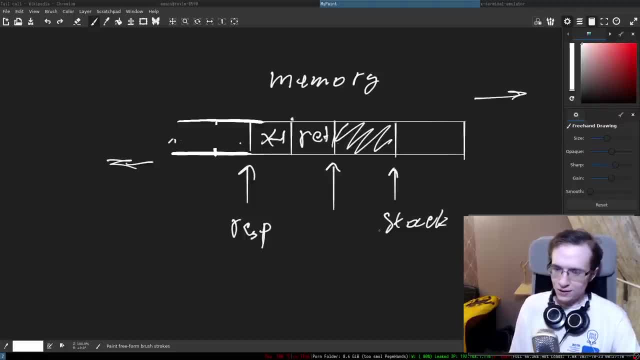 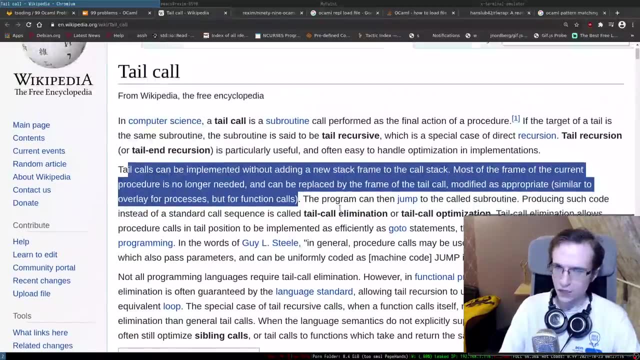 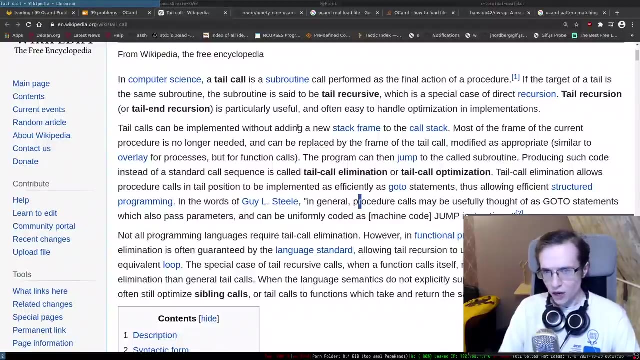 same one over and over again. so this is basically what i understand when i read about tail call optimization and like tail recursion and stuff like that. but i might be wrong. but if you read the description one more time, tail calls can be implemented without adding a new stack frame. 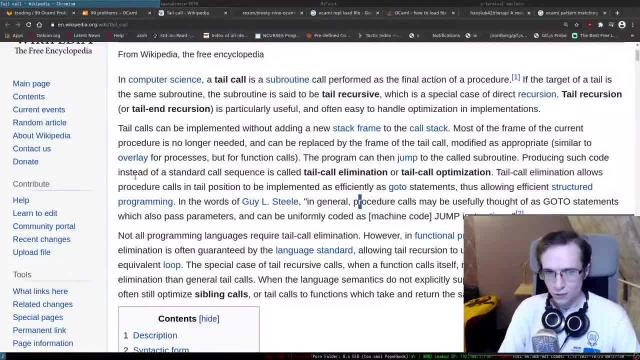 exactly as i said, to the call stack. most of the frame of the current procedure is no longer needed and it's not going to be able to do that anymore, so i'm going to show you how to do that in a little bit. and can be replaced by the frame of the tail call, modified as appropriate, so as you can. 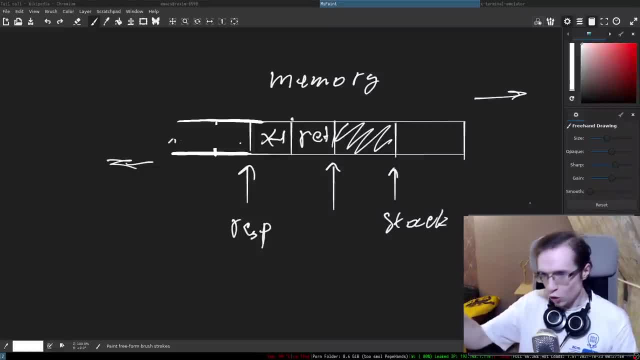 see, as already said, you have a single frame and on each call, instead of pushing a new frame, you just keep modifying the current frame, basically turning recursion into loop. this makes sense. so this is how, at least i understand it, but again, i probably got some terms wrong. i probably get some. 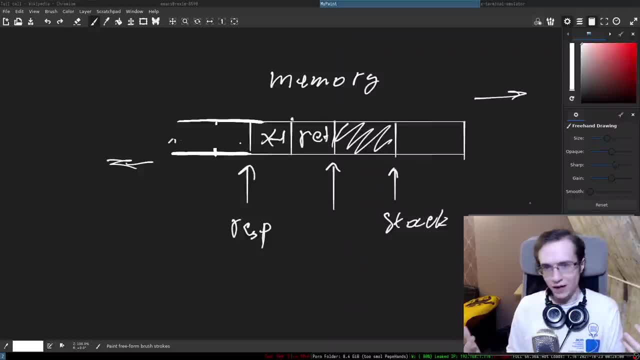 details wrong and that's why i don't have a phd, right. that's why i'm labeled as a dumb, dumb, right? so, um, yeah, so does anyone have a phd in computer science in the chat? please correct me if i'm wrong. so where did i make mistakes in here? 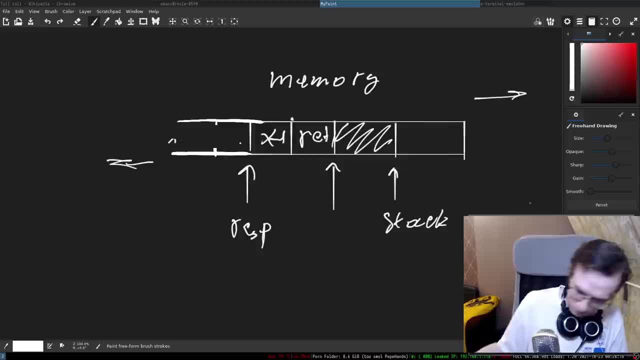 so this is how i understand it and uh so functional programming people um really like tail call optimization because it makes their slow languages look good in some certain uh situations in some certain circumstances. right, because um usually uh functional programming languages on average uh are slow for real world problems and that upsets functional programming. 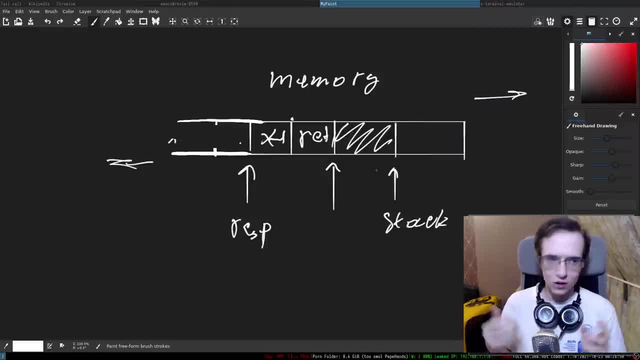 functional programmers because, you know, programmers in 2021 are like um sports fan. they're like, uh, they're rooting for their team and they get very upset when their team is not doing well. and uh, functional programmers basically found a way to make their team look good in some certain circumstances. that's why they like. 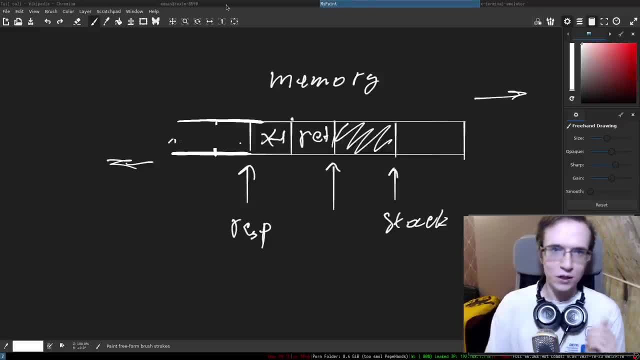 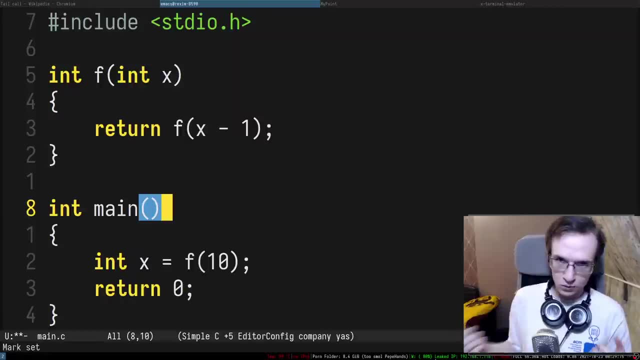 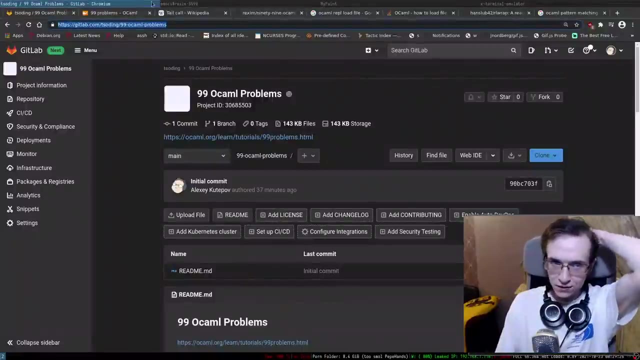 tail call optimization right, so yeah, because it allows them to optimize slow recursion that pushes a lot of stack frames on the stack and turn it into a loop, right, uh so, and they ask us to rewrite, uh, the um, the length function in a tail recursive fashion. so that's basically what they ask us all about. so, at the end of the day, let's talk about um. the second, this is the long function. uh, the long function, uh, that uh is the wrong one. uh, the um. the next mistake that you need to look at is that, uh, you need to modify it like a server. so this is what we're. 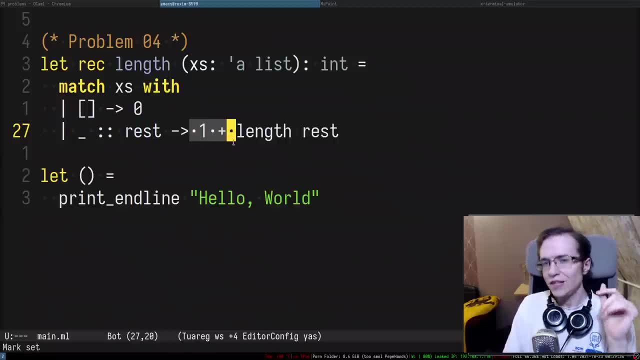 to do Right. So right now, this thing is not tail recursive right, Because calling to length is not the last thing in this entire implementation. So for this function, this function needs to wait until the call is done so it can add one to the result of that call. 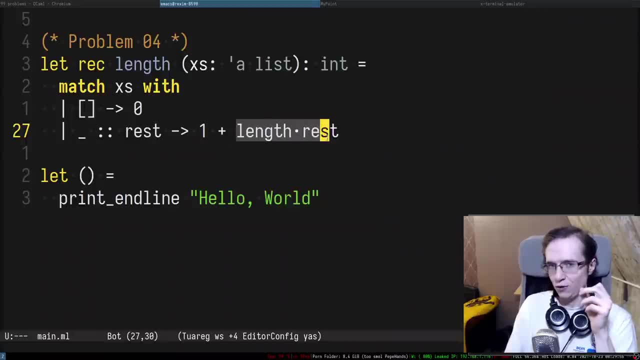 And so, because of the necessity to wait for the results of the lower call, you need to use the stack right. So you need to use the stack in here. So one like to make this entire thing tail recursive. you need to turn this thing into this thing somehow. You need to somehow make this. 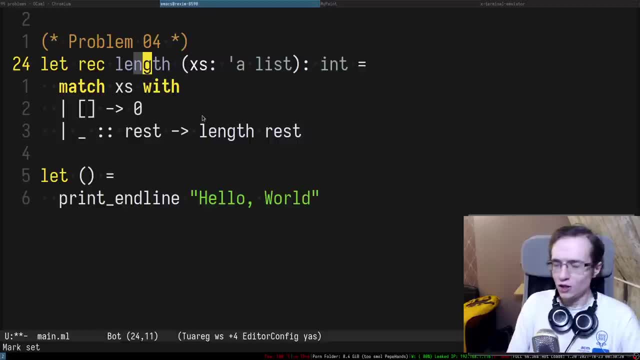 function look like this, but then it needs to compute the size of the list. Well, the usual trick in functional programming of turning a recursive- not tail call- optimized function into tail recursive is to use the stack. So you need to use the stack in here. So one like to make this. 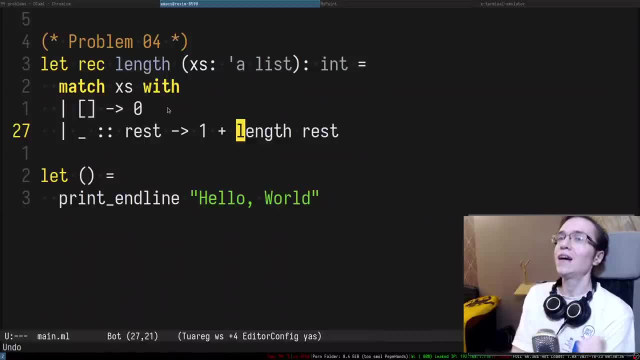 tail call optimized, one is to use so-called accumulator. There is an accumulator trick, accumulator technique, And once you learn that accumulator trick, accumulator technique, you can basically apply it pretty much to any sort of iterative recursive function to turn it into tail call function. So then it can be optimized by the compiler And who like who needs imperative. 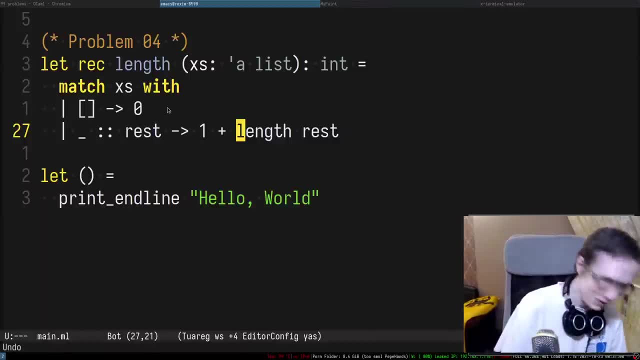 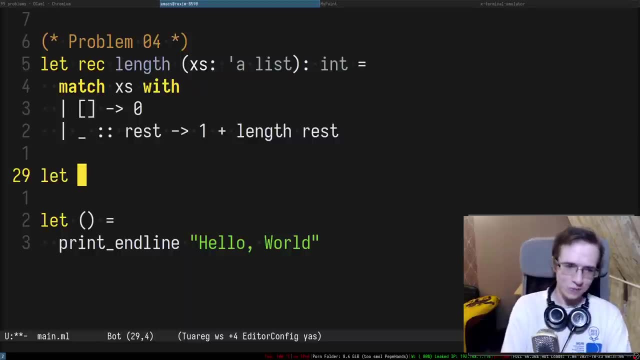 languages after that, right. So who needs imperative languages? am I right? All right, So let's actually go ahead and just implement this entire shit. So usually it is implemented like this: right Length, let's call it like a tail, right? So essentially, you. 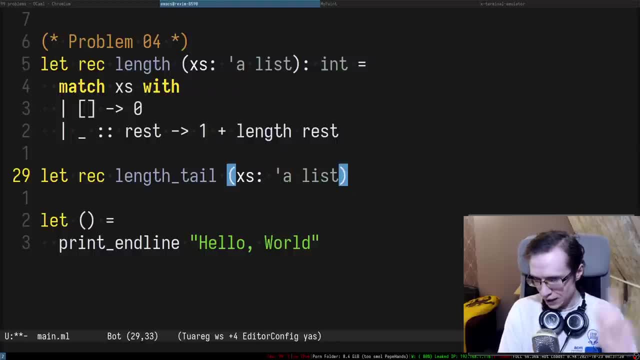 accept the list. the first thing And the second thing you accept is an accumulator. So an accumulator is going to store the final result. So it's basically the result. maybe we're going to even call it the- result. so the result becomes the input parameter for the function. so the result. 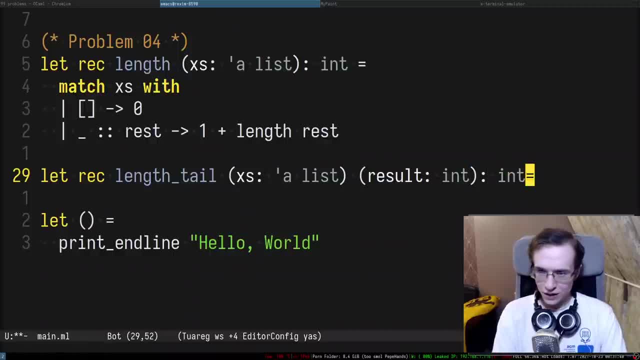 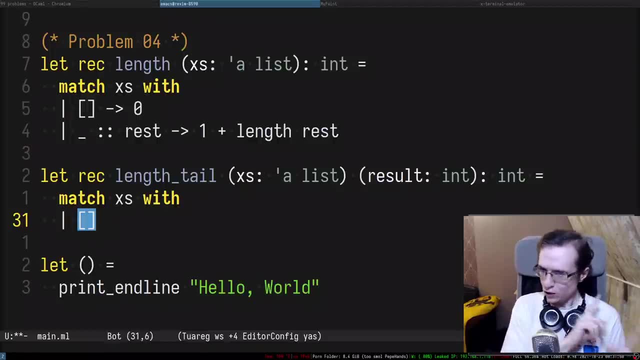 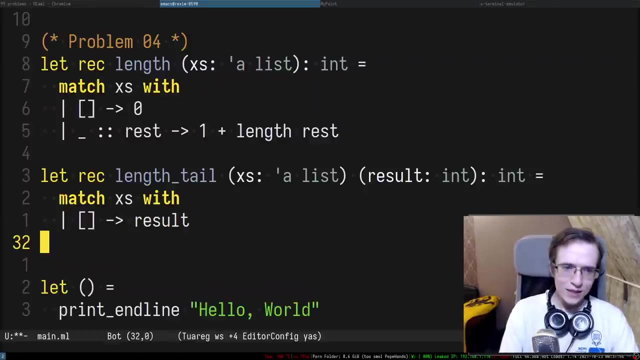 becomes the input parameter for the function. okay, so then we match access. if we encounter an empty list, we don't return zero, we return the results. we return the result. if we encounter the list that is not empty, we call the length tail again, with without the head, but with the results incremented by one. 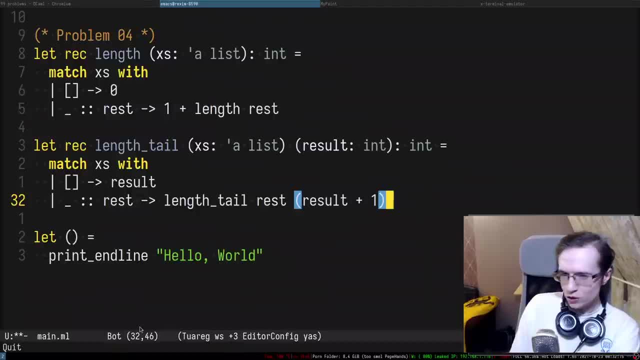 and there we go. we achieved what we wanted to achieve, so now this function is tail called right. so basically, the call, the recursive call to the function, is basically the last thing that you need to do and the result is carried through the arguments of the function right. 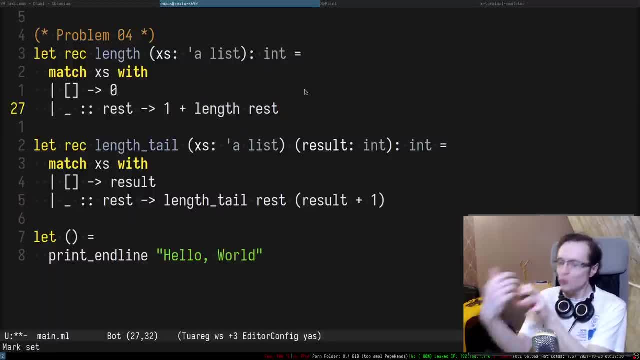 So the result is not returned, but sort of carried through each individual call, And this is something that the compiler can finally optimize and not push stack frames, You see. So that's a tail call, optimized function And the way you call this function right. 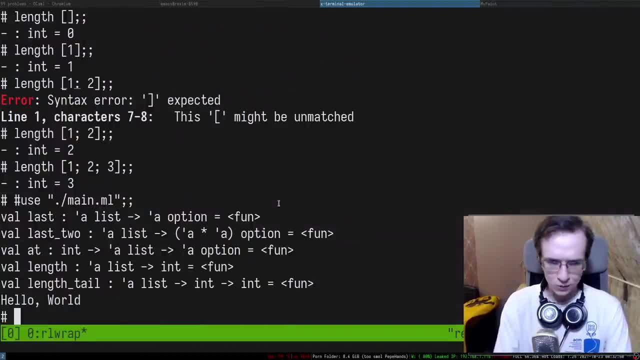 The way you call it. So let's actually use something like use, There we go. So this is going to be length tail. You have to provide one, two, three And you have to provide the initial value for the result, right? 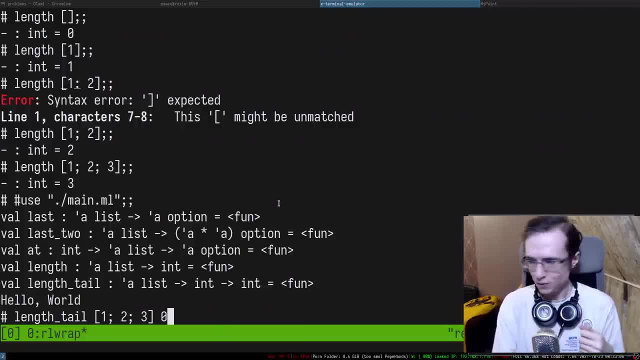 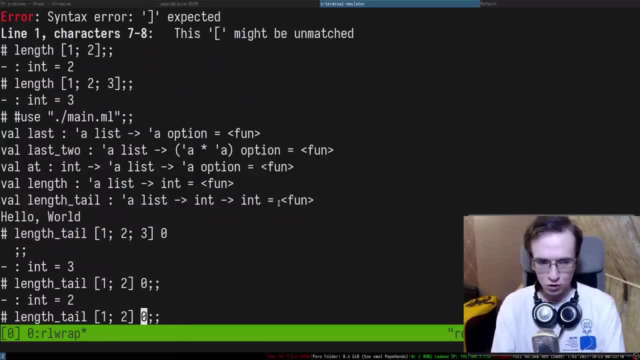 So in case of empty list it has to be zero. So that means the initial value for the result has to be zero. And there we go. As you can see, we have three elements in here. So if you have two elements, it's going to be two. 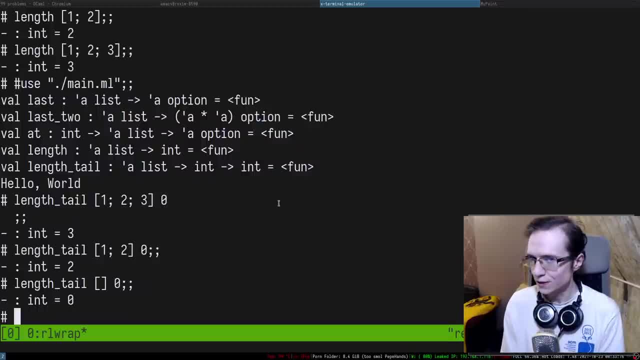 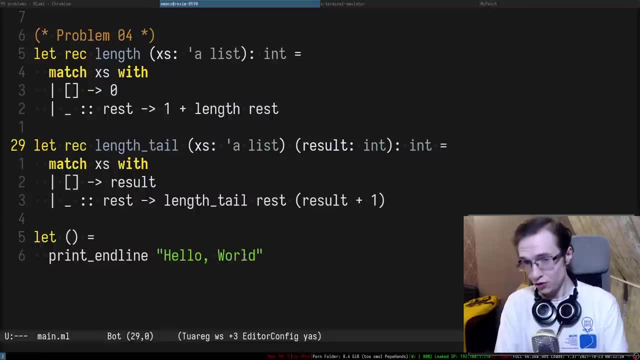 If the list is empty, it's going to be zero, right So. but it's not really convenient to have this extra element. So what usually function programmers do? they sort of like talk The um, this function under another function, that basically. 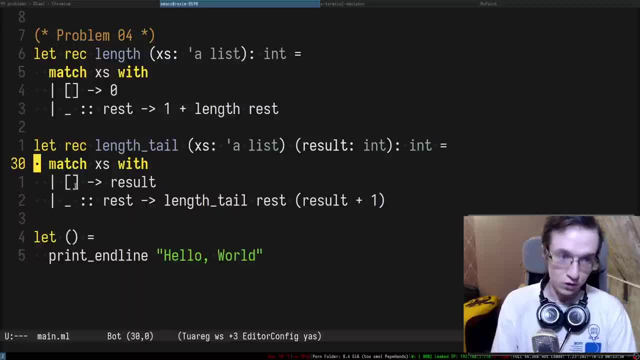 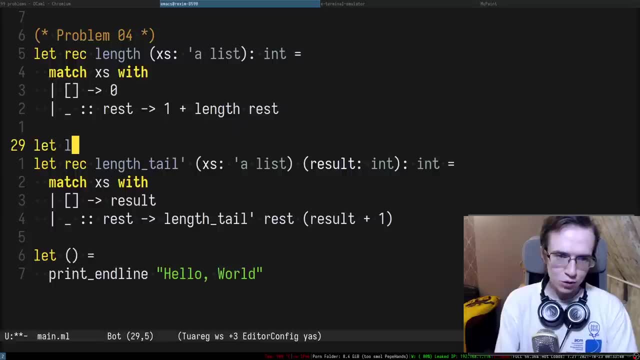 provides that, uh, that default element for the, for the results. So let's actually call this thing uh length tail, uh prime, and let's wrap it into length tail, which accepts only the list. right, It accepts only the list. 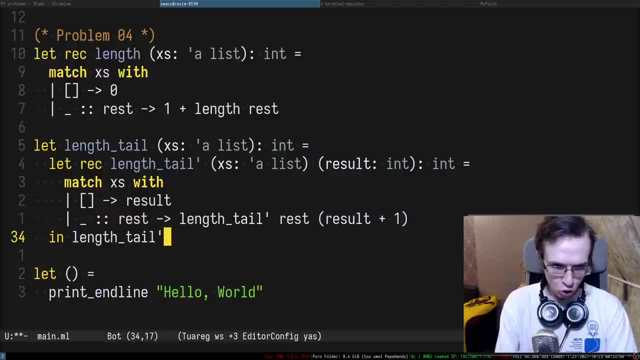 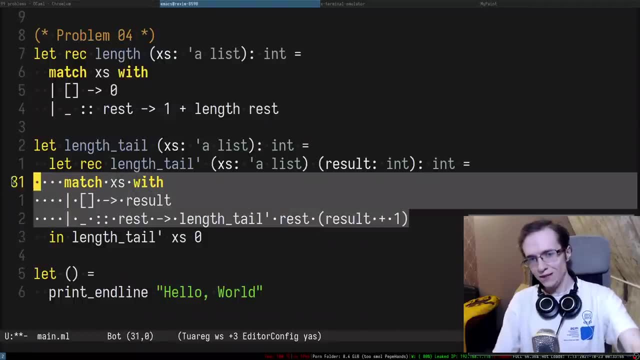 Uh, and this one becomes the inner function that we just call um, with the default parameter zero. So you see, in the camel you can actually quite easily define nested function, And this function is not going to be visible like outside of this one right. 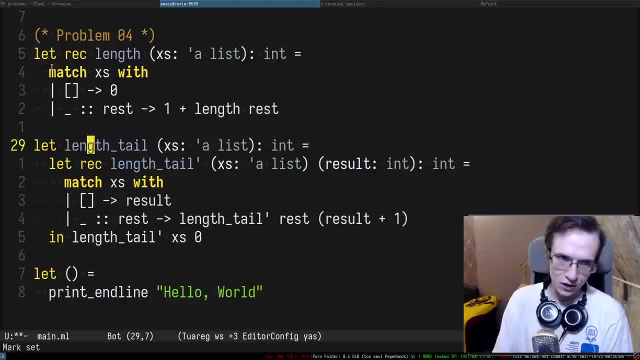 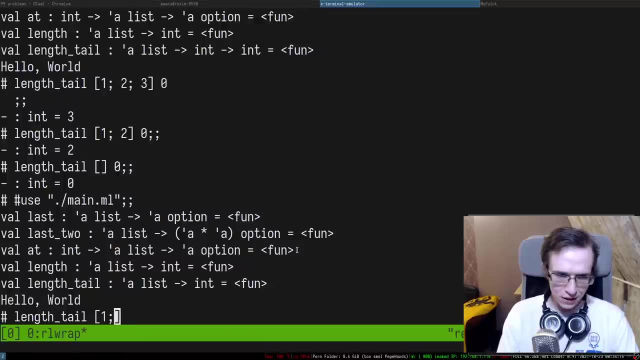 So the syntax of a camel is quite ergonomic in that case, because the inner function syntactic is not that different from the outer function and it just can quite easily wrap everything right. So, uh, let's do use- And, as you can see, everything works, and I can do now- the length tail, uh, two. 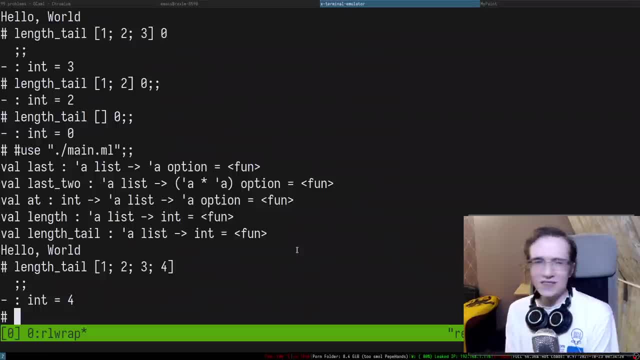 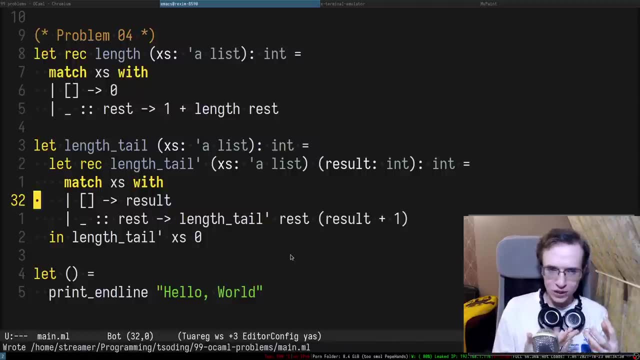 three, four and uh, there we go. So it works, but like this There's no difference between like. it's kind of difficult to observe the actual difference between like tail recursive function and not tail recursive function, because they behave the same right. 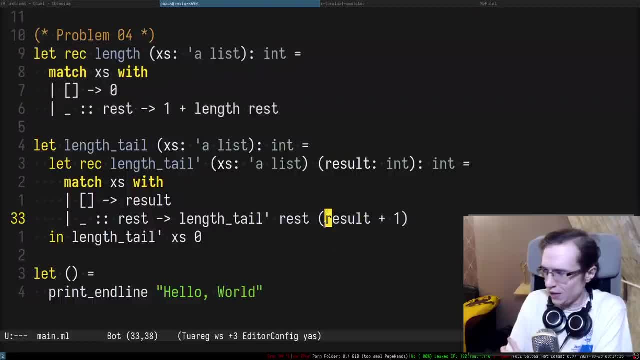 So the implementations are slightly different, but they behave the same. And do we really improved anything? Did we really improve anything, Did we? I don't know, We can try to check that. uh, let's actually write a useless recursive function like a useless iterative function. 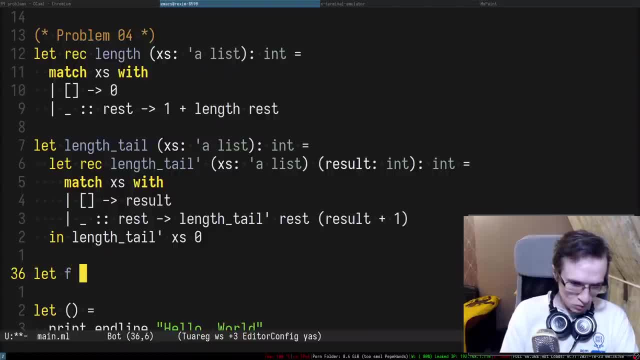 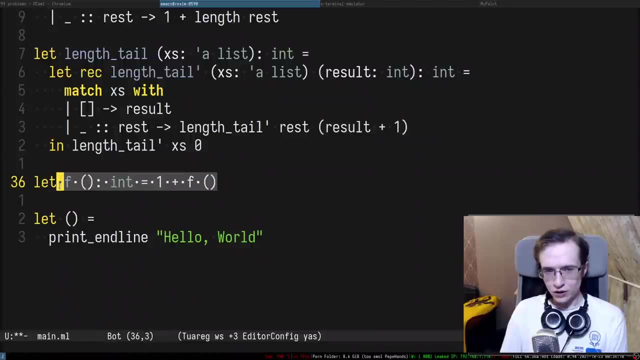 Uh, something like um, F, right, Uh, which essentially returns an integer, and uh what it does? it basically calls to itself uh, but it increments its results over and over again. So, essentially, uh, for this function to work, it needs to push things on the. 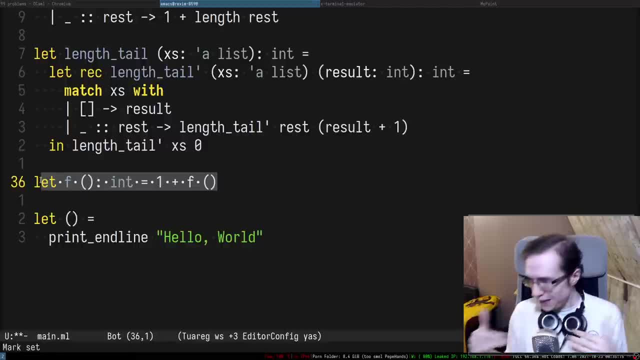 stack and since it doesn't have the um, the base, it's going to go into recursion indefinitely. and, uh, since it's not a recursive optimized, it will um stack overflow, right? Not everybody knows, in 2021, but stack overflow is not a website. 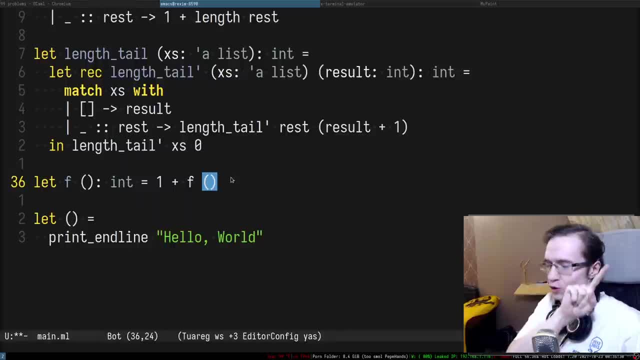 It's not only a website, but it's also an error that you can encounter if you're not careful with the recursion right? So Sorry, Uh, so, uh, yeah, let's actually try to see what's going to happen. 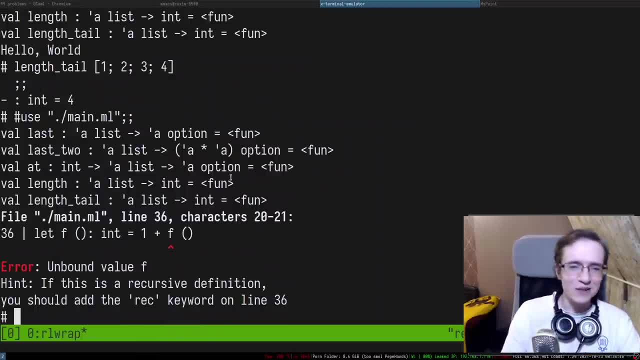 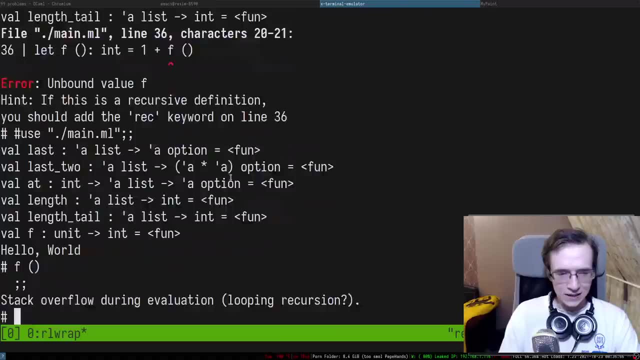 If we call this function, it doesn't even compile. Okay, So, because I forgot to mark it as a recursive one, So, uh, all right. So if I call this function, Uh, and a boom stack overflow during evaluation looping recursion, I really 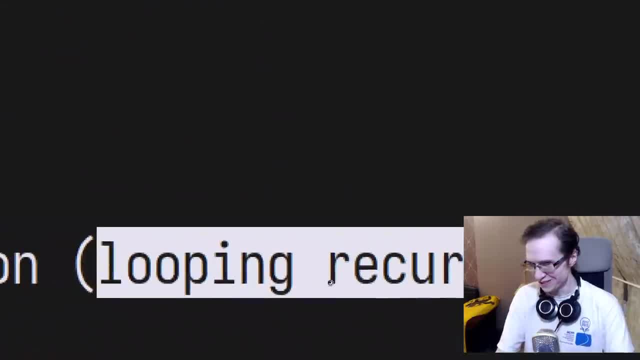 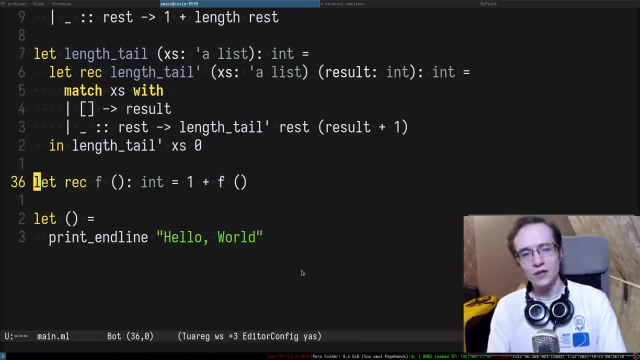 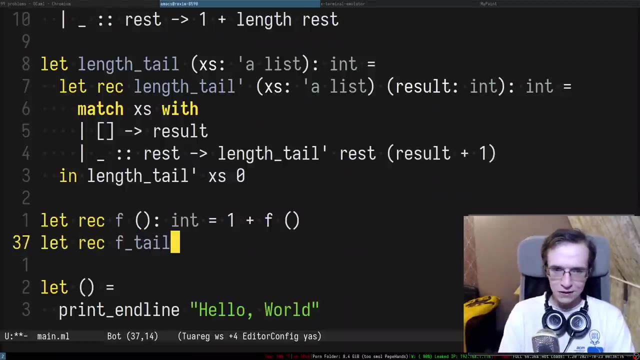 like how it asks the question: looping recursion. oh, oh, I see what you did there, buddy. Oh, looping recursion, Okay, So, uh, how can we make it? um, you know, tell recursive, right, So this is going to be, uh, F tail. 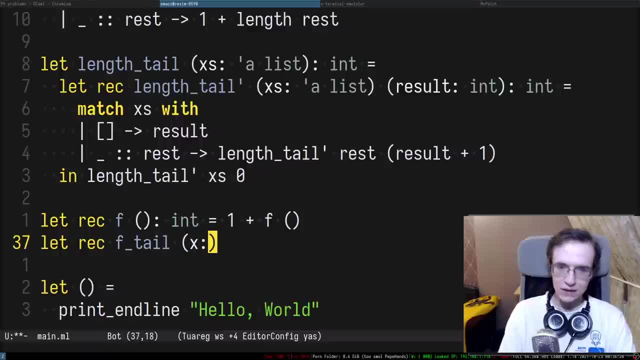 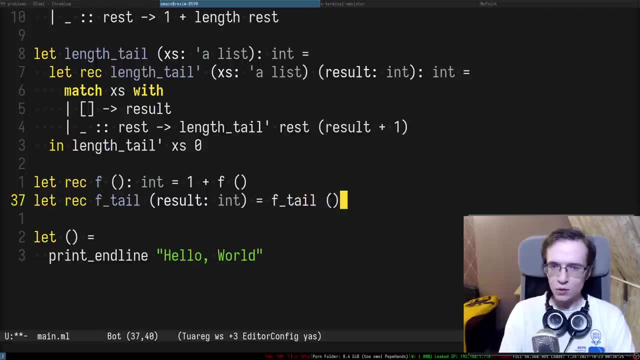 Um, and this thing is going to accept, uh, an integer instead like result. Uh, right, And what it's going to do? it's going to just call itself, but with the result incremented by one. as you can see, here we carry the result. why the return? but 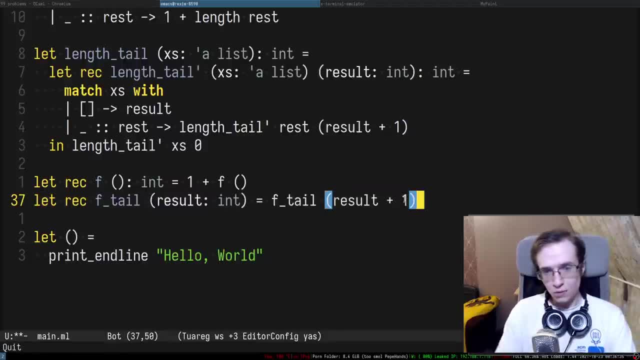 here we carry the result. why the arguments right? So, but since this thing is the last thing that we call, uh, it will be optimized and won't push any stack frames, And since it won't push any step frames, it's basically in the loop forever. and 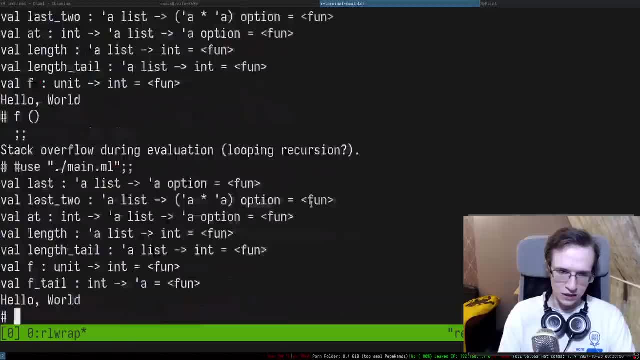 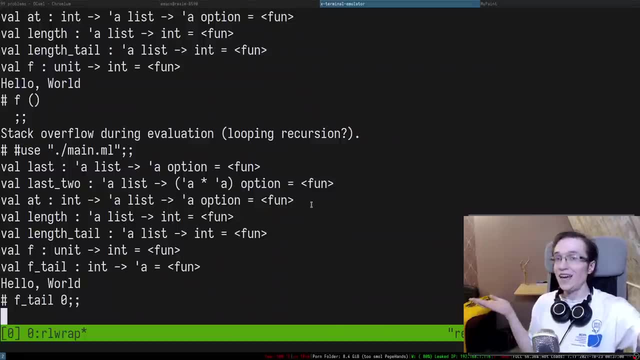 never going to stack overflow, Right? So let's actually do something like: uh, you And I'm going to do F tail zero and it's just hanging, is just looping. It's a recursive function that keeps looping and looping and doesn't stack overflow. 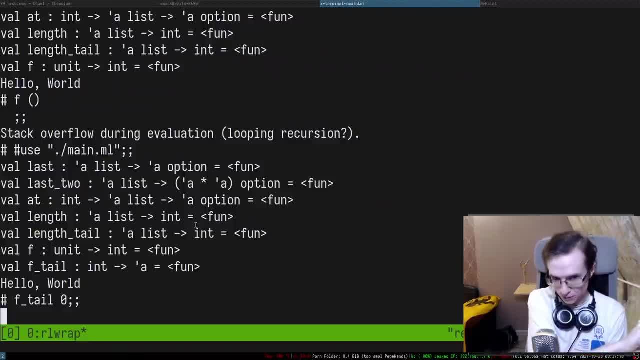 So we can clearly observe that one function pushes the frame on the stack- And that's why it's stack overflows- And another one doesn't push. So this is how you can demonstrate the difference between these functions. Mm-hmm, Uh, hash trace allows you to see the behavior of the function. 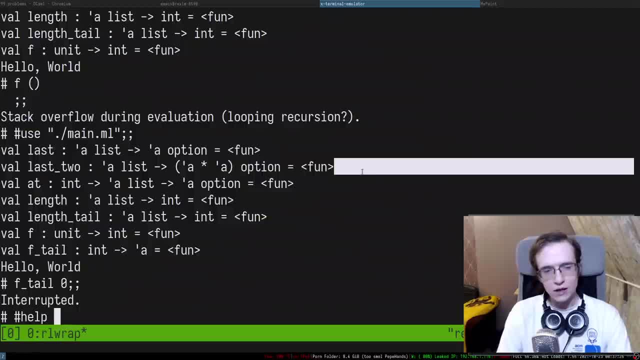 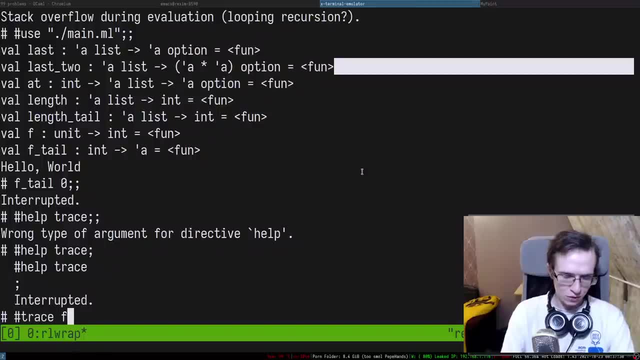 I didn't know that. Let's actually take a look at that. So can I do something like help trace uh, or whatever the fuck it is? Uh, I don't know. Okay, So trace full. uh, I don't know how to use this function. 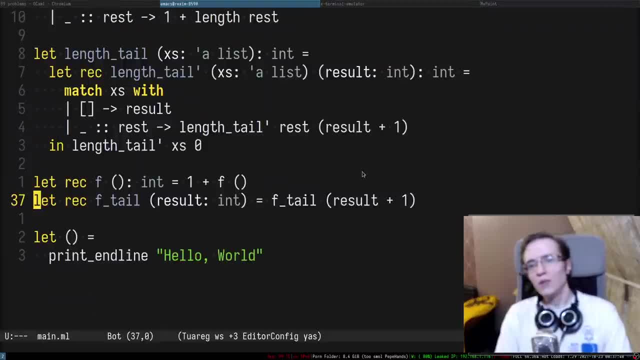 I'm sorry, but I'm going to read how to use it a little bit later, But anyway, we can actually observe the difference between the, uh the behavior, just like that, right? So one function um overflows the stack and another one doesn't overflow the stack. 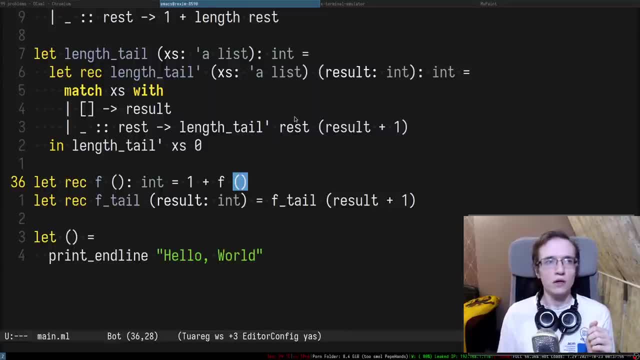 And this is something that you can use even in not, uh, functional languages. As far as I know, uh, some of the C compilers, some of the C compilers also, can perform tail call optimization. Uh, so, let's actually see, let's actually try to apply the same trick in here. 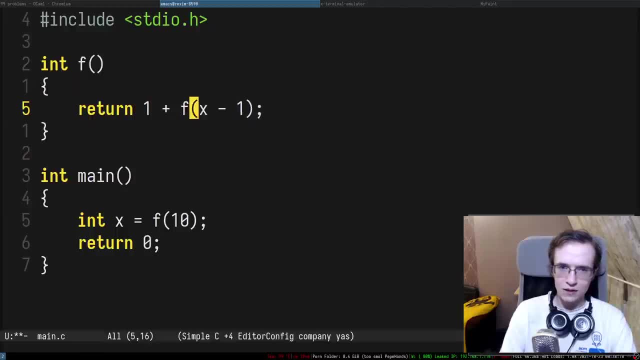 Uh, right, So if we have something like this: uh, one plus F, this entire thing is definitely going to stack overflow, right? So it's a hundred percent is going to stack overflow If I do GCC, uh, um, you know, main dot C, and then I'm going to just run this entire stuff. 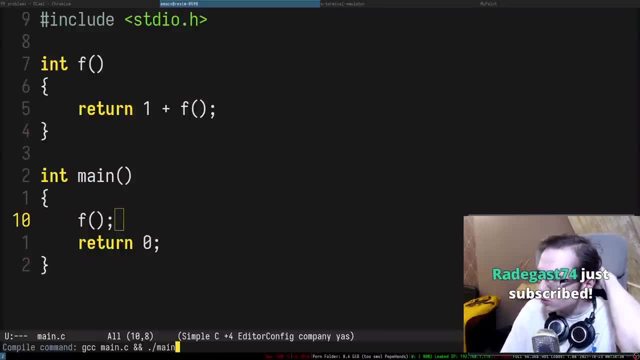 Uh, so we've got a bunch of gifted sub from the the bone Hunter. Uh, thank you so much, The bone Hunter, for five uh tier one subs and everyone who got the subs. Welcome to epic tail recursive club. Hello Ben. 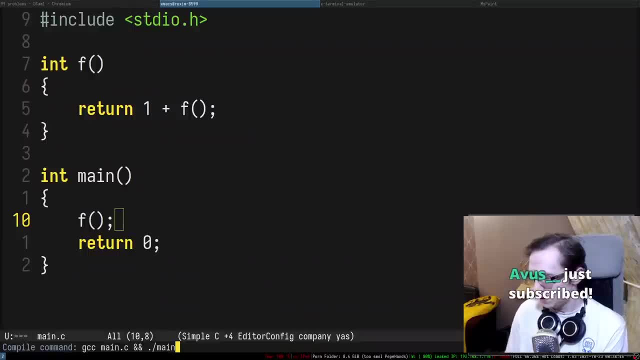 I know what the fuck is going on with me. I think I've drunk too much too, Uh. so how are you guys doing? I was going to do You're welcome, Thank you. Thank you so much, Really appreciate it. 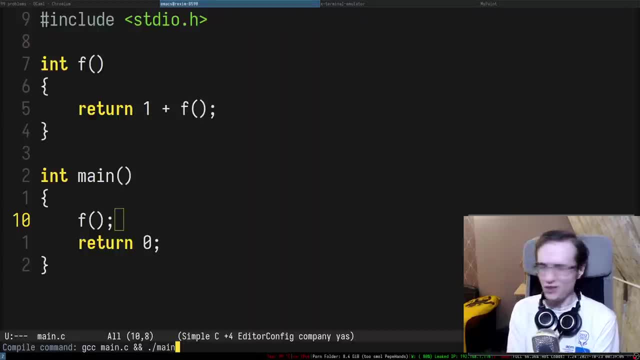 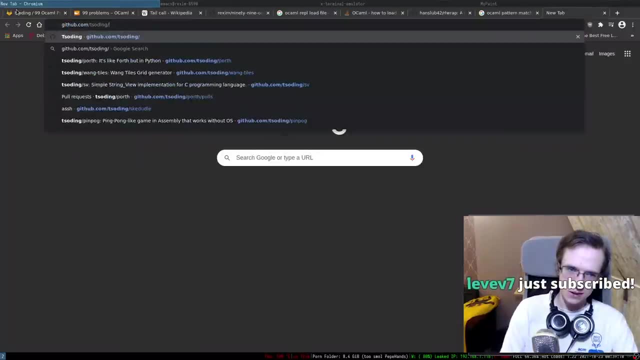 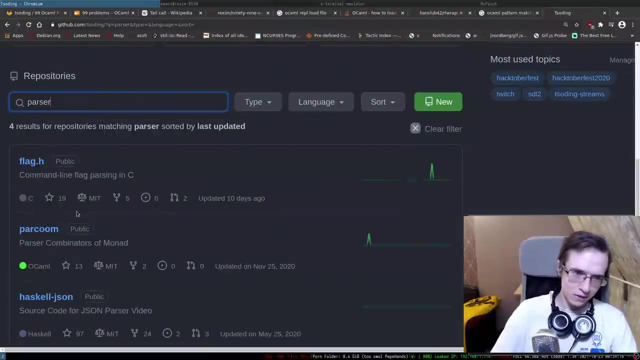 Just want you to say that your pasta committed in the camel is pretty fun to use. Somebody using it? You're actually using it. Yeah, Some time ago, uh, I implemented the pasta combinator in in a camel- Um, I don't remember. uh, pasta, uh, parkour. 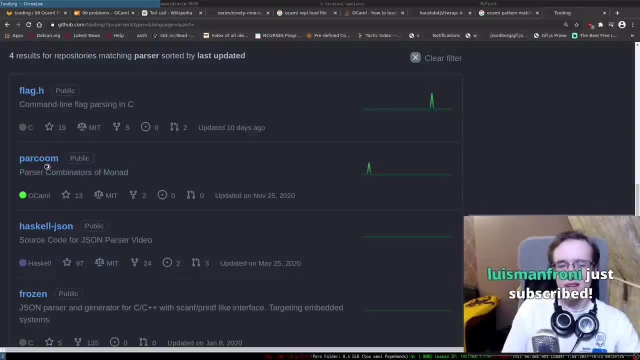 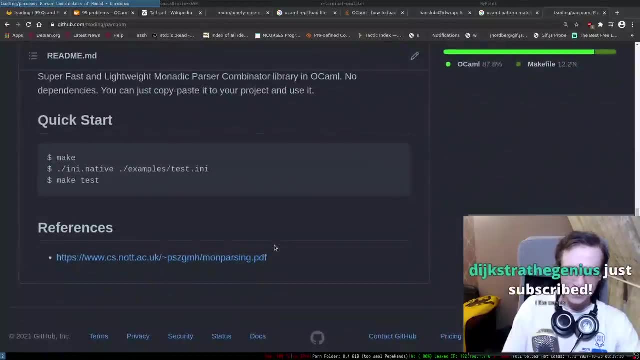 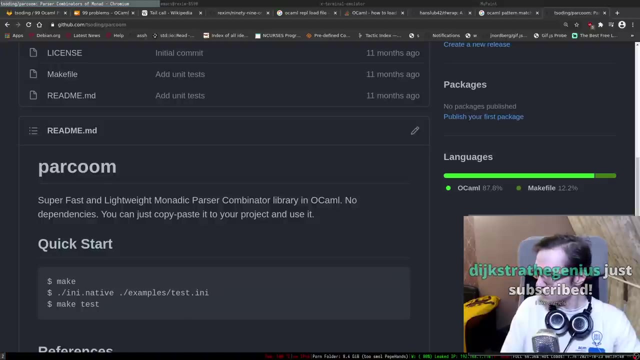 I forgot how to call it like that. It's like party combinator of mallets and park. So, uh, okay, So my, my sense of humor didn't change apparently, um, over The years. Uh, thank you. 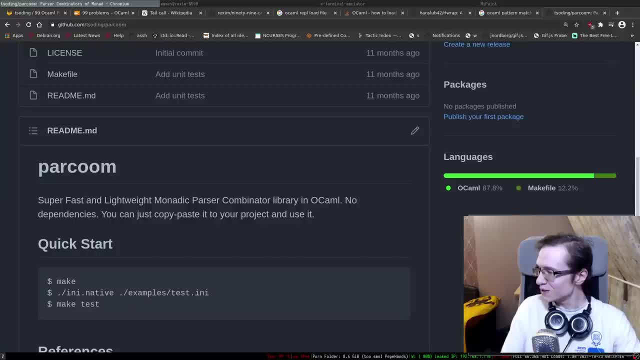 Is that a donation? Just a second. I didn't expect. uh, Dexter genius um subscribed with Twitch prime saying: I like camels, camels, I also like camels. They're pretty cool. That's why I program in Perl, You can. 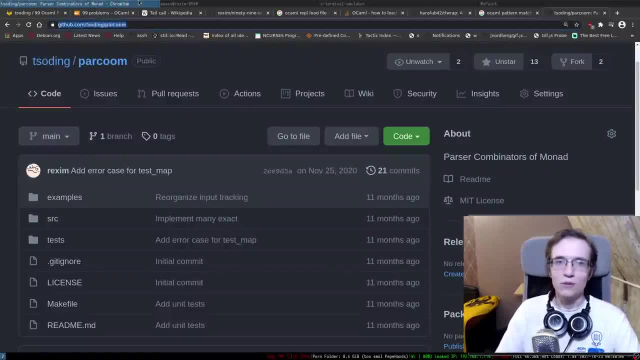 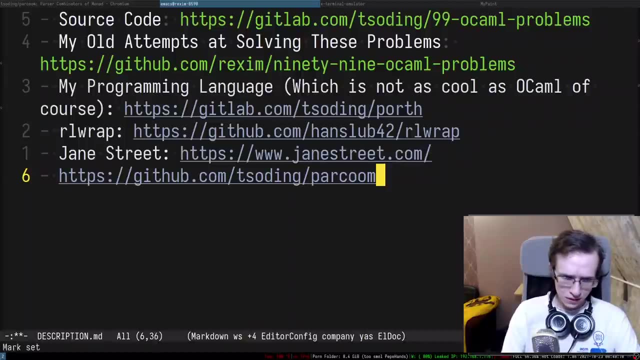 find this thing in here if you're interested, and I'm also going to put it in the description. I think I also did it on the stream some time ago. So parse the combinators of monad in OCaml. So it's actually a very simple one. It's not as generic as a lot of parser combinators. 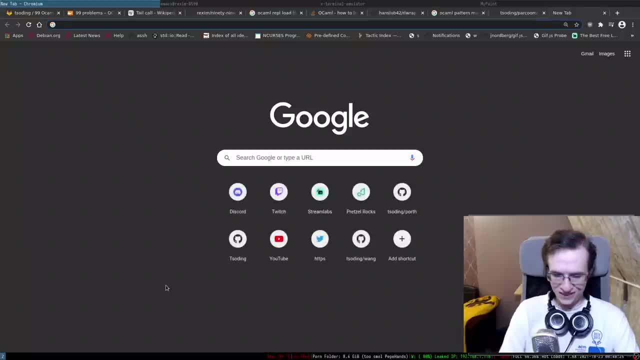 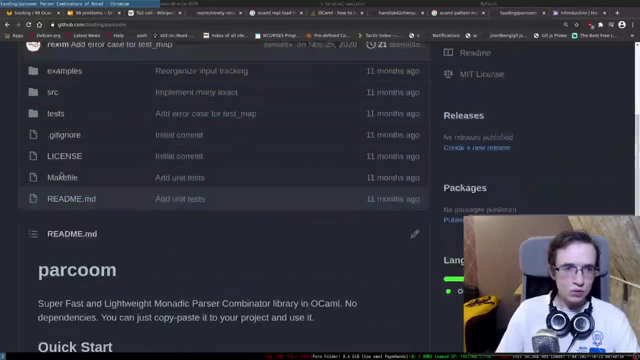 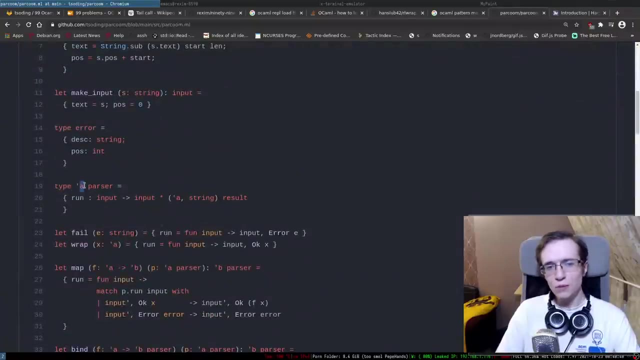 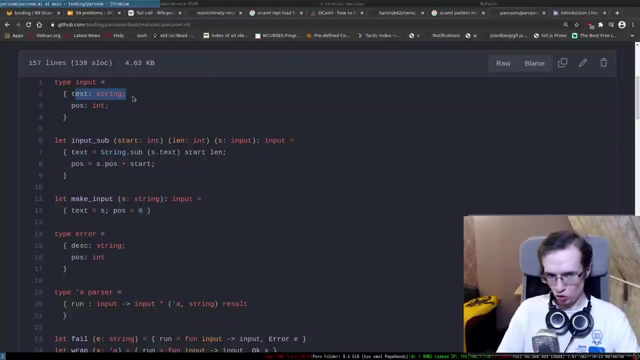 in Haskell, because if you take something like parsec, if I remember correctly, so where's the hackage? Where is my hackage, Parcumml? So this parser combinator, you can only parameterize the result, right, The input is always the string with position and the output is always the result and the. 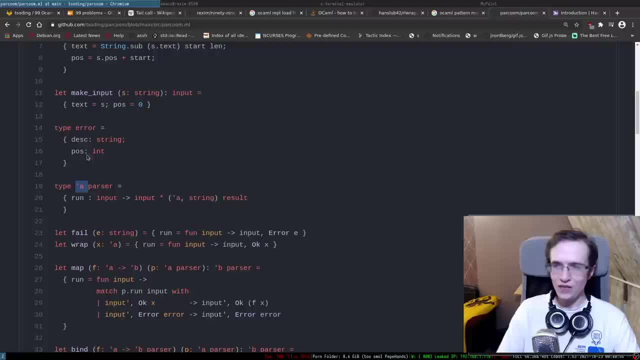 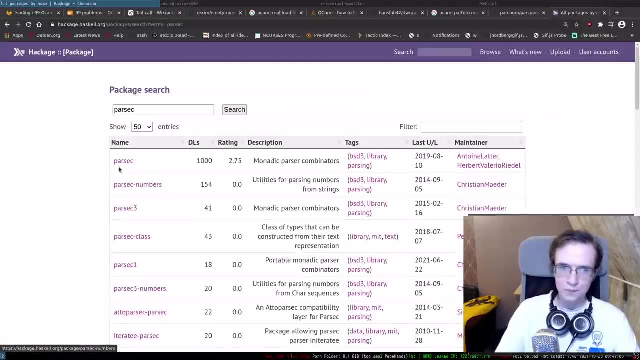 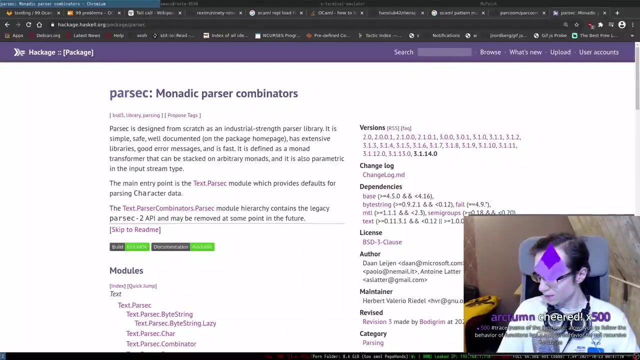 rest of the string, and so on and so forth. So the only thing you can customize in here is the result, Right, but if you take a look at something like parsec, parsec ArcToon name of the function allows you to follow the behavior of functions. 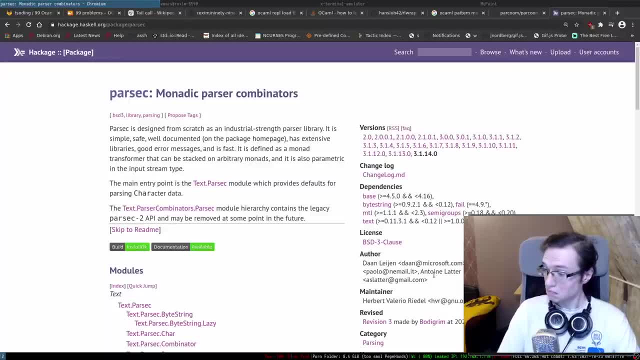 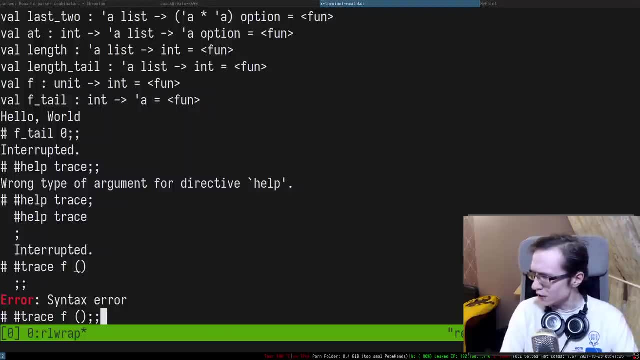 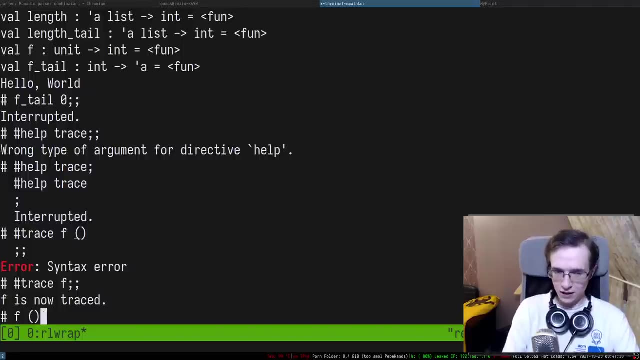 has been selected. okay, thank you so much for 500 bits. uh, let's give it a try. um, so, so i just have to do it like that name, the name of the function, okay, it's just the name of the function. is now, oh, is now traced, and then i just call this fun, okay, okay, and it's just like: keep, keep, keep. 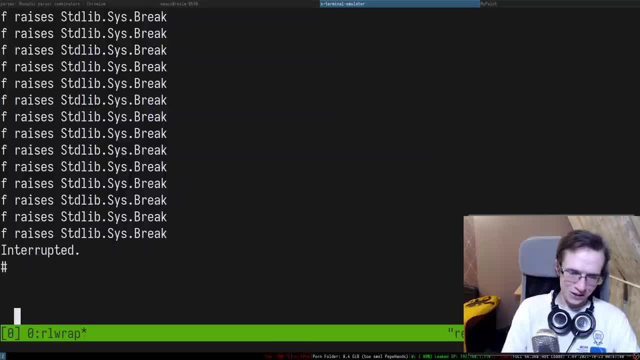 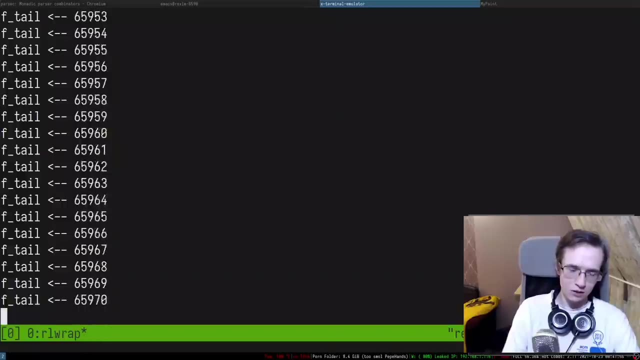 slooping and i can't, i can't stop it. ah, okay, it's stopped. uh, well, it's not tail recursive, okay, so if we trace tail recursive one, right, and it's going to be tail, uh, zero, uh, and it even shows the uh arguments. okay, that's actually pretty cool, okay, oh, oh, i know why it takes so much time. 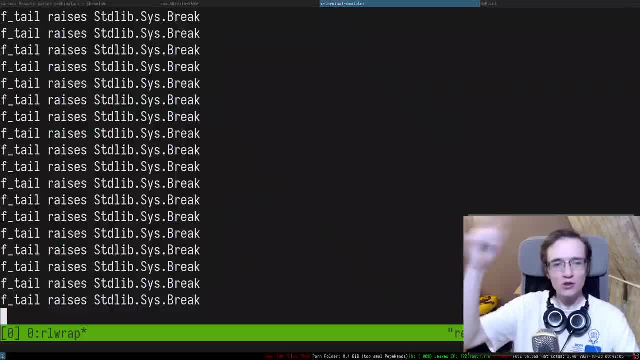 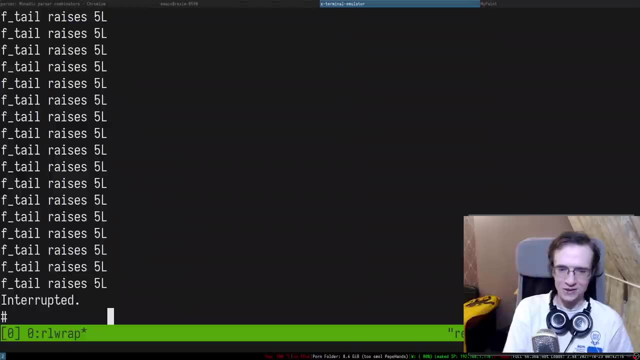 because when you control c, it rises the exception, and exception needs to go through the entire thing. oh, it keeps printing. oh my god, that makes sense. it's just basically printing, like everything that. yeah, so it's basically the stack trace, since it's a recursive. okay, that's actually pretty cool. thank. 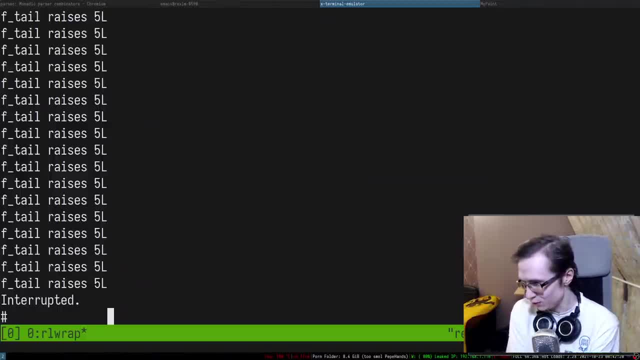 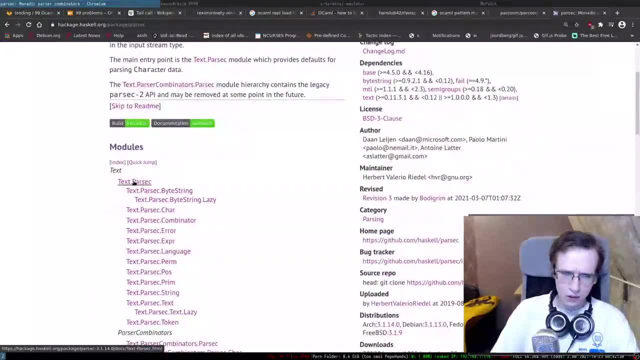 you so much, arctum. i didn't know about that, so that's very, very useful. i'm gonna use that from now on. uh, thank you, thank you, thank you, all right. so what i want you to say is that, in case of a parsec, all right, in case of a parsec, if you take a look at the parsec emitter that they they defined. 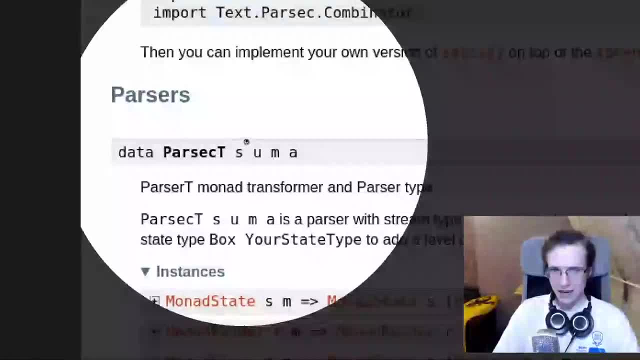 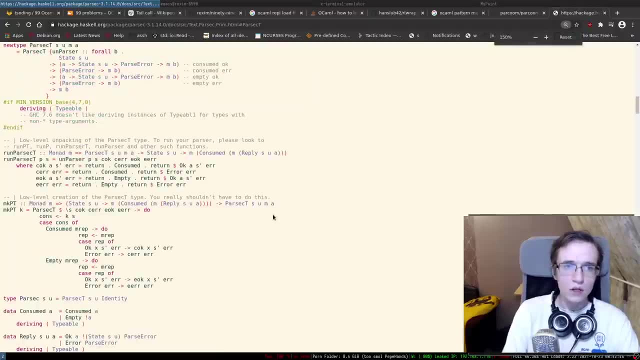 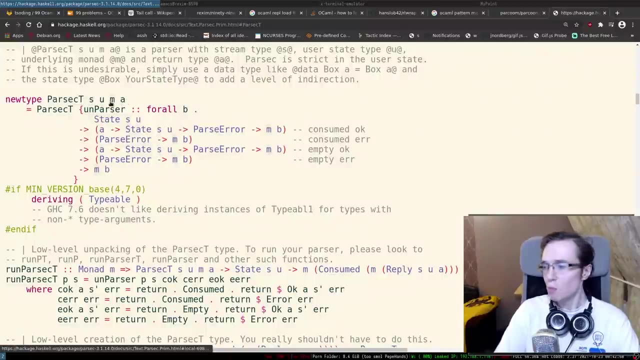 you can customize pretty much everything, like every aspect of the parser combinator, right. so if you take a look at the uh, at the definition, right. so you can customize not only the uh, the return right, a, you can customize the monet that is going to be used, right, in case of parkum, the only monet you're. 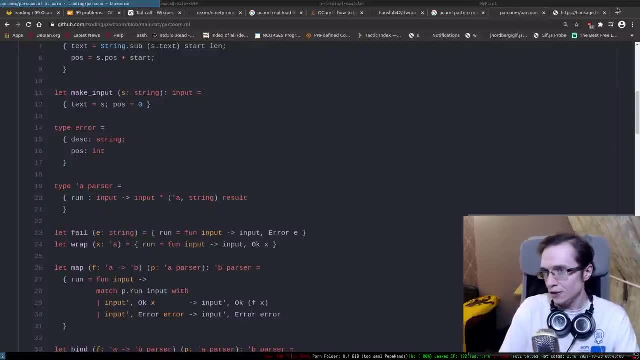 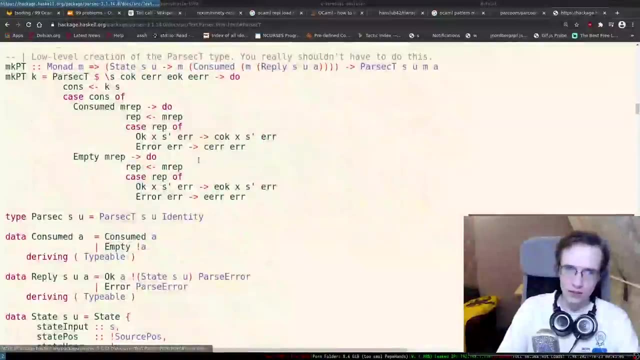 allowed to use is result. but if you want to have a different monet, well, you cannot do that in parsec you can do that. you can customize the input, the output and so on and so forth, and that's why it's a lot of like these weird things, like it's super generic, super like customizable and stuff like 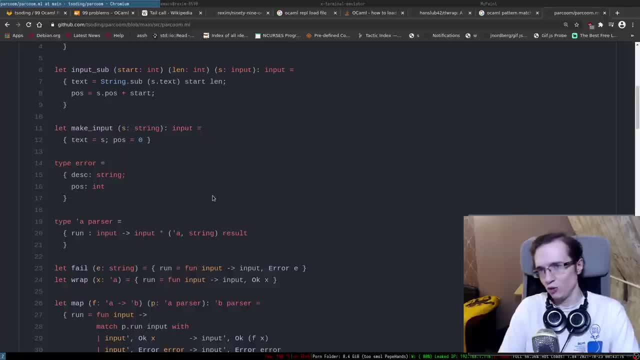 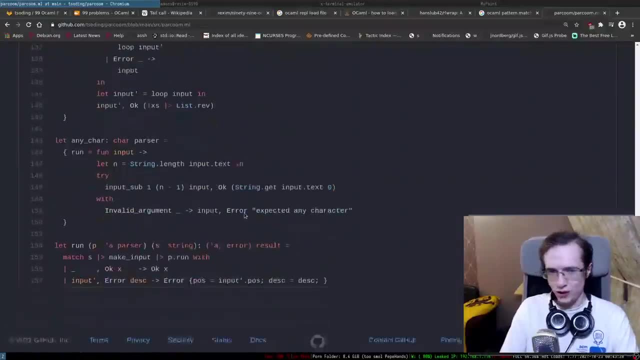 that my parsec emitter. you cannot do that. that's why it's so small, so simple and probably so fun to use, because it's not particularly customizable, right, but this is like a trade-off that you have to have to take because it's kind of difficult to make such a generic thing in a camel, uh, without. 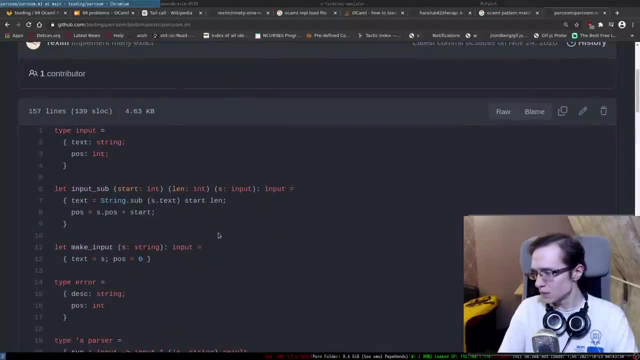 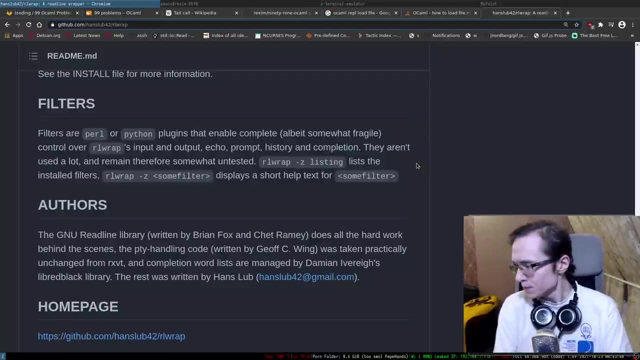 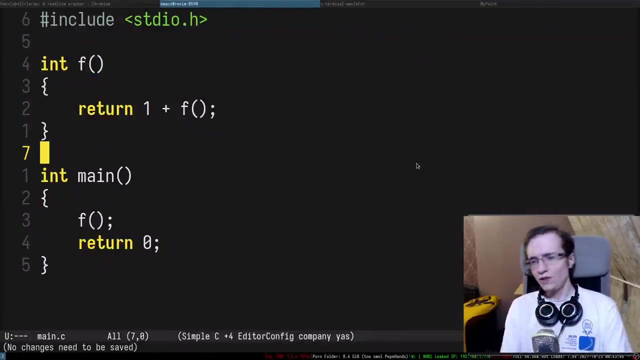 like type classes and stuff like that. but, yeah, so i've cut a couple of things out of the video, of course, to implement this thing in the camera. uh, all right, so, uh, let me, let me see, let me see. so we wanted to see if the uh c compiler actually 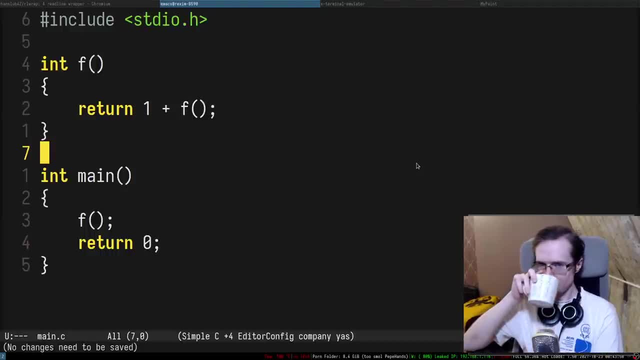 optimizes anything in terms of, like a tail recursion, right. so here is the not tail recursive function. let's see if it is going to, um, you know, a stack overflow mainc. this in the main, uh yeah, segmentation fault. so i would assume that segmentation fold will mean. 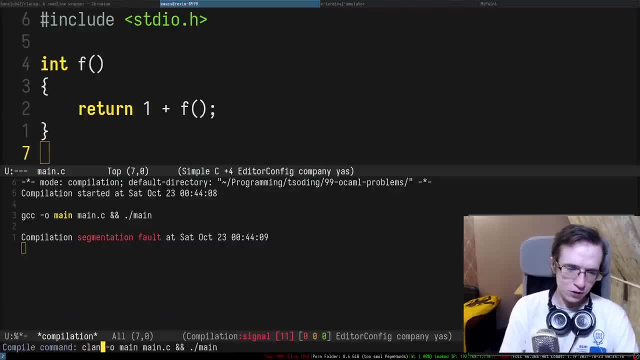 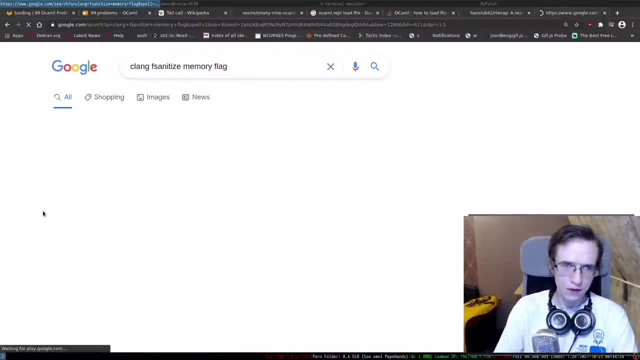 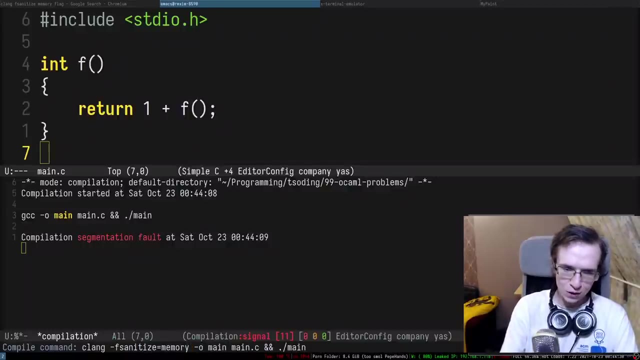 the um stack overflow. so maybe it would be nicer to do that with clank uh and clink uh. sanitize memory flag. um right f, sanitize uh memory. so i suppose it will tell me that we stack over flu if i provide this flag, hopefully. hopefully it will tell me uh. so there we go. so it's the 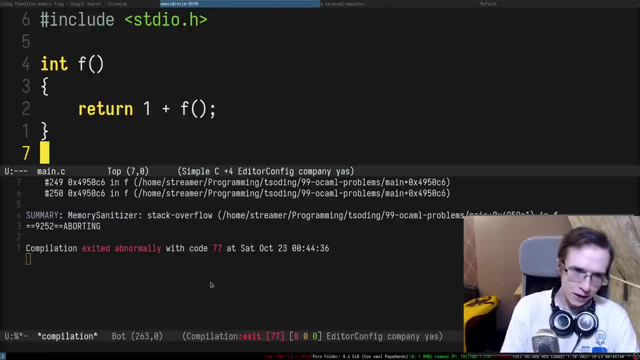 stack overflow. so now we can like clearly see that it's stack overflow. so if i turn it into sort of like a tail recursive one, so here's the result, and result is going to be simply plus one. uh right, so this is going to be zero and let's try to run this entire thing and, as you can see, 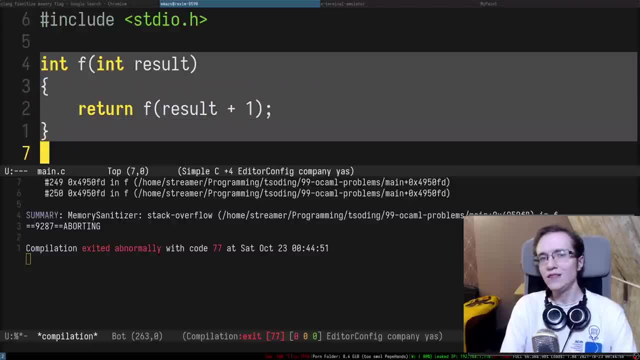 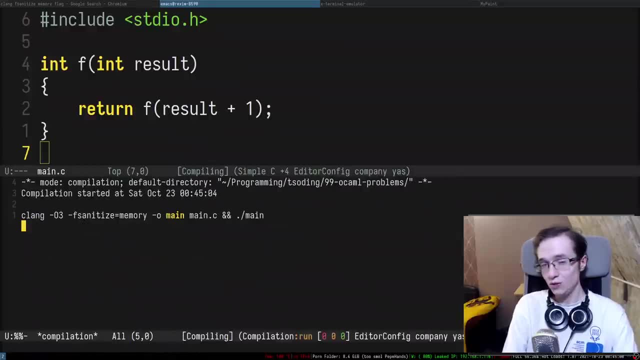 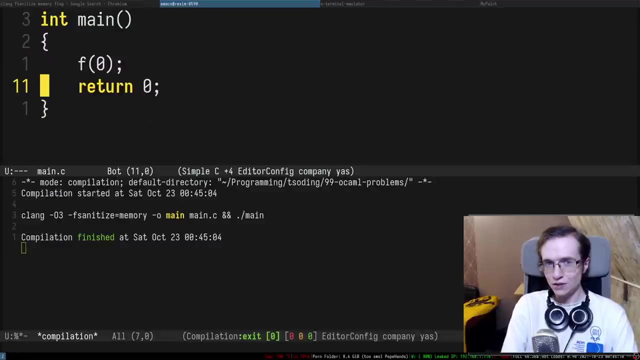 this, uh, stack overflow as well. so, uh, the compiler didn't optimize anything, but the question is what, if we crank up optimization to 03, will it do a tail call optimization? what's interesting is that it basically illuminated the entire thing. thank you, clank, very cool. so it's supposed to actually hang, but it didn't hang because you. 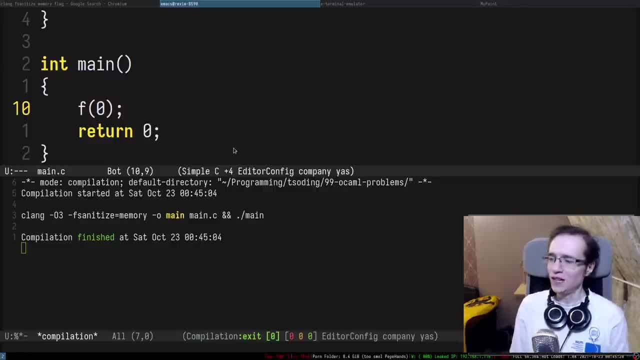 never used the result of this thing, so it just eliminated the call, like i mean, it turned into a lazy language, right? it straight up turned c into haskell, because this is what would happen in haskell. right? you don't use the result of the function. well it's, it will never be called. 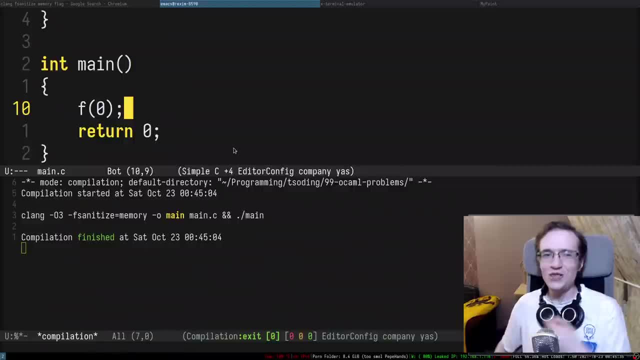 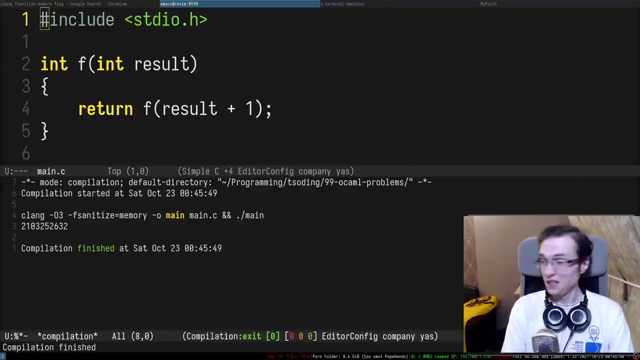 uh, right, pretty cool. thank you so much, so you don't need ghc to have haskell, so we can try to print. uh the the result of this thing to sort of force uh the the compiler to not eliminate uh the entire stuff, and it printed something. that's. that's what's interesting about it: it actually managed to print. 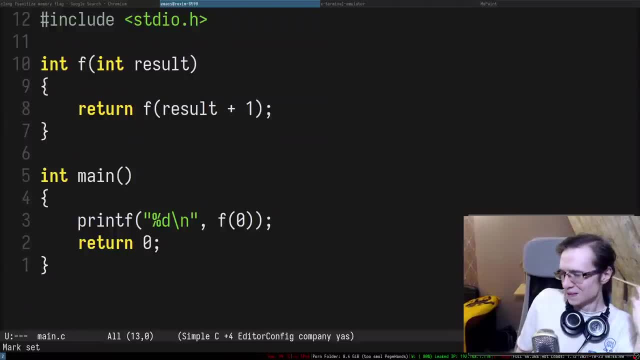 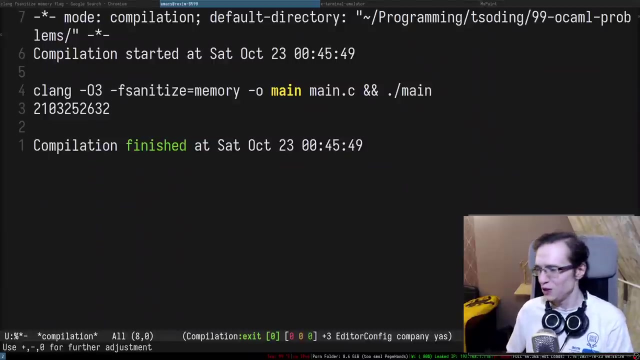 something. thank you very cool. um so, yeah, very cool. clunk sauce. yeah, i mean, we actually did all three, which is like very aggressive optimizations, but i guess in this kind of situations the optimization is too aggressive. is it different every time? uh, yeah, it is different, so it's probably printing like 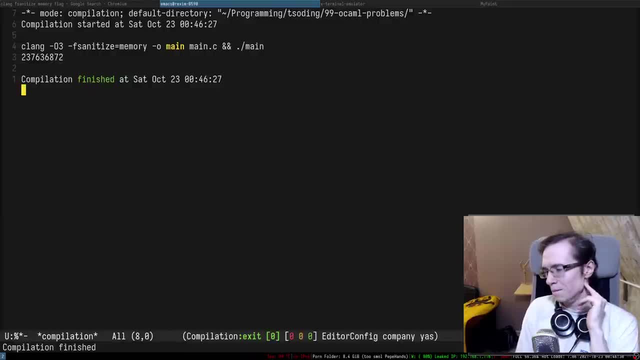 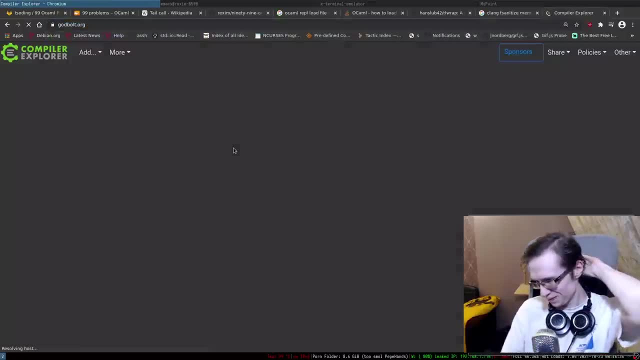 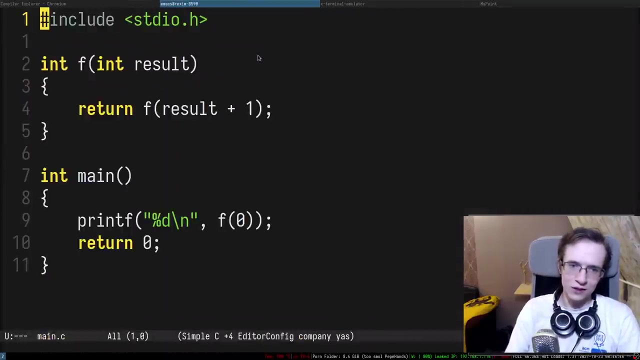 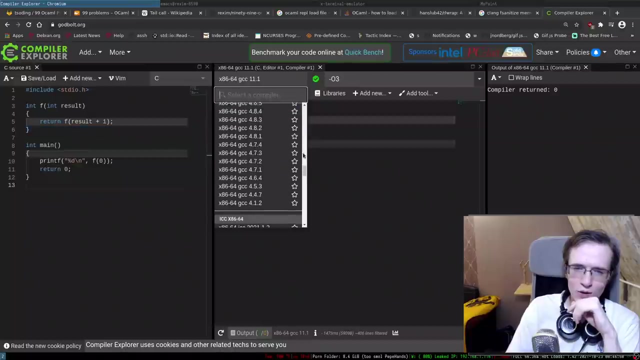 a random garbage from the stack, i would presume. um, so maybe that's what it's doing. um, uh, god the bolt. um, so let's take a look at what kind of garbage did it generate this time? okay, so, uh, clang. uh, i don't know what's my version of clank to be fast, so maybe i'm gonna just choose. 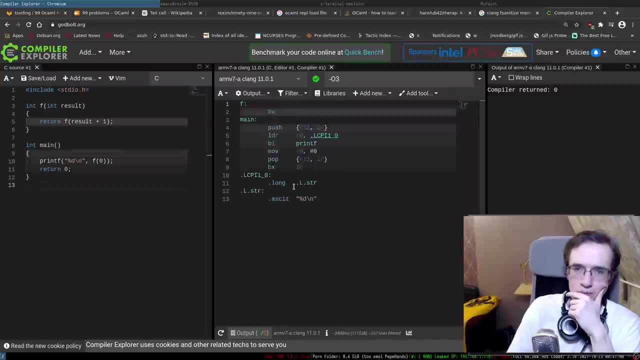 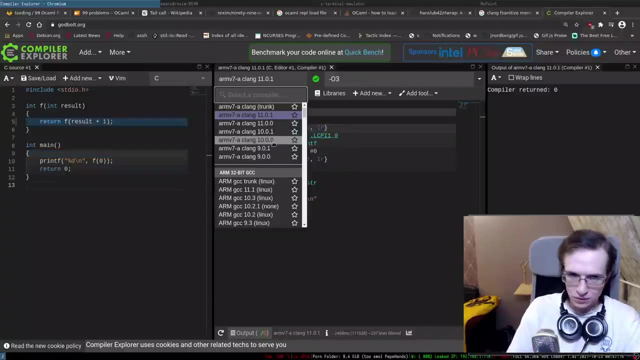 uh, like the latest one, or whatnot. so what is it doing? uh, two d r push. oh, it's r holy, okay, so i'm an idiot. uh, or maybe god bolt is not as convenient as it should be. maybe it's not me who's an idiot, oh, 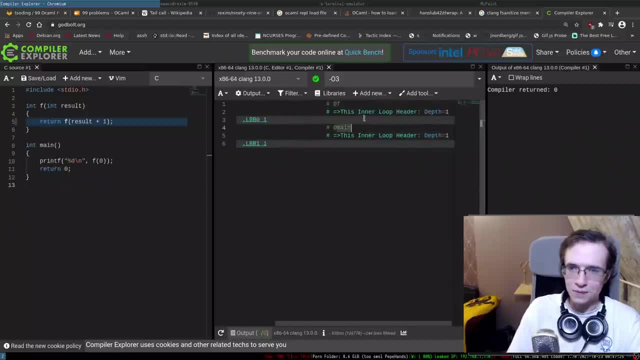 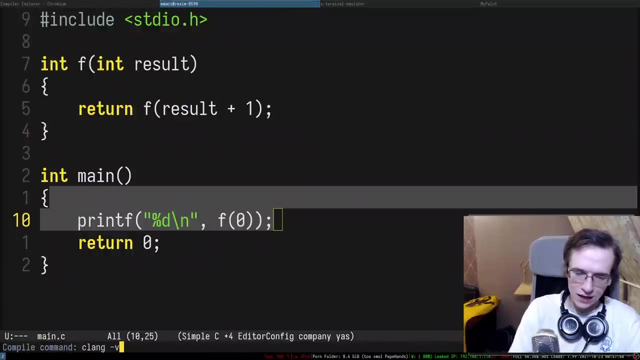 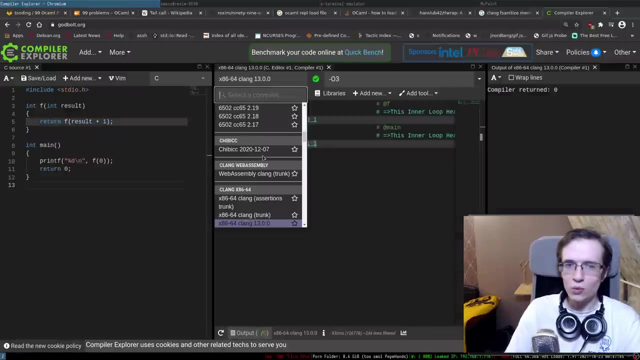 very cool. um, okay, so in main, we jump back to here. well, we're supposed to loop right. so, uh, let's maybe use the, uh, the clan that i have. uh, this is not how you diversion. this is not how you diversion. uh, 701, right, i have a pretty old one because i'm onztip in. 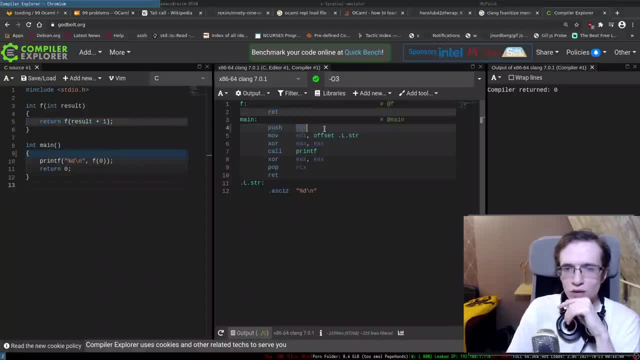 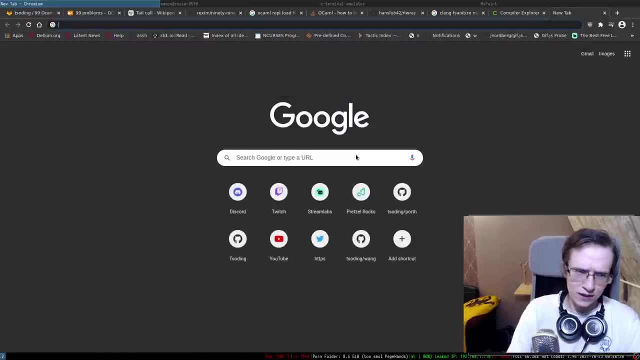 now that looks like something. okay. so we push in rex, uh ede. okay, so this is the uh, the string. we push in the string de string uh-huh. oh yeah, so essentially it prints. so the second argument, as far as know, is rsa right. so um x86 64, like system v, uh call convention. so we get a rate from provost. 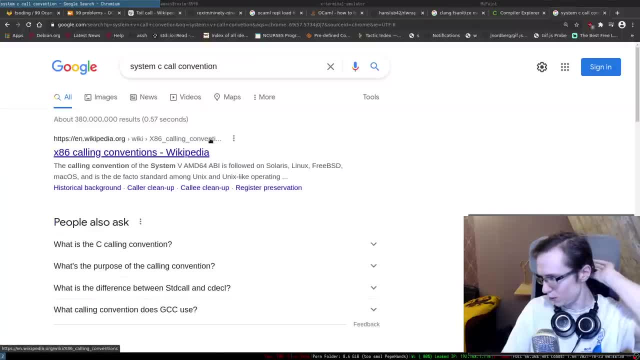 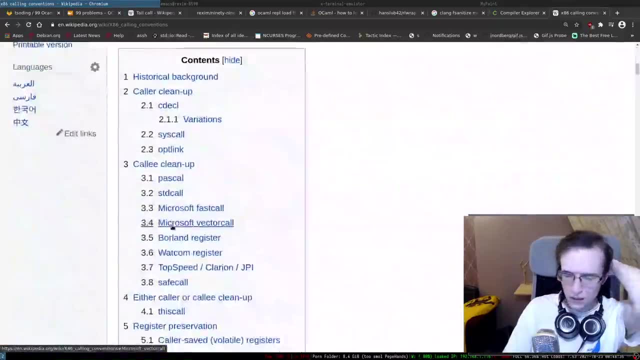 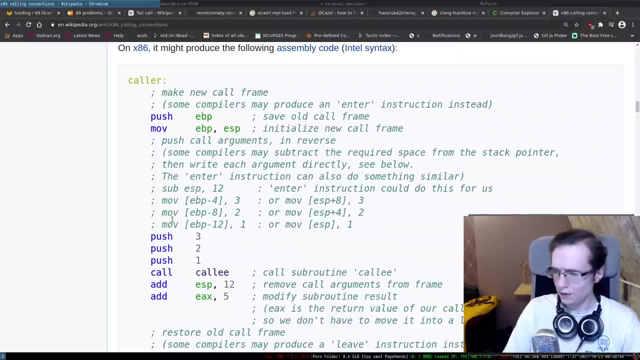 uh, thank you. thank you so much for the rate. how was the stream? uh, we're just doing some weird shit. so, as far as i know, it's first rdi and then rsi, right? so what's the second argument? does anyone remember what's the second one? but i suppose the second one is not even present there, so basically, 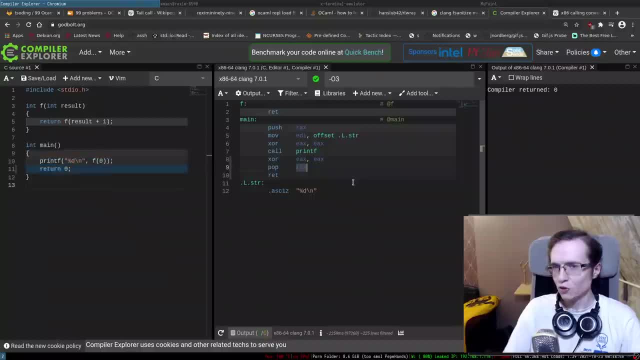 it will print a random garbage from the, from the second argument register. so that's basically what it optimized to um. is this for port? no, it is not for port. we're just exploring how c compiler may potentially perform tail call optimization. that's what we're doing. 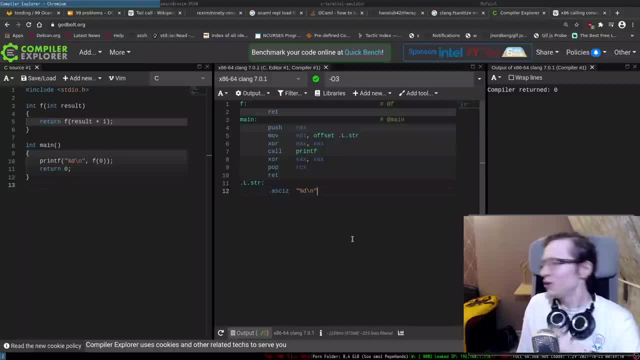 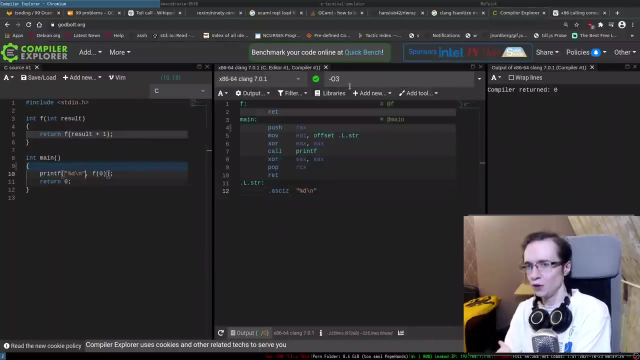 right now. uh, so we were just discussing the tail call optimization and we just want to see if any of the compilers actually perform them. so we did this thing and what's interesting is that clang on, like clang specifically of the version 7.0. uh, with o3, it illuminated this call completely. 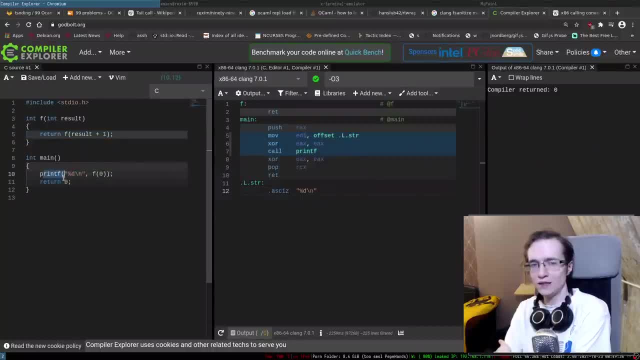 but it didn't illuminate printf. so basically it's printing a random garbage from, i would presume, rsi, right? so the first argument is rdi, the second one is supposed to be rsi, but rsi is never set anywhere, because setting rsi, i presume, was illuminated. so nice one clang. thank you very much. 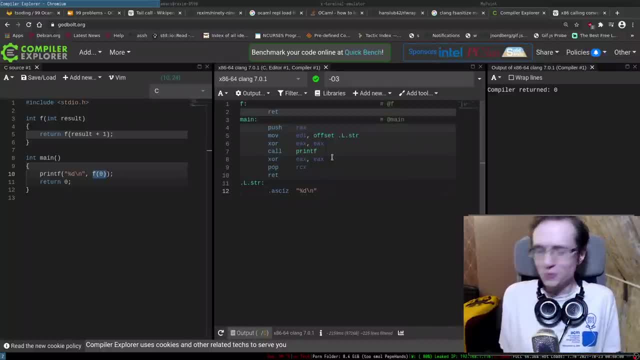 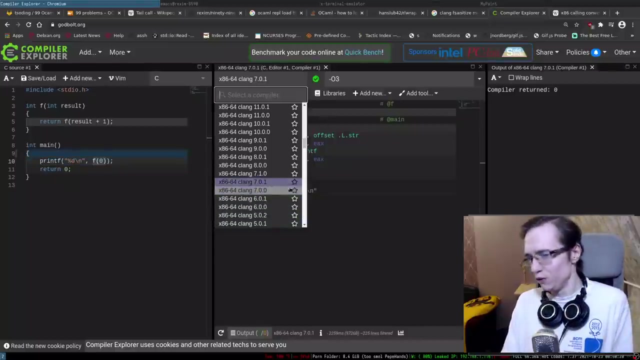 uh, isn't the code an infinite loop? yes, that's the point, uh, and it would expect it to actually loop indefinitely. but the infinite loop was eliminated. uh, and now printf just prints the random garbage from the, from the registers, so it remains so smart. well, uh, in defense of llvm and um clang, we're using a pretty old version of. 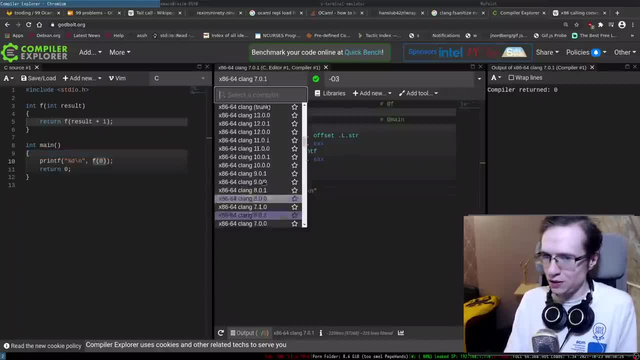 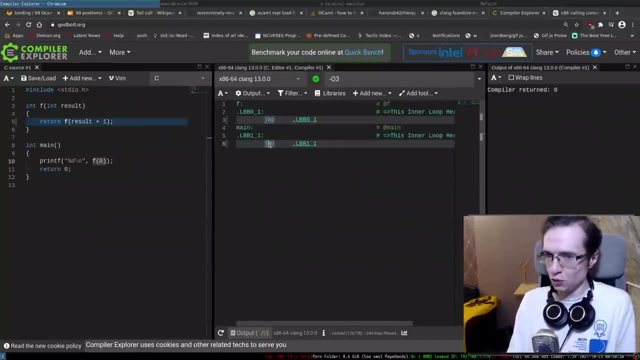 the compiler. right, because that's the version on my old debian machine. so the latest one actually produces something more reasonable. right? so the latest one produces straight up infinite loop. so jump to itself, which is precisely what i meant here. i believe it or not, it even illuminated printf. 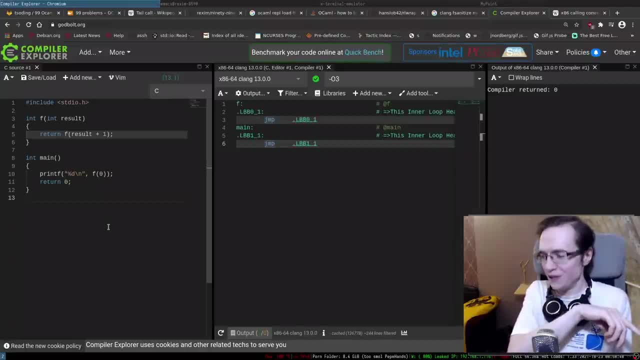 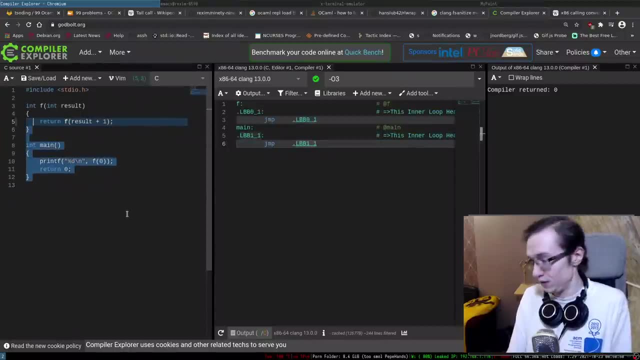 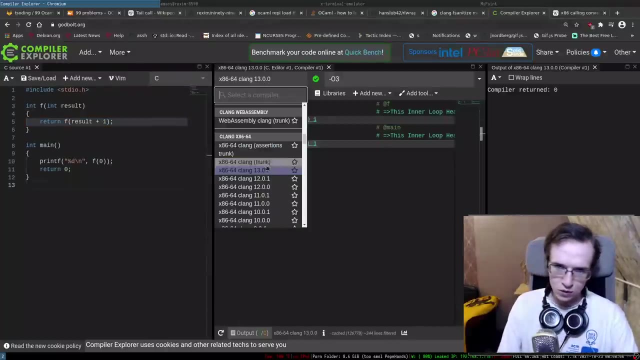 the seventh version eliminated the loop but didn't eliminate printf. the latest one illuminates printf but didn't eliminate the loop, and so this is closer to what i actually meant in here. right, so it's closer to my original intentions. can you show? oh, one on which compiler? uh, on the. 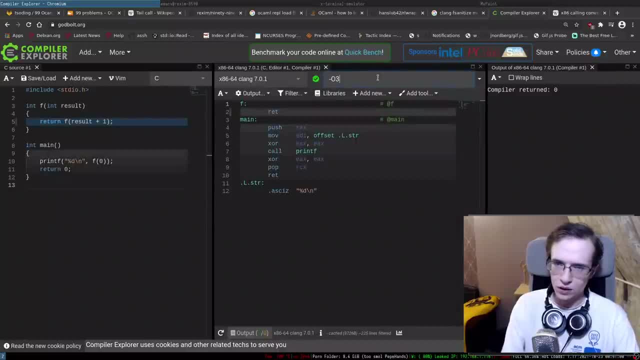 old one or a new one. so let's take a look at the old one. so, uh, this one, oh two. uh, oh two is the same. uh, oh one. um, oh one will probably a oh zero. what about those? you oh zero now produces something reasonable, like i mean. 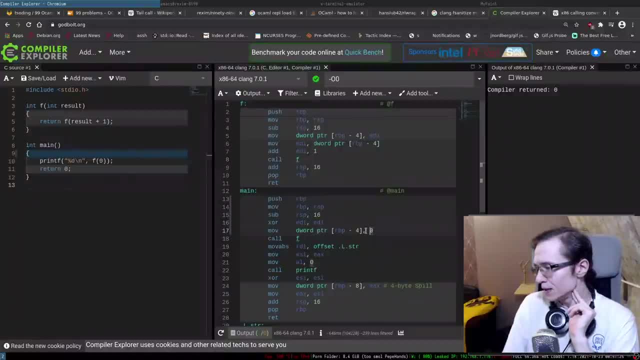 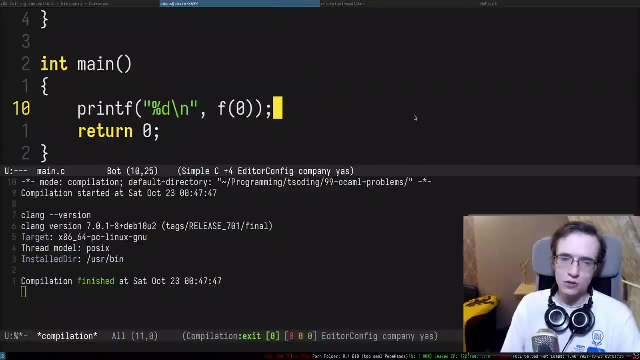 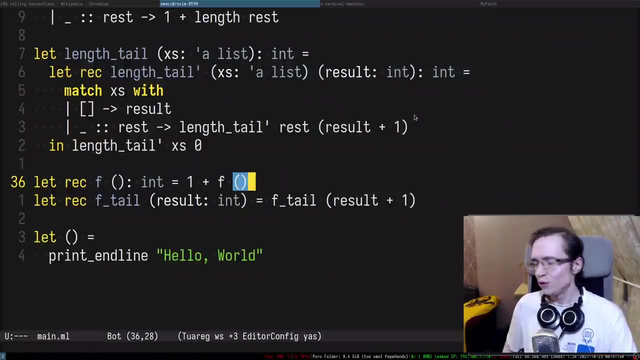 it's just that didn't apply in optimization. so let's just look straight up. uh, so anyway. uh, we just were talking about tail call optimizations because we were doing a functional program- rising girls. we're not programming in c right now, we're programming this. uh, people who came from prod, who knows what this language is? 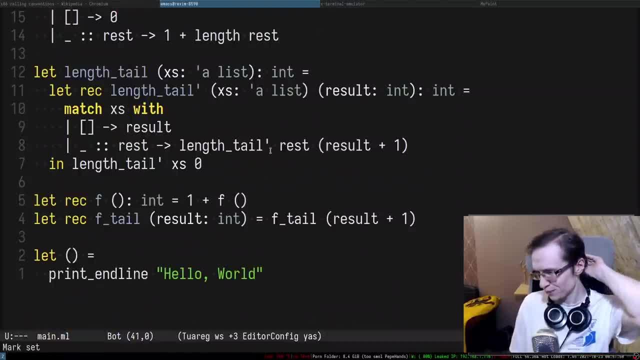 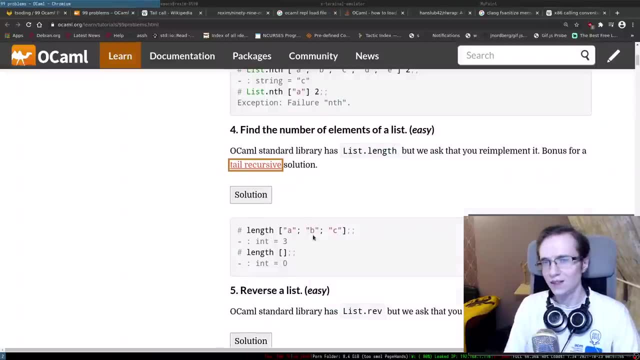 so new people who came from prod, what is this language? okay, somebody knows this language, yes, and what we're doing right now? we're solving 99 uh okamo problems. so that's the topic of today's stream. it's not sml, it's a camel actually. 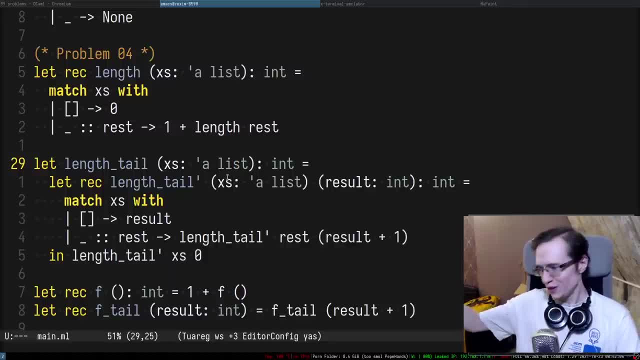 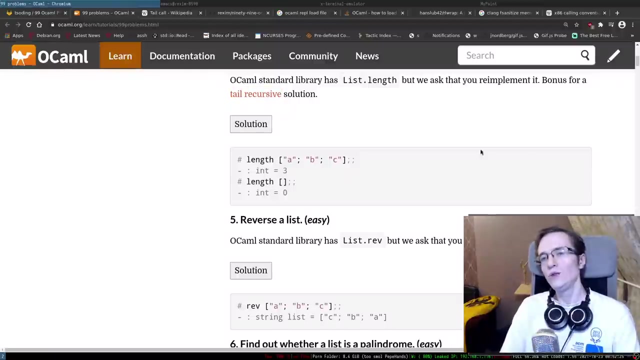 right. so the uh god ball thingy was just basically a tangent. the main, um, the main topic of today is actually, you know, solving 69 okamos problems. you can find the source code of the solutions in here. um, all right, so, oh yeah, that's pretty cool, okay. so, uh, we looked at two different solutions, right? the? 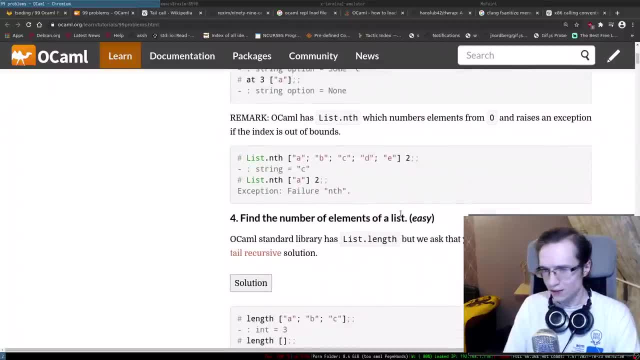 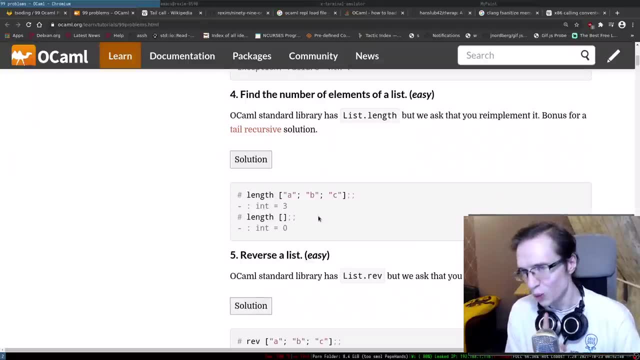 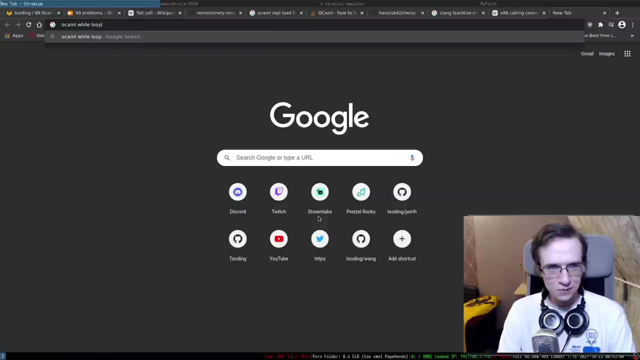 first solution is um request, recursive one, and the second one is a tail, recursive one, but not a single function programming programmer will talk about the third solution. who knows the third solution? not everybody knows, well, i mean, functional programmers know about that but will never tell you. but in a camel you can have, i think, while loops right, um loop and recursion. 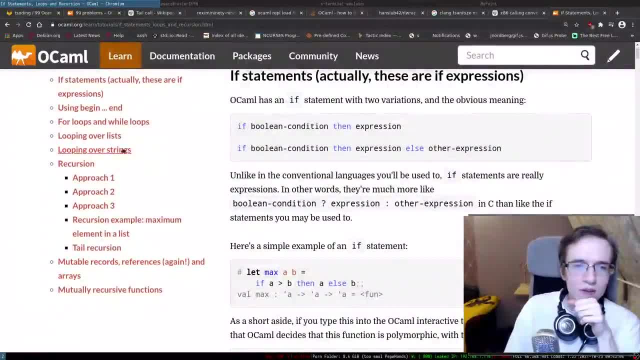 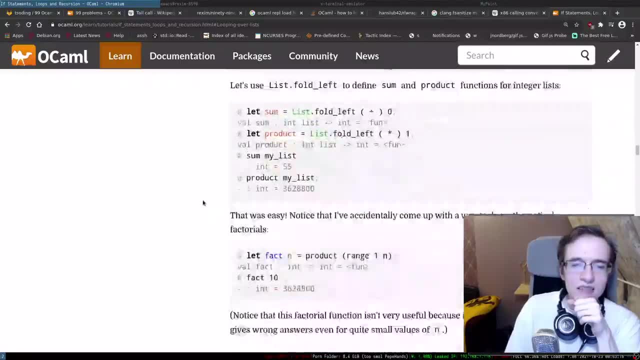 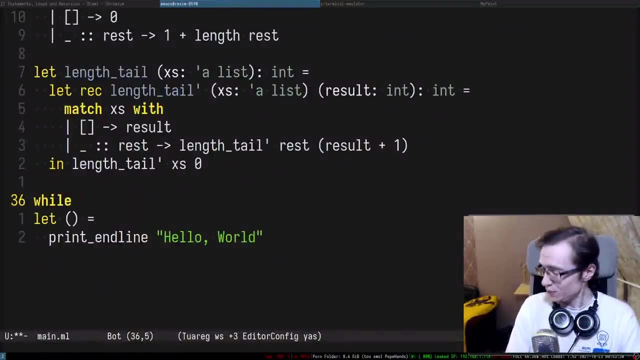 i think. do you have while loops or for loops looping over lists? i think there's only uh four loops in here, right? so if i try to do something like while there is a while, there is a while, you, okay? so let's actually call this best: uh length, right? so this is going to be access, uh a. 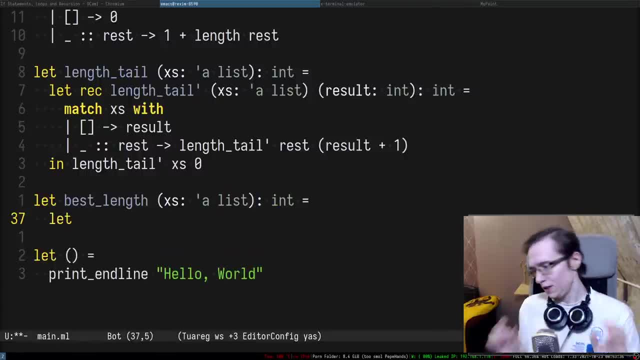 list and this thing is going to be like this. right, one thing in a camel is that, even though it's completely immutable and completely functional and so on and so forth, you can define mutable variables in there, right? so you can define variable result and it's defined. 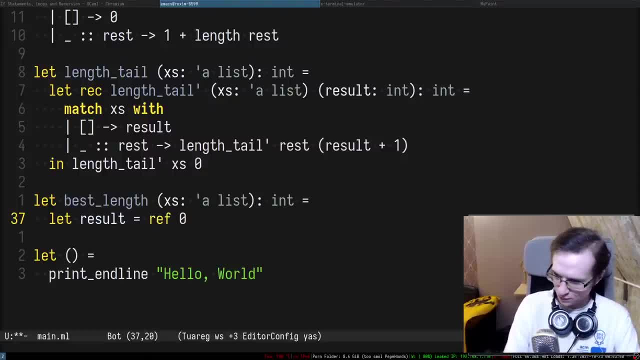 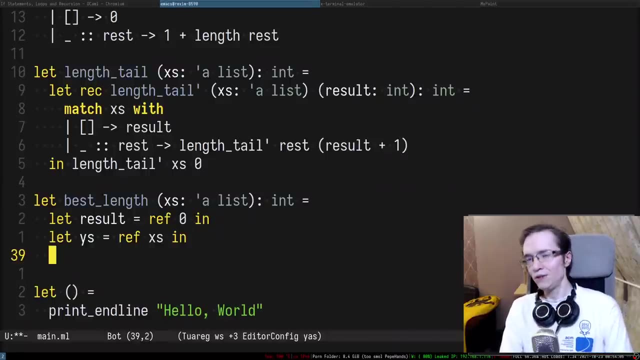 through a feature called the ref right. so you define the ref zero right and then you can have your list: uh defines uh also in the ref right. so, and one of the things you can do- you can basically have an imperative loop, uh, an imperative loop that basically loops while the 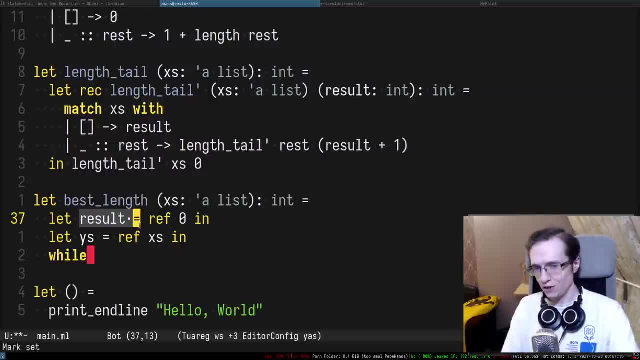 list is not empty and imperatively increments the result and then just returns the result when it's done. so this is the third solution that not a single functional programmer will tell you about, but i'm gonna tell you because i'm not a functional programmer, i'm a python developer, right? so i'm gonna. 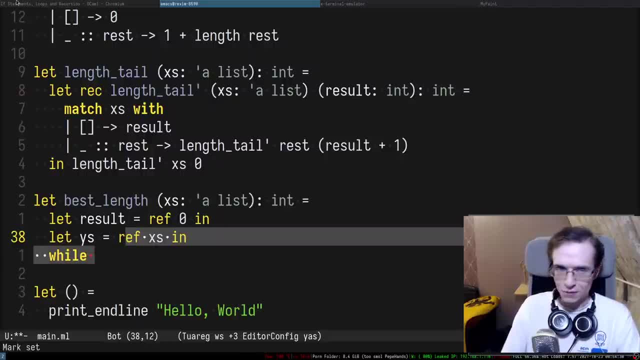 tell you that little secret that you can do this kind of stuff in a camel, but i forgot how to use while loops. okay, so this is how we do that. you do while true, do blah, blah, blah. so, if i remember correctly, uh, to read a value from a ref, you actually use exclamation mark, mark and you. 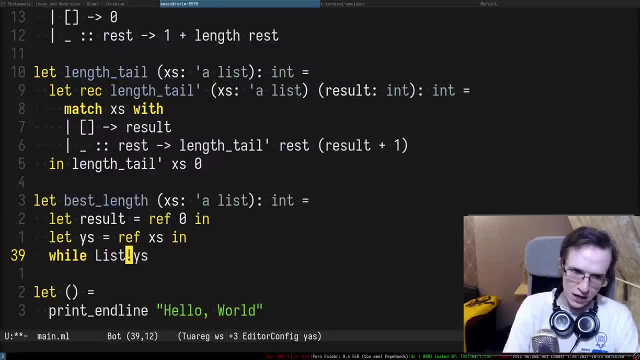 sort of dereference it. so you basically read this entire thing and then, uh, you can check if this in this entire thing is equal to an empty list. while this thing is not an empty list, do result, equal result plus one, and then wise, equal, um, wise list, uh, i think, tail right, uh, list tail, and then done. 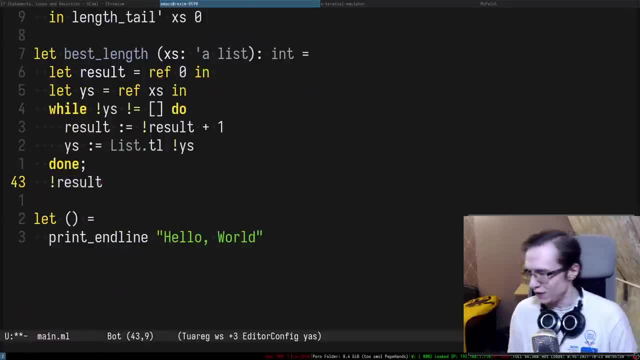 there we go, and after that you simply return whatever you have in the result or do a rewrite. that's exactly what you're seeing: the same thing. i'm not gonna do it because you won't see it, so we'll just make it simple and it's just another teacher's. 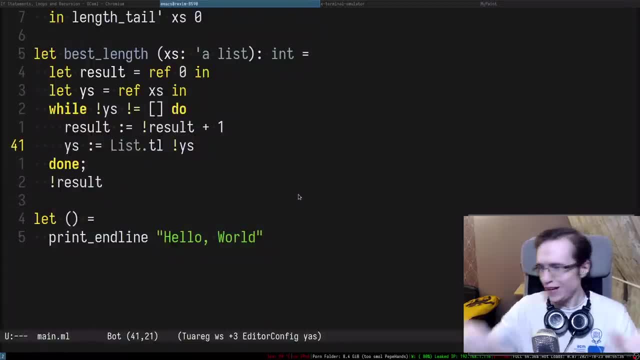 test this is. it's a first class test, so i'll show you later how to do this. so we go right here. what we're doing is we're adding the tool under this one, the third secret solution that nobody except me will tell you. i wonder if it will compile. actually, you can see. 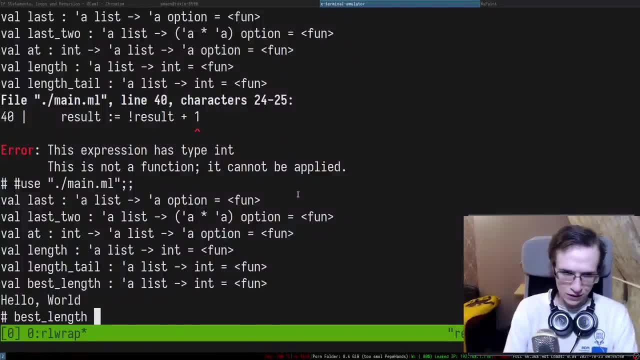 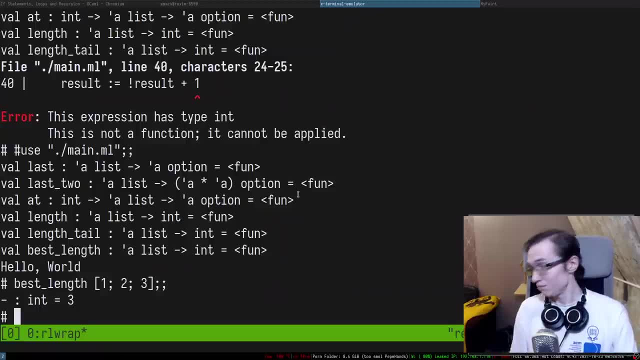 okay, so, user, and it does not even compile. oh yeah, because you have to if you have like a um, you know, One, two, three, It also works, It also works. So this is the best way to compute the length of the list in a camel. 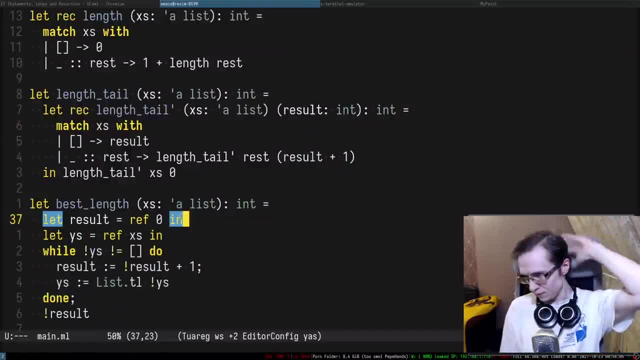 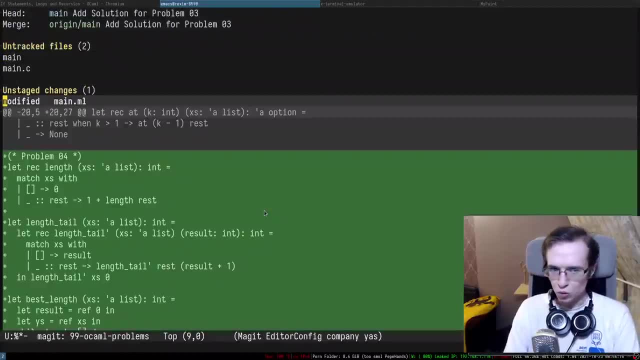 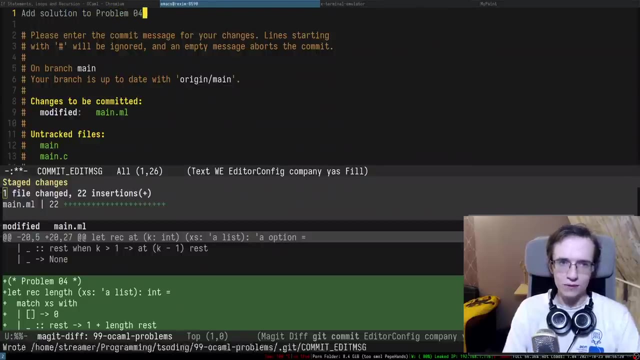 This is the best one. So, all right, Let's do a committee, committee And maybe even pushy pushy, Add a solution to problem 04.. And I'm going to push that right into the repo. And the repo is public. 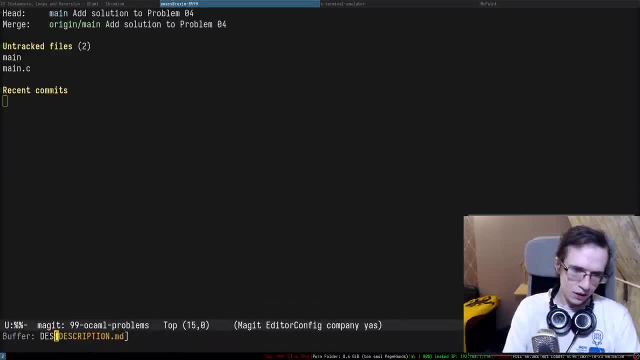 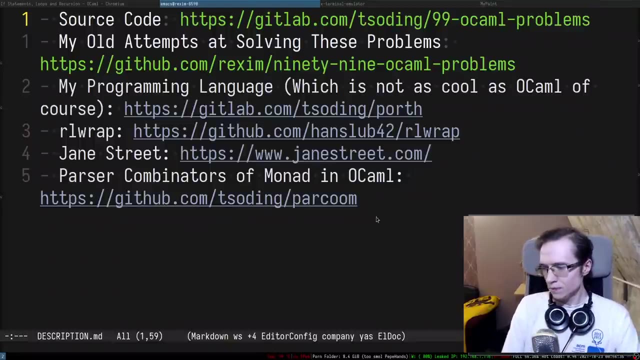 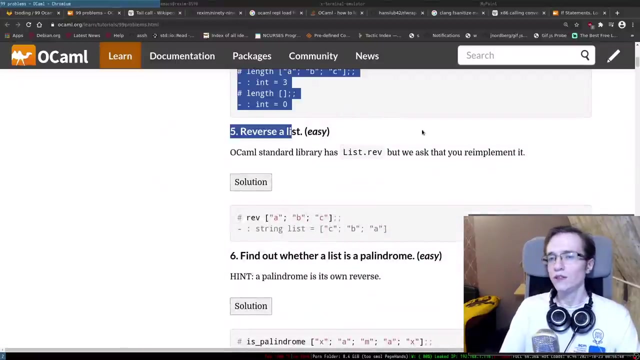 You can find it in here, And if you're watching on YouTube, you can find the repo in the description. It's the first link in the description, So okay, So reverse list. This one is interesting. This one is interesting. 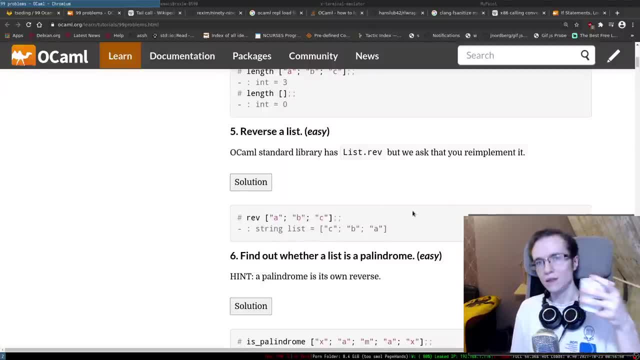 How do you even reverse a list? Well, You can use while. Oh my God, I just got a perfect idea. Holy shit, Here's an idea: Solve all of the 99 OCaml problems in OCaml in imperative style, using mutable variables for loops and while loops. 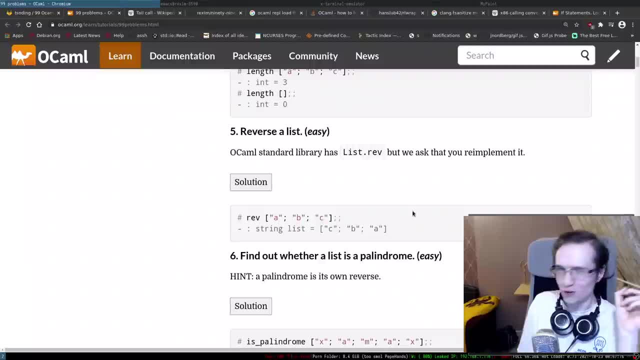 And just like promote that shit on all of the social media to piss off all of the functional programmers. That's beautiful. I want to do that now, Holy shit. I want to solve all of them in imperative style in OCaml- Yes. 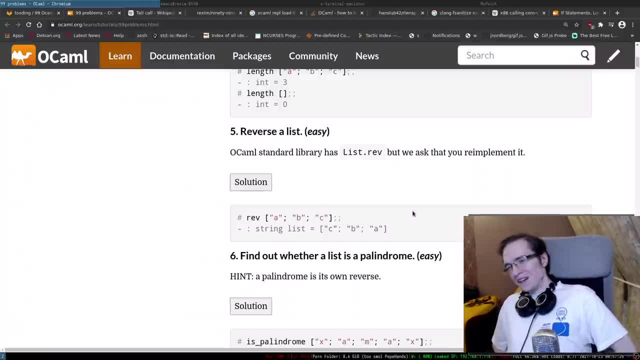 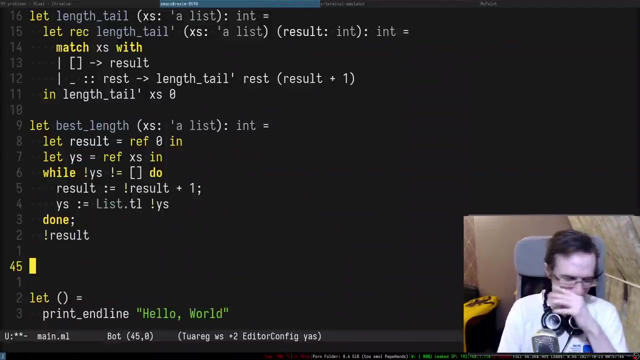 That's actually so cool. I want to do that. Oh, Oh, I don't know. I'm too tired. to be fair, I'm kind of too tired for this kind of shit- Too old, Oh dear. I already have enough people telling me that I'm programming things wrong. 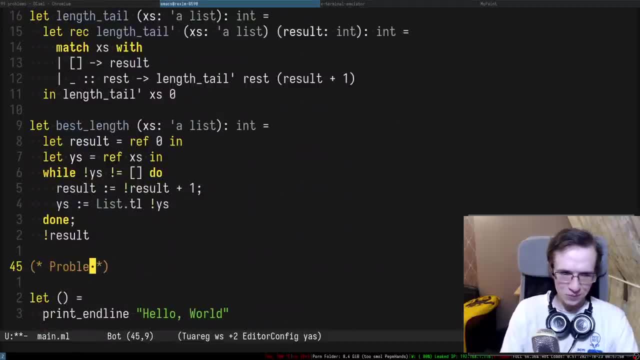 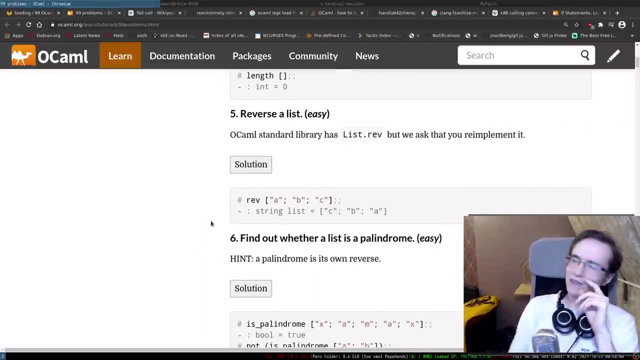 So All right, Problem 05.. Problem 05.. So I think what's cool is that you can kind of reverse the list by doing the accumulator thingy, I think, Because once you push into accumulator you sort of push things in a reversed order. 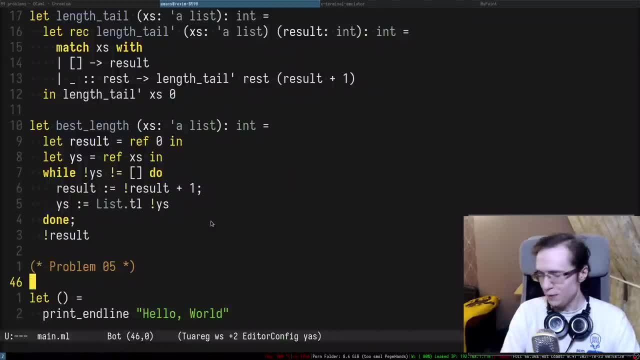 All right, So let's go ahead and do that, And maybe this is going to be the last problem, because I'm feeling a little bit tired already. So, yeah, Let's do this as the last problem, And then we're going to wrap things up. 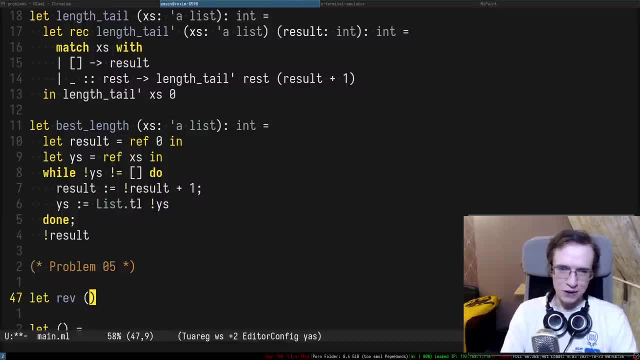 And I'm going to think about, you know, 99 OCaml problems, but imperative style And, by the way, so maybe I can even stream that, Because imperative OCaml is easier for people to understand than the functional one, Right? 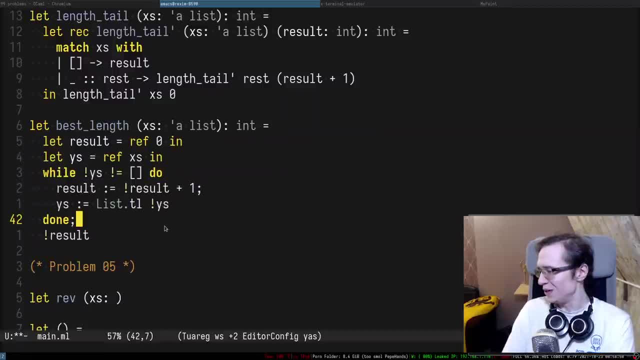 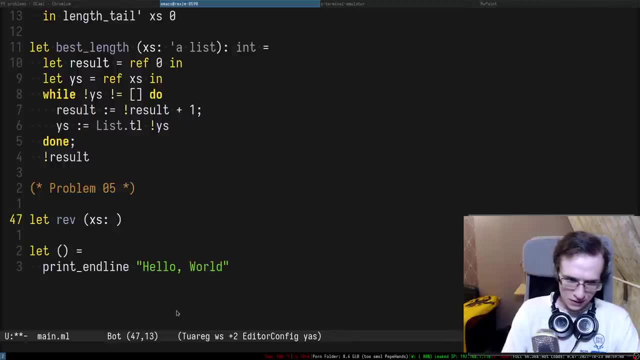 Because it's just, yeah, It's just like Python, It looks kind of like Python, So Okay, So this is the list. It's actually a list And we can have something like an accumulator, Right? So it's going to be like that. 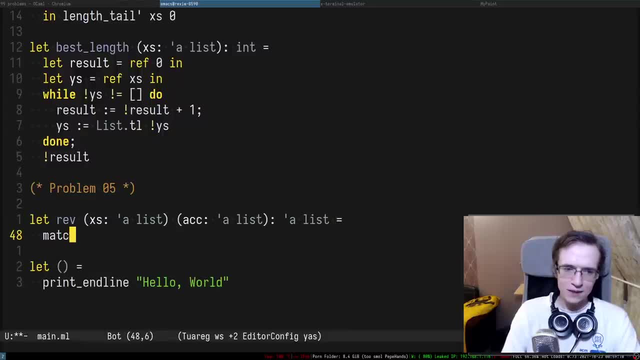 And then we're going to return this list. So we're going to match access And if access is empty, we're just returning the accumulator. If it's not empty, Right, We do a reverse where we provide the rest, But we append X to the accumulator. 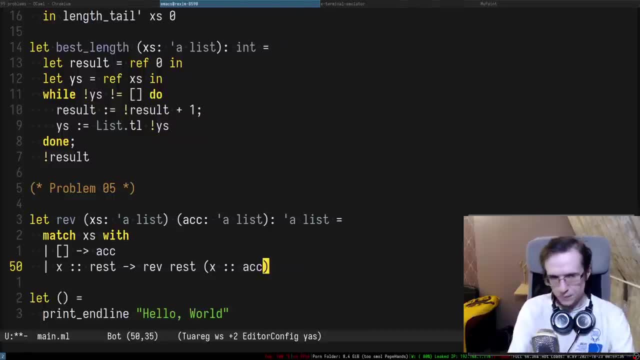 So here is the thing. So, essentially, how do we work with all of that? I wonder if I can just use- I think I can use- tracing to demonstrate how this entire thing works. So yeah, Thank you so much, Arctoon, for teaching me about trace. 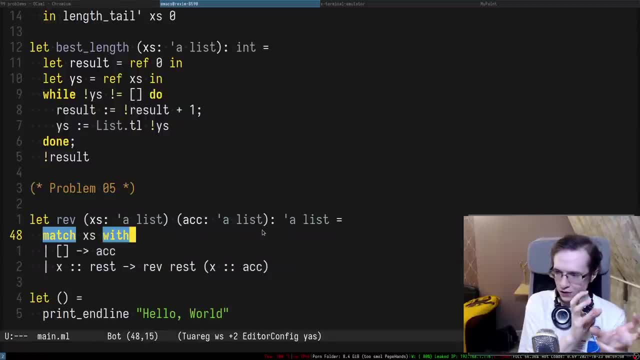 Because I think I would be able to use it today And I would be able to demonstrate how this reversing actually works. Because what it does? it chops off the head of the access and pushes it into the accumulator on each iteration. So basically, like push and pop and push and pop, push and pop. 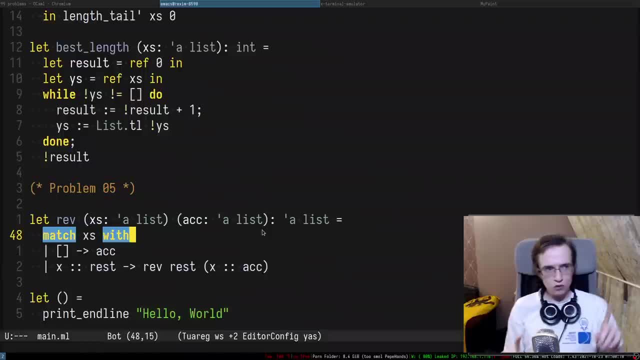 And that's why it's like a reverse. It's like having two stacks: If you pop from one stack and push to another one, the second stack will be reversed version of the first one, Right? So? and this is basically the same situation. 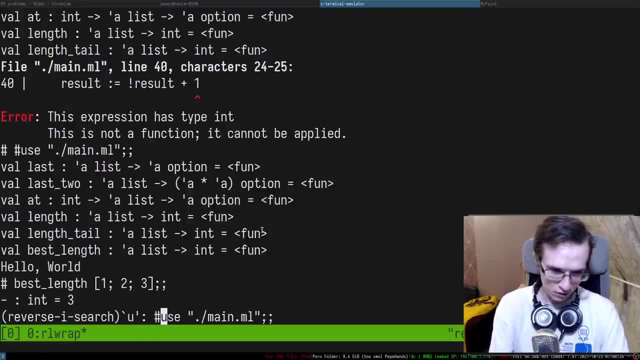 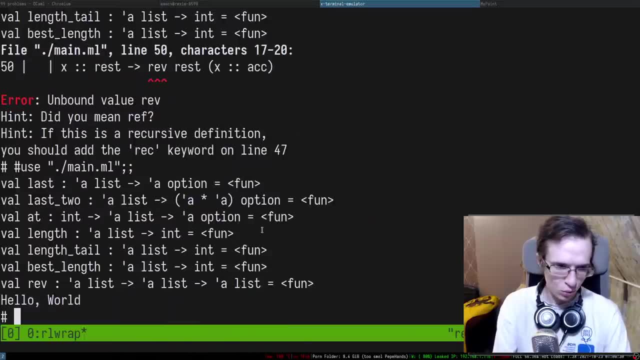 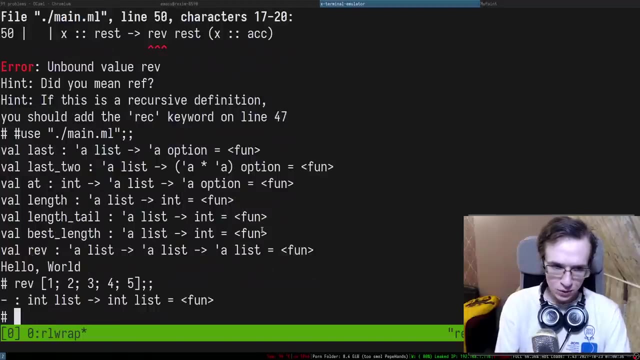 And I wonder I can actually demonstrate that with a trace. So let's kind of do use, And of course I forgot to mark this entire thing as a recursive one- Use one more time And if I try to reverse one, two, three, four, five, it will. 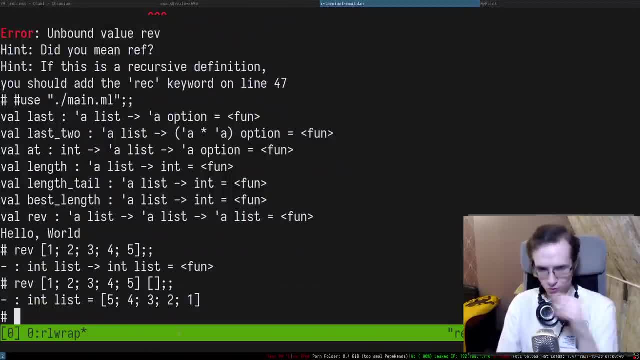 Oh yeah, I forgot to actually provide the empty list. There we go, So, as you can see, the result is actually reversed, But the way it works Like Towers of Hanoi. Yeah, It's kind of like Towers of Hanoi. 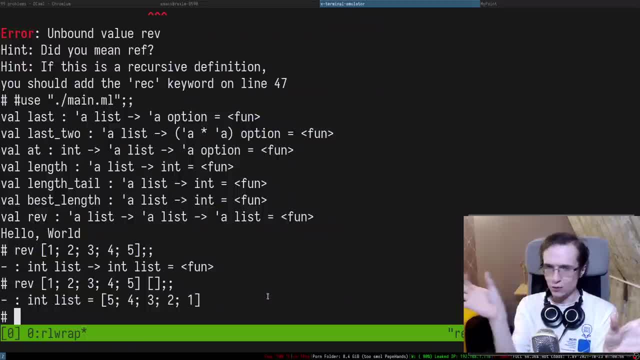 So essentially We have two towers in here. The first one is an input And the second one is an accumulator Right. So we just push into another one. Can we try to do trace rev Right? So rev is now traced. 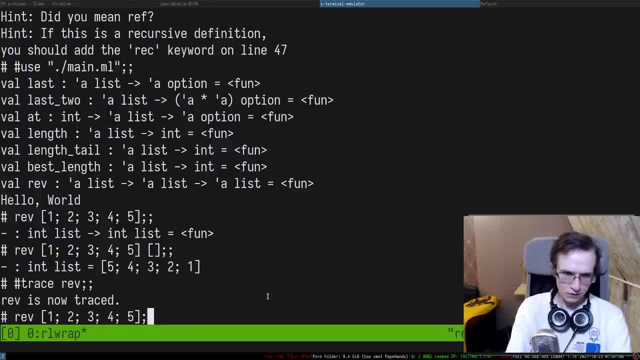 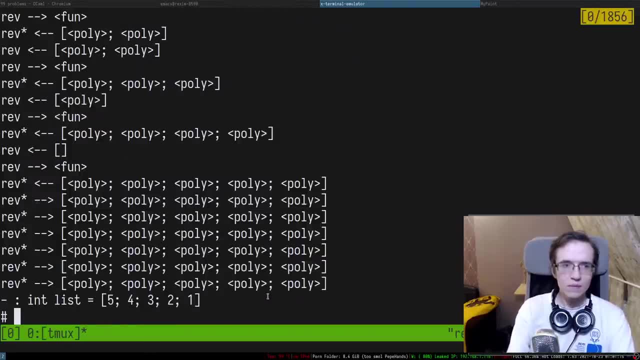 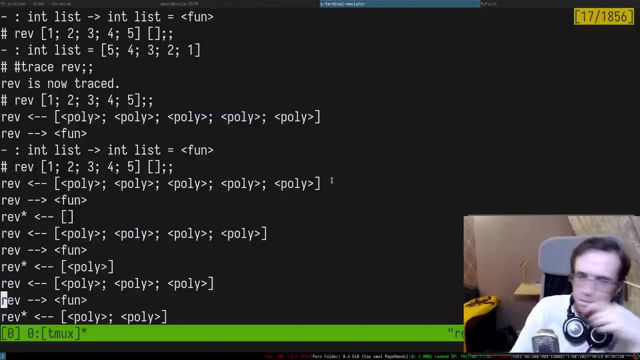 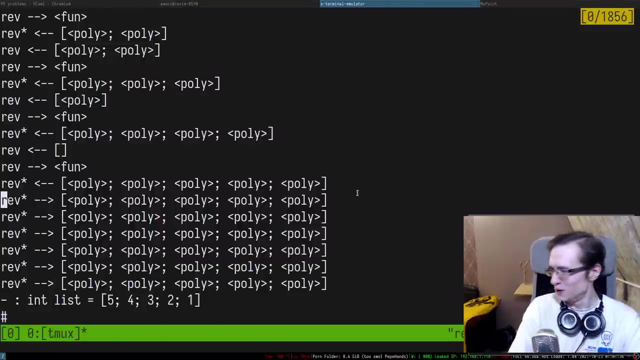 And if I do one, two, three, four, five, Oh yeah, Of course. Okay, So poly, poly, poly, It doesn't really tell me much. Okay, That's very cool. Roly poly, Roly poly. 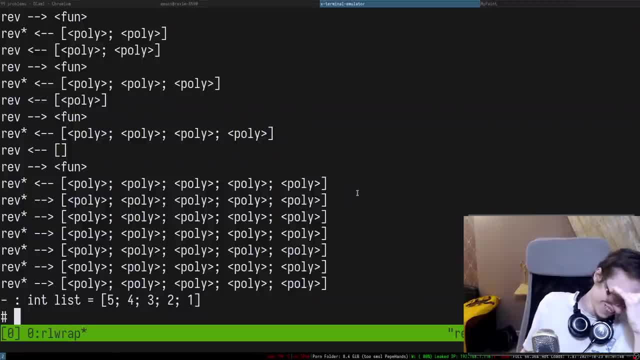 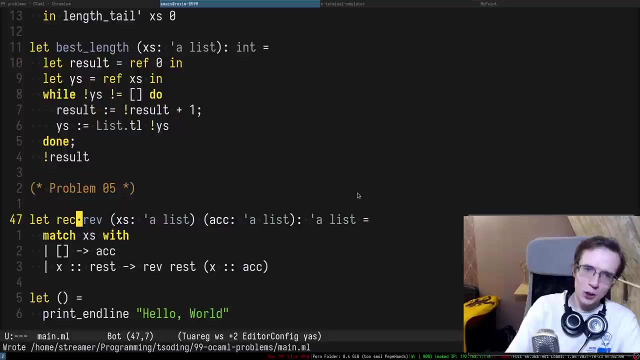 Roly poly wants a crack. It's cool, We can try to. maybe Is this because it's carried. Probably This is the special behavior. Oh, okay, I see What if we make it uncurried? So can we try. 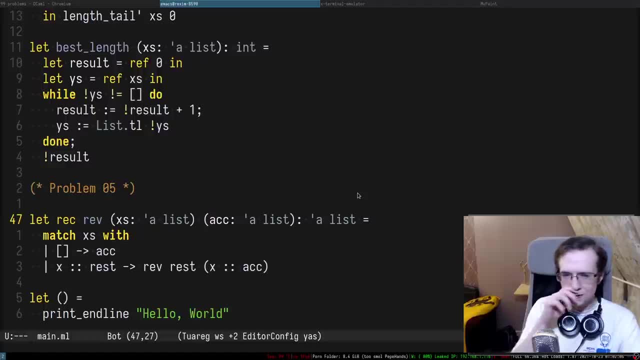 Well, in case of making it uncurried, will it be still? Yeah, it will be still recursive, or something. Okay, So we can try to do that. So it's going to be access And we're going to just do it like that. 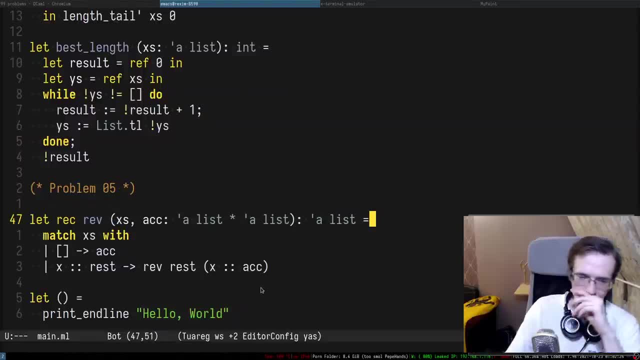 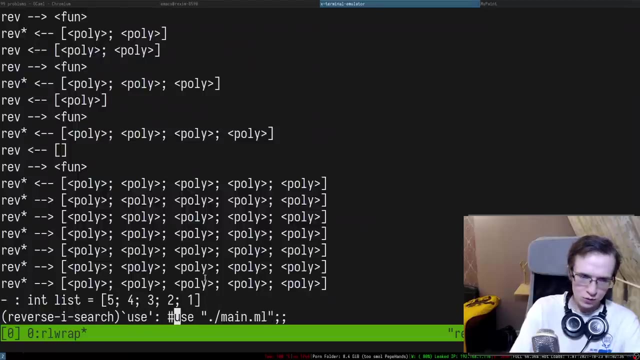 Right. So if I try to do it like that, will it give me more information about this thing? Probably not, It's just probably not. And then if I do reverse, this is going to be the rest. And yeah, use. 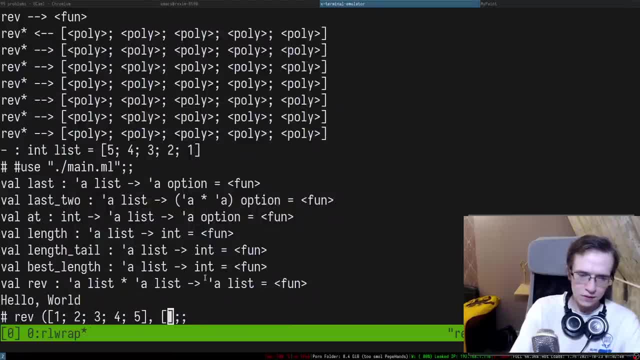 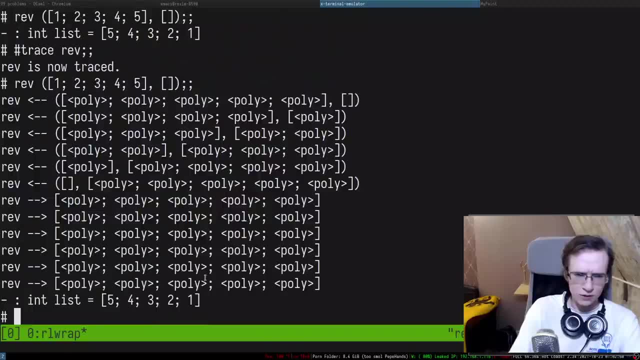 And now if I call this thing: Yeah, I forgot to trace, Probably not, It's probably not going to. Yeah, Well, this is a little bit better. So that's at least something that I want to see. I would like to see the actual elements in there. 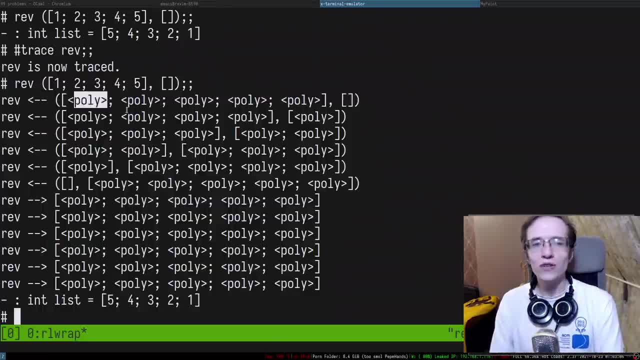 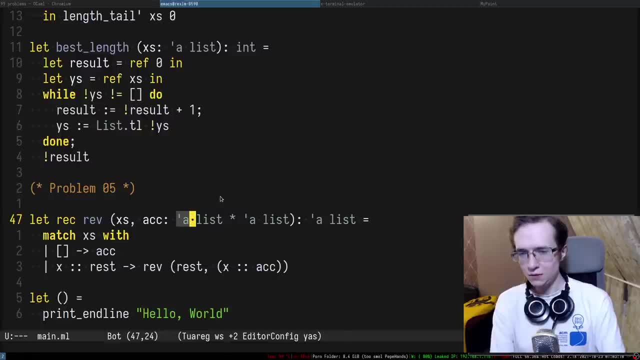 You know what? It's probably polymorphic argument. That's probably what it means. It's a polymorphic argument. Can I make it print actual values? if I specify that these things have to be integers? Okay, So that's probably something that we can do. 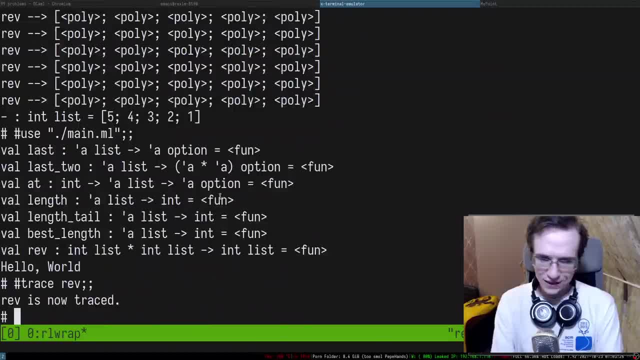 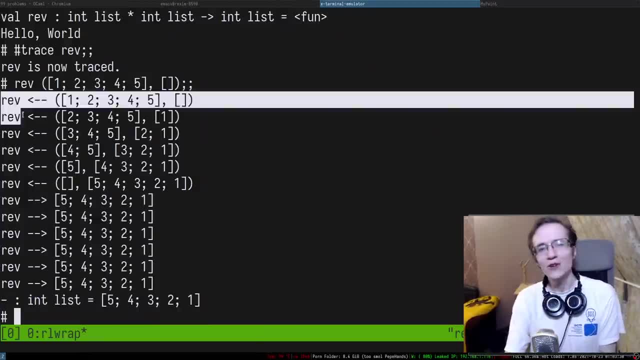 So let's reuse this entire thing, Let's trace that thing one more time And then do it like Perfect. You can now clearly see the whole dynamics of the language, You see? So here is the first argument. Here is the second one. 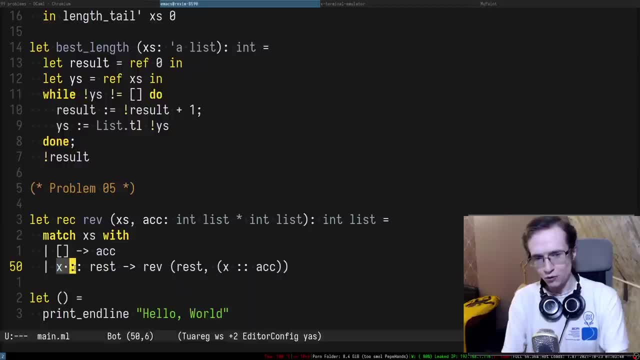 Right. So in here, on each iteration, we chop off the first element from the axis and we add them to the accumulator, And once we reached the end, we just return the accumulator. So look, Here is the list. We take one and push it to the accumulator. 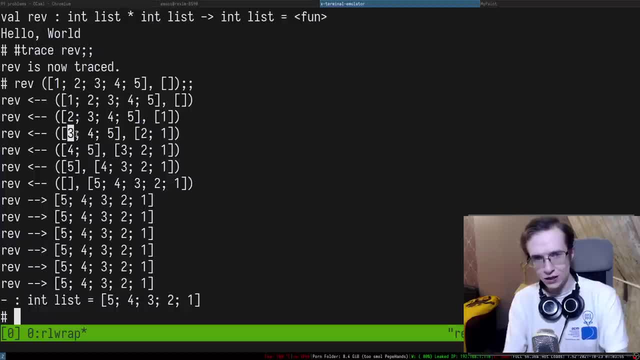 Then we take two, push it to accumulator Three, push it to accumulator Four, and until this thing becomes empty. And as soon as it becomes empty we return the accumulator. So this is how we reverse it. So I really like that. I can actually visualize that process. 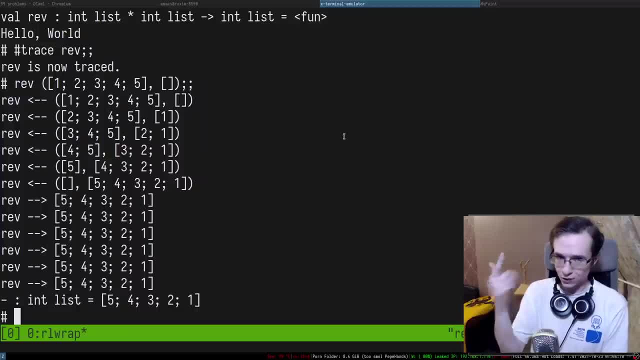 because this is how I see that in my head when I'm writing this kind of recursive things. But it's kind of difficult to explain what's going on here And I'm really glad that with the trace I can at least show what the hell is going on. 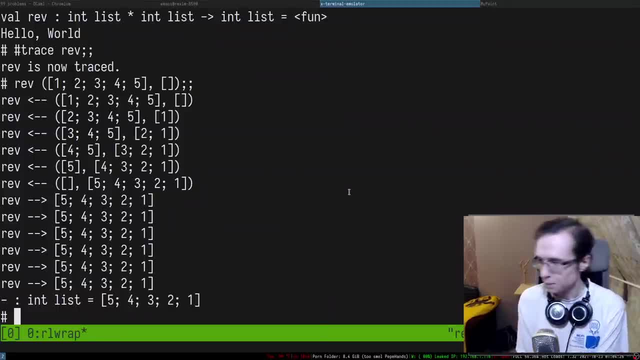 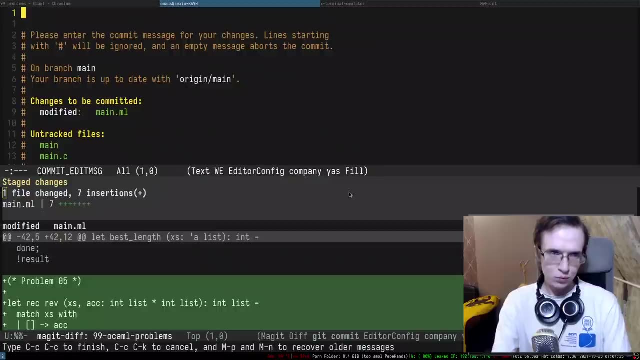 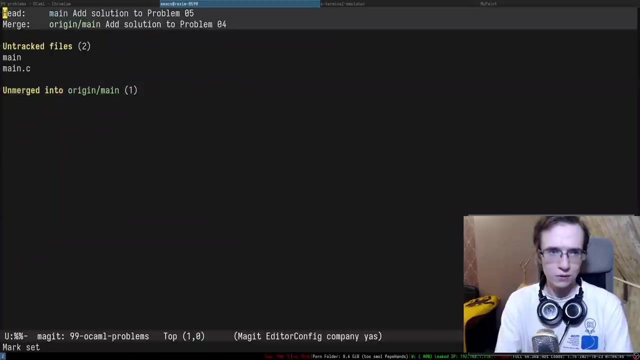 This is actually very cool, So, yep, So yeah, that's pretty cool And I'm going to do a committee, committee And then push, push, add solution to problem 05.. And I'm going to push that right into the repo. 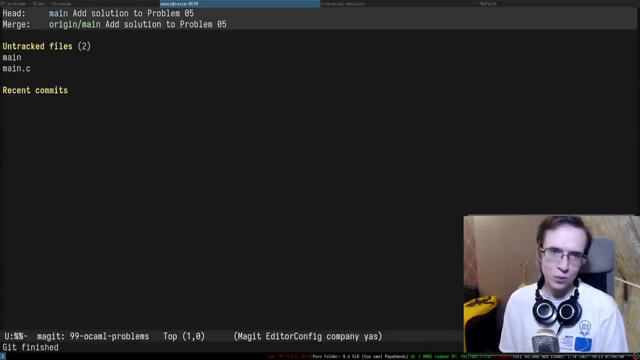 Okay, so I'm already a little bit tired. already We managed to solve five problems today But, to be fair, majority of time we were primarily discussing functional programming and different concepts in functional programming and optimization and stuff like that. So today's stream was not about solving these problems. 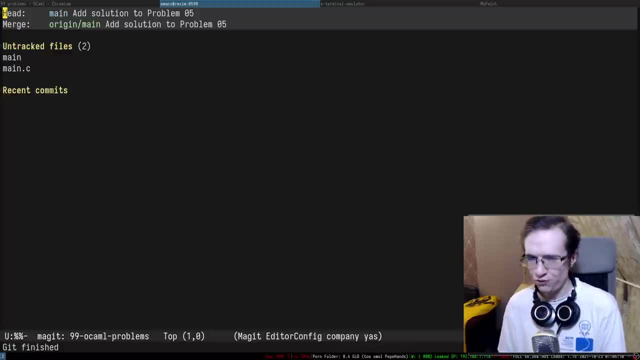 but more about discussion of functional programming, which I find to be very productive. I think today's stream was very productive and I hope it was very educational for people who only get into functional programming. All right, So I guess that That's it for today. 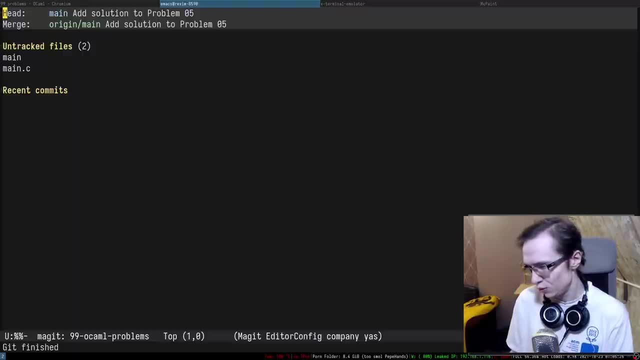 Thanks everyone who's watching me right now. I really appreciate it. So we're going to have more Porth streams in the future. So it's just like a- you know, random chill stream to get like a break from Porth. 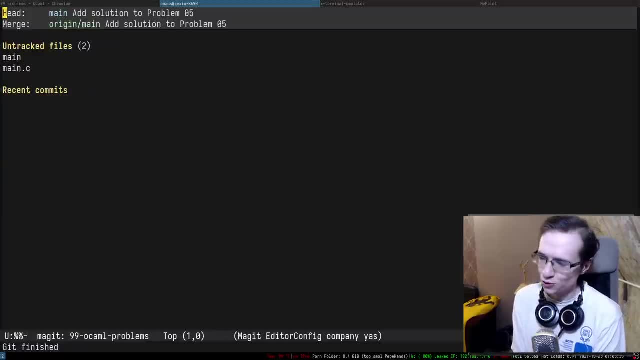 And then, yeah, I'm going to go. Thanks everyone for watching. Really appreciate that. Thank you for all of the subscriptions, donations and bits and stuff like that. Especially appreciate that. And let's maybe rate somebody because we got rated. 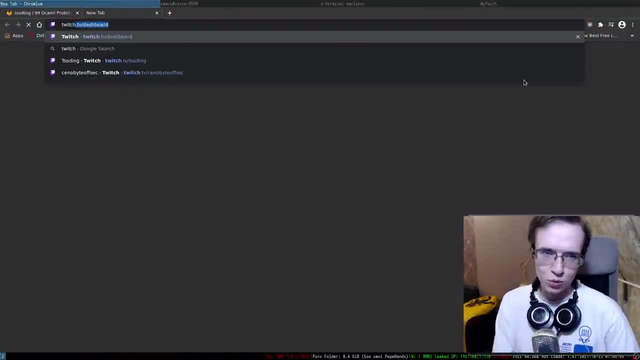 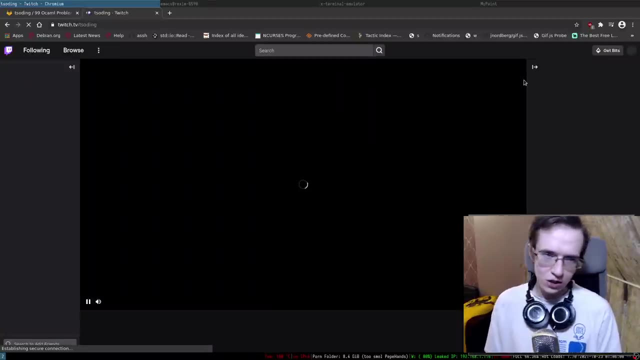 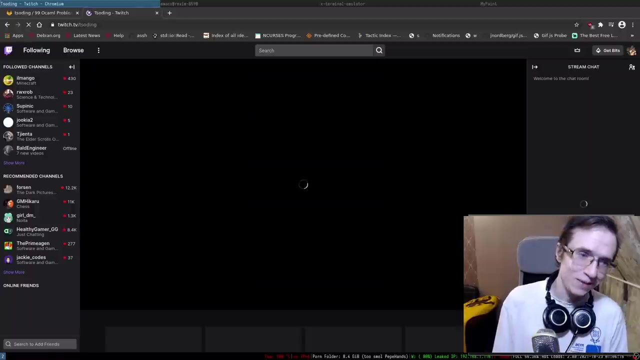 By Mr Provod, So maybe we want to rate somebody back. So is anyone streaming any functional programming on the software development section of Twitch? Okay, Okay, So we already rated Supinix, So maybe we can find somebody else. 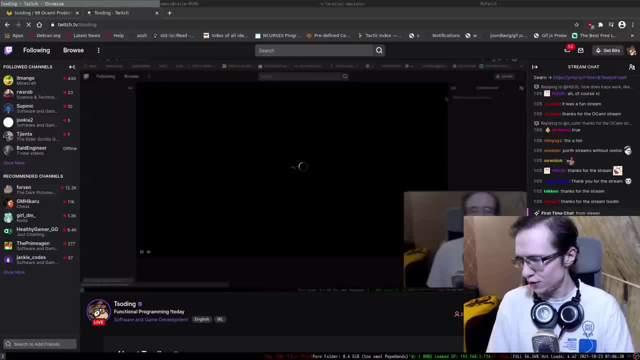 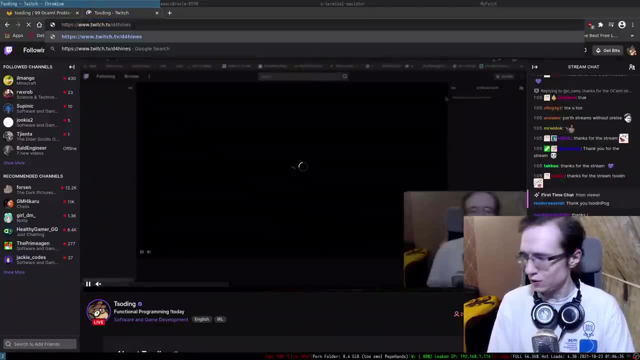 D4 Highness, I guess. So who's D4 Highness? Is that somebody who's doing functional programming? Are they doing functional programming? If they're doing functional programming, I'm actually down to rate them. Recursive Twitch: Yeah, it just goes recursively. 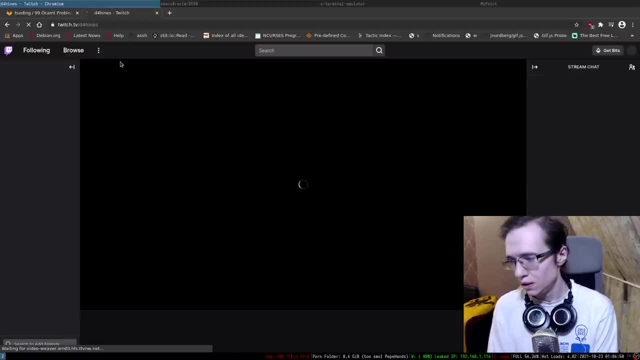 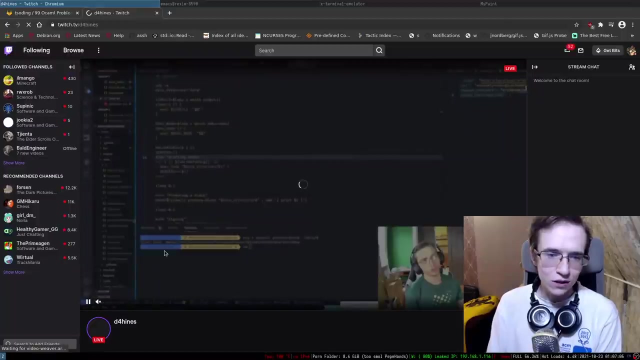 Just broke my tea, The fuck. It makes it really painful to rate people Like holy shit. So looks like they're alive, I hope. What are they doing So? what is this language? I don't recognize this language. 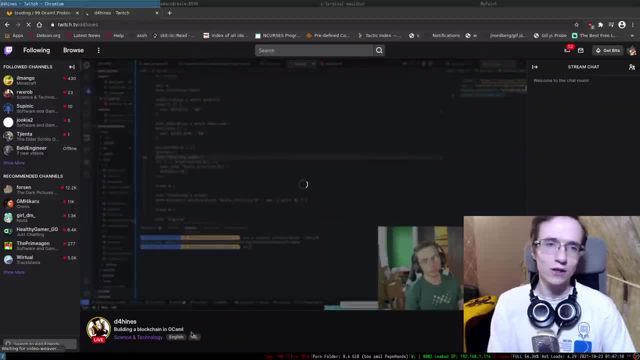 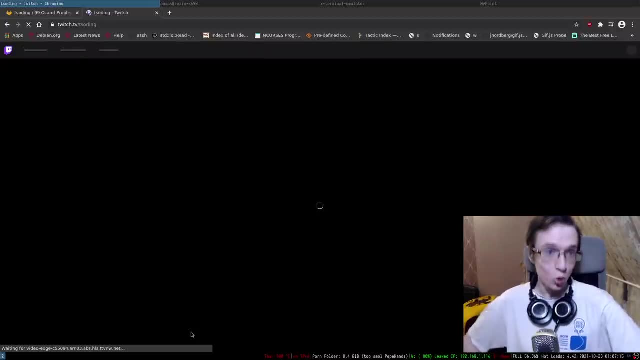 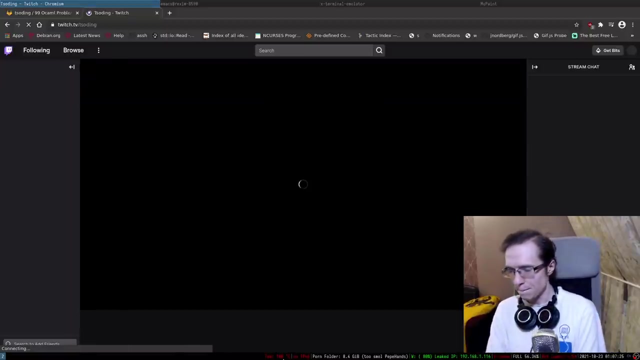 It's a shell script. Oh, building blockchain on a camel. Okay, this is perfect. Let's actually rate them. Okay, Blockchain on a camel- Holy fucking shit, Mine got un-be-fucking-livable. All right. I wish Twitch was a little bit faster. 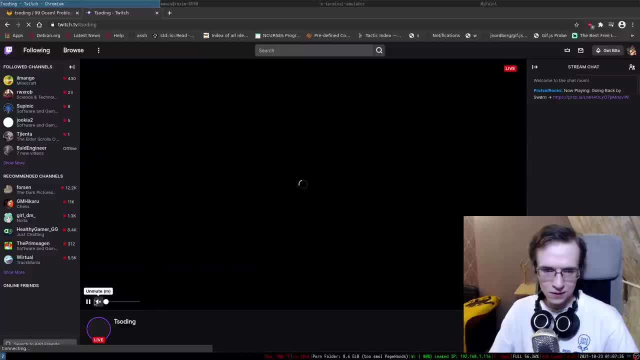 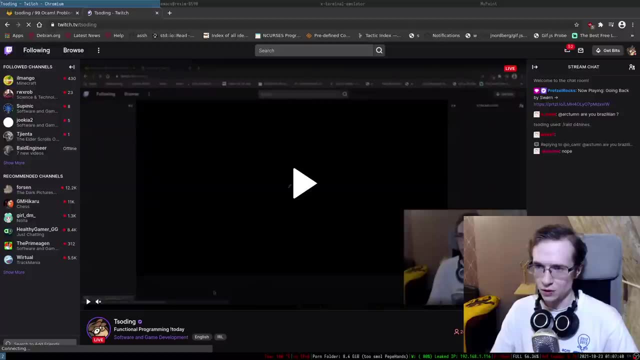 Cool, I already pressed the rate command and it's still being slow. Come on, you can do that Twitch. come on. Okay, I believe in you. It's already showing, but it doesn't show me the button yet. 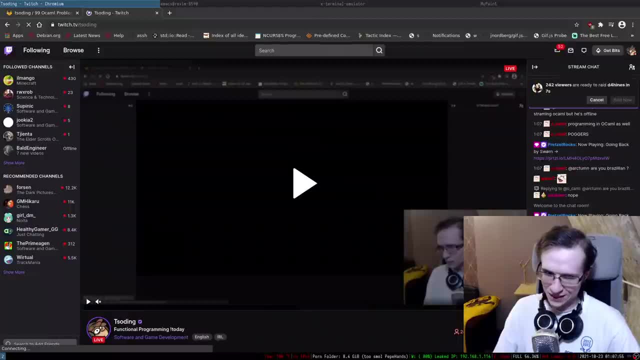 That's how slow it is. All right, Get ready for the rate, boys and girls. Get ready for the rate, And I see you all next time. See you all next time, Love you all.